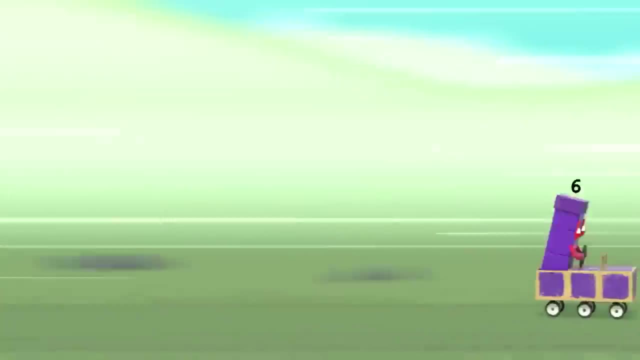 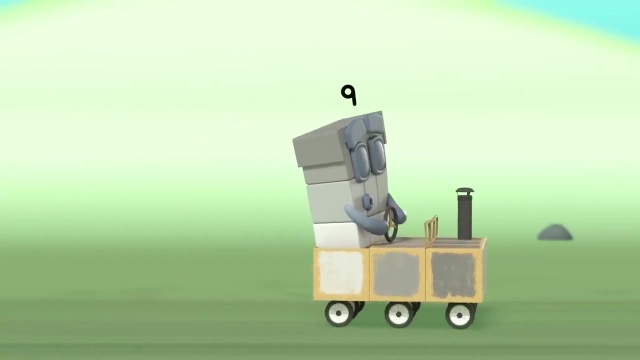 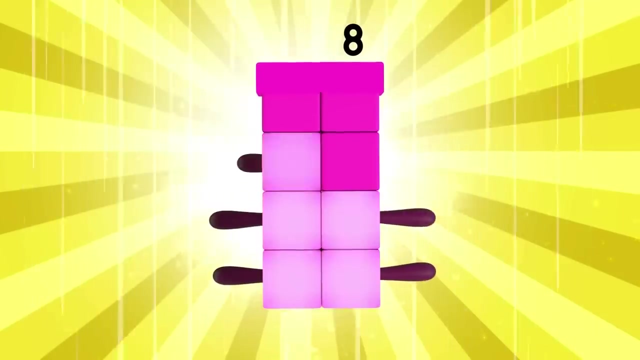 Nice day for it. And what makes it really surprising is that nine's in last place too. Well, next to last, Keep pedalling, Ron. Octoblock Race One, two, three, four, five, six, seven, eight. 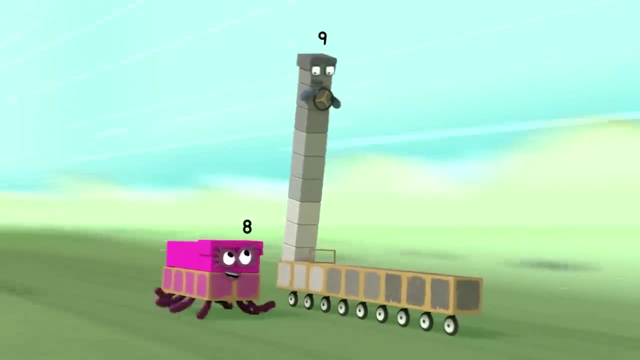 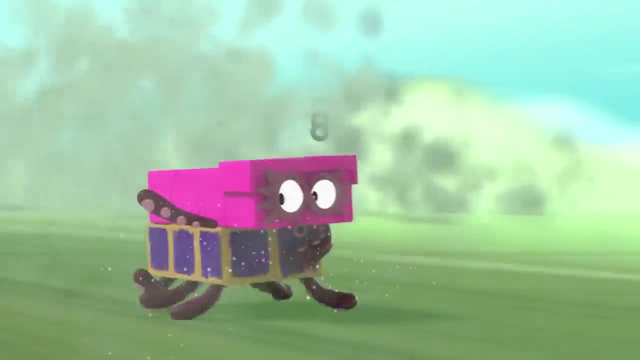 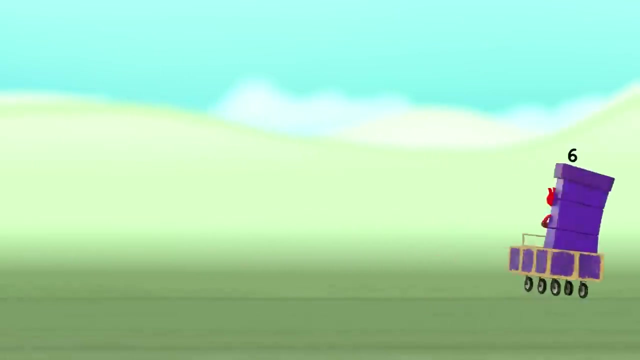 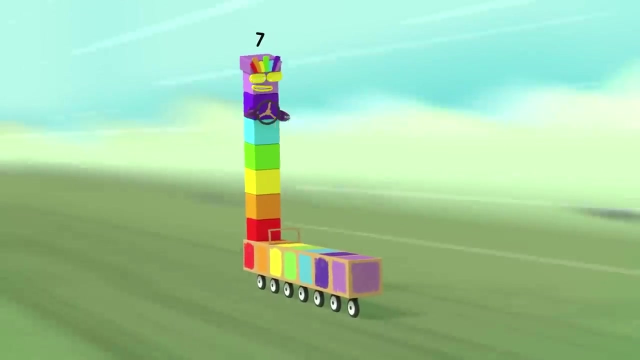 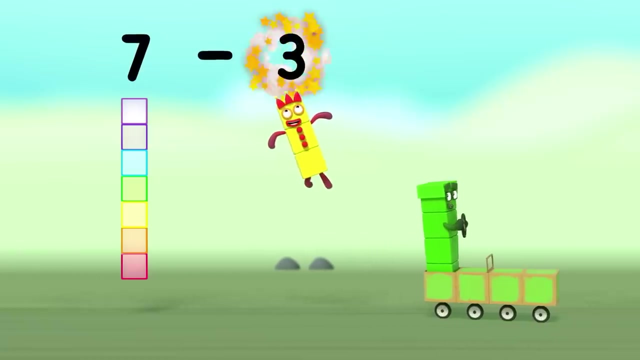 Great Eight's in trouble. Those two quadroblocks are about to go. Oh, Eight Minus two Equals six. Look out, Phew, That was lucky. Ah, Oh Oh. Seven Minus three Equals four. 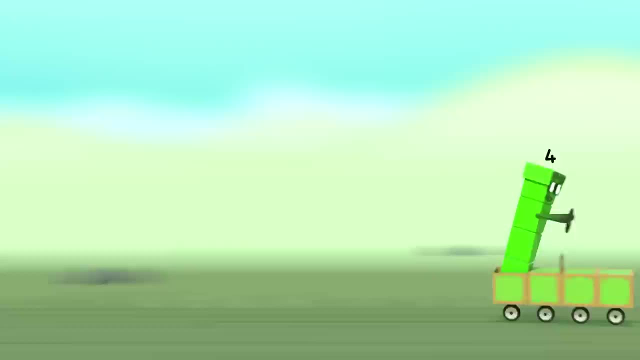 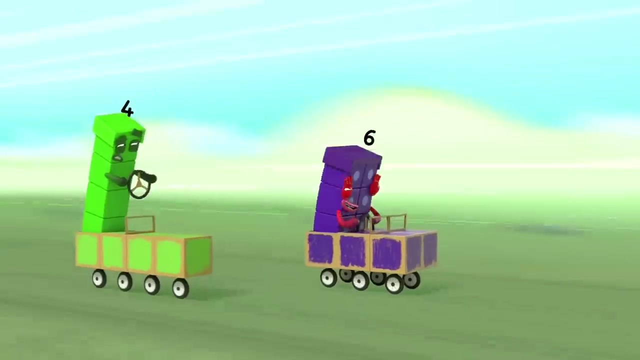 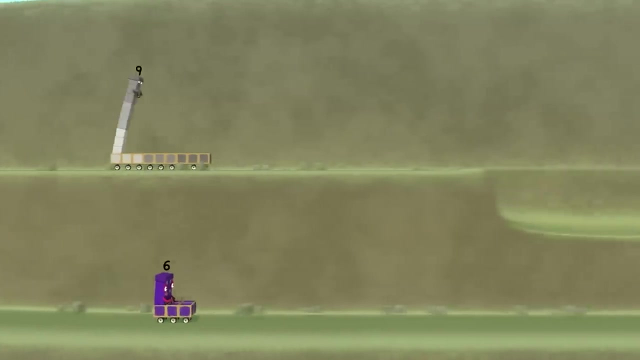 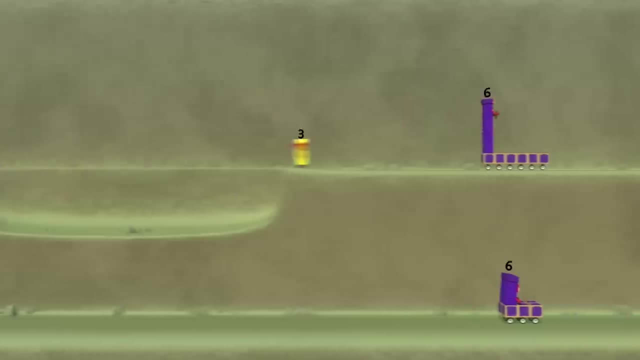 Mind that dip Nine minus three equals six, And the double dips, Six minus three equals six. Nine minus three equals six, And the double dips, Ah Minus three equals three. And what a close shave for a nine Six, cutting it fine there. 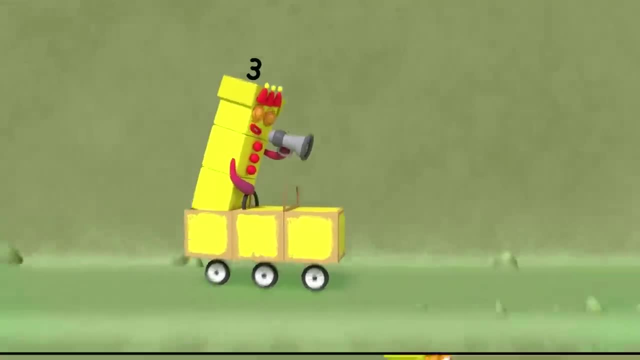 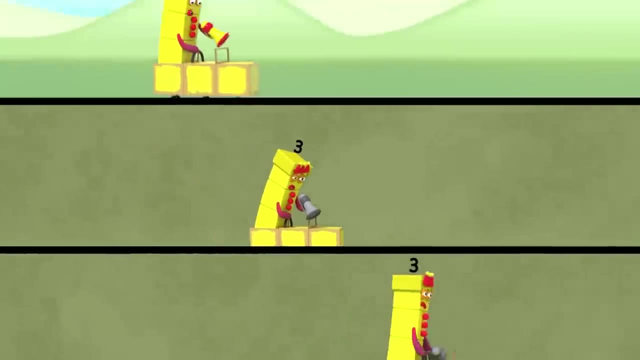 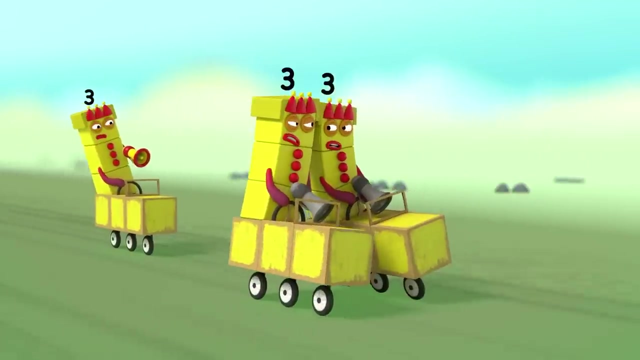 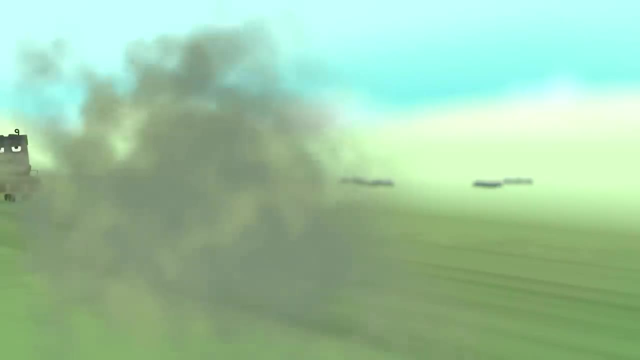 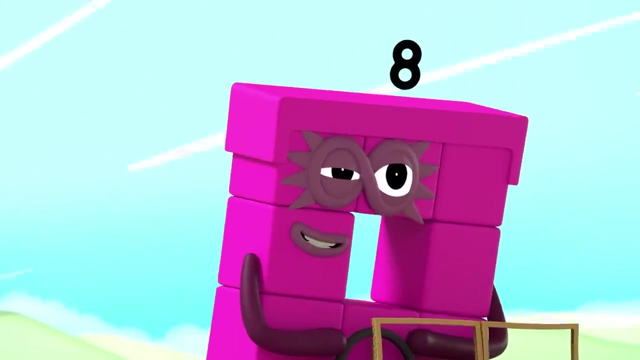 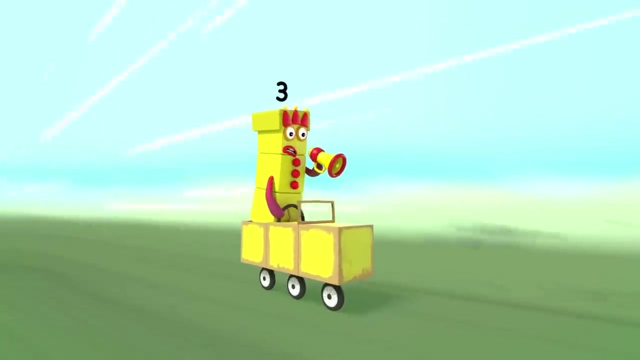 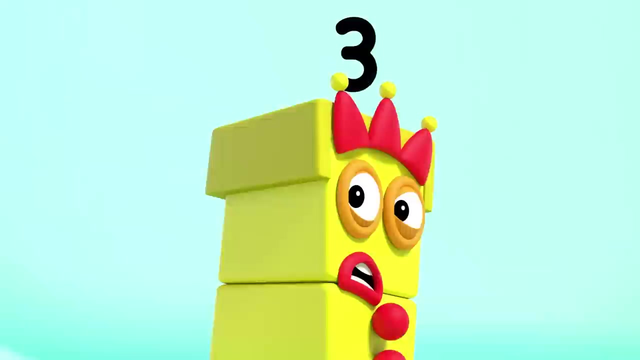 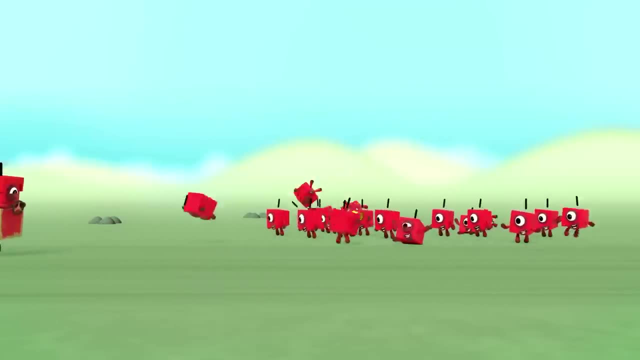 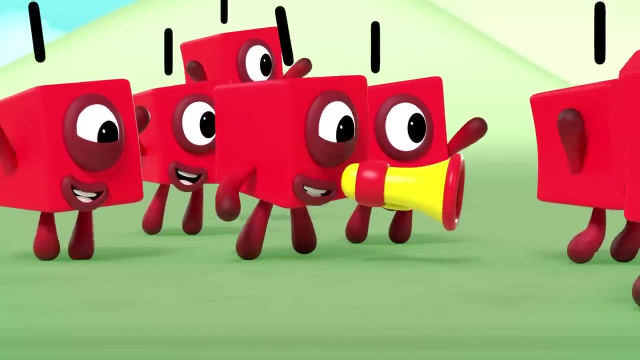 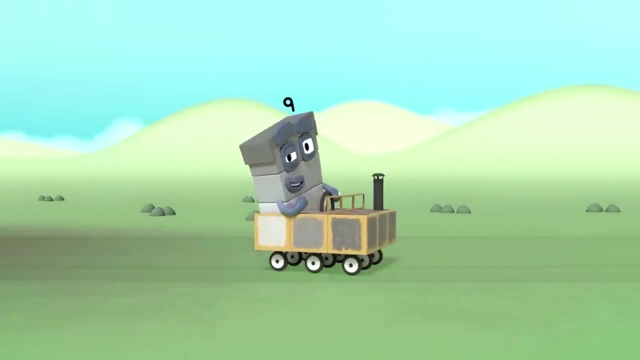 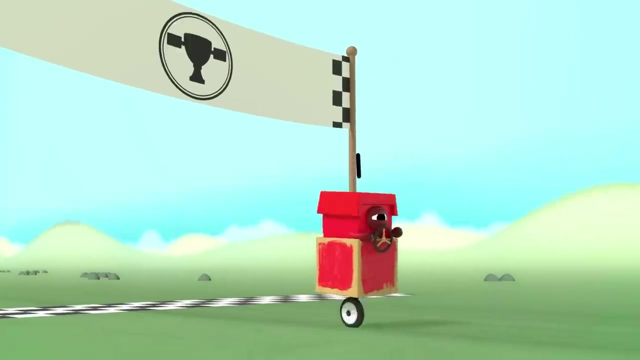 Octoblock coming through, Uh-oh, Uh-oh. And it's one in the lead, followed by one, But here's one coming up on the inside. Nine waltz sequels, Nine, Nice day for it. I'm first, Oh yeah. 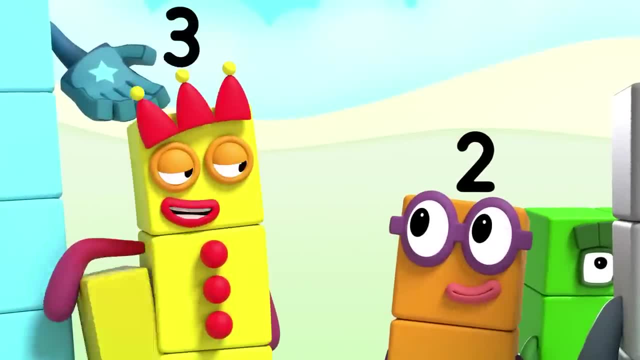 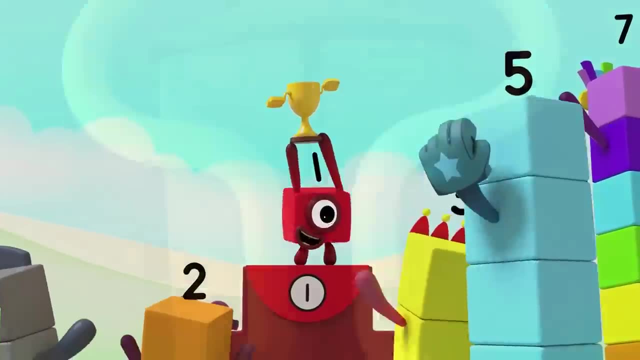 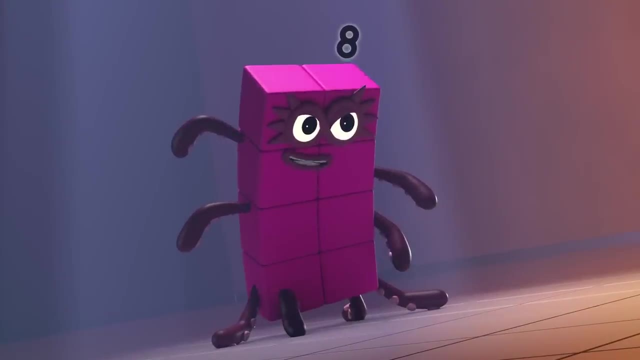 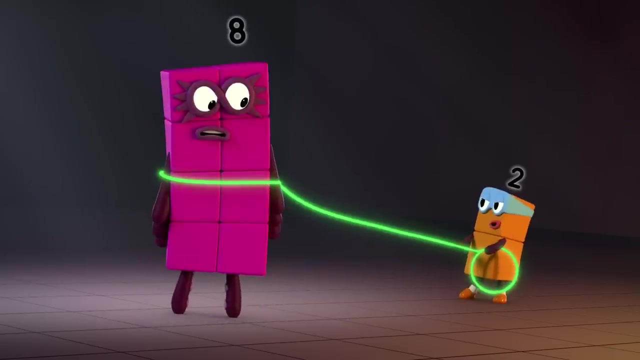 Well, I said only one can lift the trophy, and I was right. Surprise, surprise, custard pies. Your days of naughtiness are numbered. terrible twos, One, two, three got you Octoblock break. That rope is made from pure. 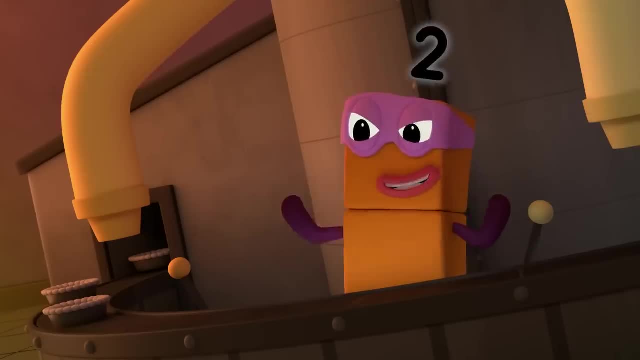 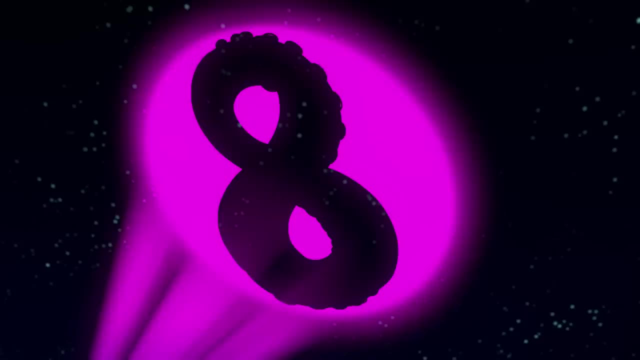 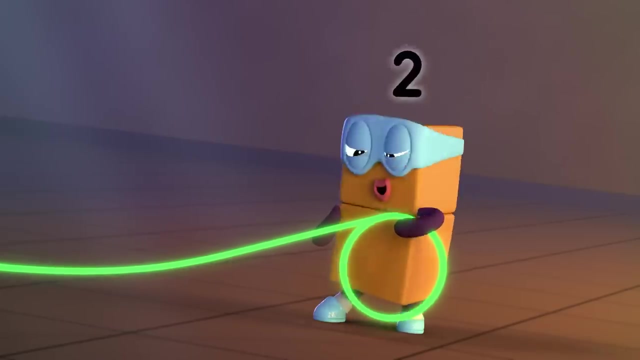 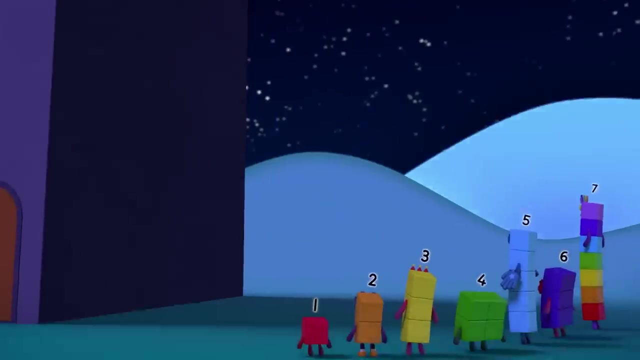 Oh, Octonite, your powers are useless? Maybe so, but I can still do this. The Octo-Signal. My friends will be here any moment And they will fall straight into our troublesome traps. Don't be so sure. Octoblock needs us. 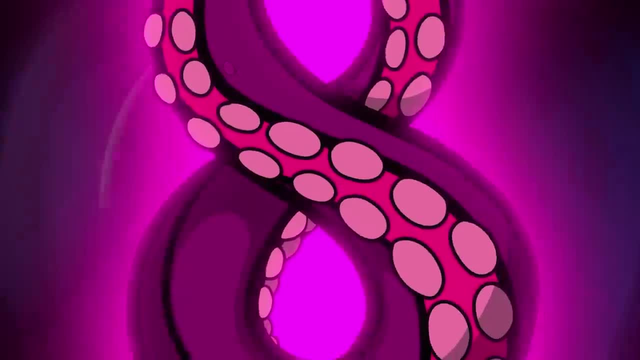 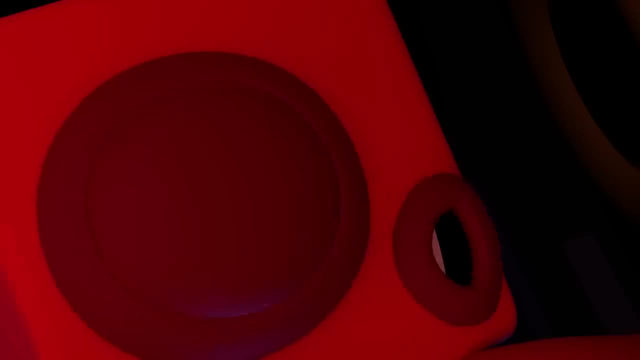 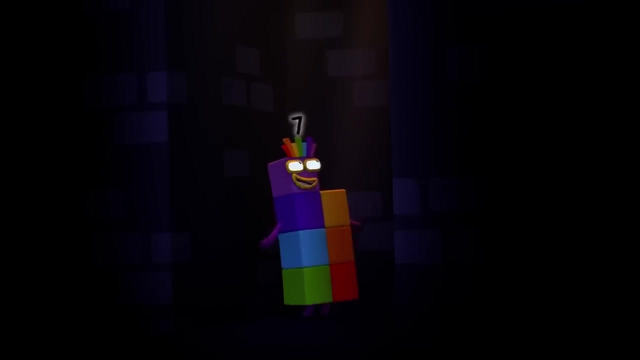 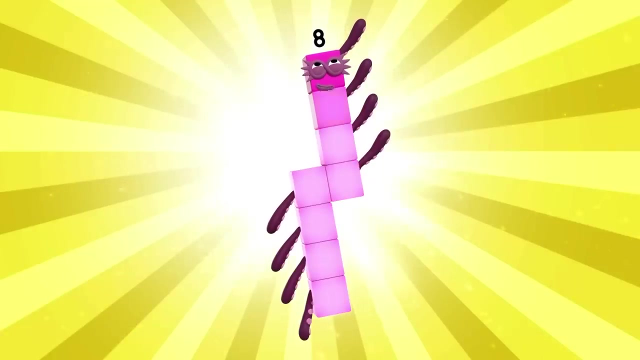 Splitter in here. That wasn't very lucky, But that was: Seven plus one equals Eight Octoblock. leap One, two, three, four, five, six, seven, eight leap. Ha Ha Ha. 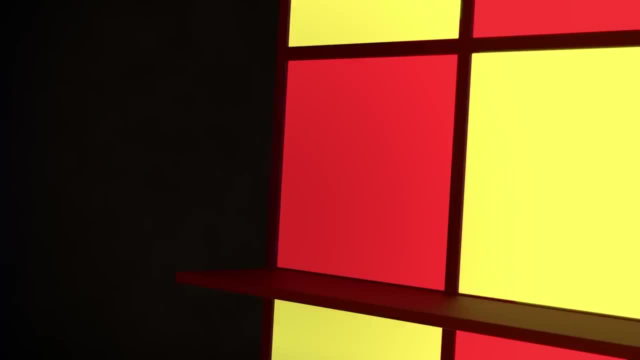 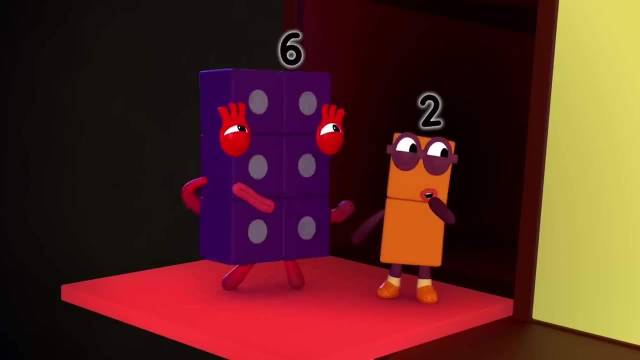 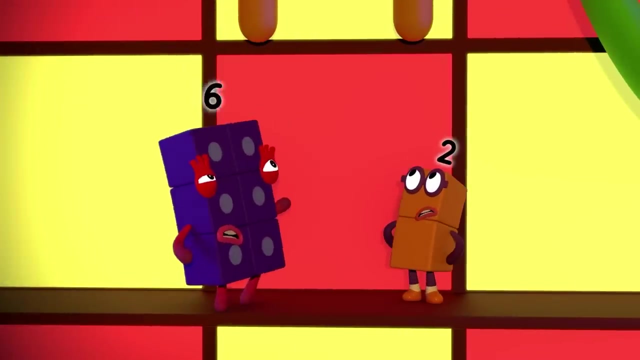 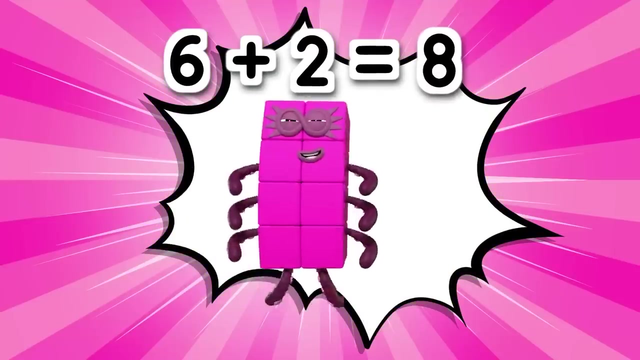 Ah, Snakes and ladders, My favourite game. Oh, let's play together: Two, One, two. hey, Someone's cheating. Six plus two equals Eight. Octoblock leap. One, two, three, four, five, six, seven, eight leap. 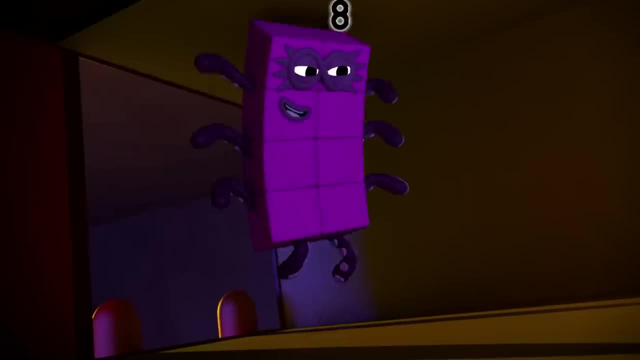 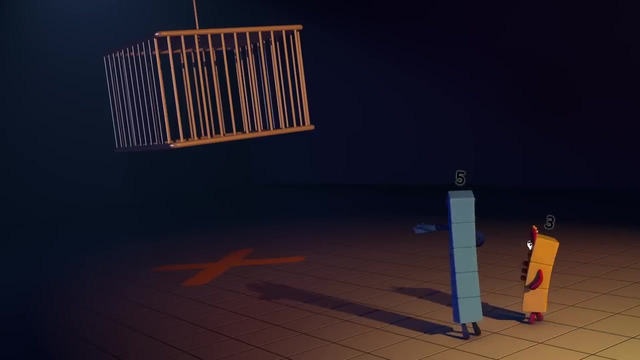 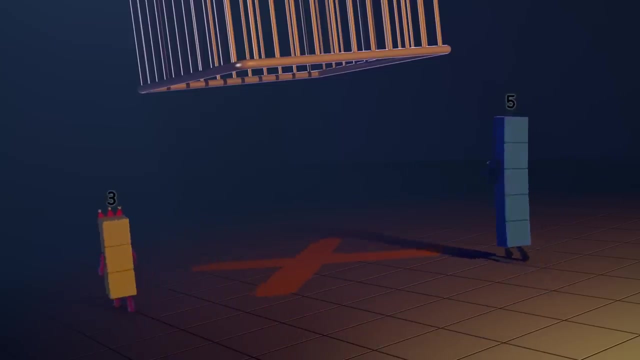 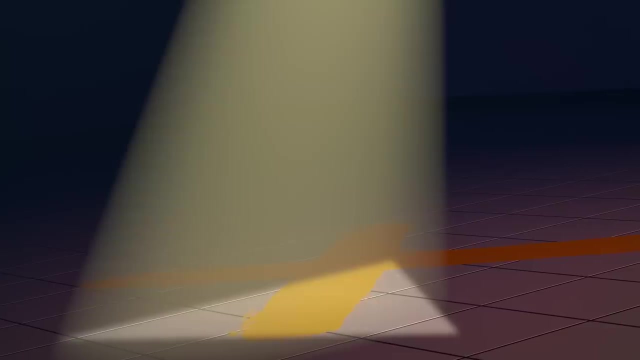 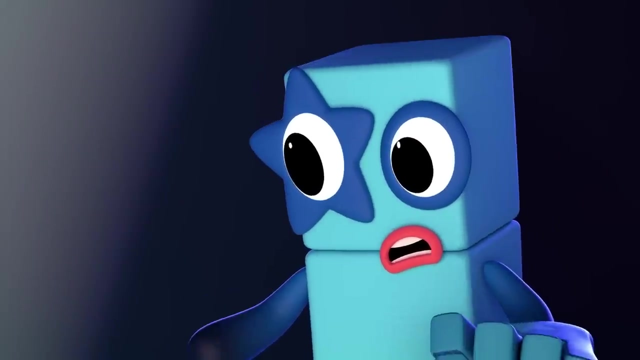 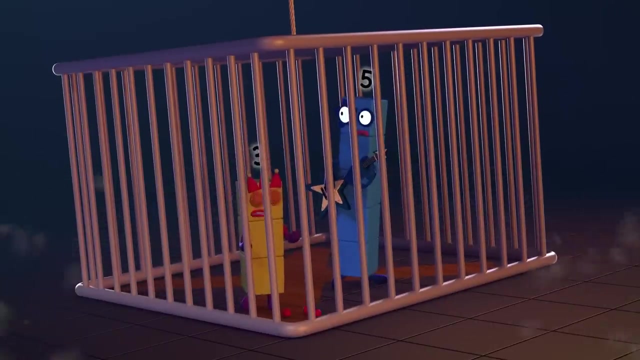 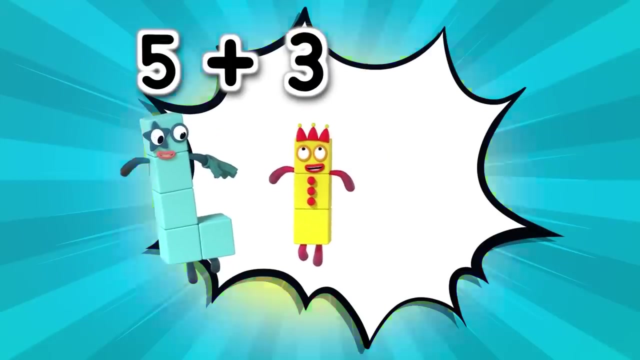 They won't catch us that easily. Don't walk under the cage. I could just resist it. three, Oh, I'm a star, I'm a star. Hey, I wasn't finished. Grand finale. Five plus three equals Eight. 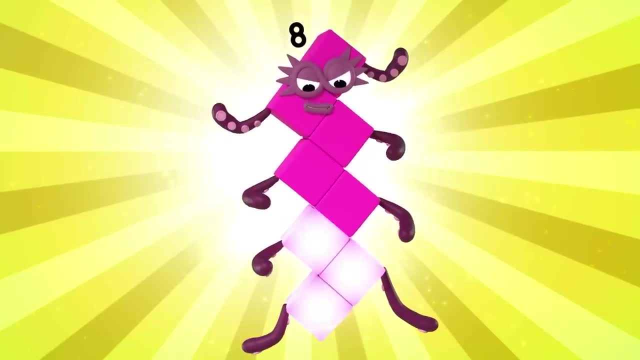 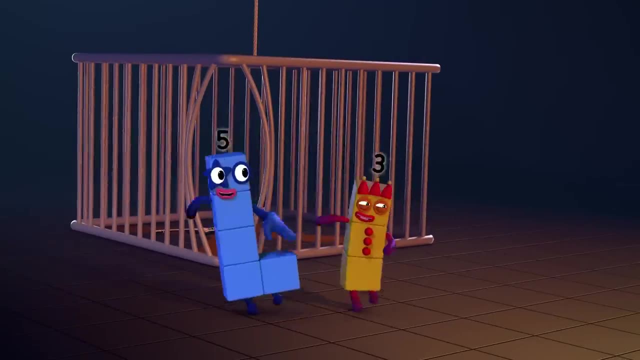 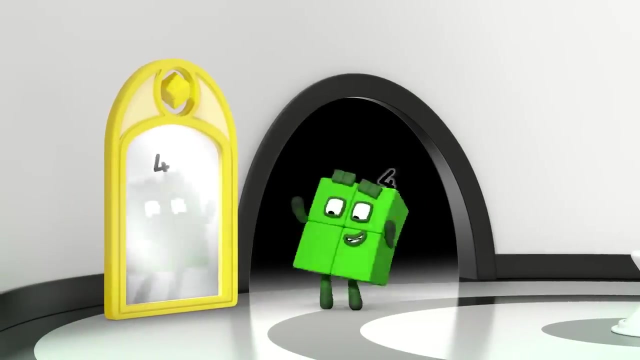 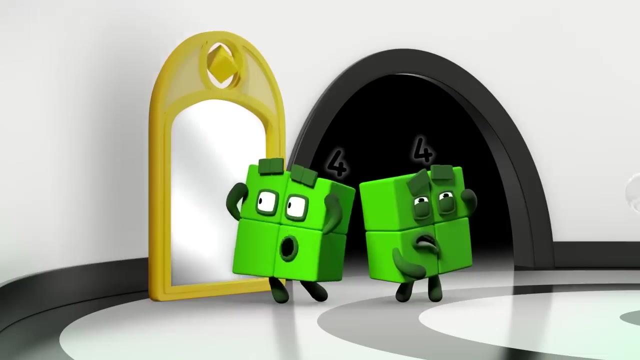 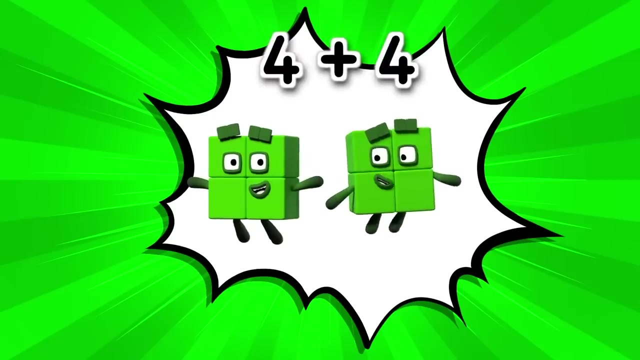 Huh, Octoblock 10!. One, two, three, four, five, six, seven, eight Burn. Hello, Hello, Ooh, round things, It's got us Four plus four equals Eight Octoblock. 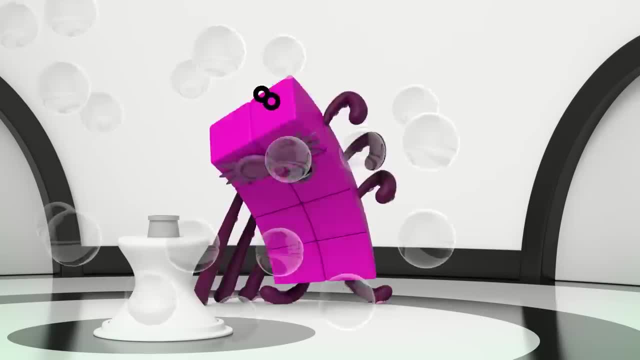 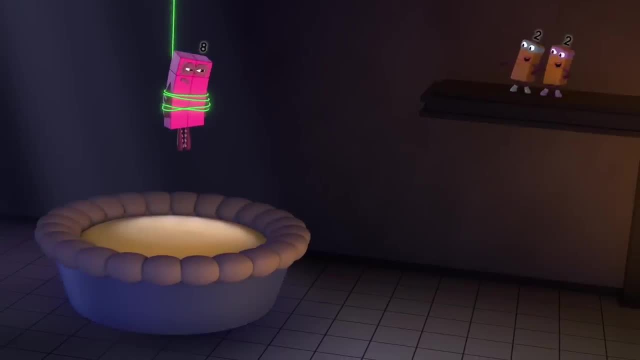 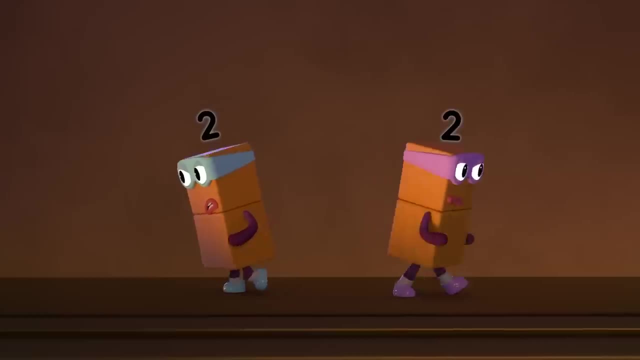 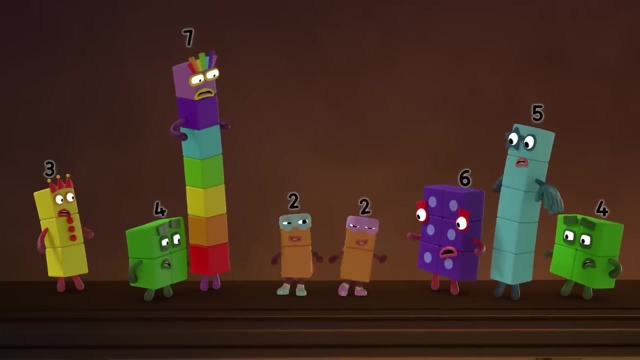 One, two, three, four, five, six, seven, eight, Pop, Prepare to be pied Spiderblock. Stop right there. We have you outnumbered. Maybe so, but we've still got a trick or two up our sleeves. 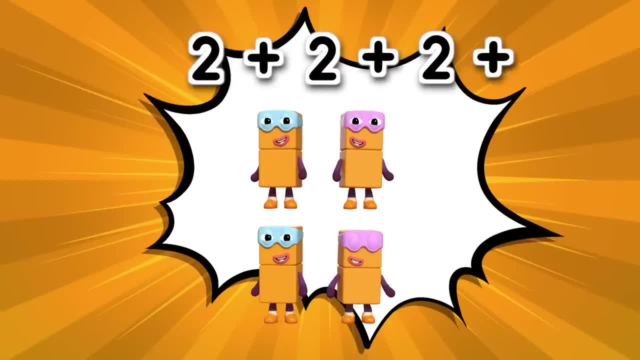 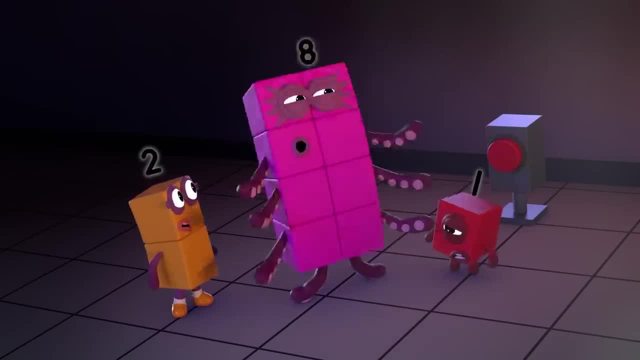 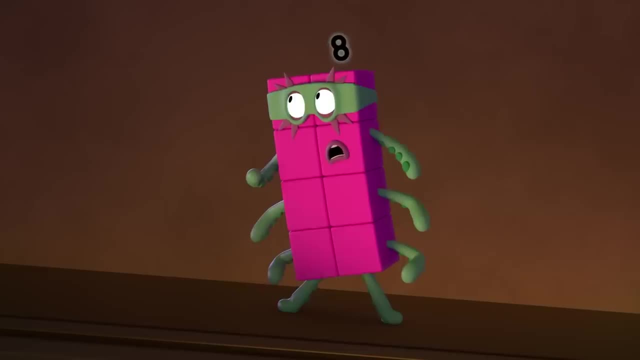 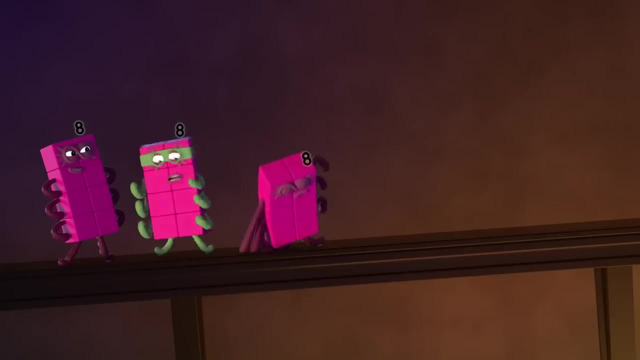 Two plus Go. Two plus two plus two Equals. Eight Ugh. Four terrible twos make one Octo-Naughty. You've met your match. Octoblock, Don't count on it. Octoblocks Assemble. 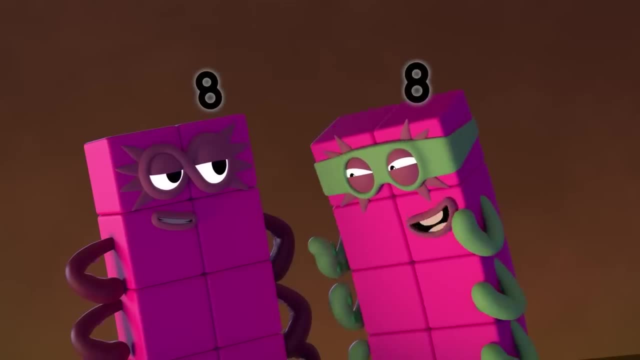 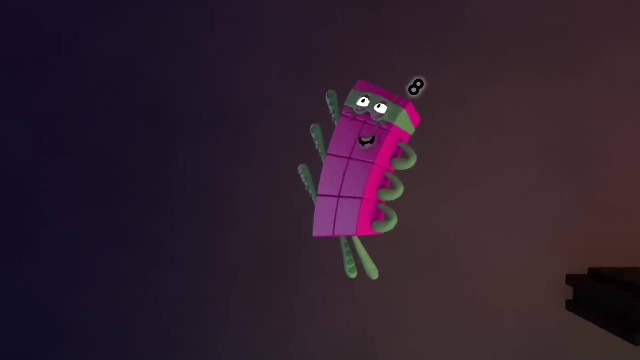 Your number is up. You'll have to catch me first. Octo-Naughty escaped oin' your牙 nail Escape Eight, seven, six, five, four, three, two, one escape, Uh-oh. 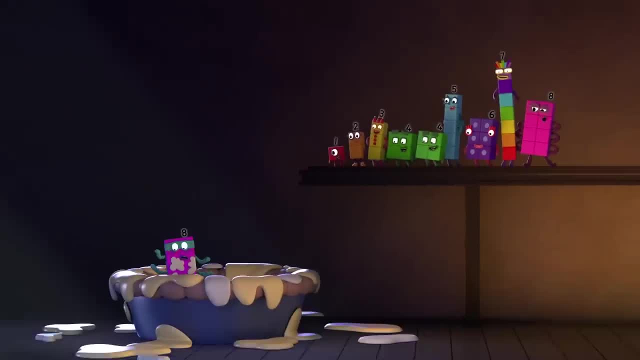 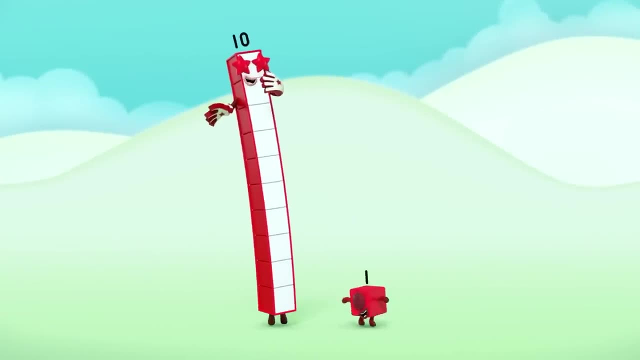 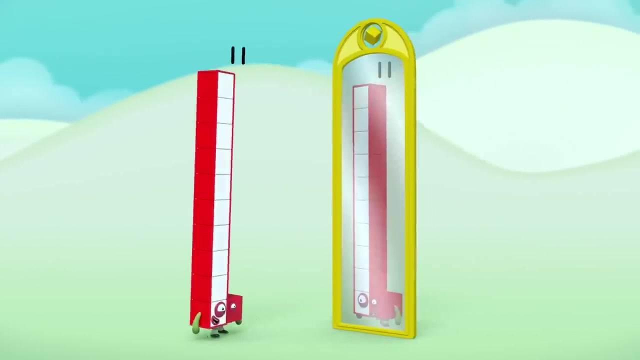 I spy with my little pie. a very naughty number. block Ten, Hello one. What shall we play today? Ooh, um, Hmm, What was that? Who was that? A new number? block Ten plus one equals eleven, Hello. 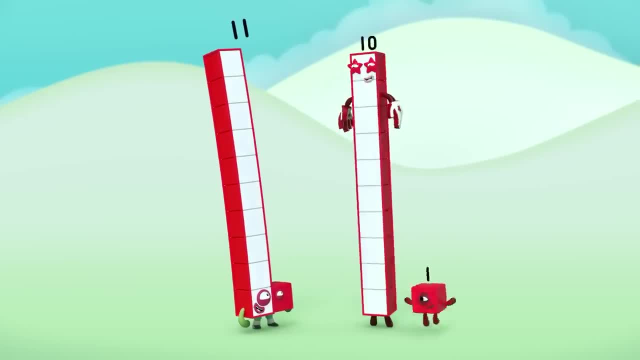 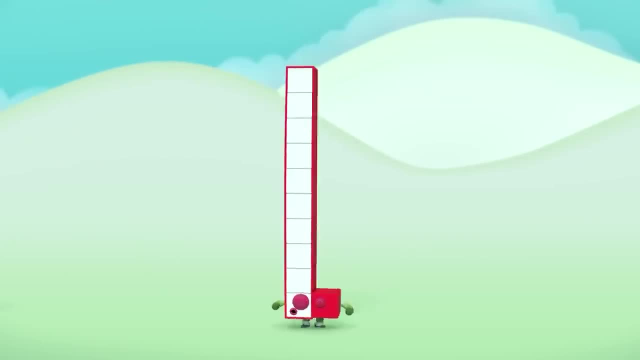 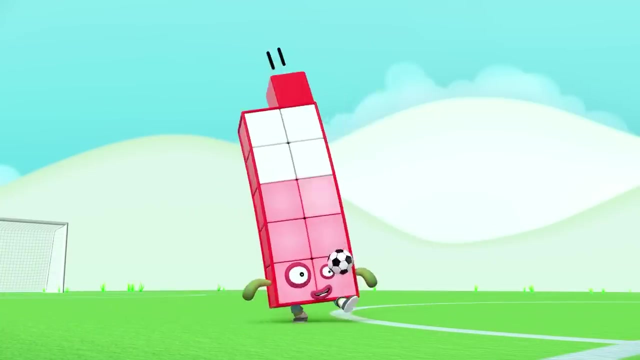 I'm eleven, So am I, And I'm ten and one. That's better, Ooh Whoa. One, two, three, four, five, six, seven, eight, nine and ten, And one more is eleven. 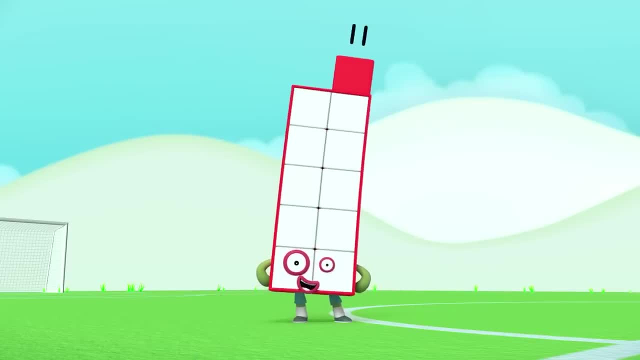 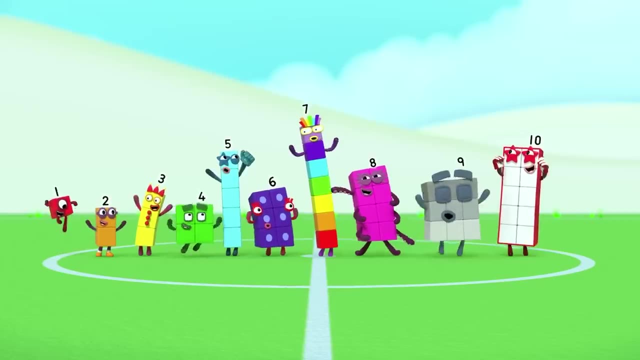 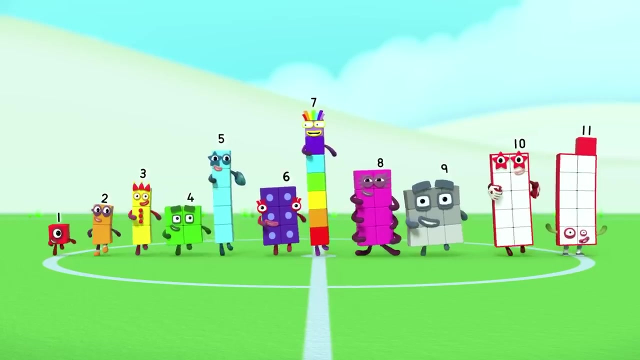 I am eleven And I love football. Wow, Let's play football. Hooray, Hooray. One, two, three, four, five, six, seven, eight, nine and ten. One more is eleven. We're on our way to victory. we're on a roll. 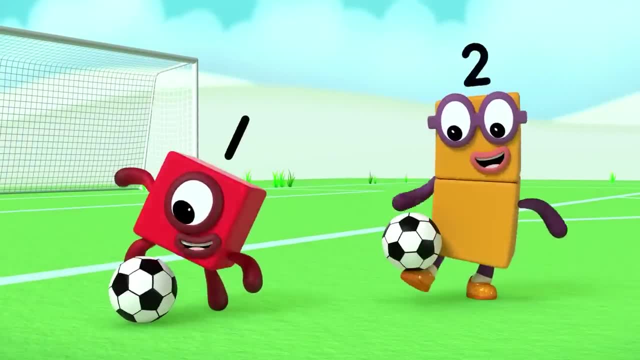 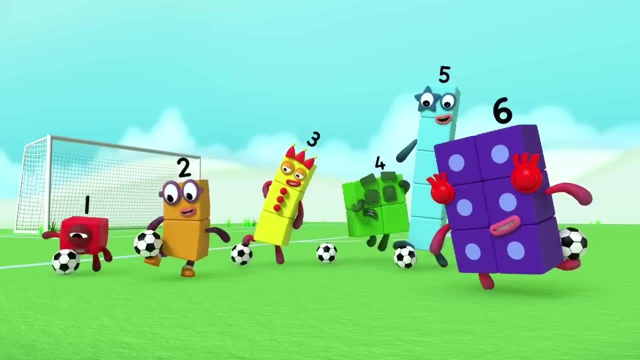 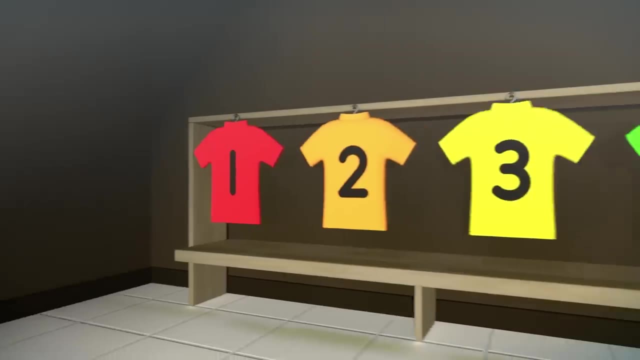 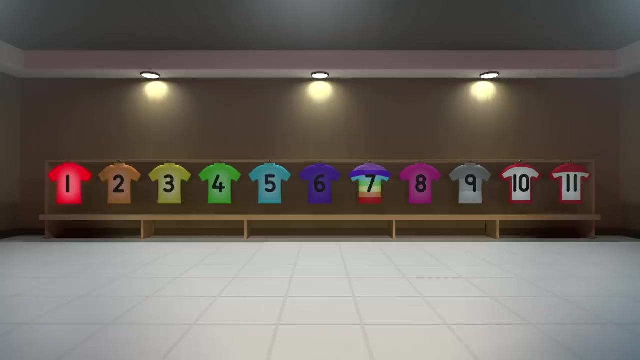 With ten on the pitch and one in goal. We will never be denied. We'll take it in our pride With ten and one, ten and one eleven on our side. Football shirts. football shirts And ten And one more. 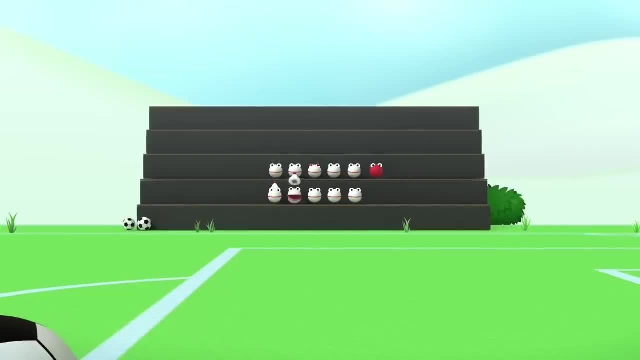 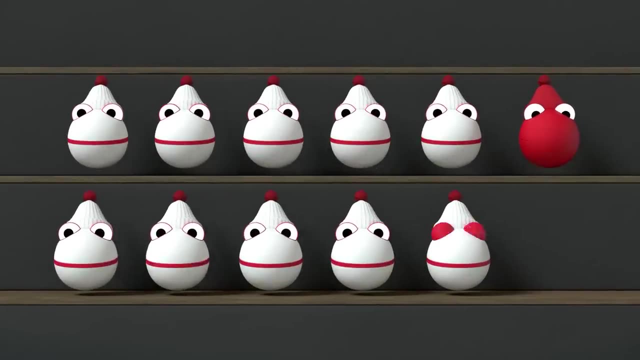 Is eleven. Hooray Bobble hats. Bobble hats One for every number. blob Bobble hats One, Two, Three, Four, Five, Six, Seven, Eight, Nine And ten And one more is eleven. 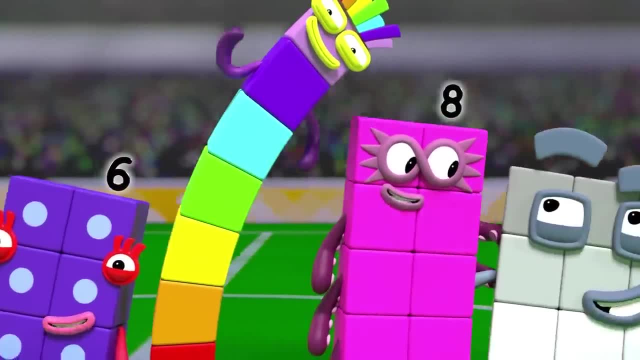 Hooray, We're on our way to victory. We're on a roll With ten on the pitch And one in goal. We will never be denied. We'll take it in our stride With ten on the pitch And one in goal. 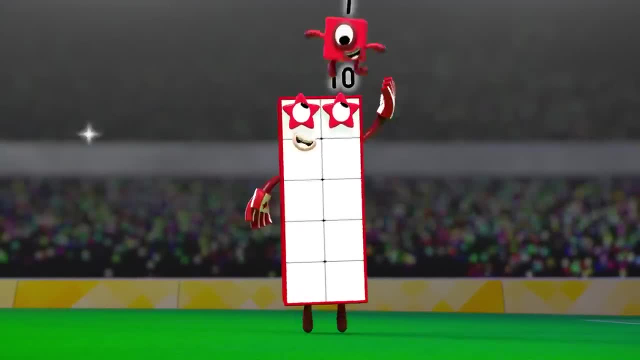 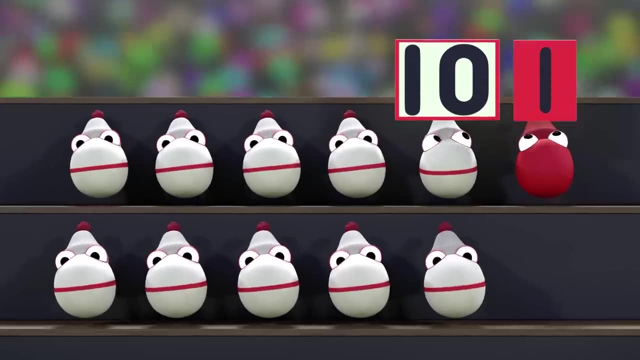 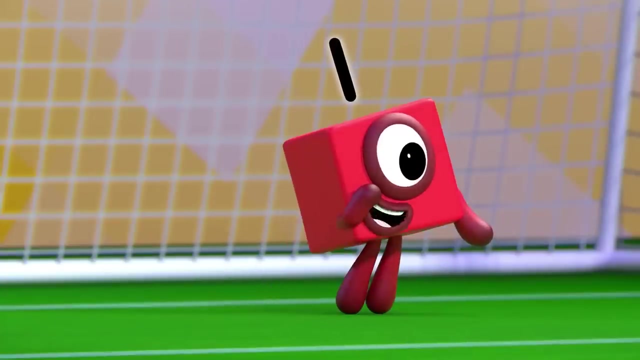 We'll take it in our stride With ten and one. Ten and one Eleven on our stride. One ten, One, one, Ten And one Eleven. One ten, One, one, Ten And one Eleven. The number blocks are out on the pitch for the big match. 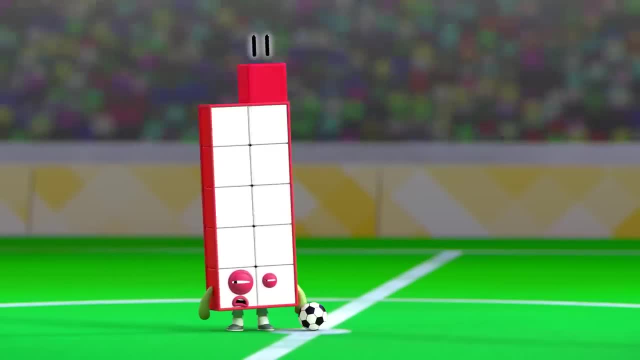 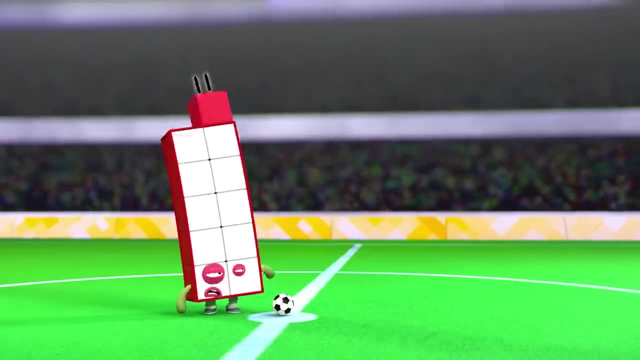 And their captain Eleven looks ready to lead the team to victory. Something's wrong. What can it be? I've forgotten something. The oven's on. The oven's on. The oven's on, But we don't think he knows what's going on. 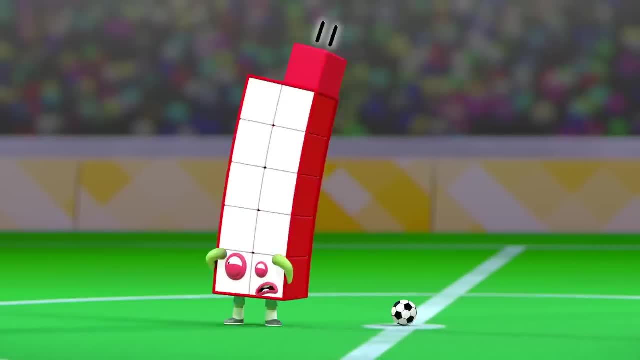 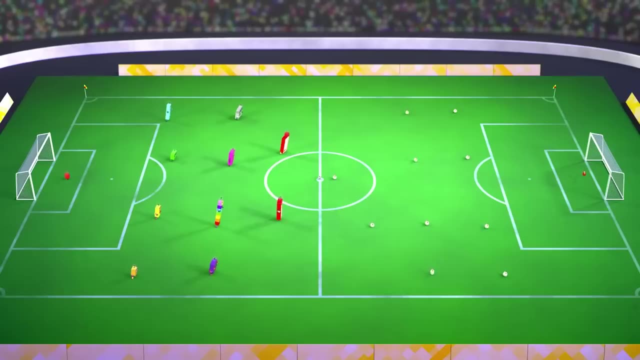 I think the aerlya has Speed. remainder No clue. Oh no, No problem, We could climb it up the pitch. It would be great There. Now that's it. You think you can beat us? Yes, We have the power now. 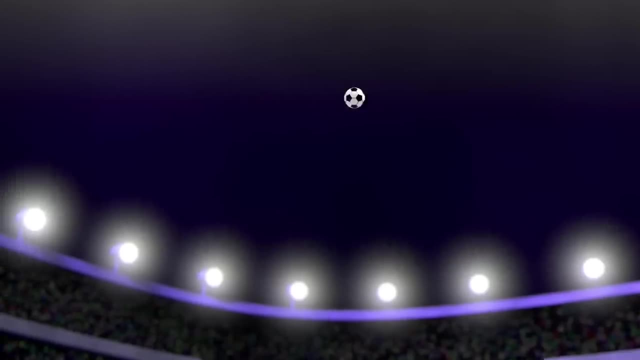 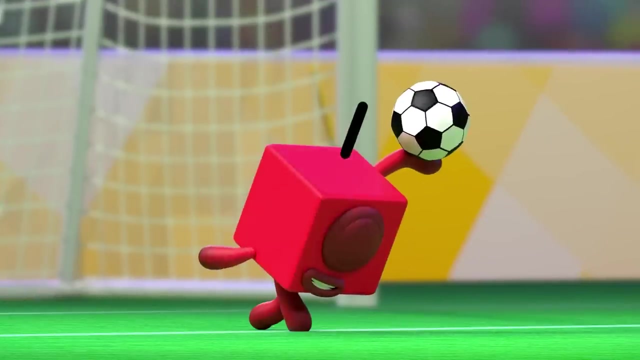 Oh, big fans. One sun in the sun. Big fans, Big fans. What's going on? Look, Only two flower children are getting married, Two and one. It's the release of the big Schnapps. They won't let you go. 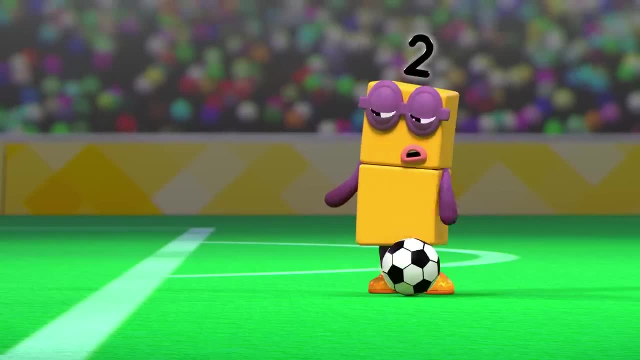 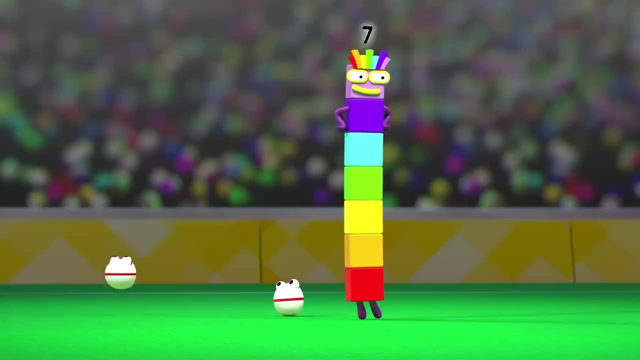 I can't. The Schnapps are coming to get them. They are here. It's a big ball. I'm going as fast as I can. The number Mega Balls is off. Four, five, six, seven, eight, nine and ten. 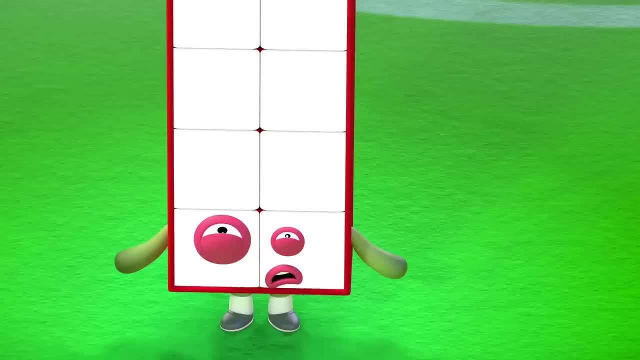 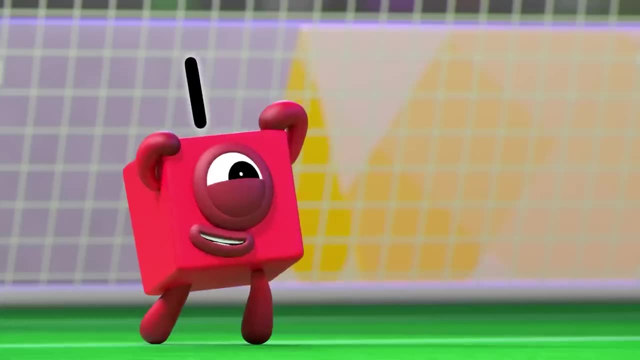 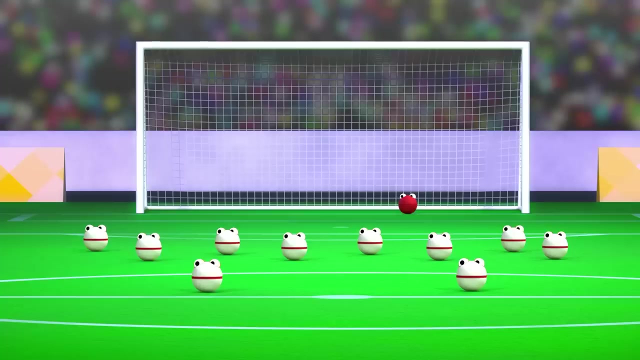 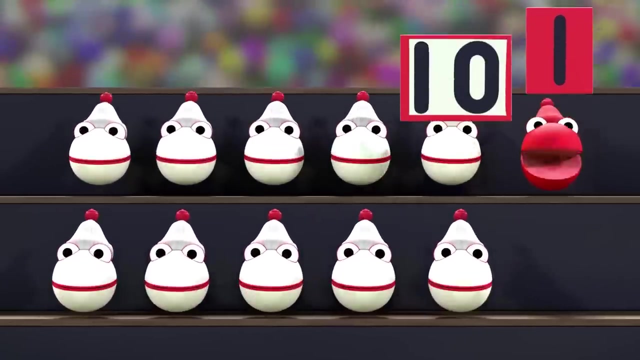 Now pause it to eleven. Ten passes, eleven seats for the header and, oh my, Splits into ten and one to reach the ball. Incredible, And It's a save. What a save. Ten and one, ten and one, eleven is the best. 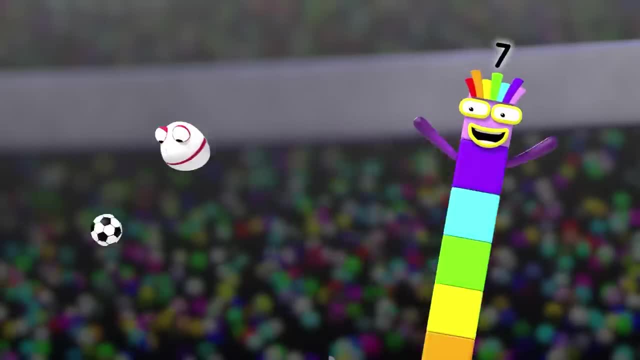 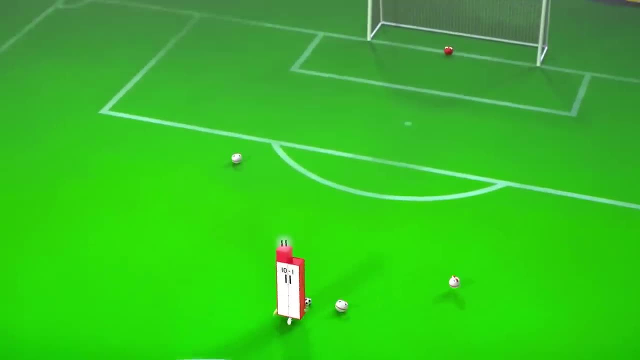 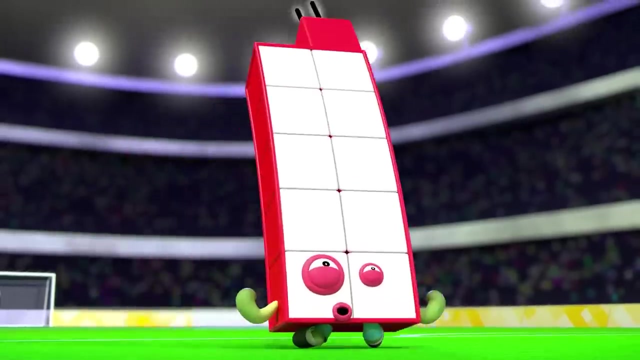 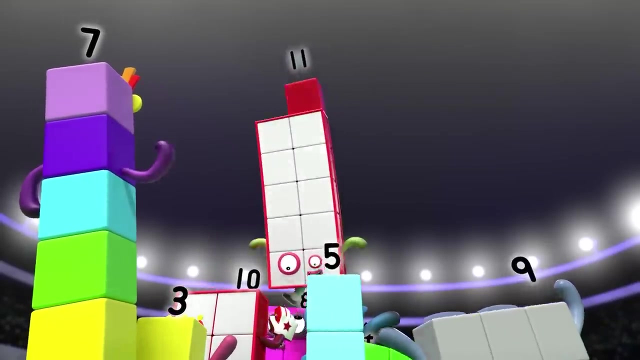 Number Blob passes to Number Blob. who finds Number Blob? And a lovely hitter there to Number Blob. Look eleven. Who heads it to eleven? And it's eleven, Eleven, Eleven, Yeah, Yeah, Yeah, Yeah. We're on our way to victory. we're on a roll. 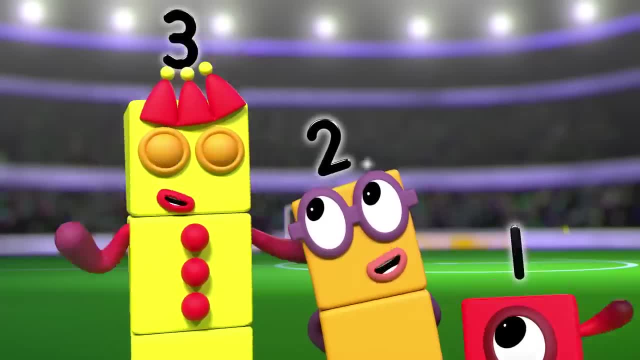 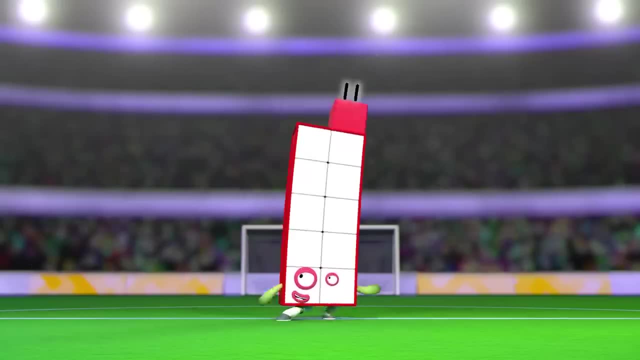 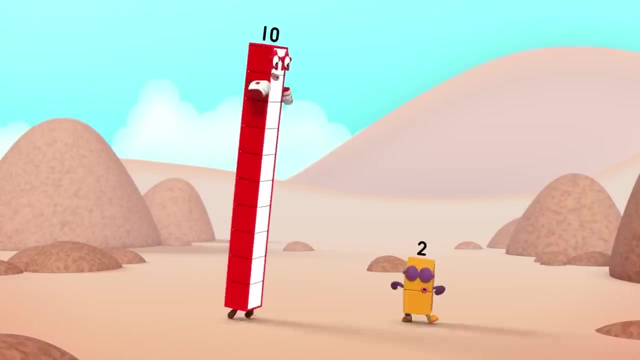 With ten on the pitch and one in goal. We will never be denied. we'll take it in our stride With ten and one, ten and one, eleven on our side. Ten and one, ten and one, eleven on our side, Ten And two. 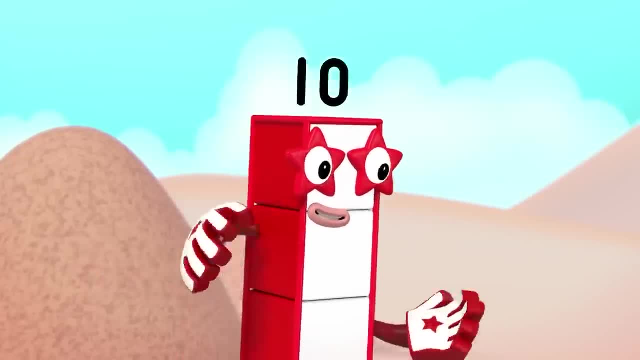 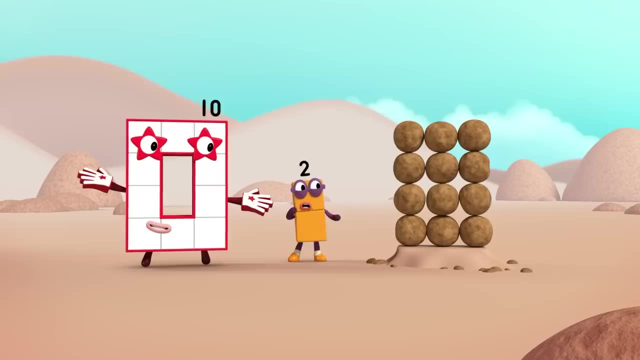 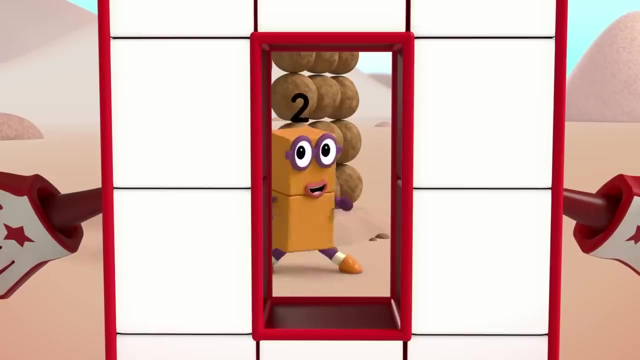 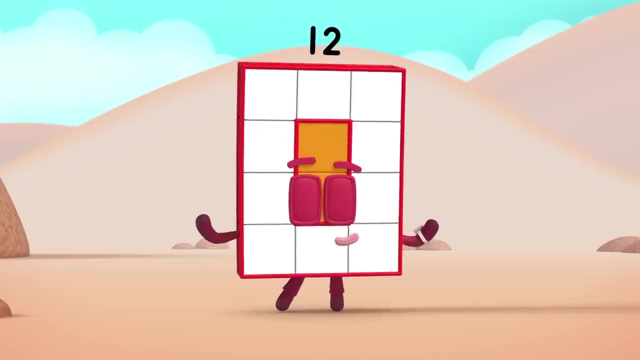 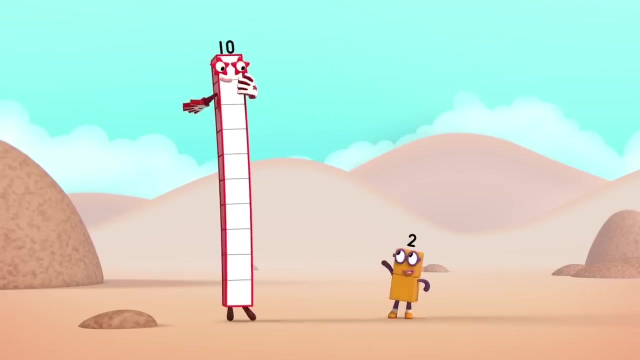 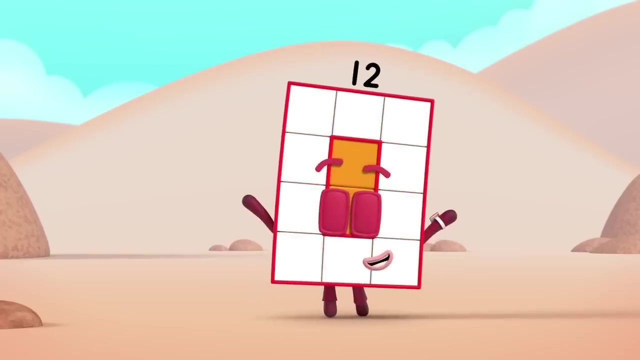 Ten And Oh, Look at that, Hey, What am I? A rectangle With a hole. Come on then, A whole new rectangle. I'm new, I'm twelve, I'm Ten And Two, I am 12, and I am a super rectangle. 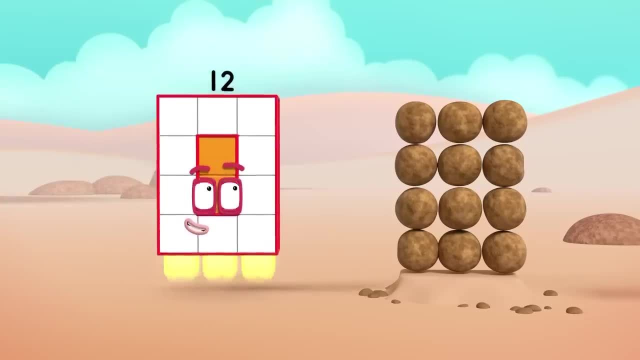 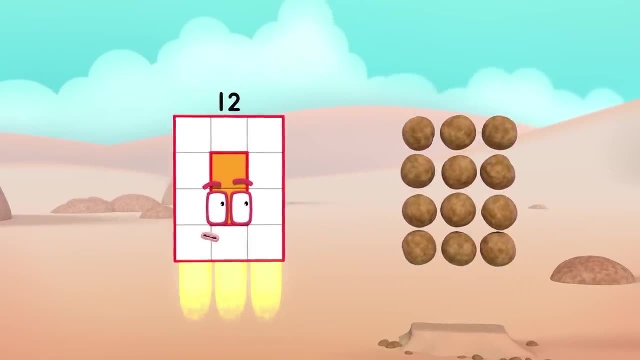 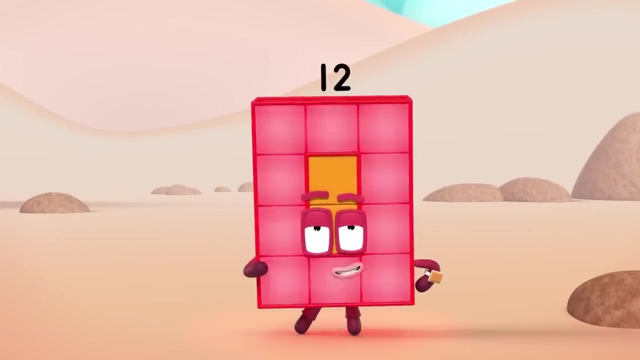 The rocks are in columns and rows. My blocks are in columns and rows. My blocks are in columns and rows And that's called an array- Array. Hey, I'm Rectangular 12,, I'm 10 and 2. I make arrays. that's what I do. 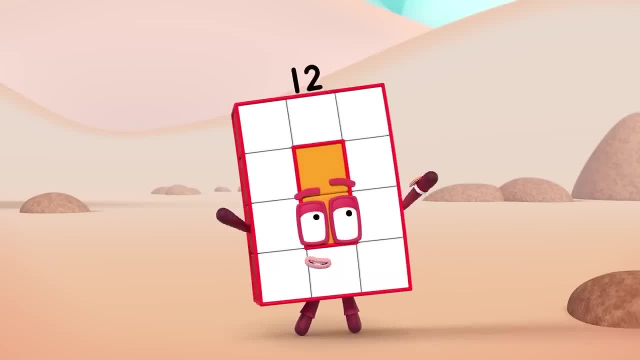 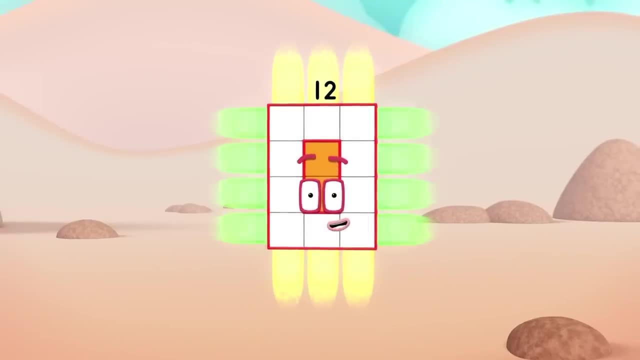 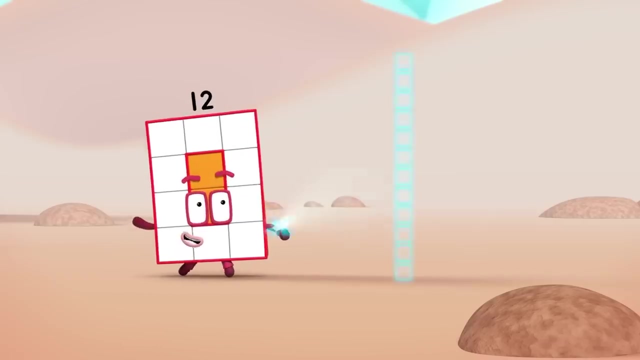 When I put my blocks in columns and rows, I make an array and my rectangle goes like this: Three By four. Today's the day for an array display Actively. I can make arrays all day. I make arrays in many ways. 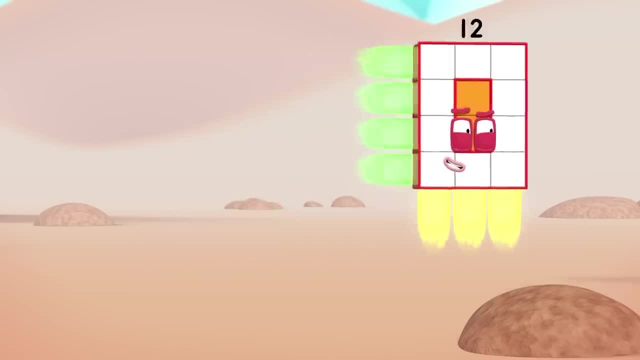 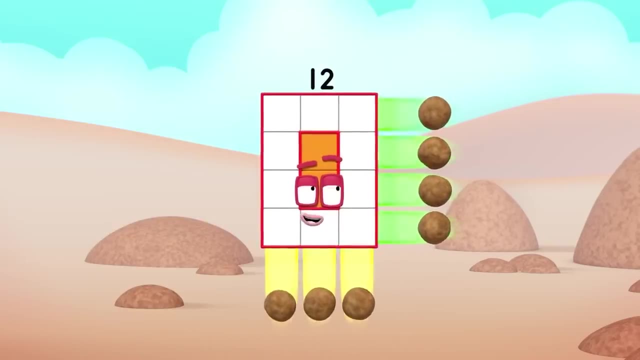 Stand back, let's play arrays away. Three by four is my first array. Three, lots of four, you could put it that way, And if you're not following what I say, I'll rectify that right away. Breakaway Three, fours. 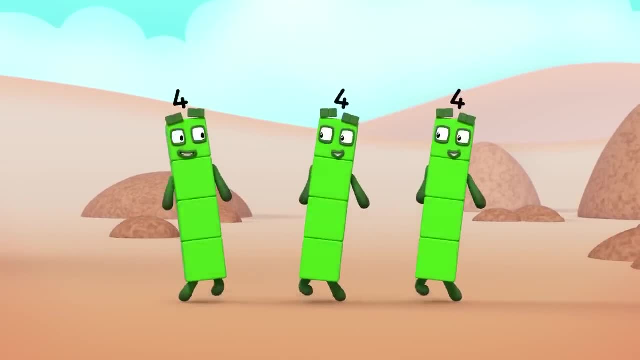 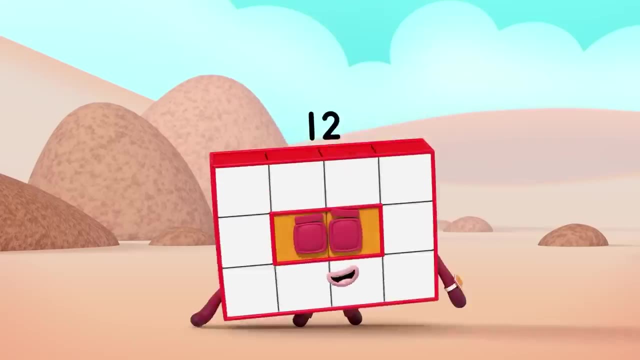 A four and a four and a four Rectangle rise Turn. I'm Rectangular 12, I'm 10 and 2. I make arrays. that's what I do When I put my blocks in columns and rows. 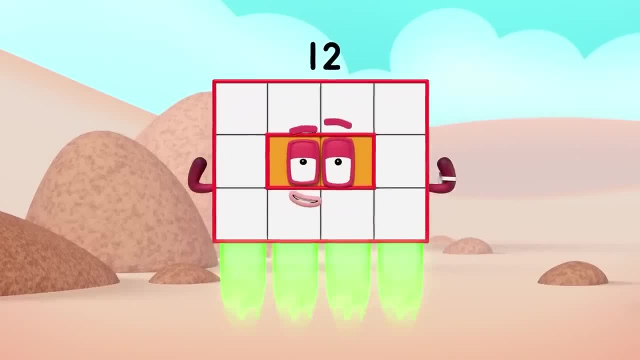 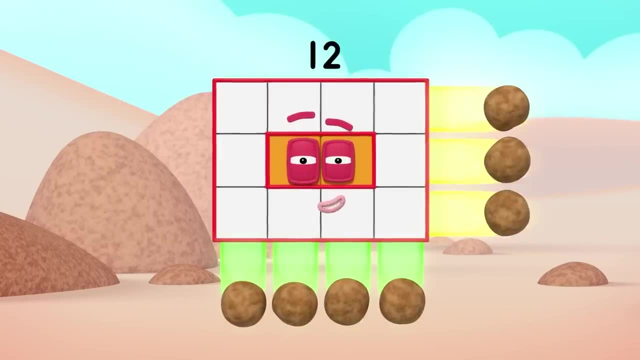 I make an array and my rectangle goes like this: Four By three, Four by three's. my next array: Four, lots of three, you could put it that way- And this rectangular display is about to show you how it's made Breakaway. 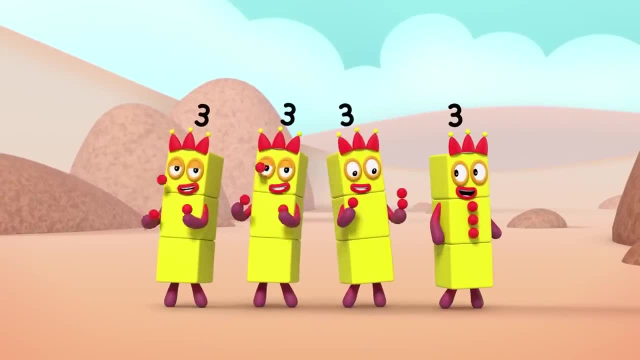 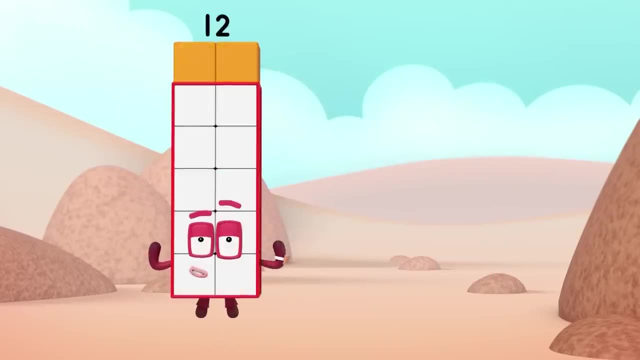 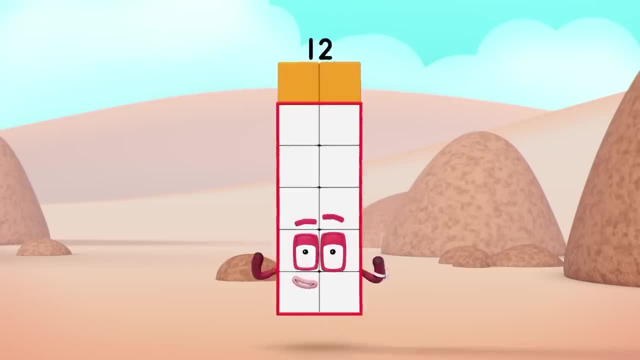 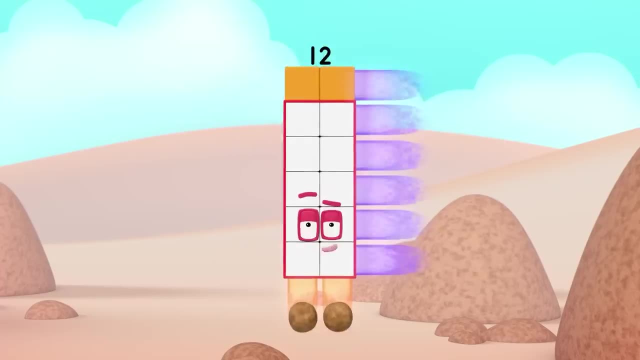 I make an array and my rectangle goes like this: Two By six. Two by six is another way. Two, lots of six. do you hear what I say? Another rectangular array. So let's split without delay. Breakaway: Two sixes. 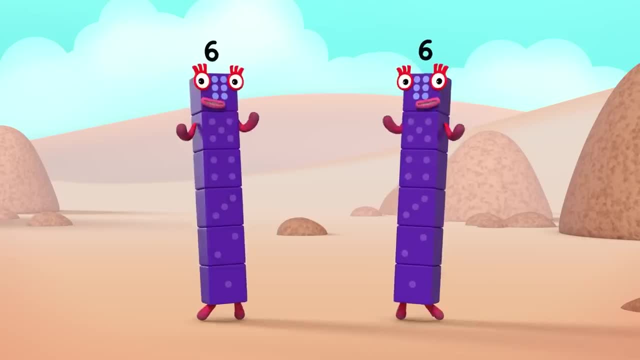 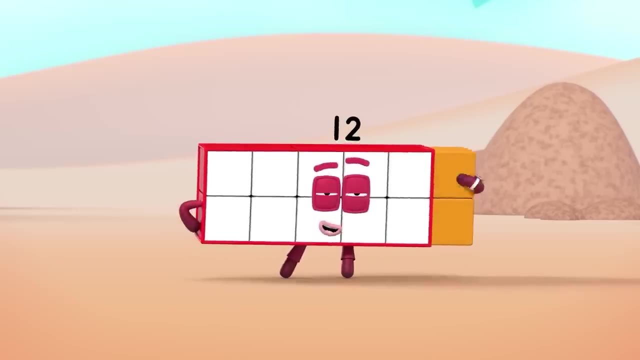 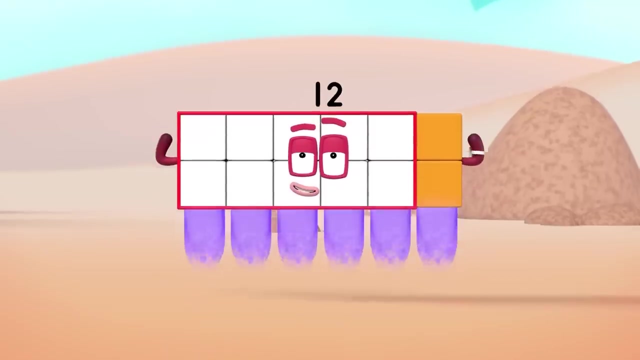 Let's roll Double: six, Ten, I'm, Rectangular 12,, I'm 10 and 2.. I make arrays. that's what I do When I put my blocks in columns and rows. I make an array and my rectangle goes like this: 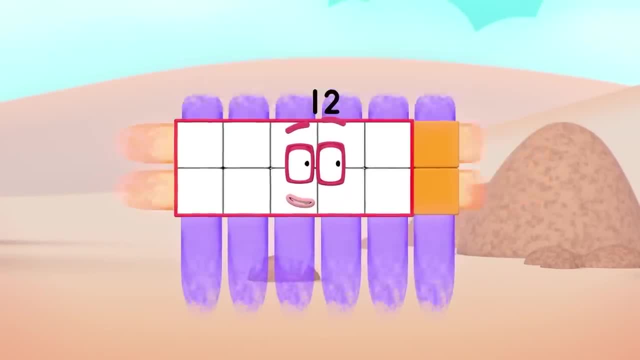 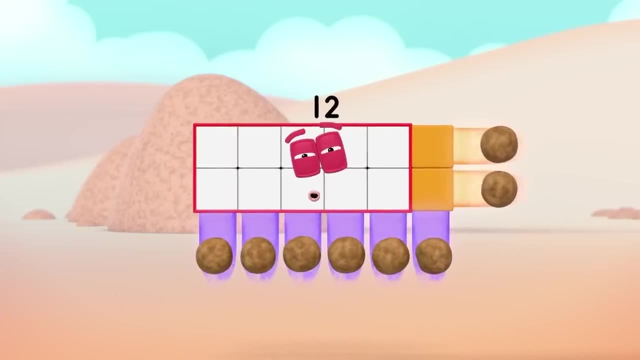 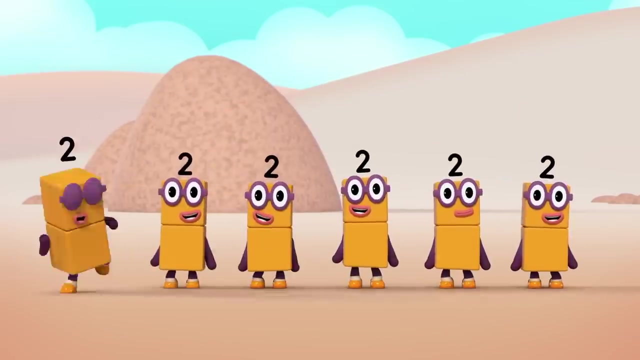 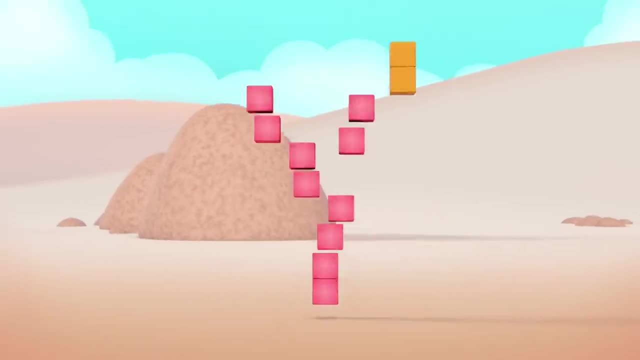 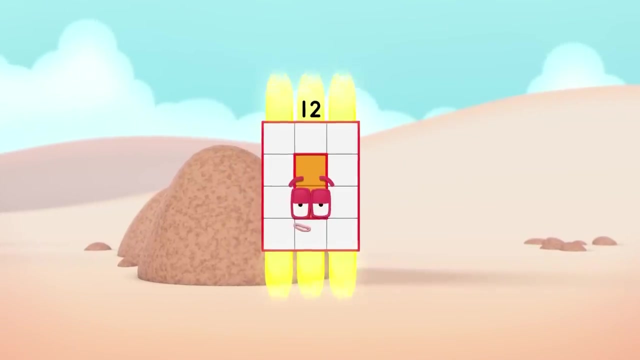 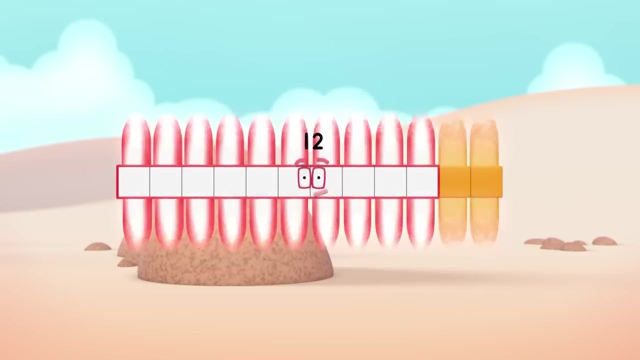 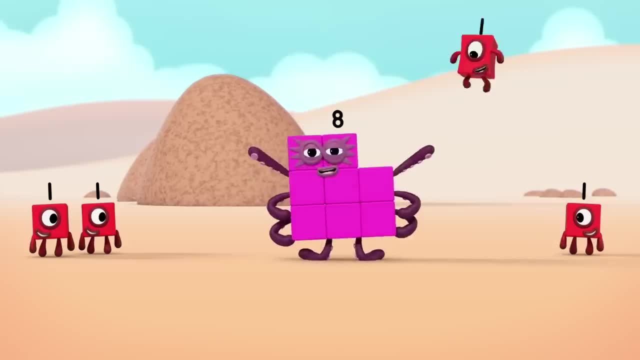 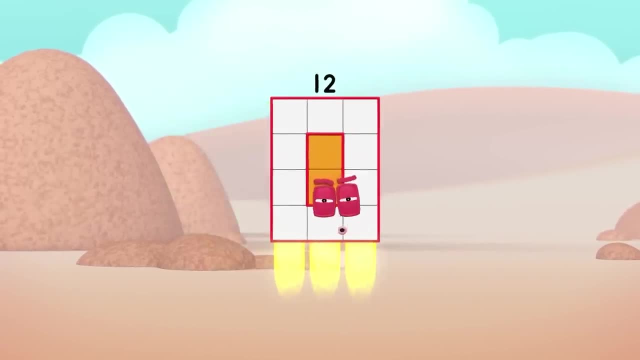 One, Two, Three, Four, Five, Six, Seven, Eight, Nine, Ten, Eleven, Twelve- It's a new craze to coin a phrase. You'll be in a daze when you fix your gaze On my amazing array displays. 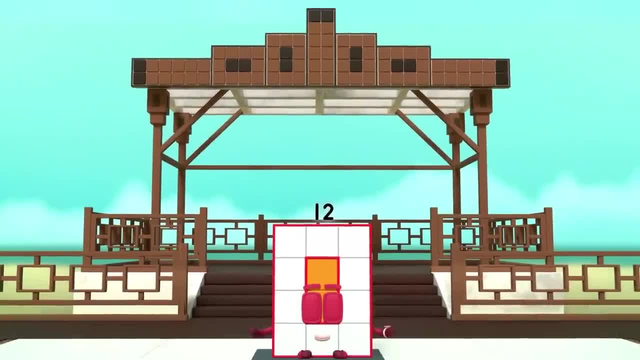 I'm Rectangular 12,, I'm 10 and 2.. I make arrays. that's what I do. I make arrays, that's what I do. I am twelve, I am three by four. I am a rectangle Turn. 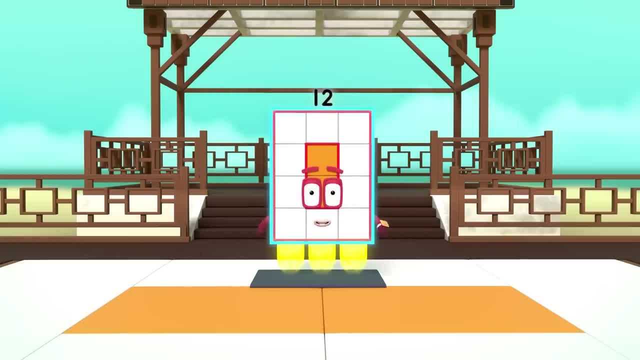 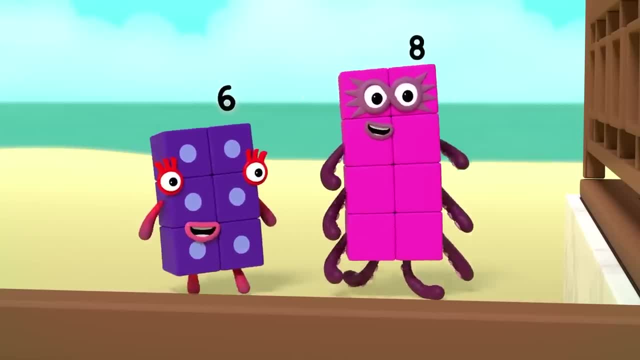 I am also four by three And I am a super-rectangle. I can take many forms, Switch. I am six by two. Turn I am two by six. I am a small animal. I can hit small animals. I am a big machine. 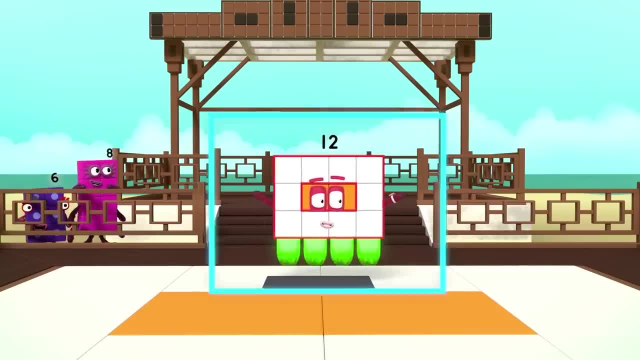 And I am a small bigаю On and off. I am a 12!. I am a three by four. I am a rectangle. I am a three. I am a rectangle. I am 12!. I am a three by four. 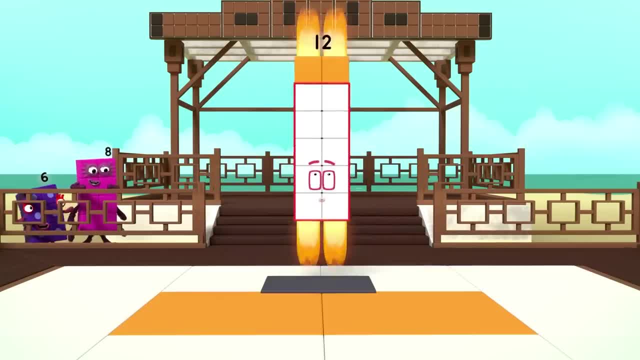 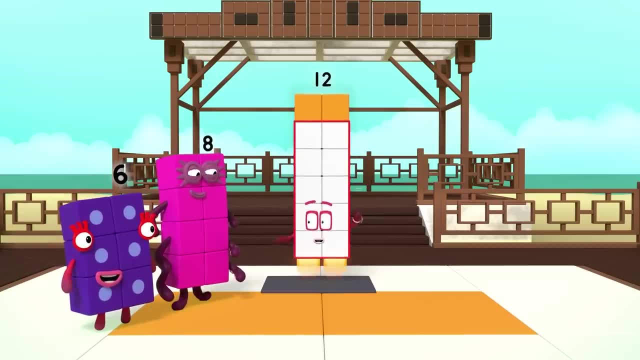 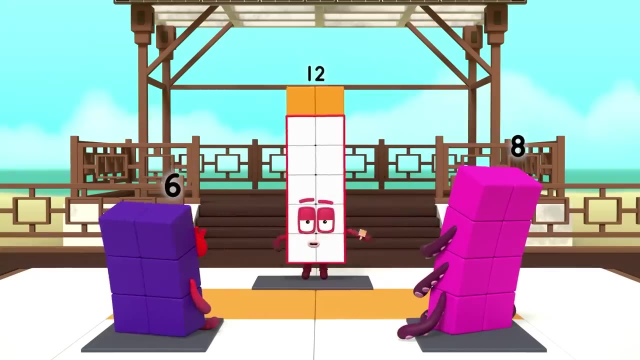 I am a rectangle. I am a rectangle. I am a rectangle. Turn I am a rectangle. Welcome my friends. Would you like to master the way of the rectangle? First you need to stand, so your front makes a rectangle shape. 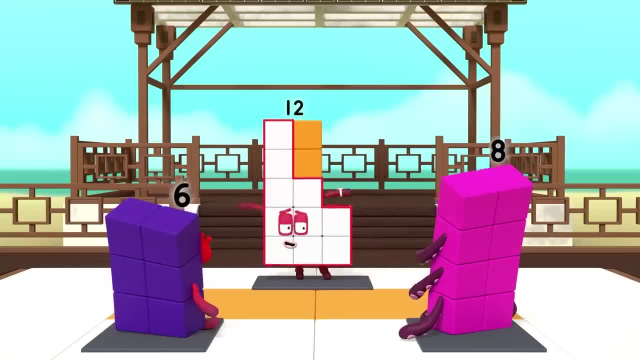 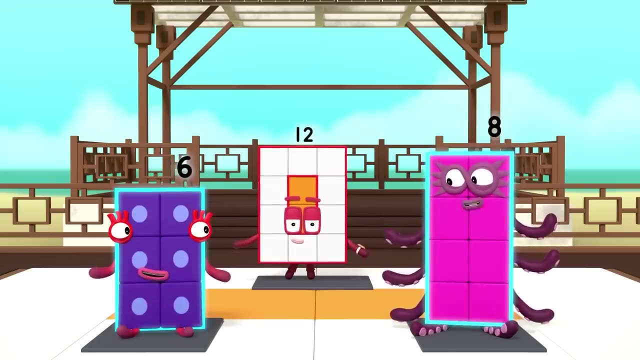 Watch and tell me when I'm making a rectangle. No, No, Yes, Well done. Now look at your own fronts. What shape are you making? I'm a rectangle, That's right. Your blocks are arranged in neat columns and rows. 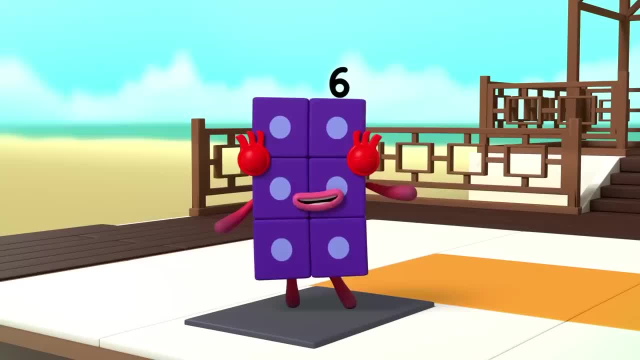 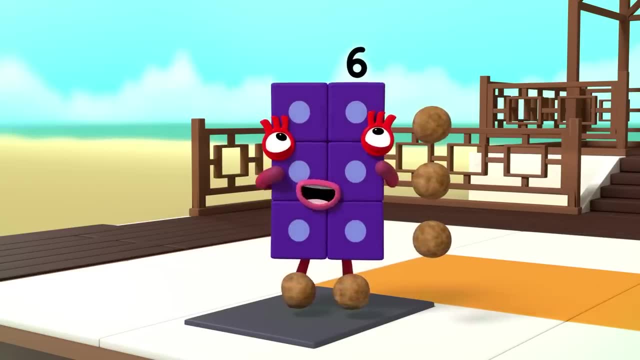 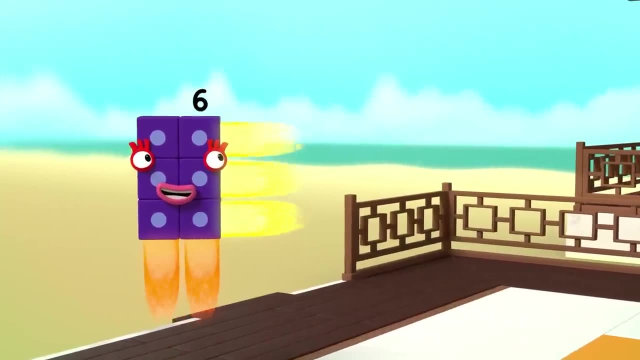 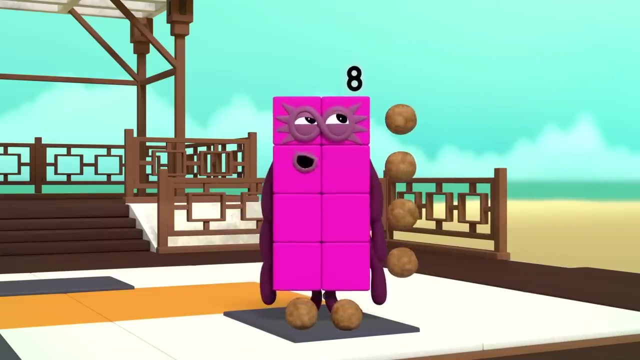 Now concentrate on how wide you are. I am six. I am two blocks wide by three blocks tall. I am two by three. I am a rectangle. Woo-hoo-hoo. I am a Eight. I am two blocks wide by four blocks tall. 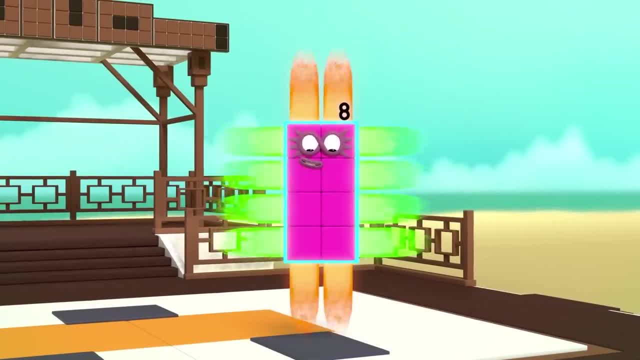 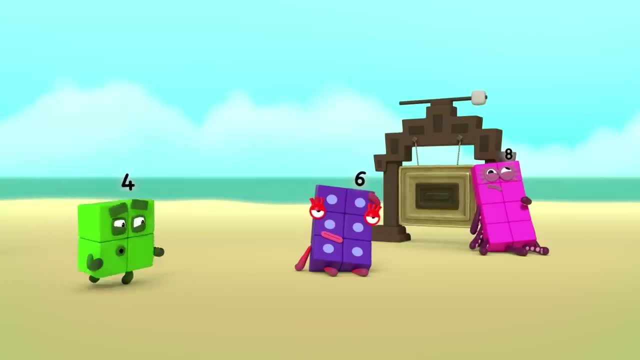 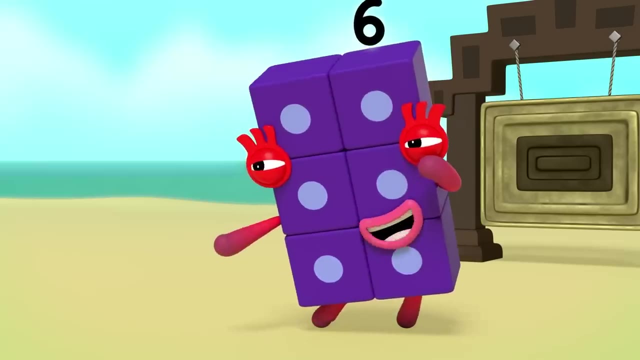 I am two by four. I am a rectangle Up, up and away. Woo-hoo-hoo, Oh, I heard a bang. Are you okay? Six, I'm more than okay. I've mastered the way. Hey, where are my rays? 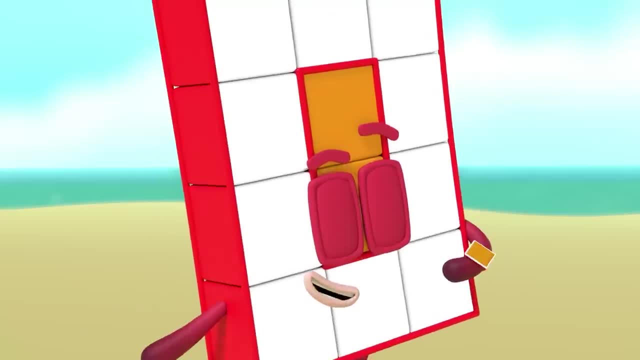 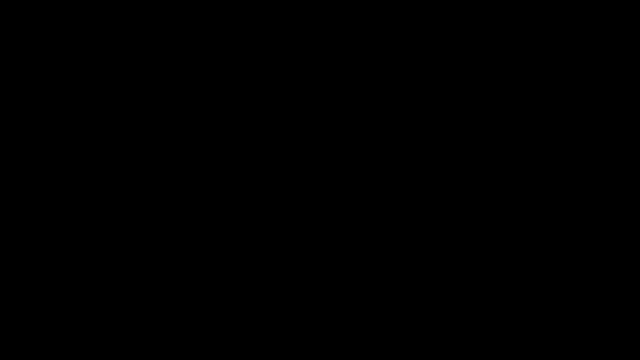 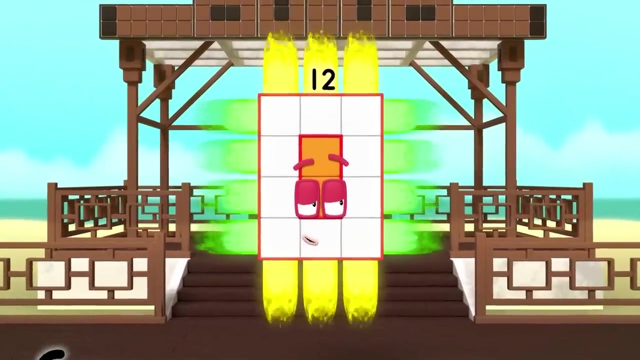 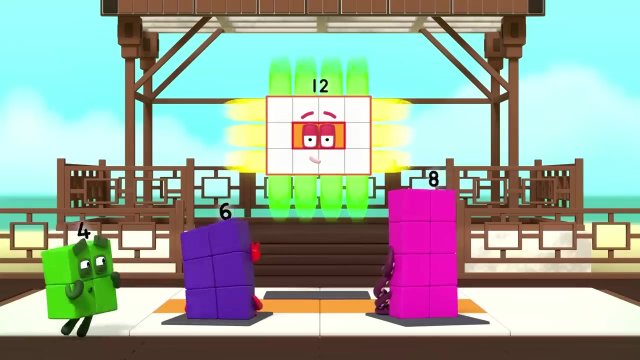 You need to concentrate. It gets easier with practice, So let's practice. It's time for the turn. I am twelve. I am three by four, which means turn. I am also four by three. See, Woo-hoo, I am six. 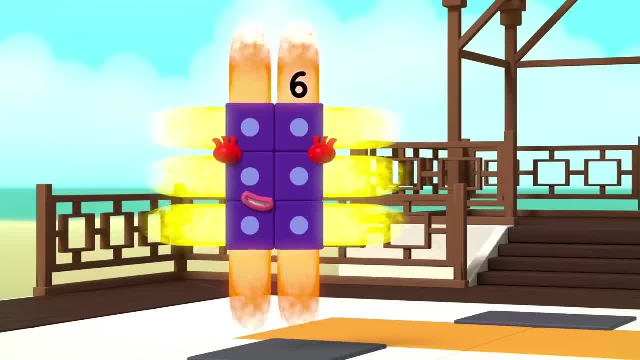 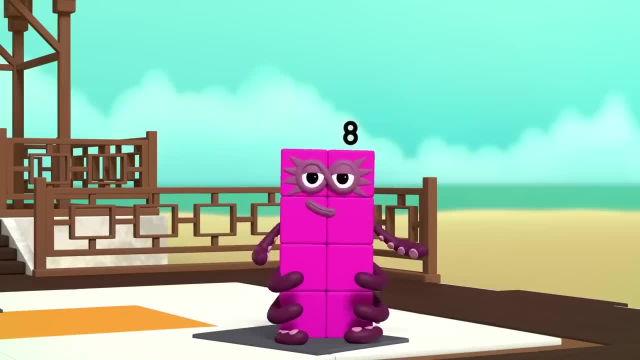 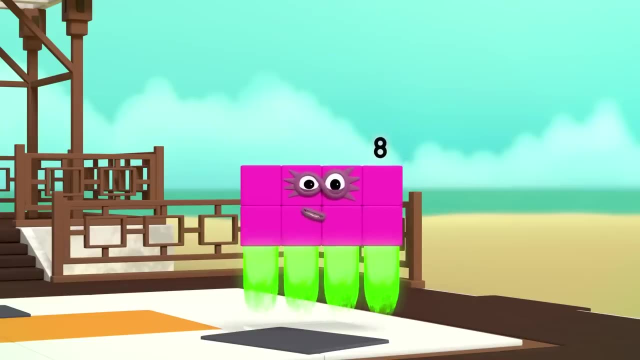 I am two by three, which means turn. Woo-hoo, I am also. So three by two, Woo-hoo-hoo-hoo, I am eight. I am two by four, which means Octoblock turn. I am also four by two. 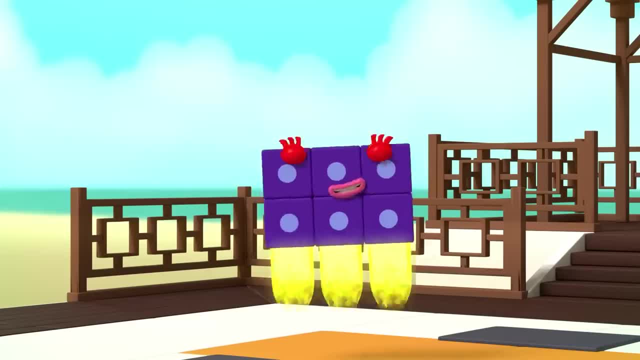 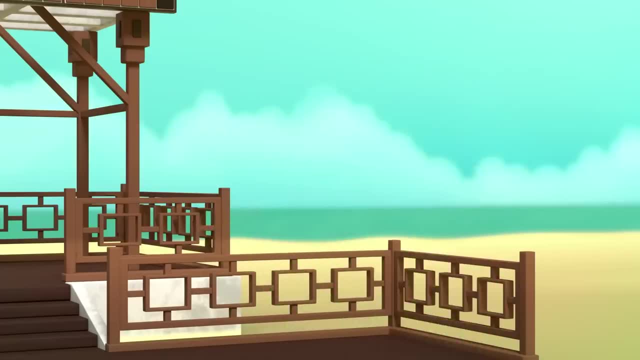 Ten, Two by three, Ten, Three by two, Ten, ten, ten, Woo-hoo, Let me try that. I am four, I am eight, I am two by four. Woo-hoo-hoo-hoo, I am eight. 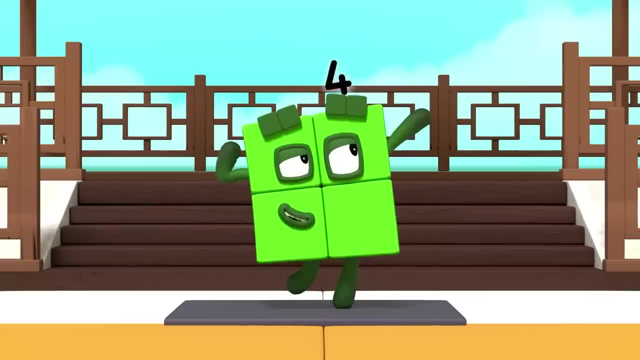 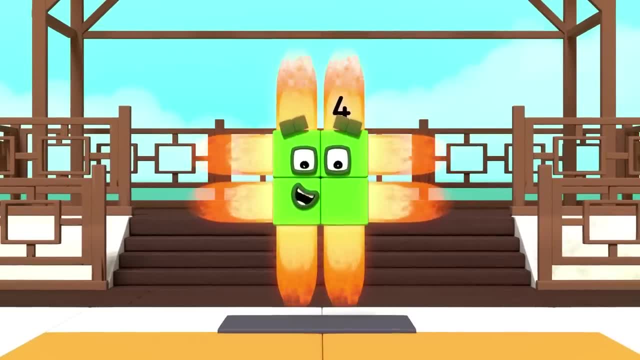 I am two by four, Which means Octoblock turn. I am also four by two. I am two blocks wide by two blocks tall. I am two by two, Yay, And I am also Turn Um Two by two. 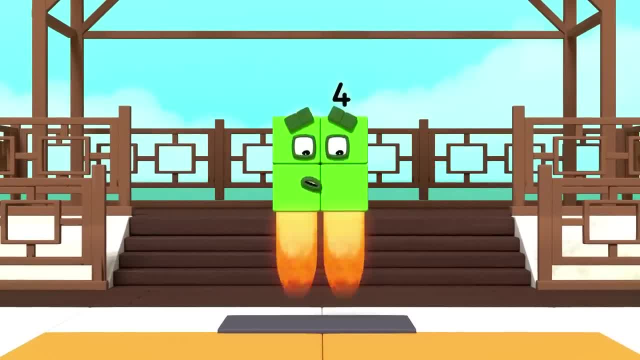 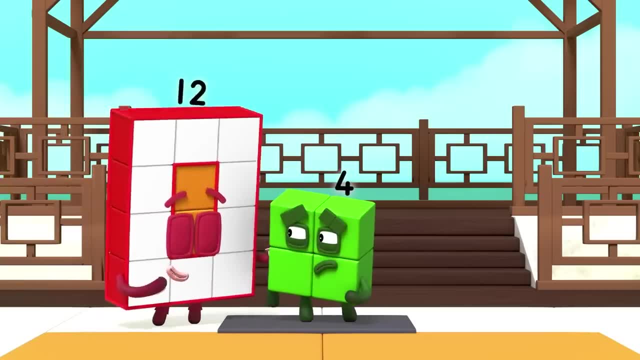 That's the same again. Did I go wrong? No Four, You're a special kind of rectangle that is the same number of blocks wide as tall. A square, A square, Woo-hoo, Oh, Oh, Oh, Oh. 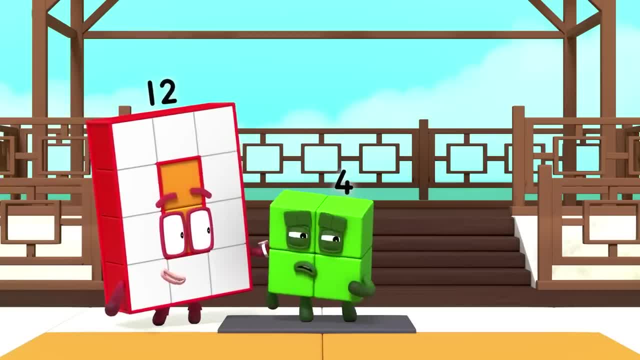 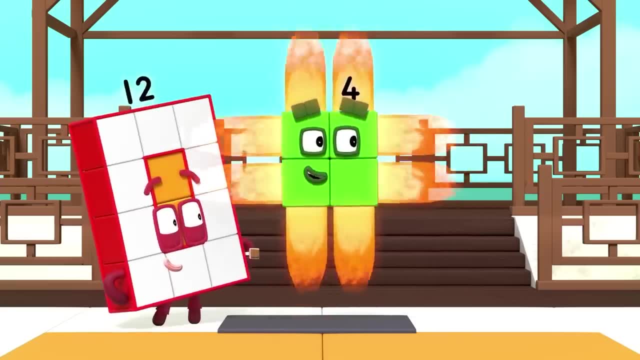 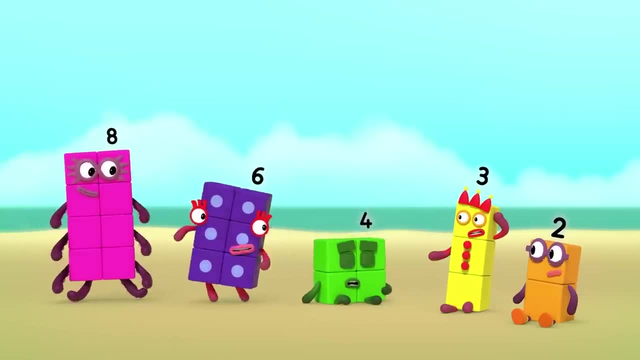 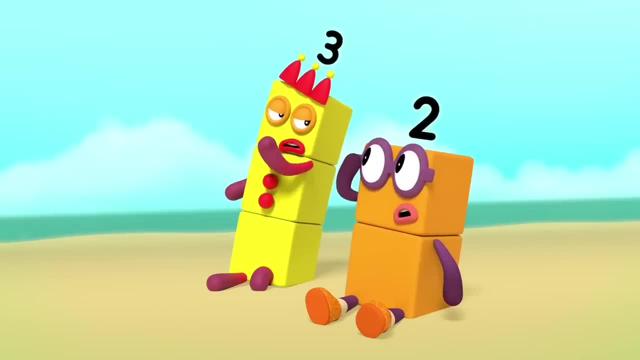 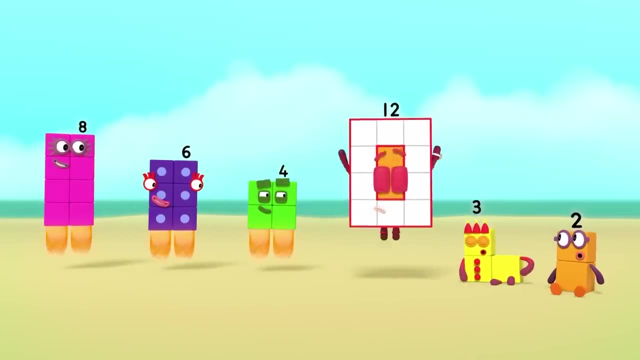 Oh, It's all right for some. I can't make big, wide rectangles. Whoever said rectangles had to be wide? Oh, Number blocks stand tall. Now what should I do? Oh, Oh, Oh, Oh, Oh Oh. 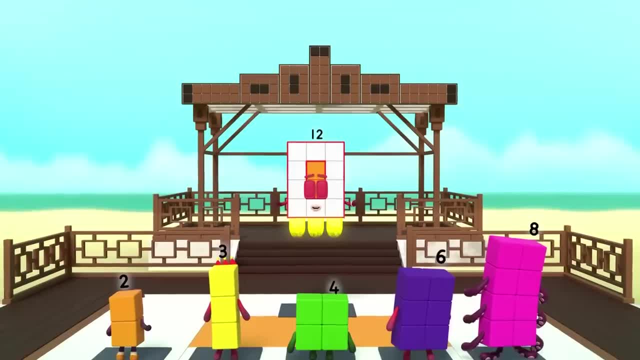 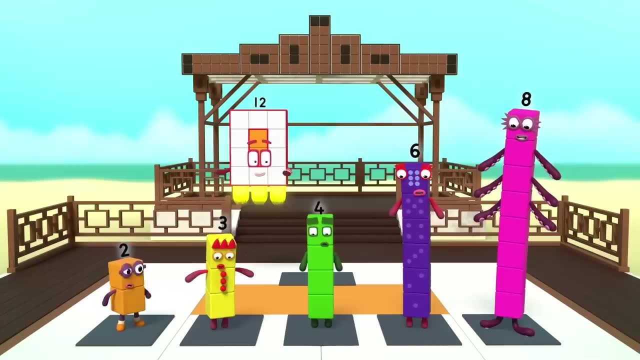 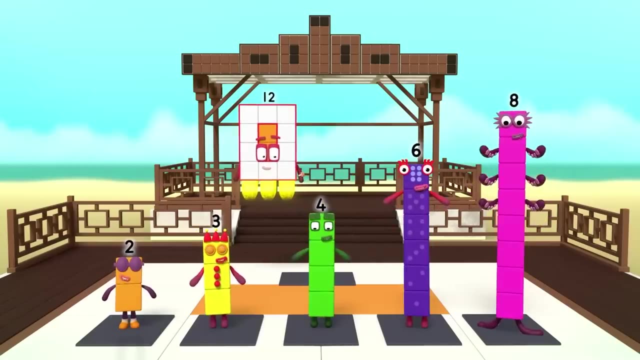 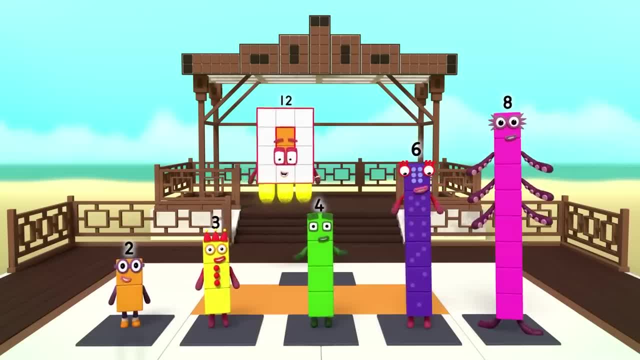 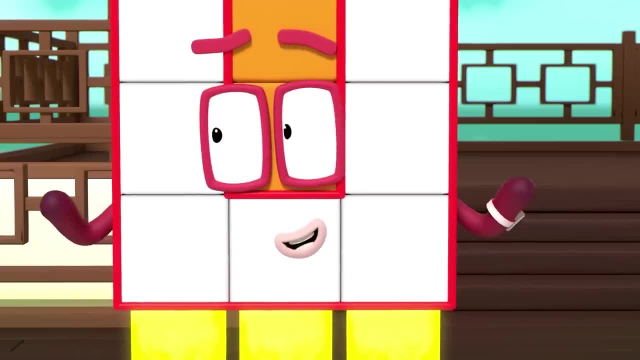 Three, Four, Six, Eight Blocks tall. I am a rectangle. Maybe I shouldn't have told them Weee. Oh well, Too late now. Whoa, Whoa, Woah, Whoa, Whoa, Whoa. 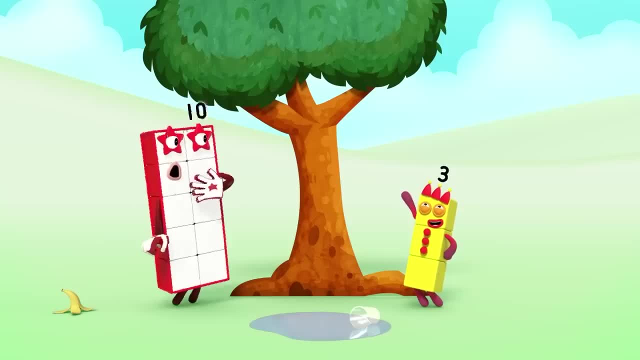 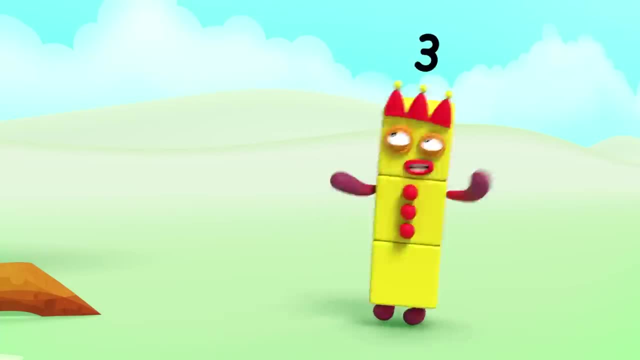 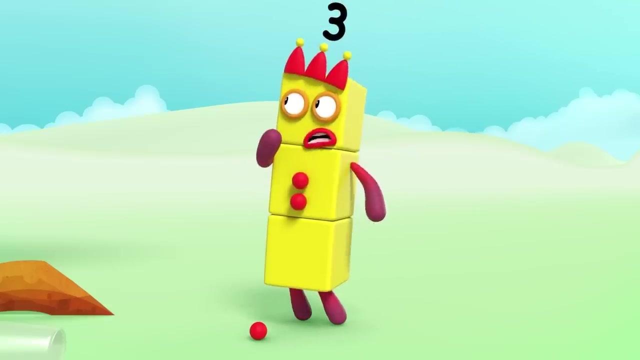 Three, Oh, sorry, Ten. I'm just so excited to show you my new trick. Look at this. Oh, Is that it? No wait, I'm not having much luck with my today. Oh no, My new trick. 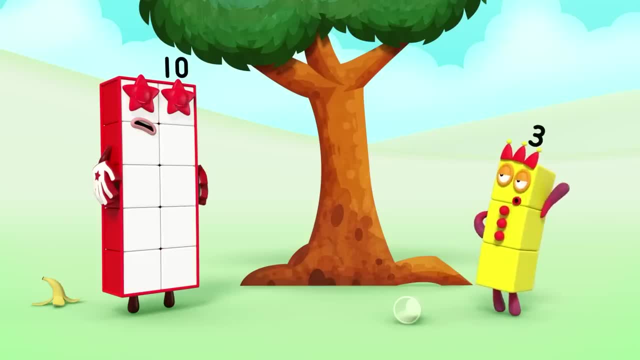 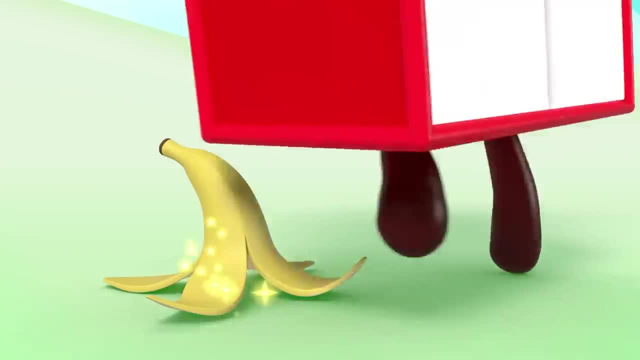 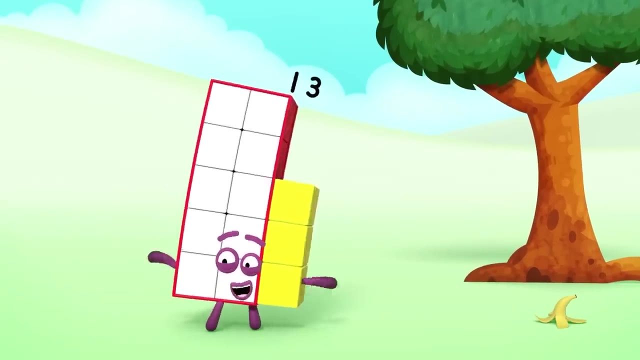 Ready, steady, go. Ooh, Oh Unlucky. Oh, Hi, Who am I? I'm one, two, three, four, five, six, seven, eight, nine, ten, eleven, twelve, thirteen. 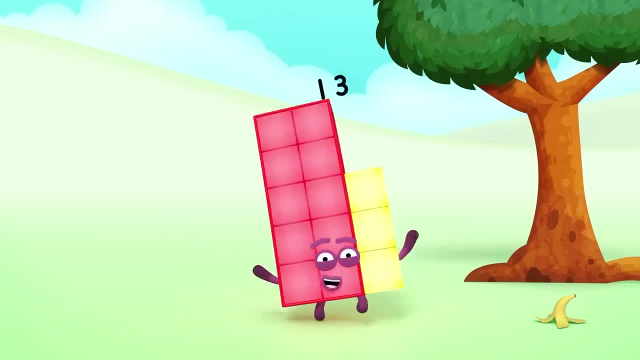 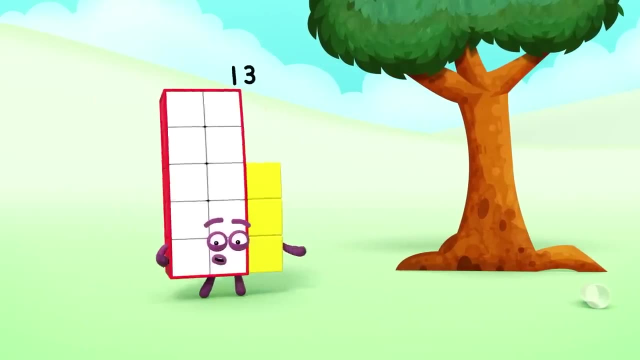 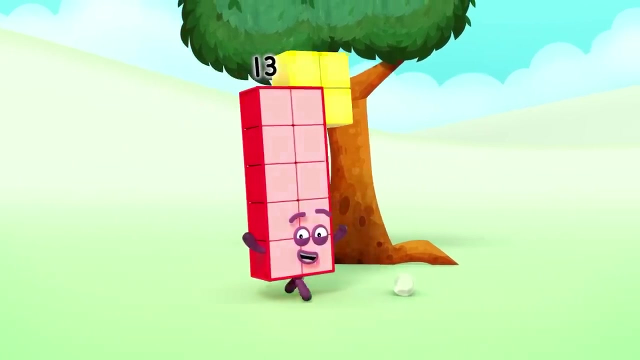 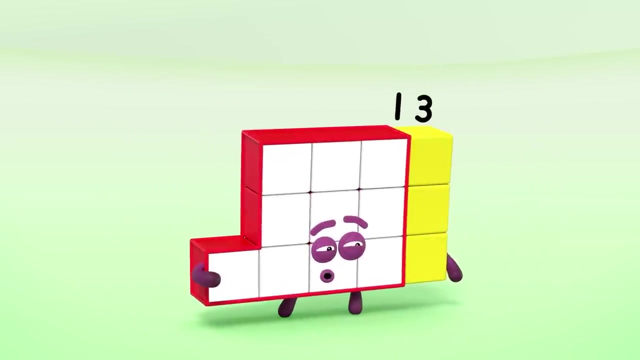 Whoa What, Wow, Whoa Oh. my three fell off, Never mind, Oh, Oh, Oh, Oh, Oh, Oh, Oh. This is so funny, I am 13.. Oh, whoa Ha. 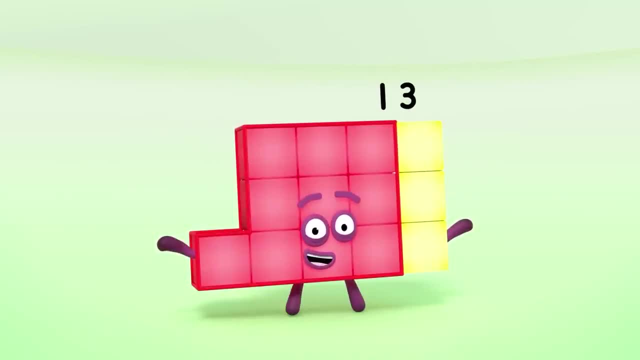 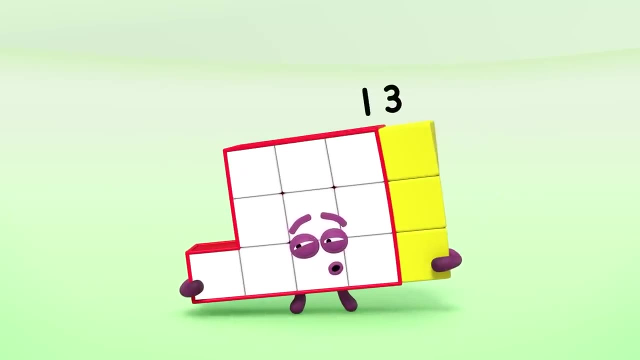 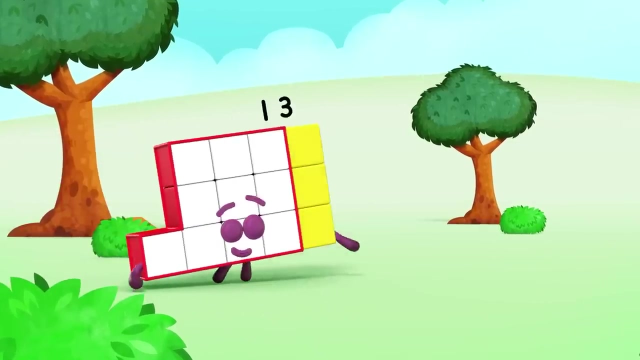 Oh, Unlucky, Try again. I am 13.. Ha, Oh, Yay, Ooh-hoo-hoo Ha, And I think I might be a little bit. This is me, ten and three, expecting to run out of luck. 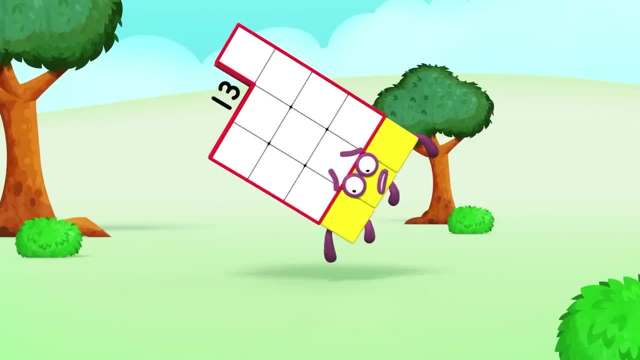 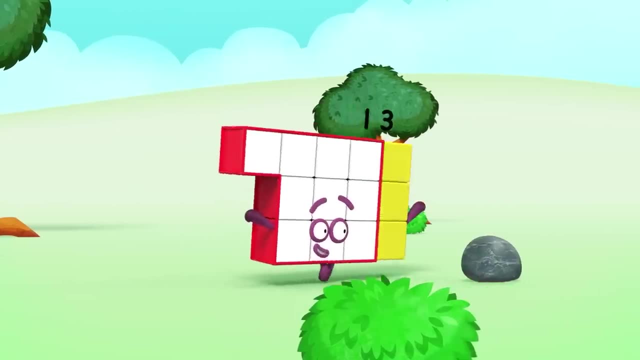 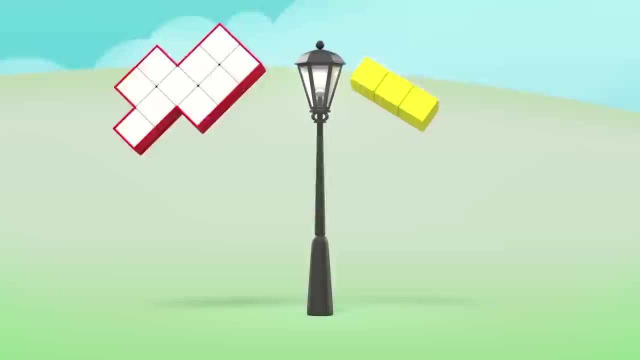 It's all jolly japes. when I get into scrapes I'm always coming unstuck. I'm the clumsiest number you've ever seen. unlucky number thirteen. It's happened again. a three and a ten. somebody should tell him that it's happened again. 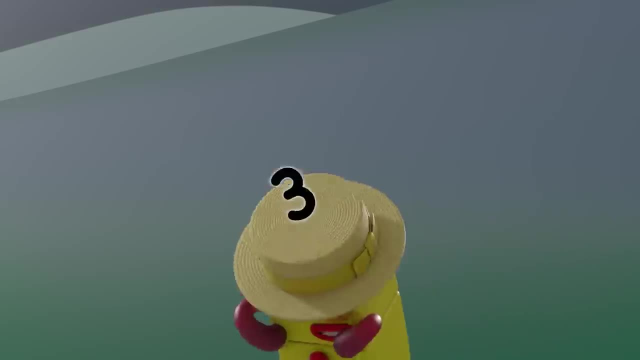 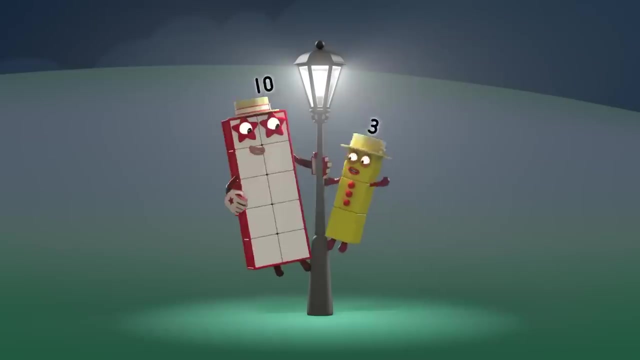 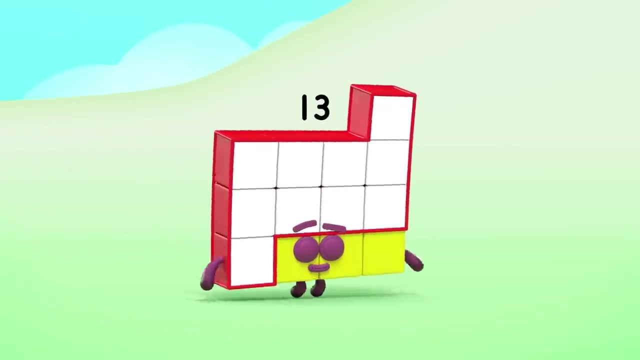 I don't have the heart to be fussy or picky, but he's falling apart. he's a bit unsticky. It's happened again and no one knows when somebody should tell him that it's happened again. Me again, three and ten expecting to fall. 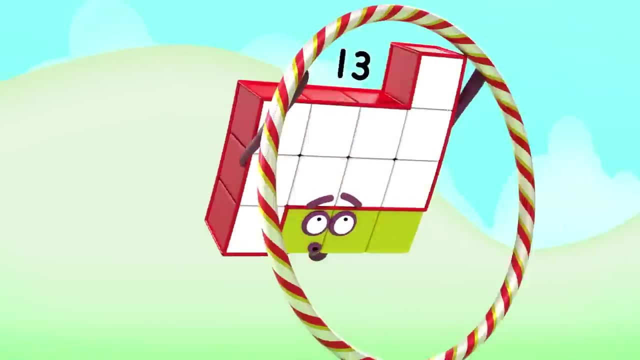 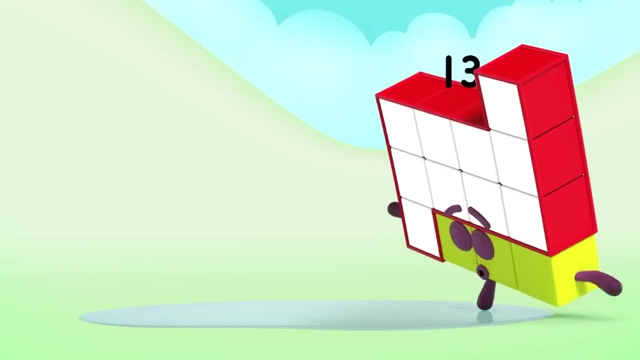 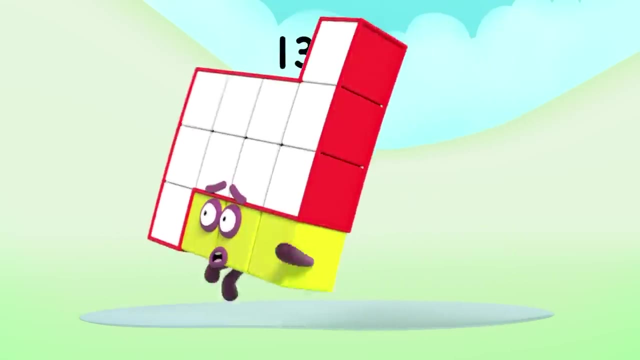 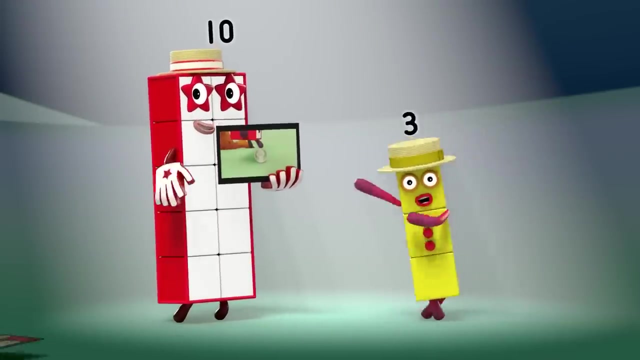 I fall down a hole, I jump through a hoop and step in the puddle. that seems to sum up my role, And wherever I end up, I might get slain. unlucky number thirteen. It's always the same. when he says his name, somebody should tell him that's the name of the game. 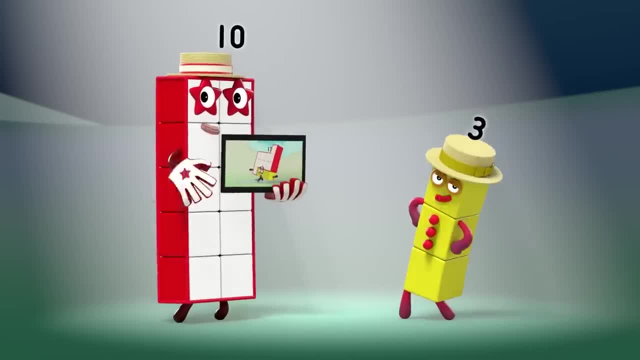 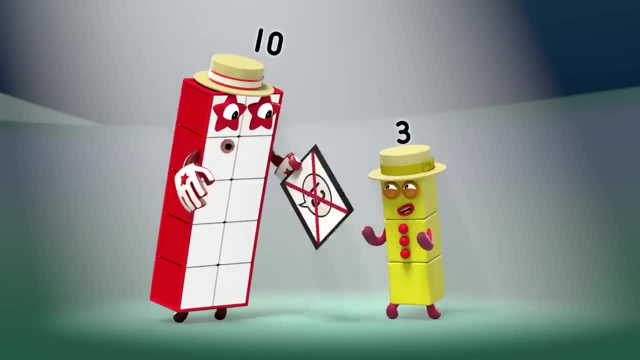 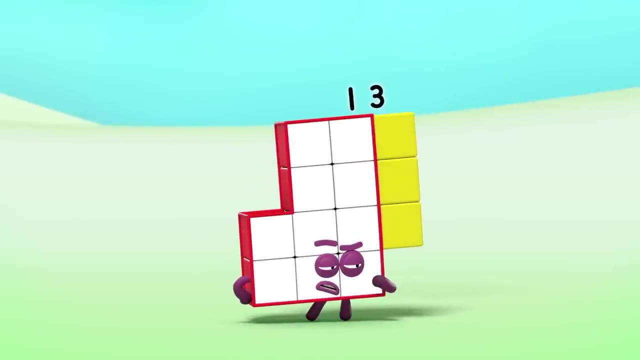 It's happened before, a total disaster. but he's going to need more than a sticking stick. It's always the same. we know what to blame. somebody should tell him not to mention his name. It's getting routine. I say I'm thirteen. 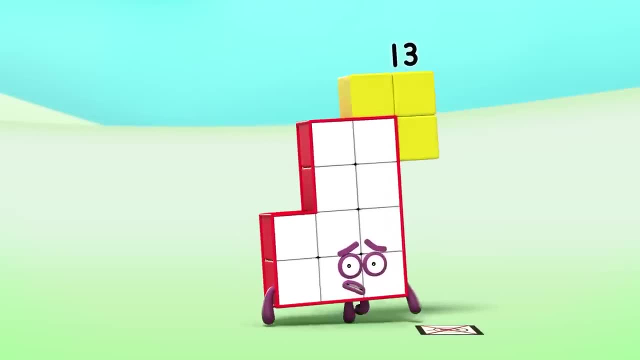 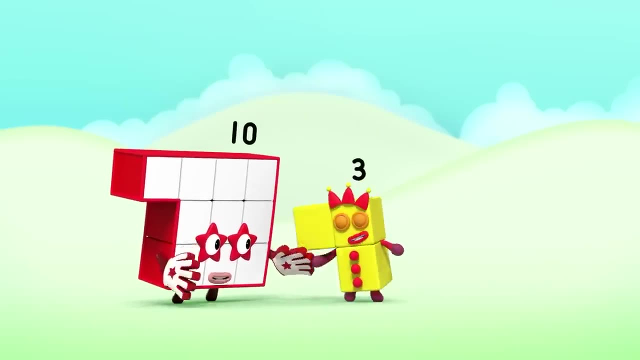 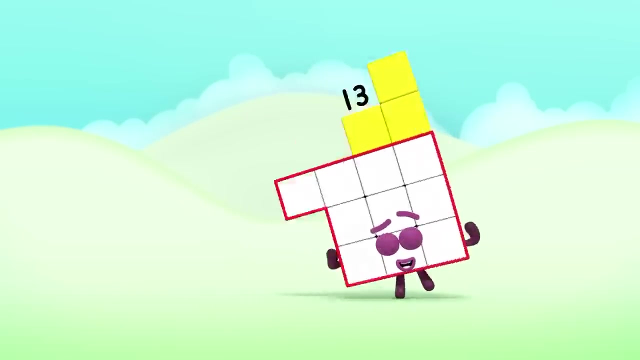 Keep it together. this is absurd. You know what I mean. I say it's thirteen. End of my tether. don't say that word. It's always the same, it's getting routine. They ask me my name. I say I'm thir. 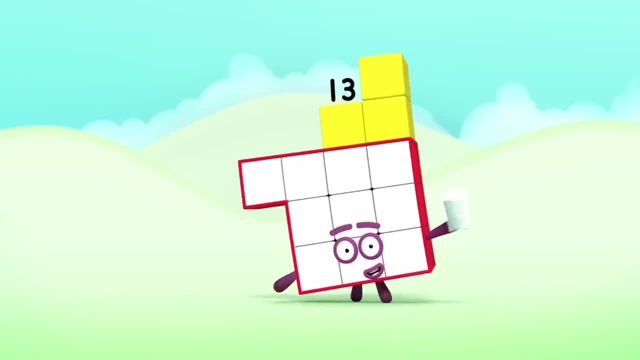 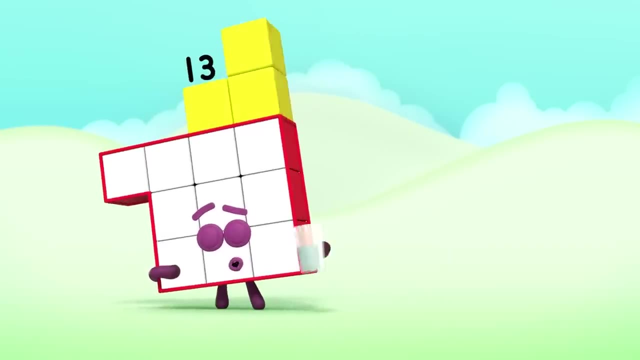 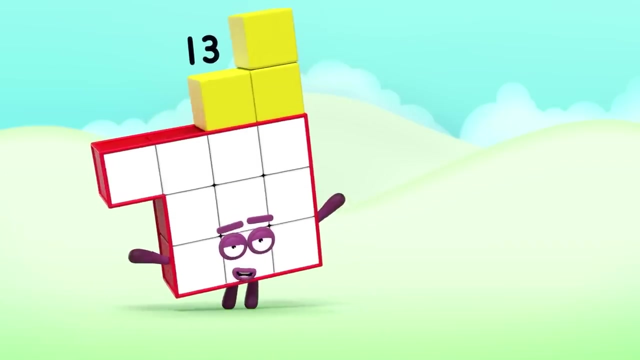 Thirsty, I say I'm thirsty. They ask me my number. you know what I mean- And I always say: it's thir Thursday. I always say it's Thursday, Andy, Jack, and it's their time. This is me. ten and three, turning this into a game. 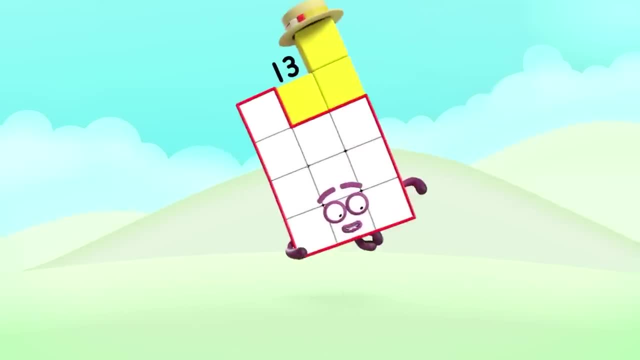 I'm changing my name. I say I'm thir. I'm changing my name. I say I'm thir. I'm changing my luck. I won't come unstuck As long as they don't say my name. Call me one more than twelve or ten and three. 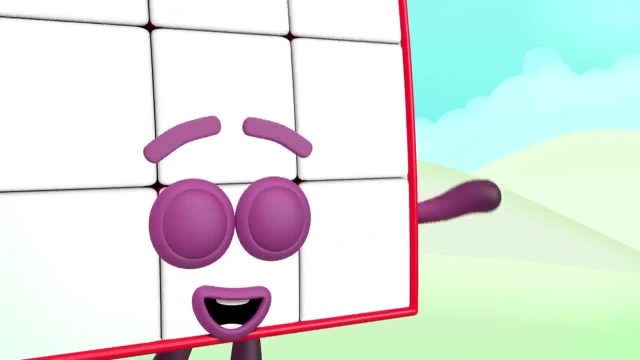 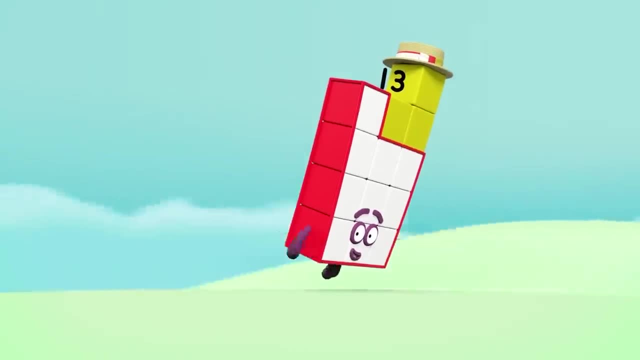 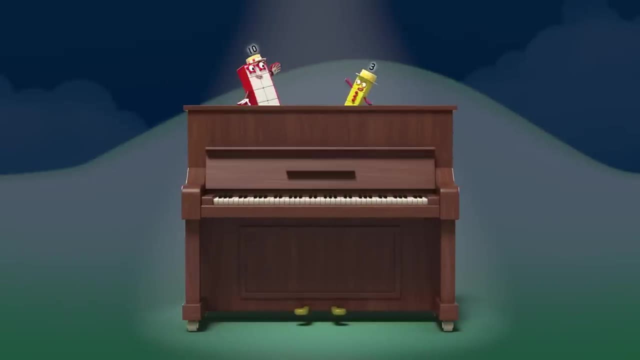 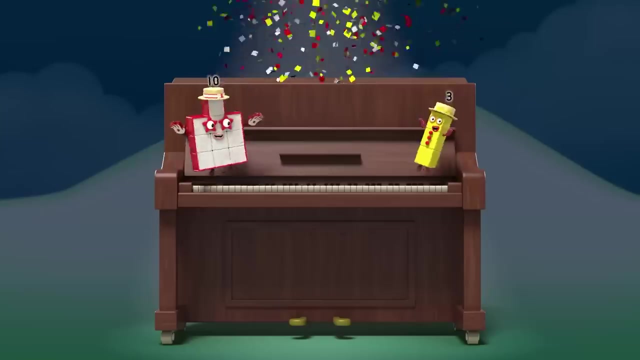 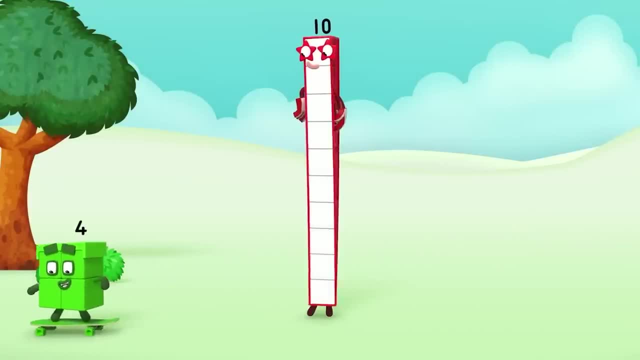 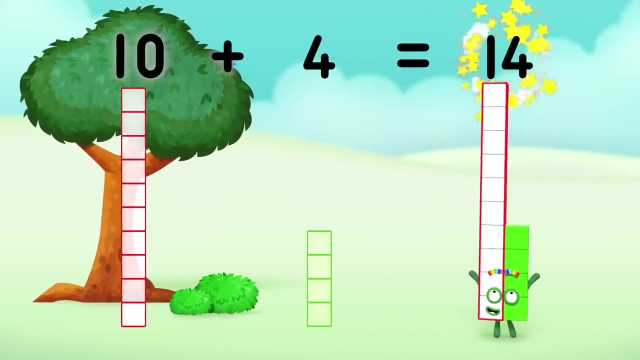 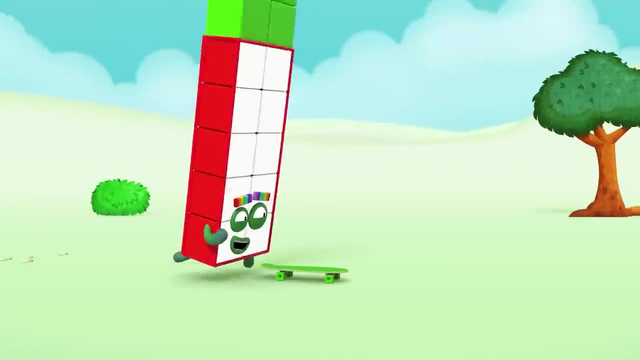 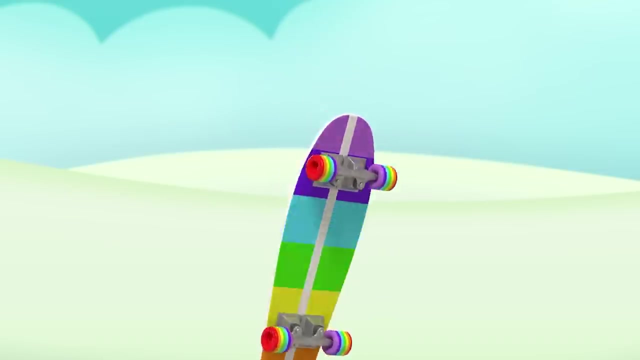 Hello ten, Hello four. Look at my new skateboard: Square wheels. Ten Plus four Equals Forty. Whoa, I'm a totally new number, dude. Check it out. Sweet stripy skateboard, I am 14.. 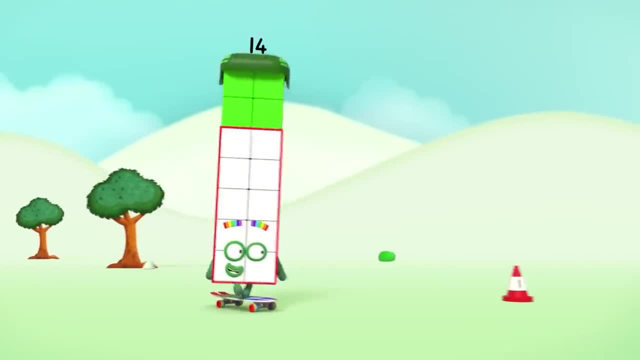 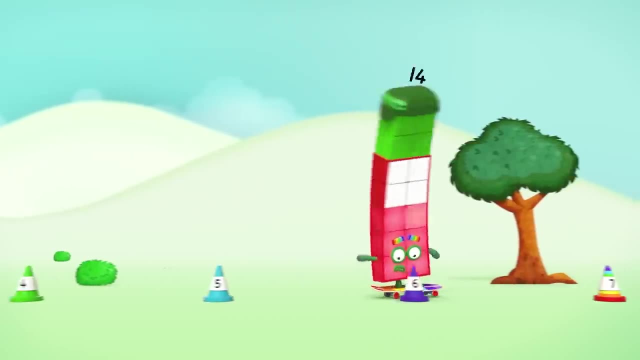 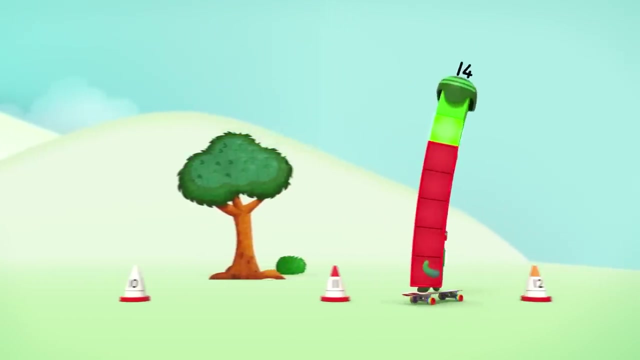 And I live to skate One, two, three, four, five, six, seven, eight, nine, ten, eleven, twelve, Thirteen, fourteen extreme. I want to be a skater, I want to be greater than the rest. 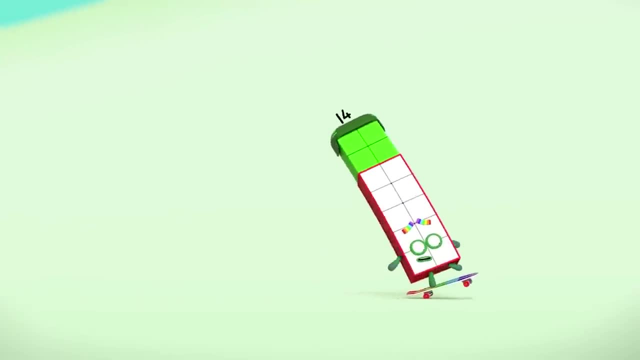 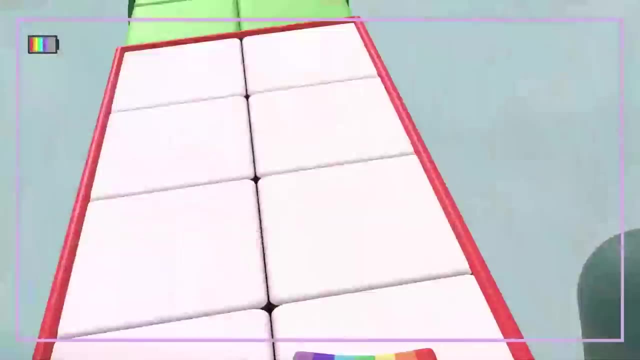 I'm going to ride to a tail slide. I want to be better than the best. I'm going to nail all the tricks, All the ollies, pops and cake flips. Trust me, sooner or later I'm going to be a skater. 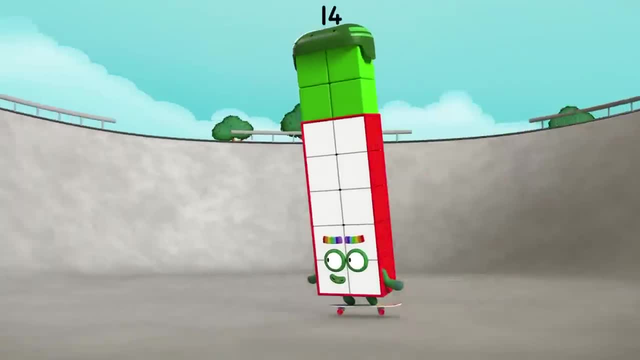 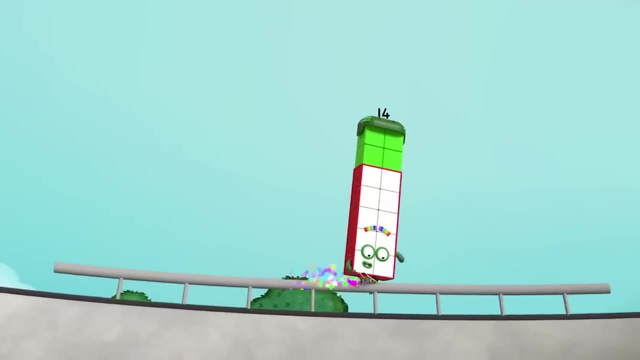 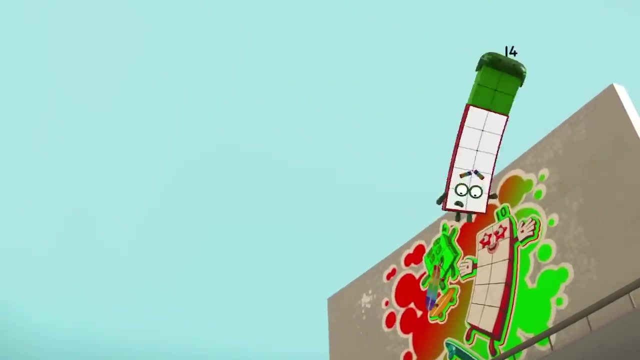 I'm 14,, I'm ten and four, I'm also double seven. I'm riding on an elevator straight to skater heaven, And whenever I get into a fix in the middle of one of my brand new tricks, I've got my lucky double to get me out of trouble. 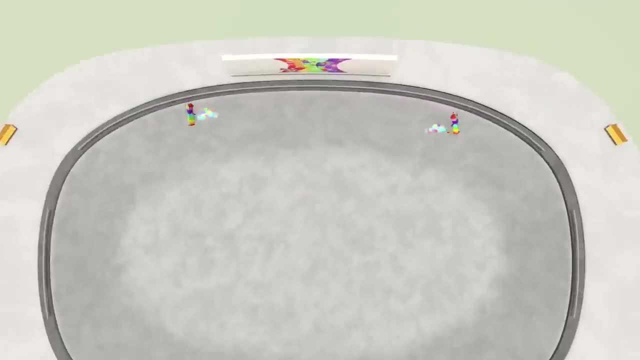 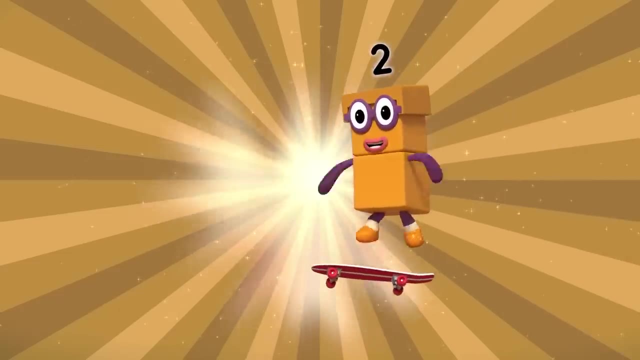 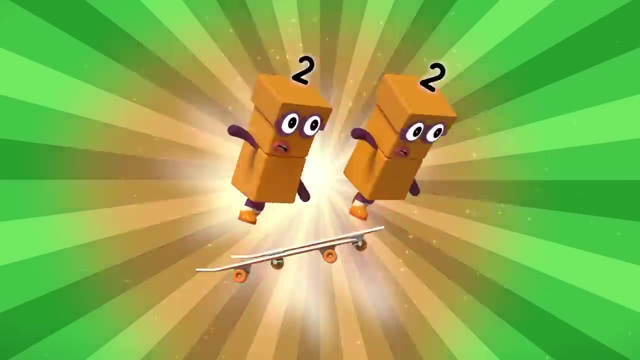 Lucky double seven. Maybe you've got a lucky double too. Hello, I'm two, I'm two and I can split into ones. Double one, double the fun. I'm four and I'm double two. Whoa, two, twos. I think we may need grippy shoes. 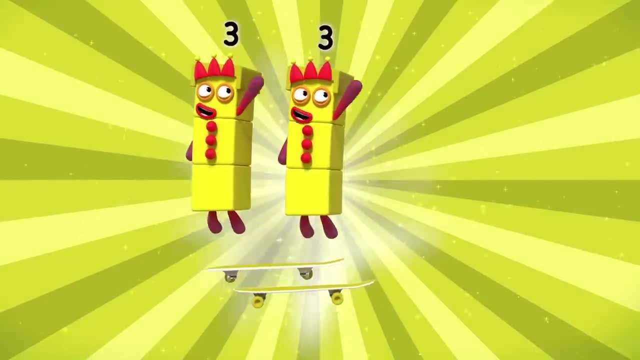 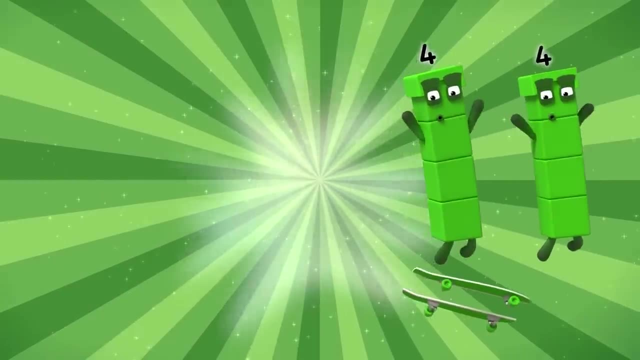 I'm six and I'm double three. Well, look, you're saying, look at me, I'm eight and I'm a four and a four, Double four. have you seen us before? I'm ten and I'm double five. 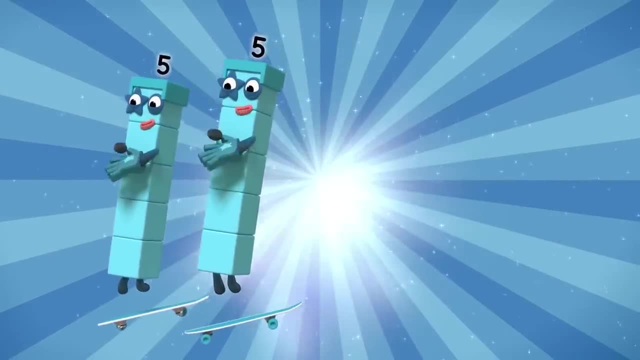 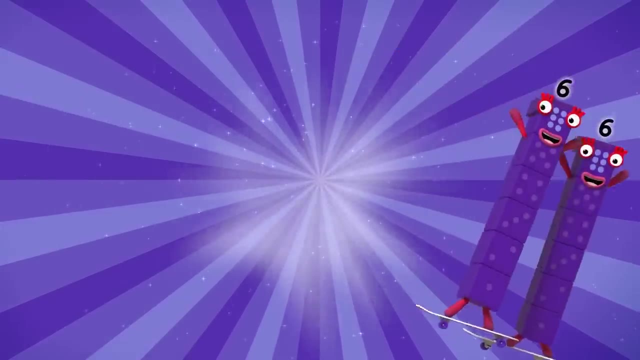 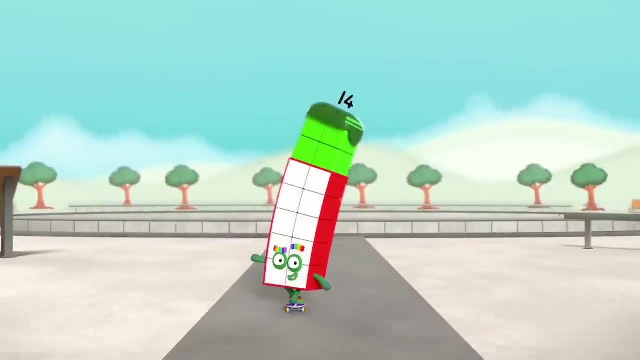 Two big hands? No, we can do a double five hand jive. I'm 12, and I'm double six. We don't need dice to do these tricks. I'm extreme 14, and I'm keen to show you what my lucky double seven can do. 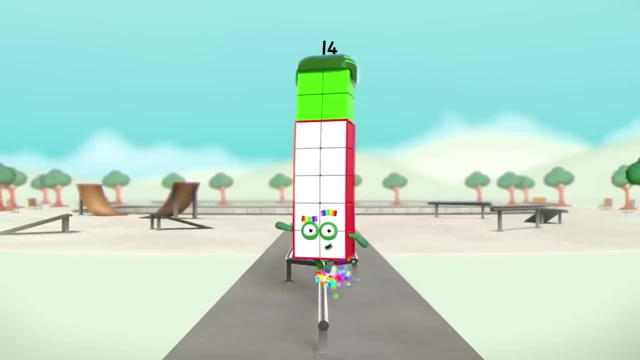 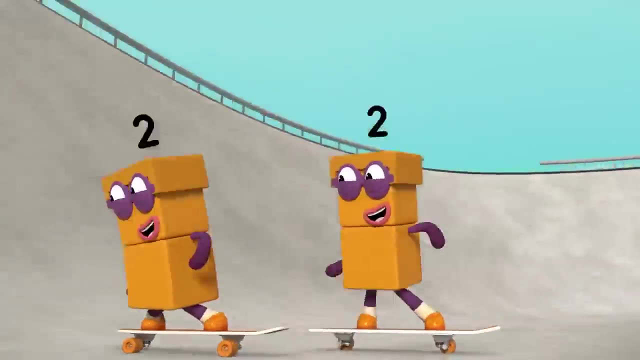 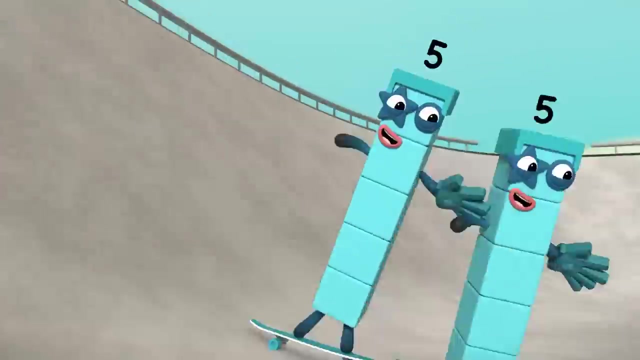 Lucky double seven. Maybe you've got a lucky double too. Double ones make two. Ten. Double twos make four, Four. Double threes make six. Six. Double fours make eight, Eight. Double fives make ten, Ten. 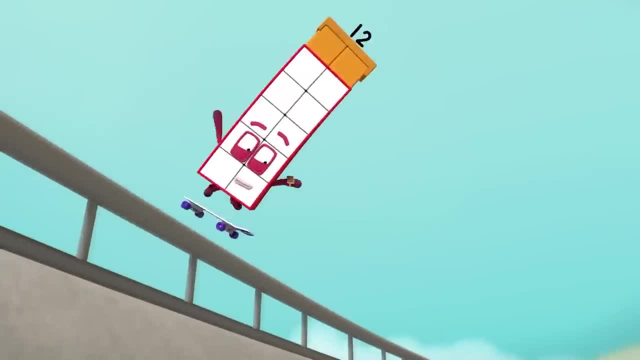 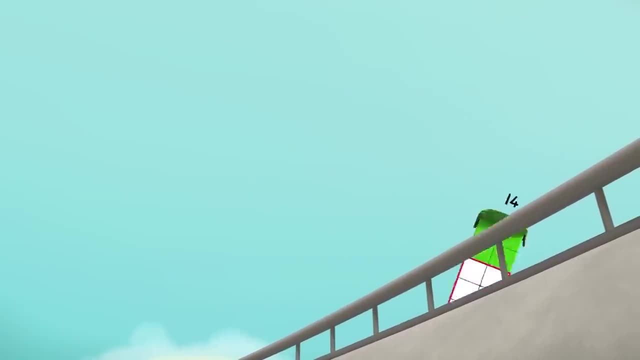 Double sixes, Twelve, Twelve, Double sevens make 14.. Ooh, that's us Extreme 14. I'm 14.. I'm ten and four. Ten and four. I'm also double seven. I'm riding on an elevator straight to skater heaven. 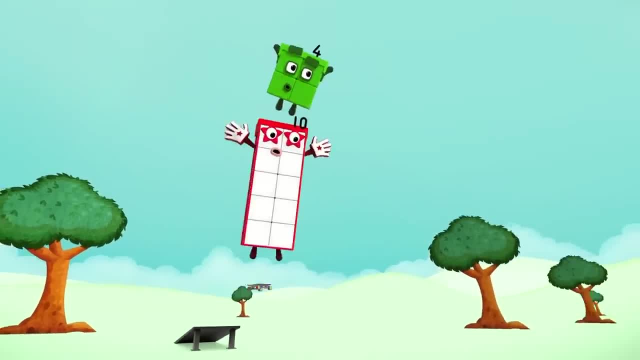 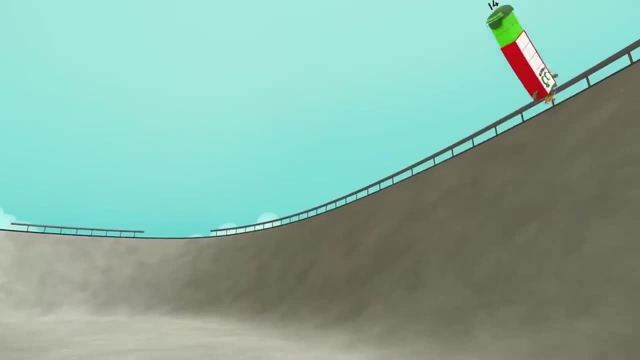 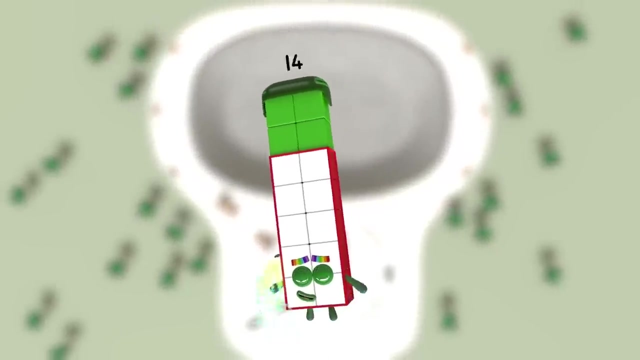 And whenever I get into heaven I'm going to do the�. I'm really really low Still good, Yeah, Well done. In the middle of one of my brand new tricks, I've got my lucky double To get me out of trouble. 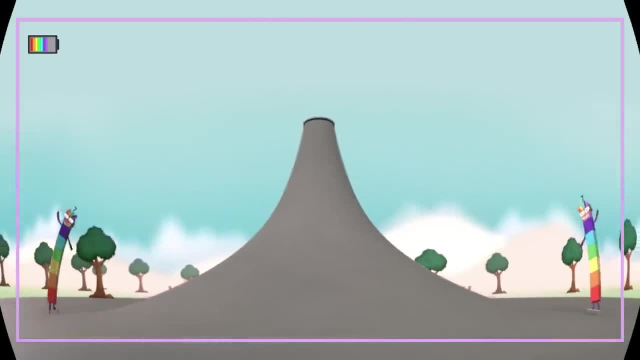 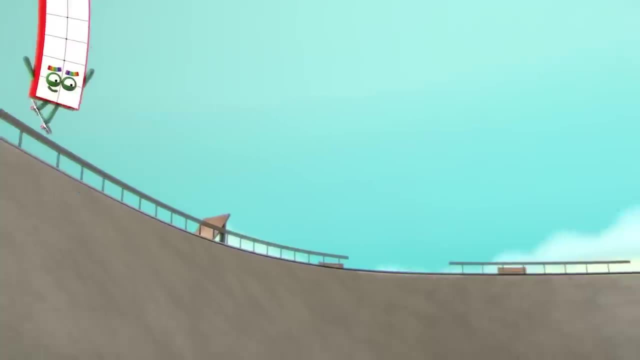 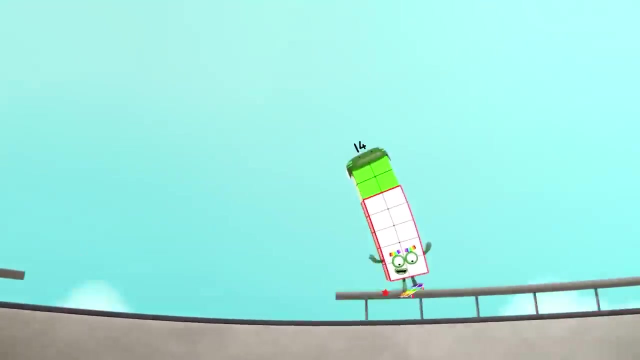 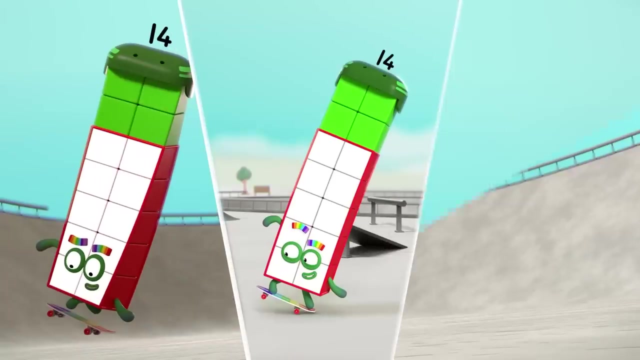 Lucky double's a fun. Maybe you've got a lucky double too. I wanna be a skater. I wanna be greater than the rest. I'm gonna ride, do a tail slide. I wanna be better than the best. I'm gonna nail all the tricks, All the ollies, pops and cake flips. 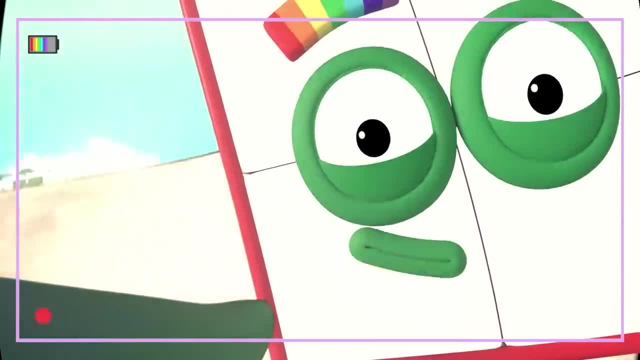 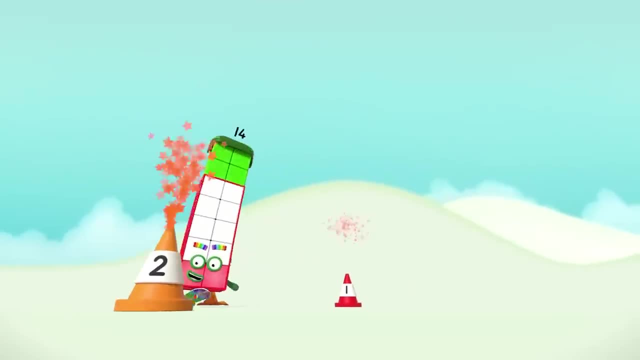 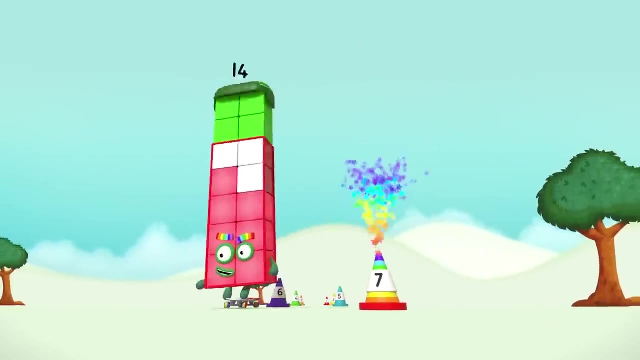 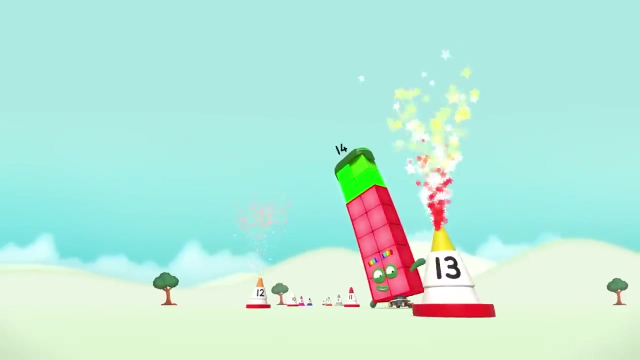 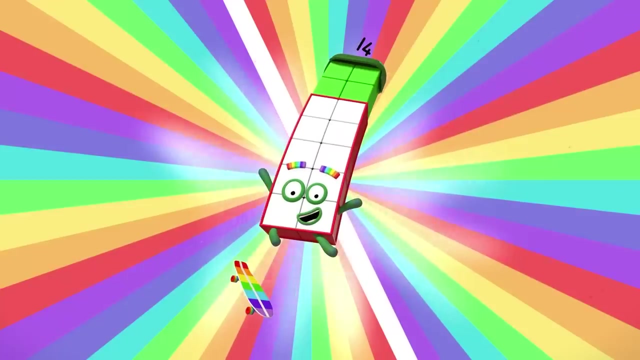 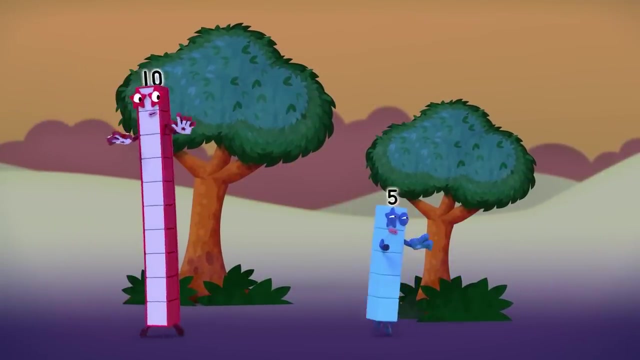 Trust me, sooner or later I'm gonna be a skater. One, two, three, four, Five, six, seven, Eight, nine, ten, Eleven, twelve, Thirteen, fourteen. I wanna be a skater. Yeah, Hush, hush. Ten plus five equals fifteen. 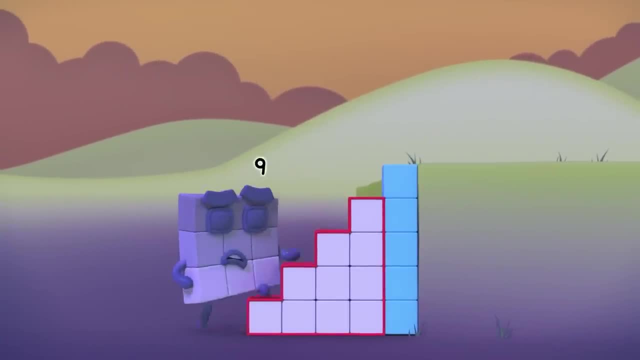 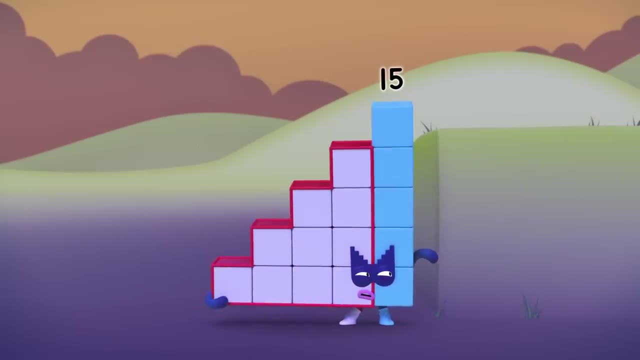 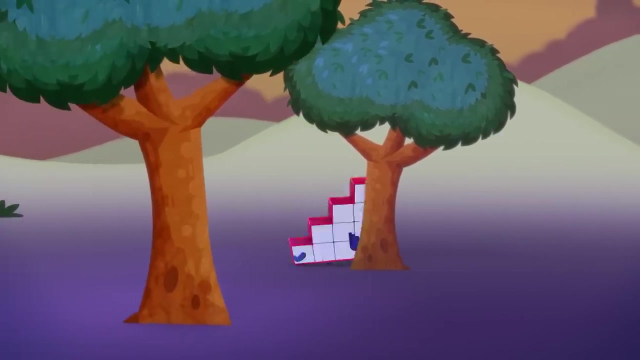 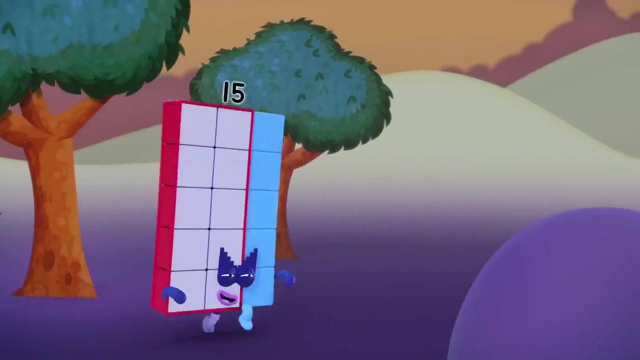 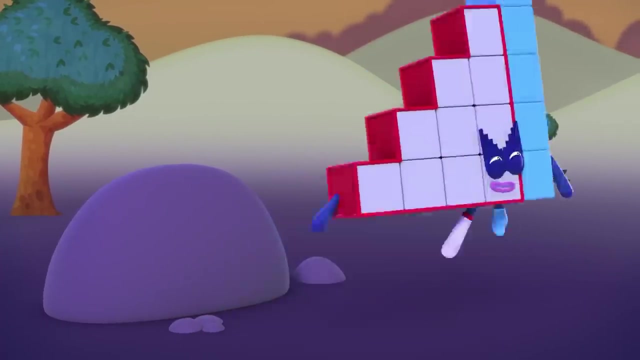 Hush, hush. I am fifty And I am a super special, step-shaped secret agent. I'm a number with ambition. I'm a number on a mission With a talent that you won't believe, Despite my size. I'm a master of disguise And I've got a little trick up my sleeve. 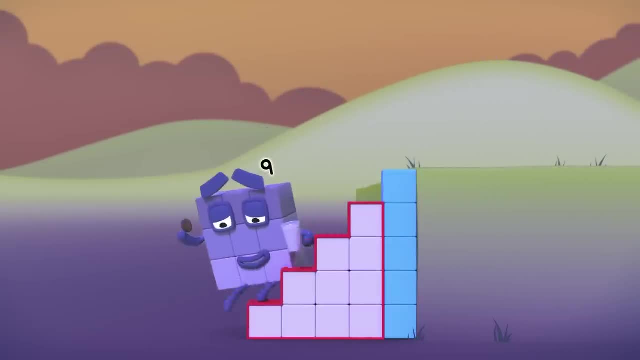 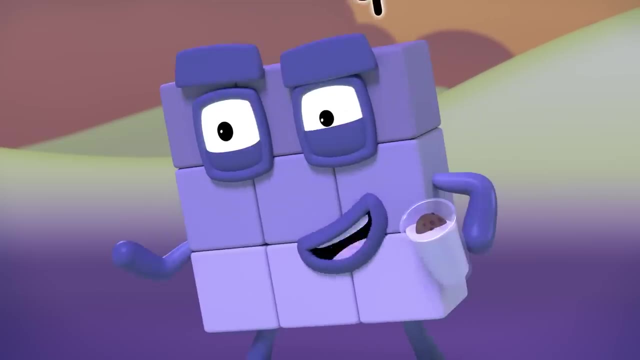 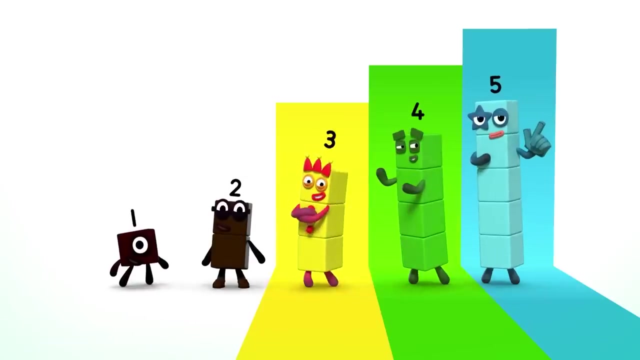 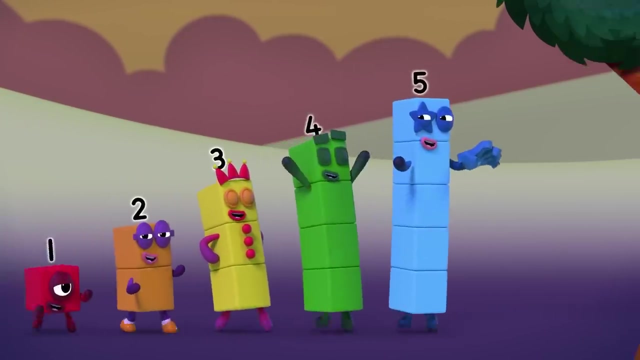 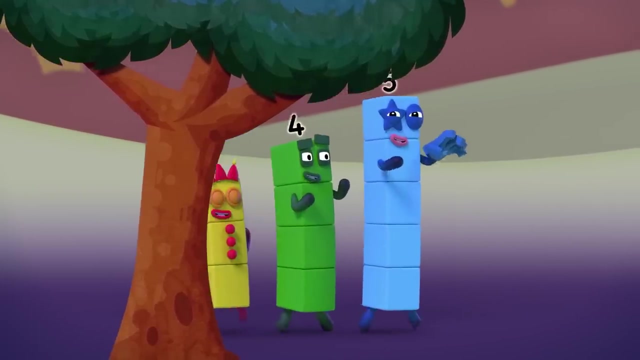 Hush, hush, Help, My biscuit has fallen into my milk. This is a job for Step Squad Five, Four, Three, Two, One Step Squad. We're the Super Special Secret Step Squad. We can make your problem disappear. We're the Super Special Secret Step Squad. 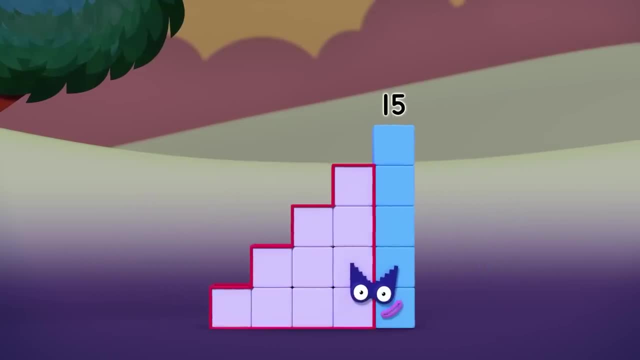 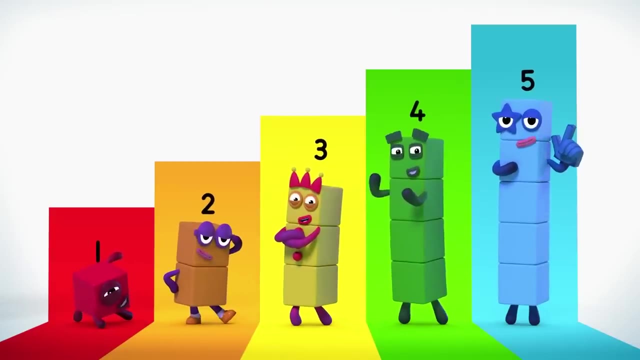 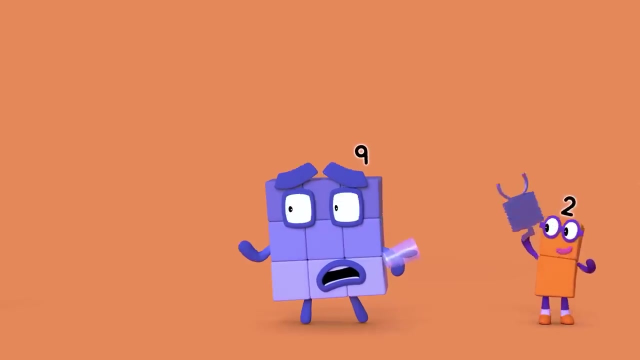 We're gonna make it better. You'll never even know I was here. The Super Special Secret Step Squad is here. Step one: remove the milk. That'll get you started. Step two: remove the biscuit, And now we're on our way. Step three: replace the milk. 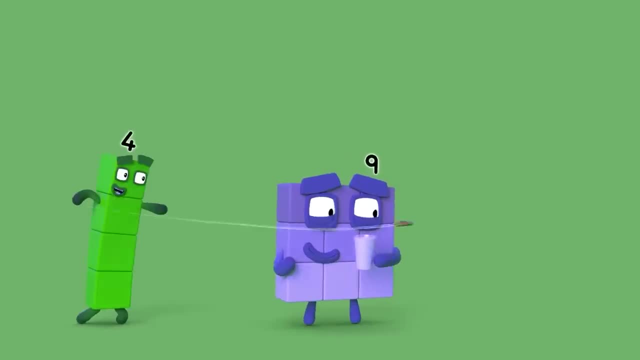 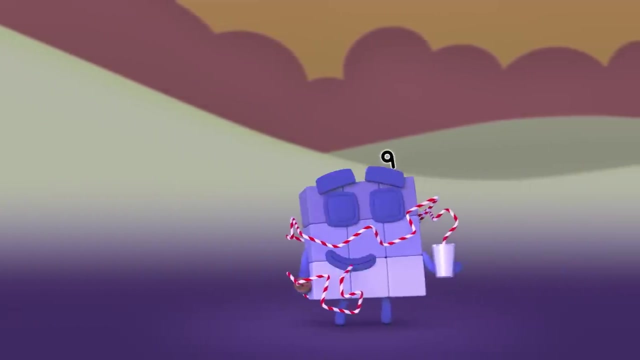 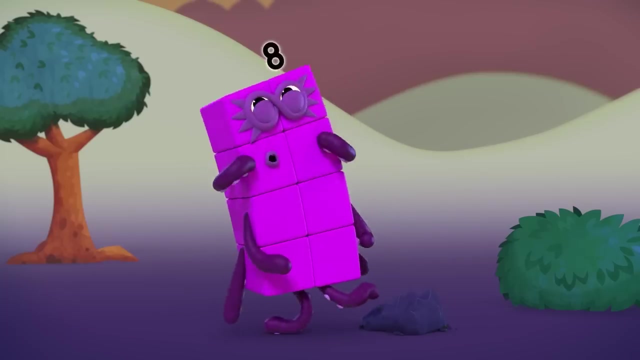 Oh, Don't be downhearted. Step four: replace the biscuit, We're gonna save the day. Step five: We're going to overdrive As we give you a straw, Thanks, And vanish away. Yum yum, Octoblock. ouch, I've got an octo-boo-boo. 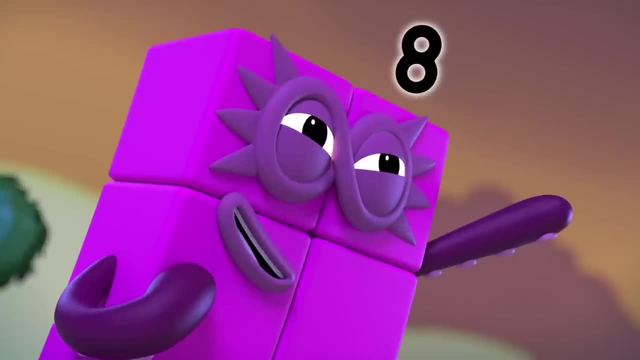 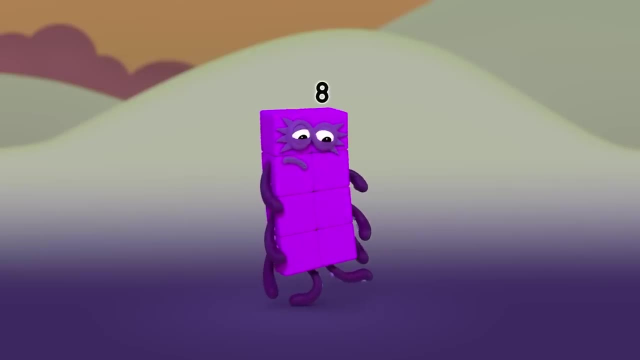 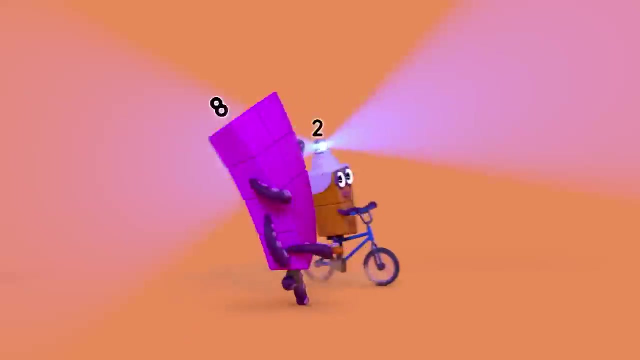 This is a job for Step Squad. The Super Special Secret Step Squad is here. Step one: check the boo-boo, That'll get you started. Step two: knee-no, knee-no, And now we're on our way. Step three: see the doctor, Don't be downhearted. 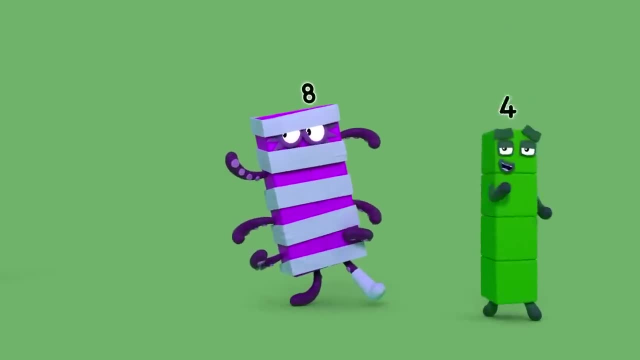 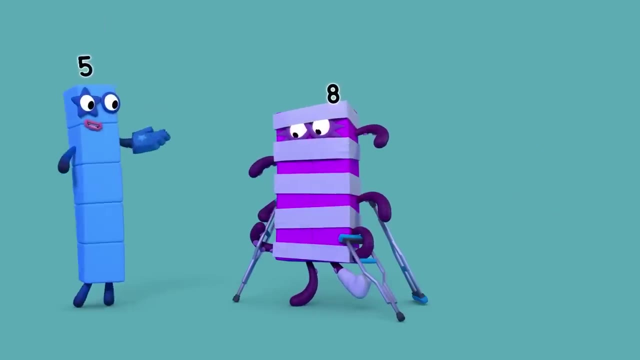 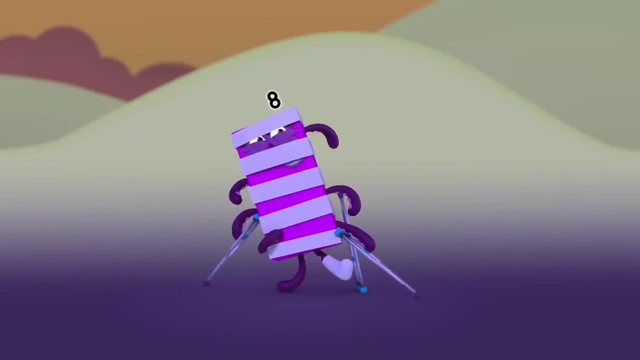 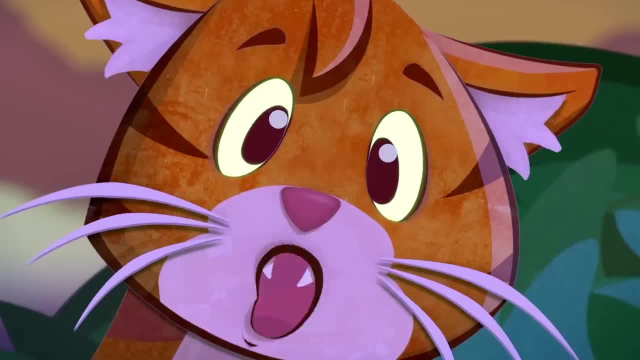 Meow, meow. The Super Special, Secret Step Squad is here. Step one: get a ladder, That'll get you started. Step two: light up the tree, And now we're on our way. Step three: call an alien, Don't be downhearted. Step four: beam up the cot. 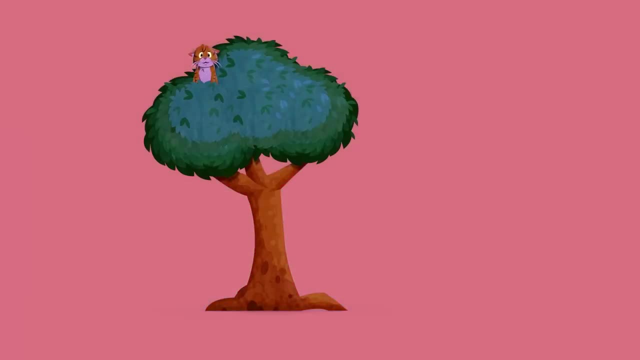 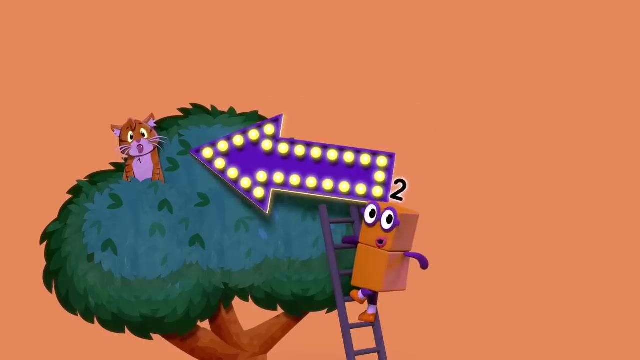 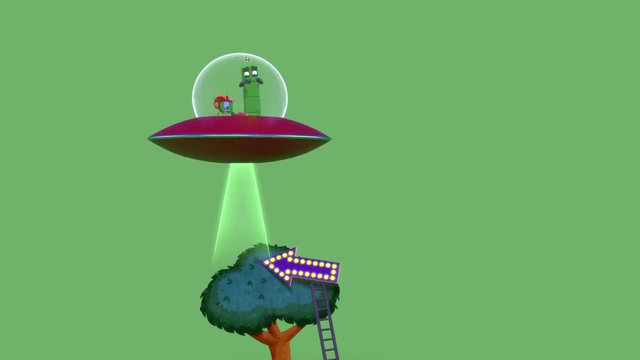 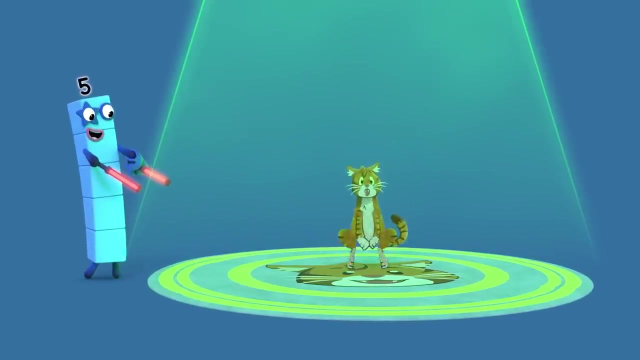 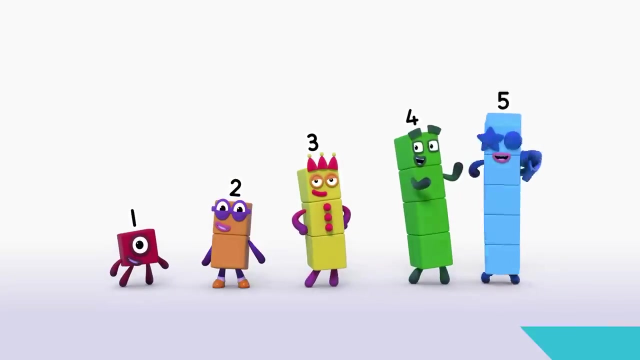 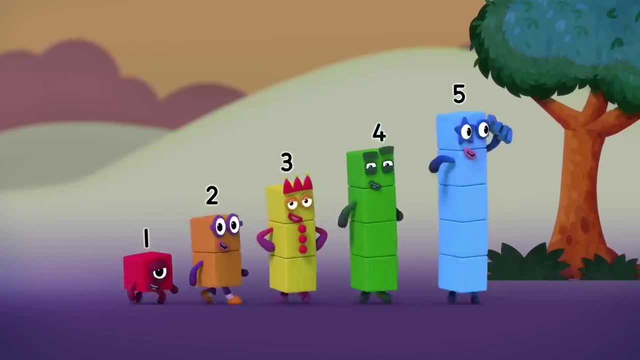 We're gonna save the day And vanish away. Step six: use the's Step five. we go into overdrive As we beam it back down And vanish away. Five, four, three, two, one Step Squad. We're the super special secret Step Squad. 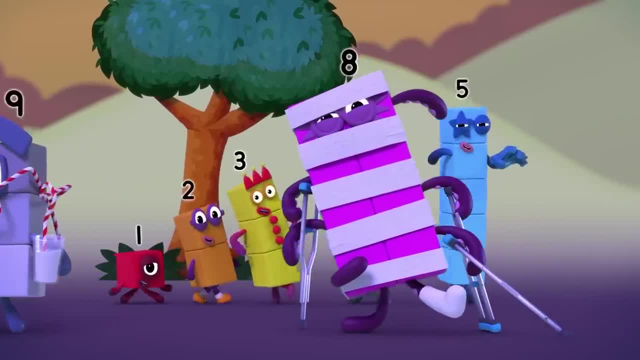 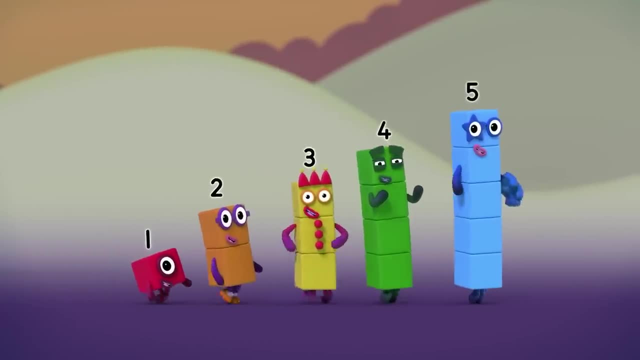 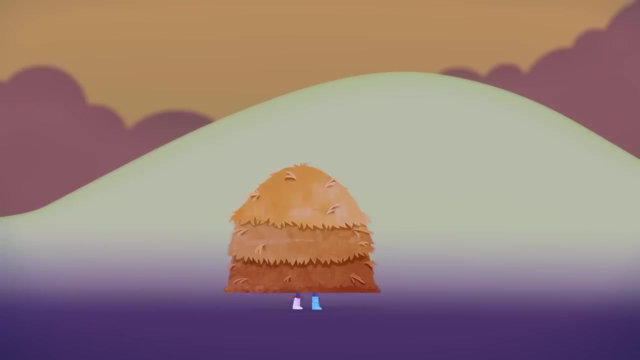 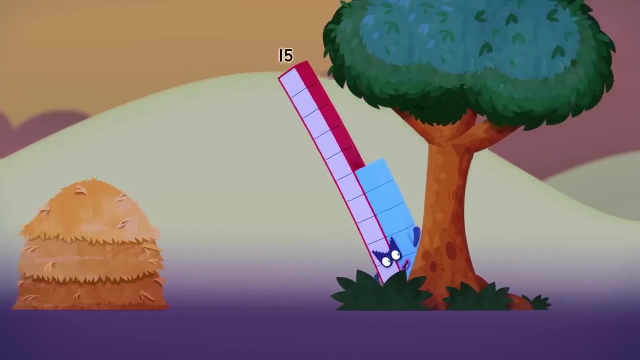 We can make your problem disappear. We're the super special secret Step Squad. We're gonna make it better And you'll never even know we were here. I'm a number with ambition. I'm a number on a mission, With a talent that you won't believe, Despite my size. 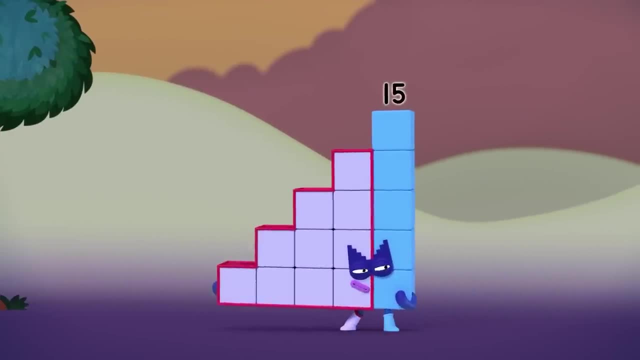 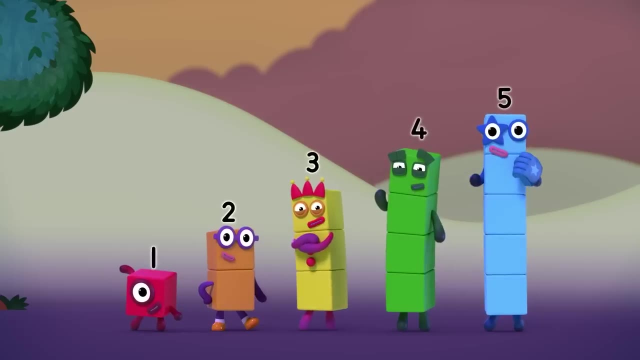 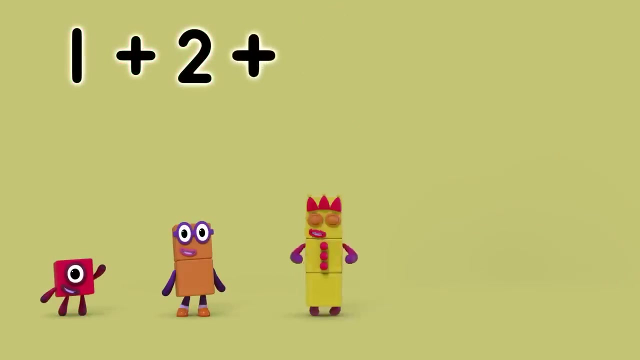 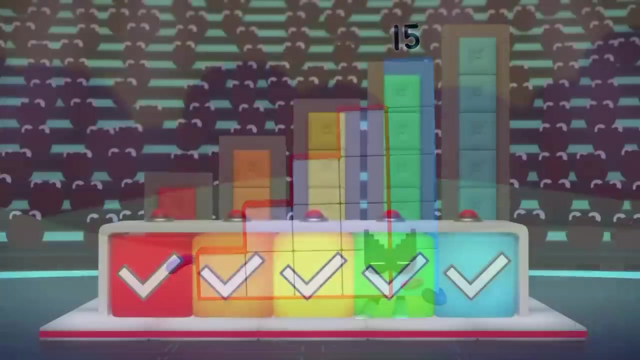 I'm a master of disguise And I've got five friends Who will come and solve your problem. Then we'll leave, Cause we're the super special secret Step Squad. One plus two plus three plus four plus five Equals fifteen. Hush, hush. Welcome back to Fifteen's Minute of Fame. 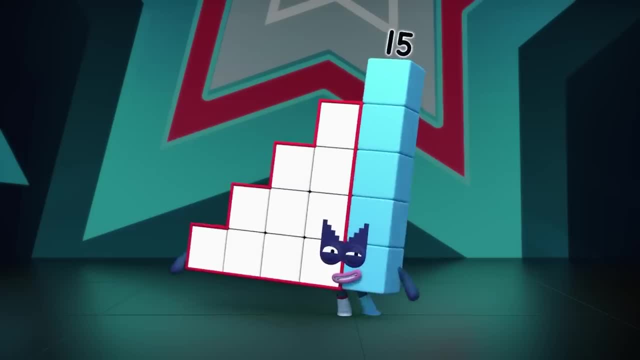 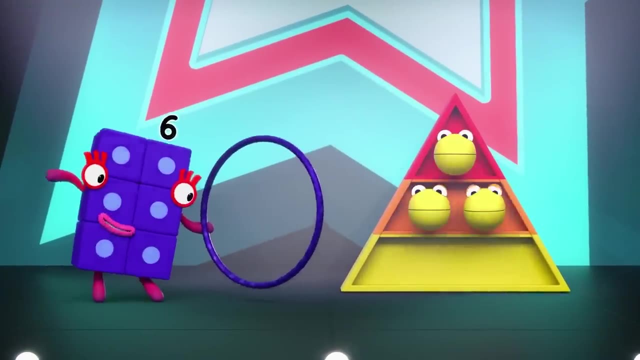 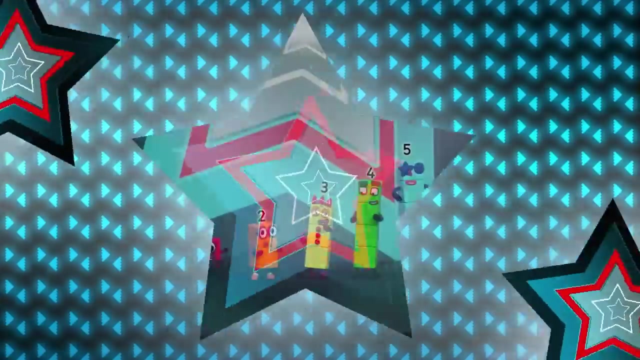 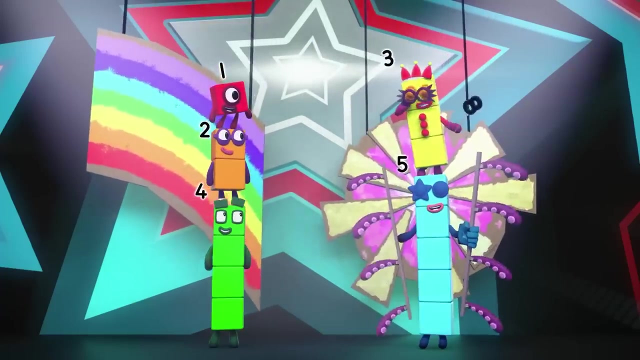 The show where number blocks show you their tremendous talents. So far tonight we've seen Six and her boxcar In number blocks One, two, three, triangle, Four, five, six, triangle, Impressive impressions. Octoblock to the rescue- Oh, that's lucky. 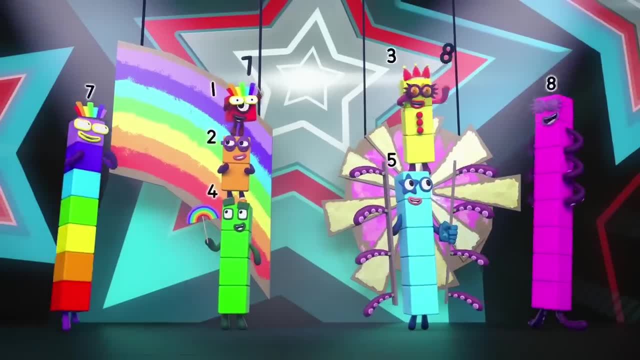 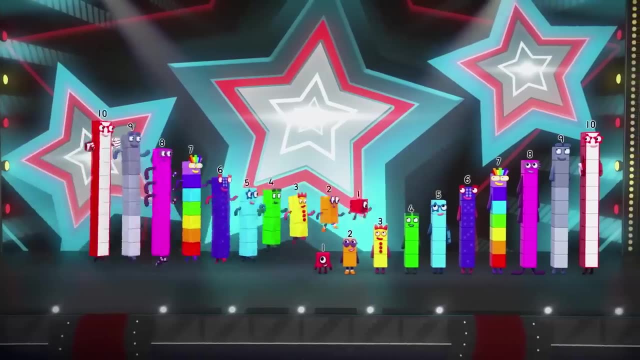 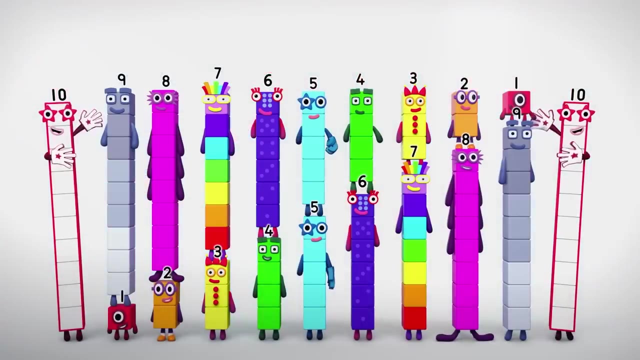 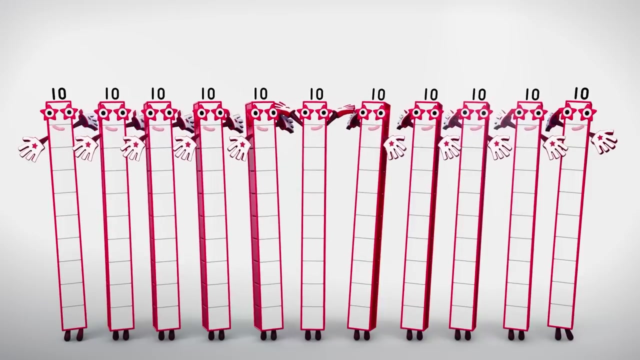 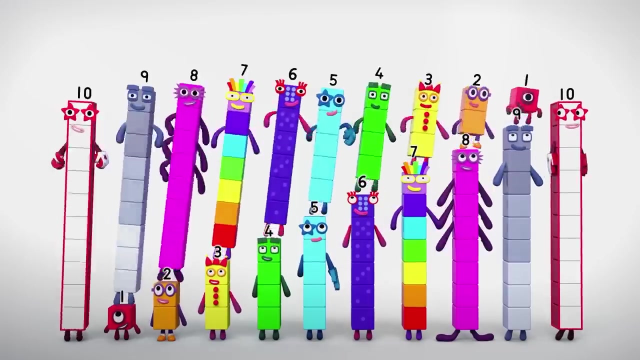 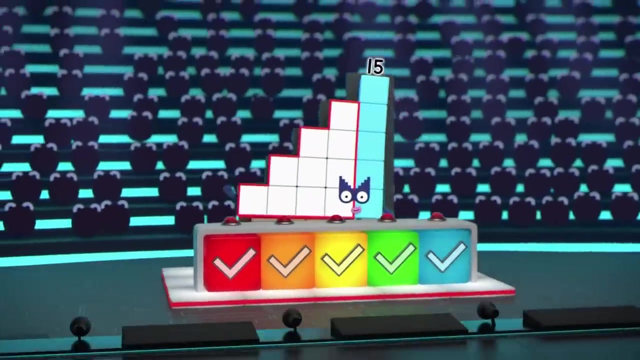 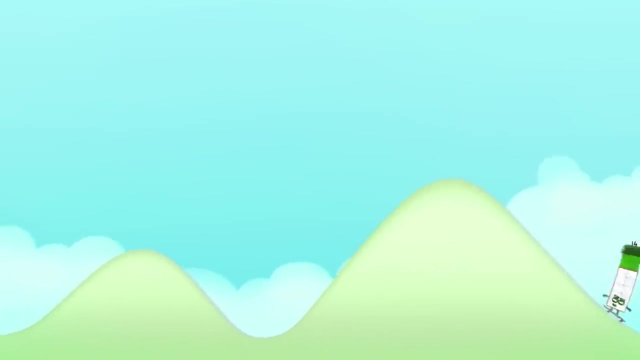 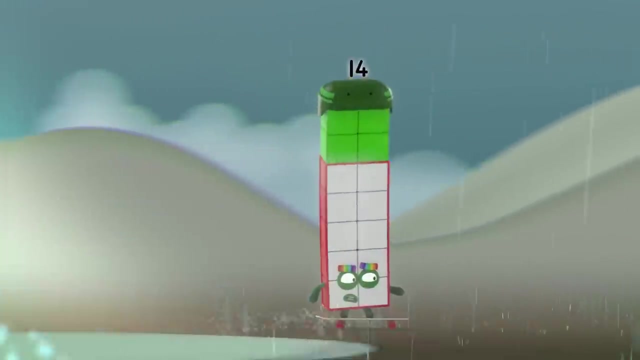 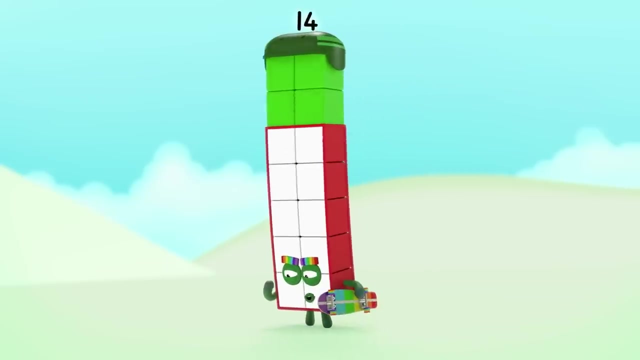 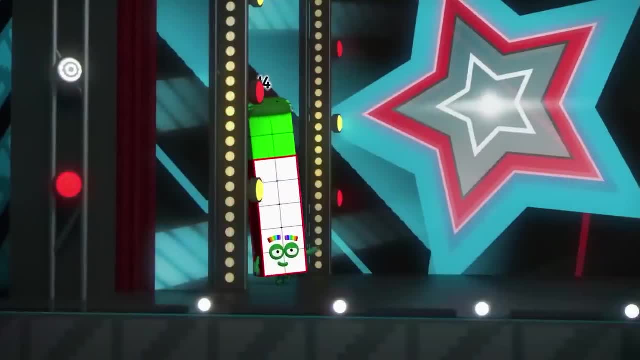 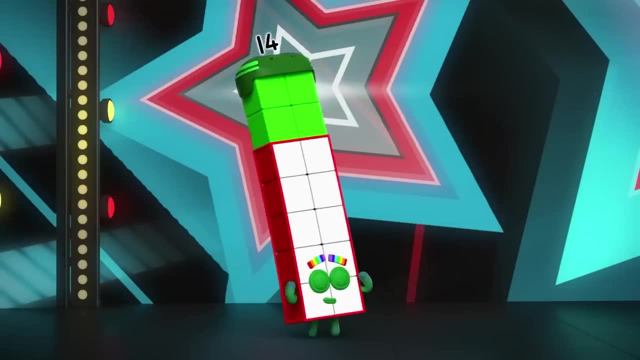 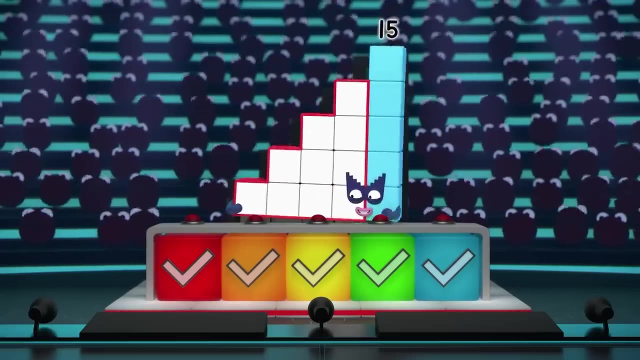 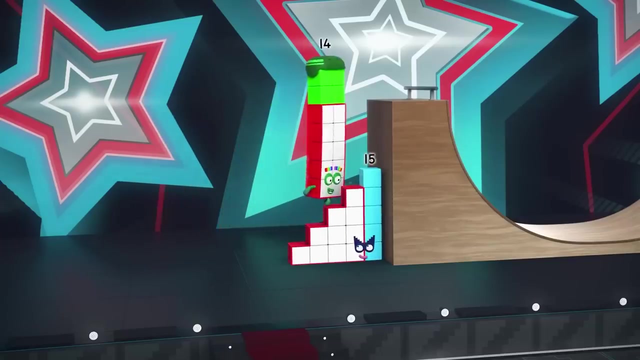 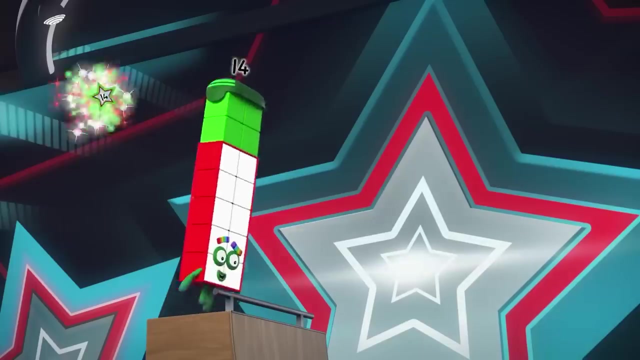 makes perfect. welcome to 15's minute of fame. show us what you've got- 14.. no problemo, but i need a volunteer for this trick. no, no, i'm not the act he is, i'm just helping him take a decision. the next level: 14. oh no, i forgot my skateboard. 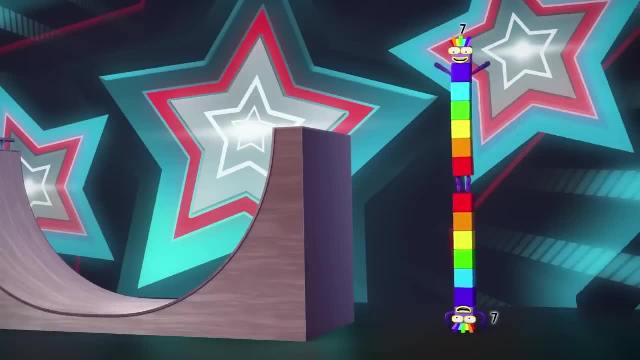 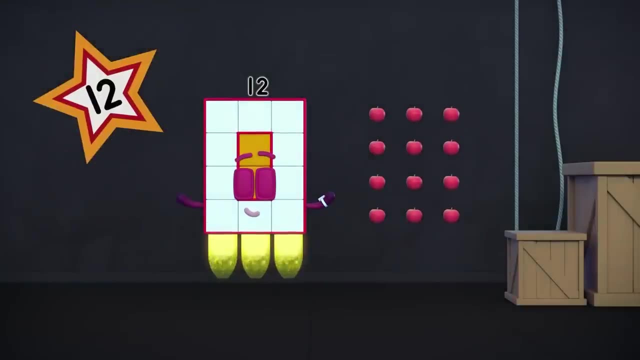 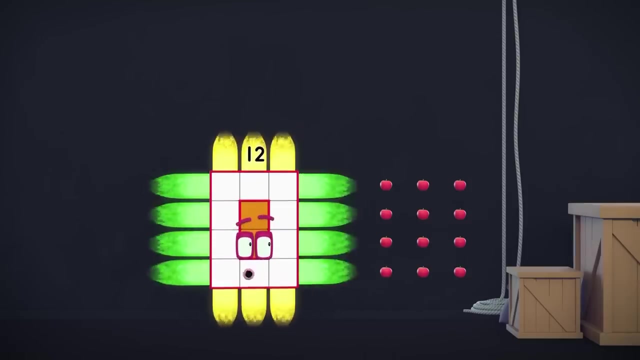 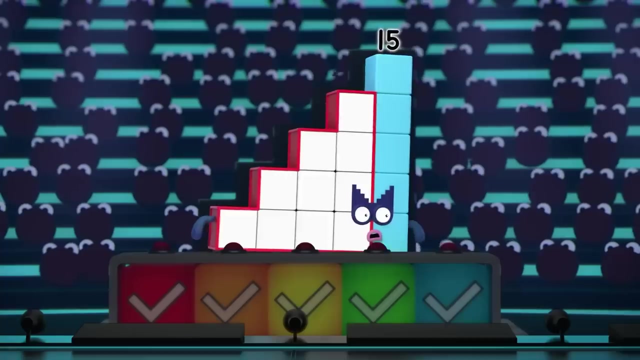 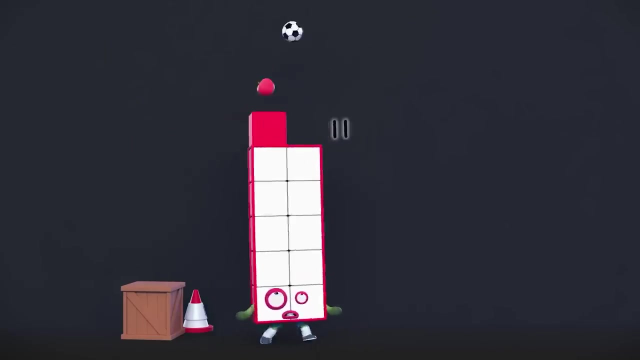 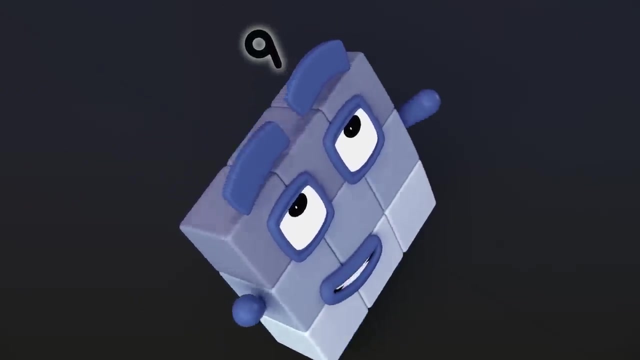 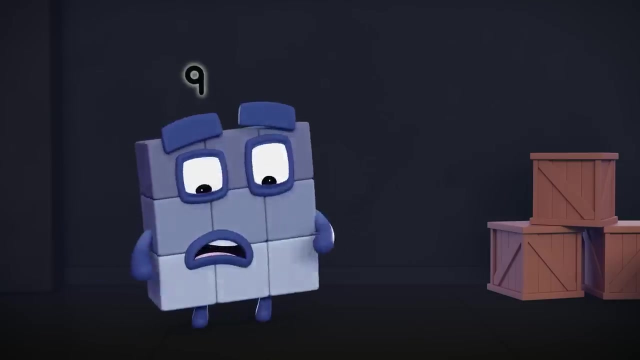 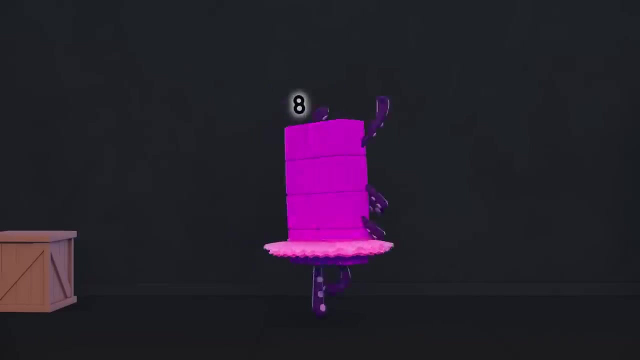 yup, that was lucky, double lucky, i found it 13. 12.. no, no, three by four, switch, two by six, 11. oh dear, i've got it nice. eight octoblock pirouette: one, two, three, four, five, six, seven, eight pirouette seven. 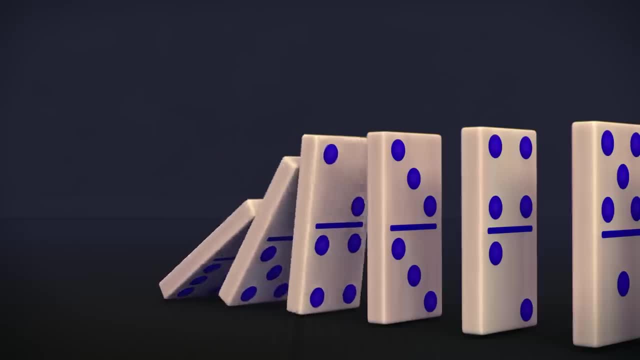 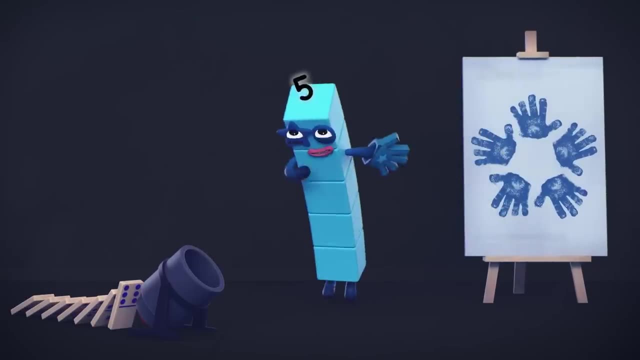 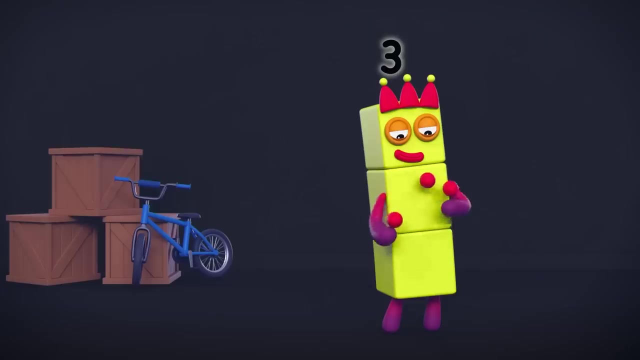 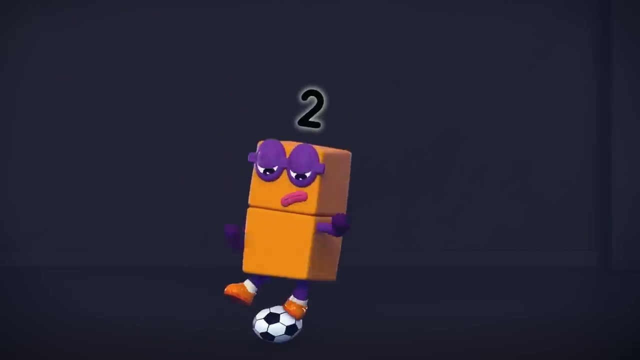 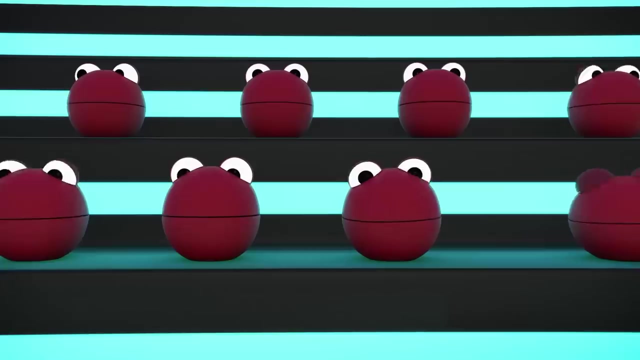 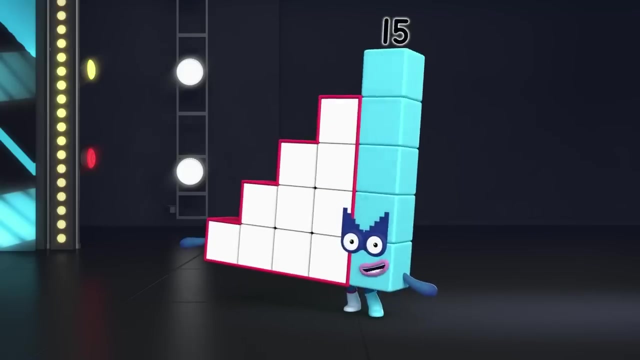 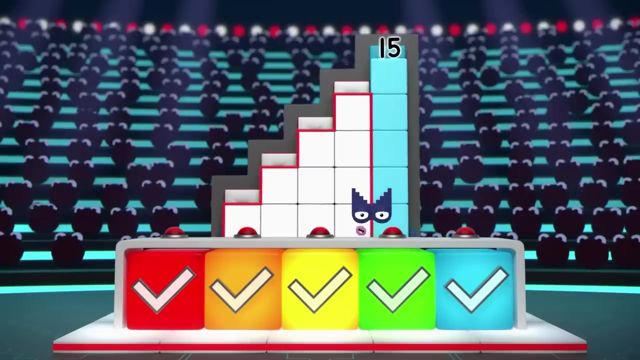 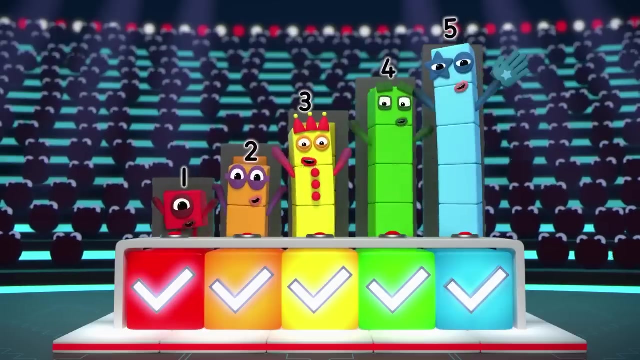 lucky me. six, five, four, screw, screw, screw, screw, road thing. three, oh look at me. two, one ups, two ups. anyone lost a football or a skateboard? zero, nothing to it. haha, let's see what our judges made of that hush 12.. everyone's a winner. 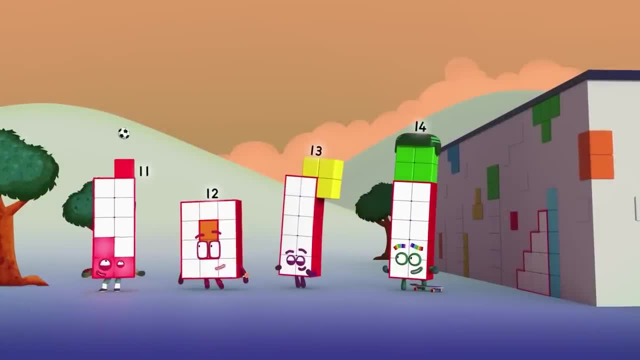 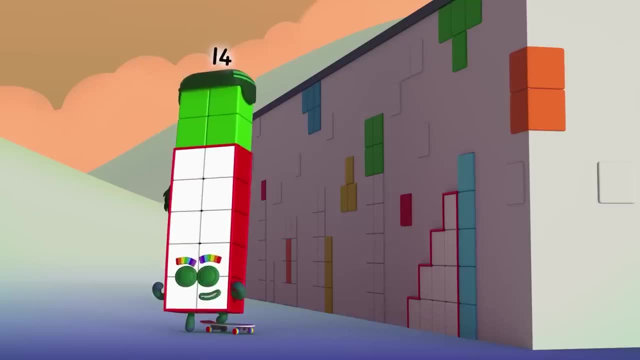 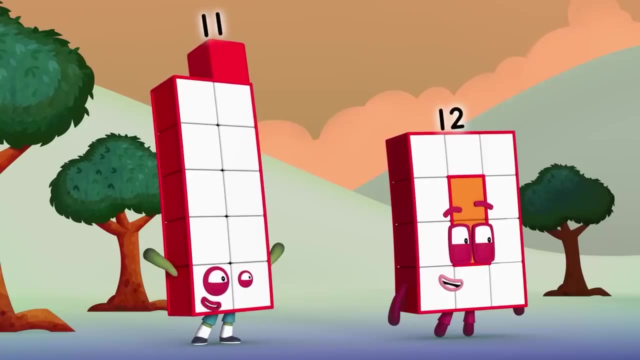 everyone's a winner. Two, three, four, five, six, seven, eight, nine, ten And one more is eleven. Whoa extreme. Let me try. Two heads are better than one Great idea. Fourteen: Everyone grab a partner for a head-to-ball contest. 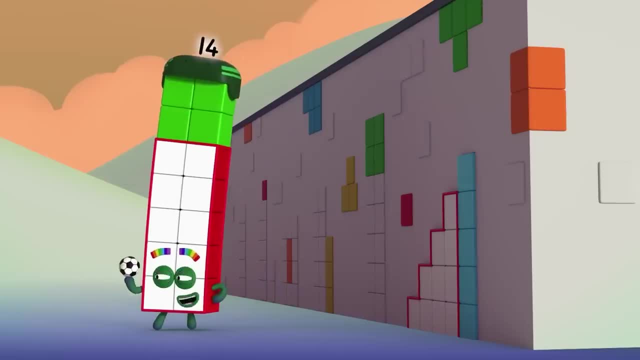 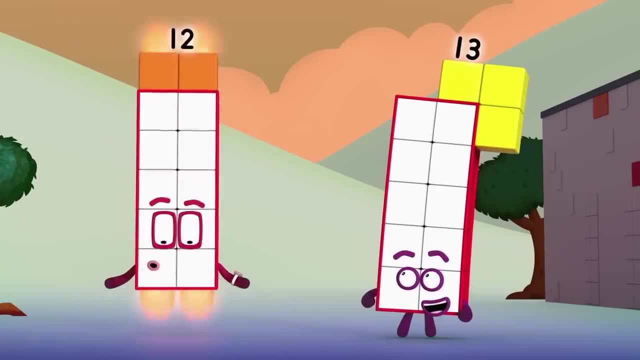 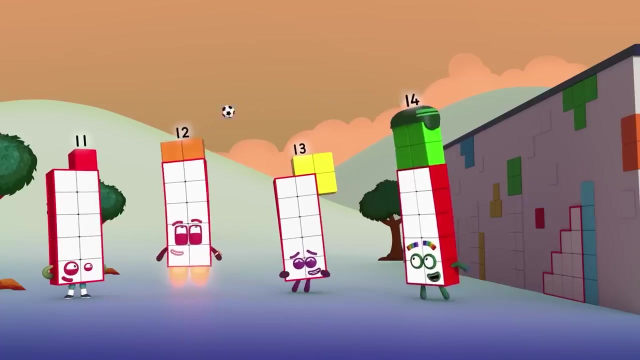 I'll be the ref. Awesome, I'll pick twelve: Time for this super rectangle to get in shape. Switch Two by six. I don't have a partner, Unlucky me. Agent Fifteen: here I'll be your partner. 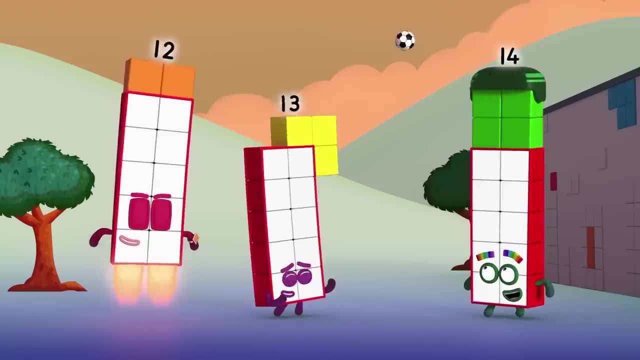 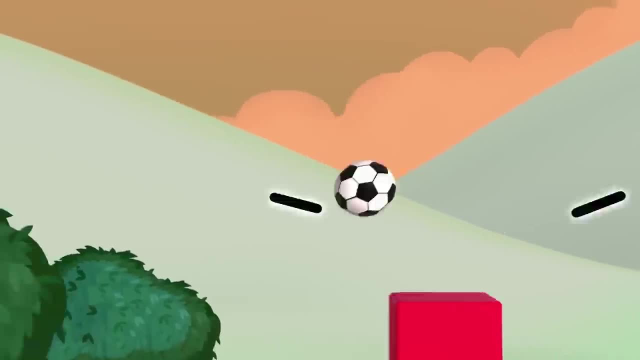 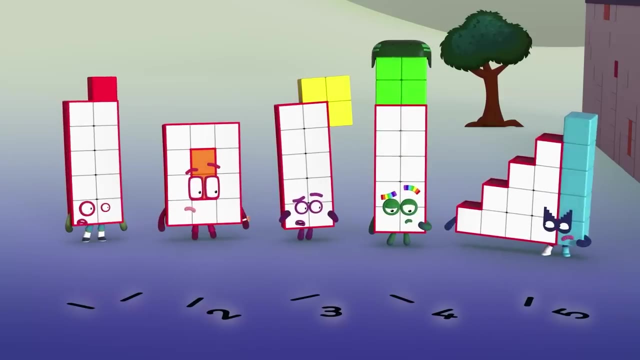 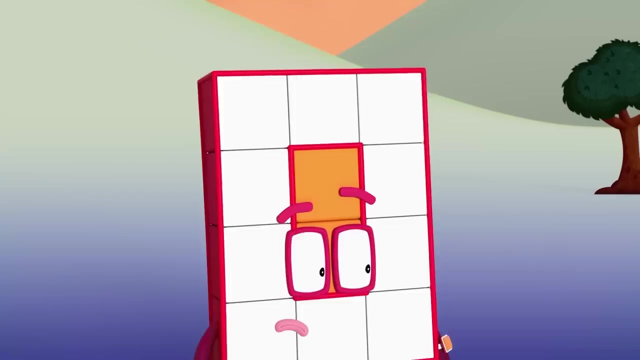 Don't say my name, Don't say Thirteen. Yes, Is everyone all right? Are you all right? Sorry, who are you? Good question, I have no idea. We've lost our numberlings. Numberlings Jumblings, more like. 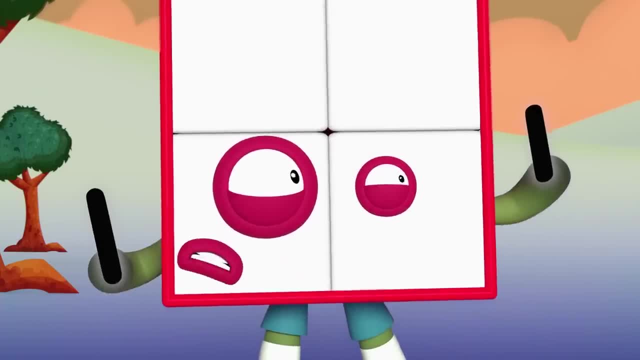 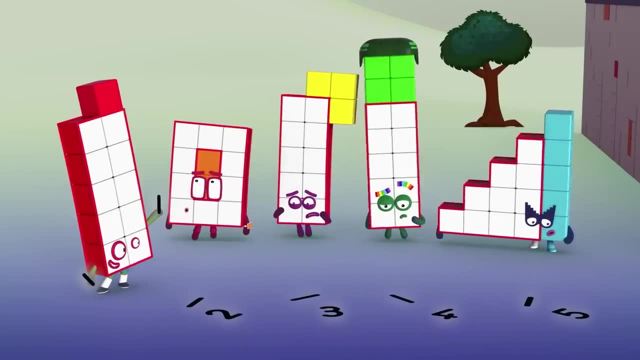 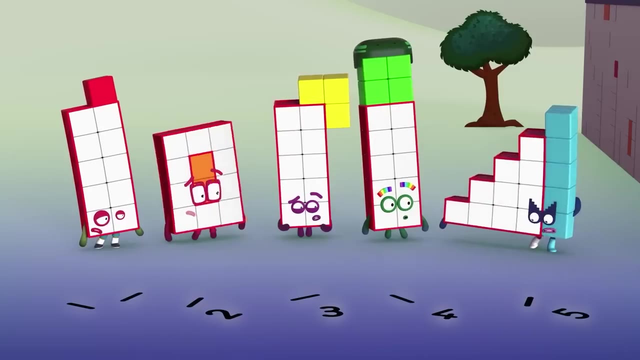 Anyone recognise their own? There's a lot of these ones. Oh, I remember It's a one. Anyone feel like number one? Oh, We've all got more than one block. I've got one. Um, well, more than one anyway. 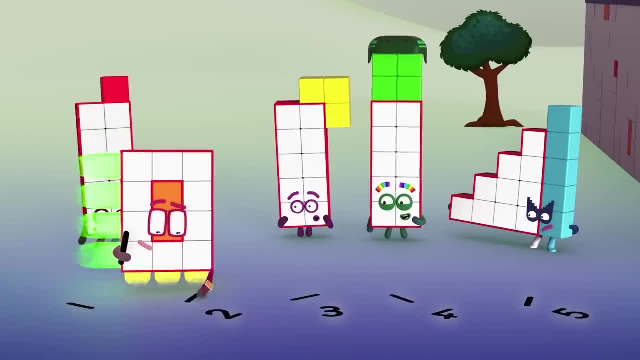 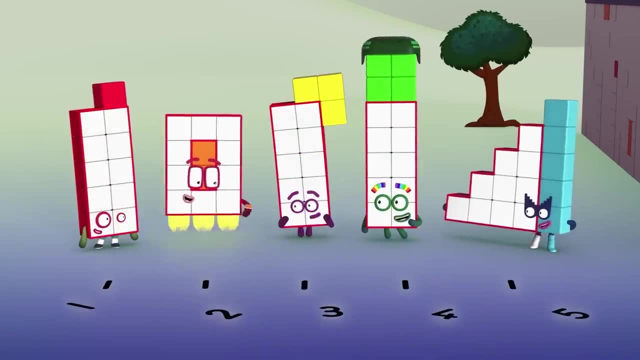 Arranging things neatly in rows can help. Oh, Oh, Oh, Oh, Oh, Oh Oh. Let's put all the ones here. Oh, Oh, Oh, Oh, Oh Oh. And then this feels right: One, two, three, four, five. 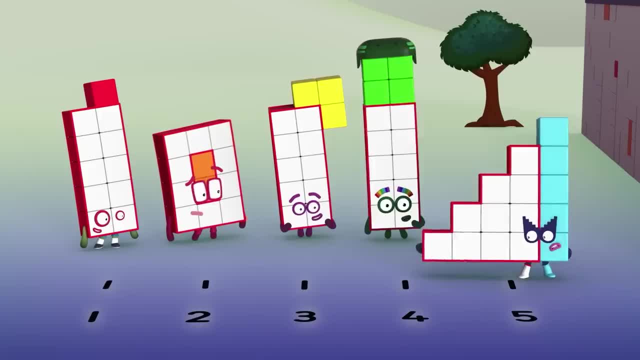 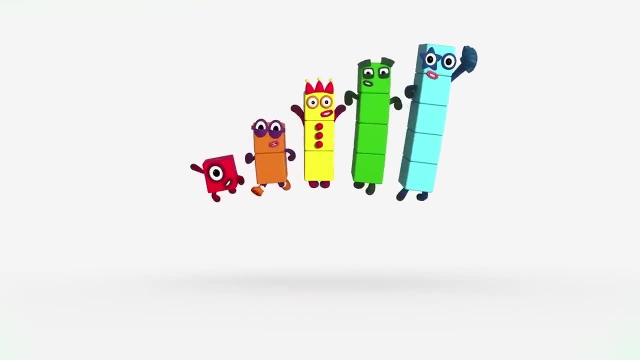 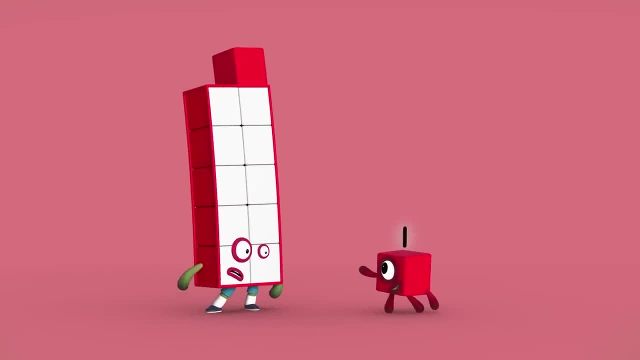 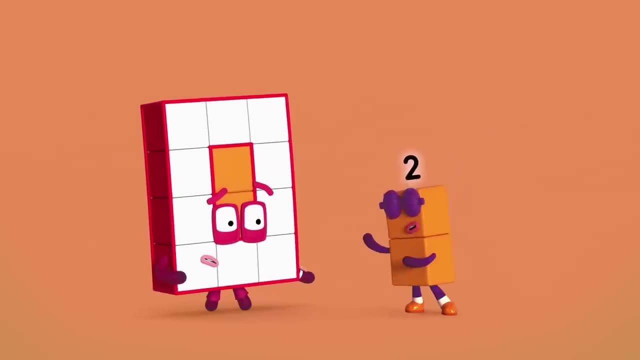 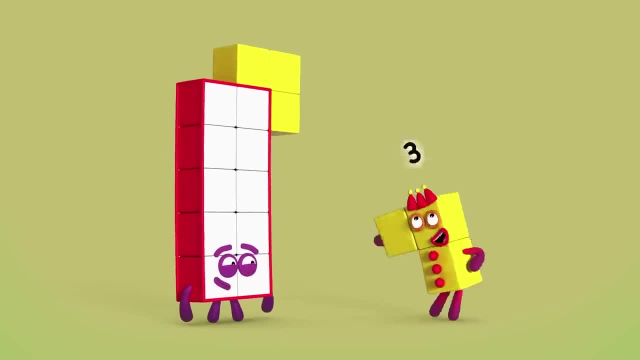 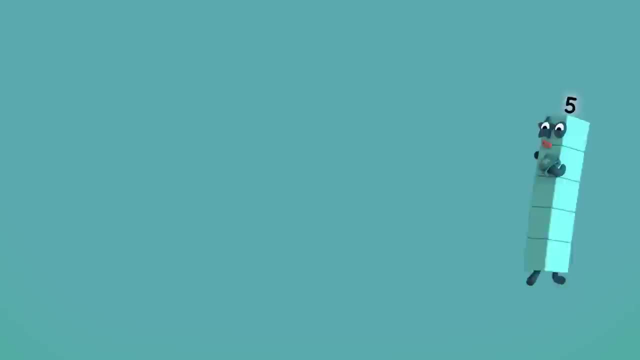 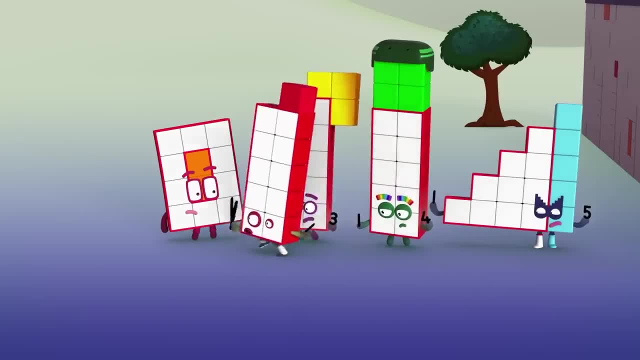 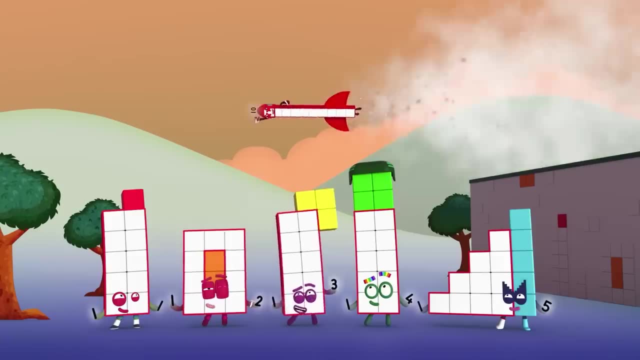 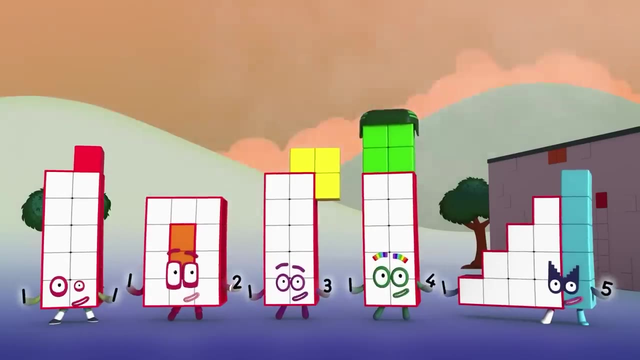 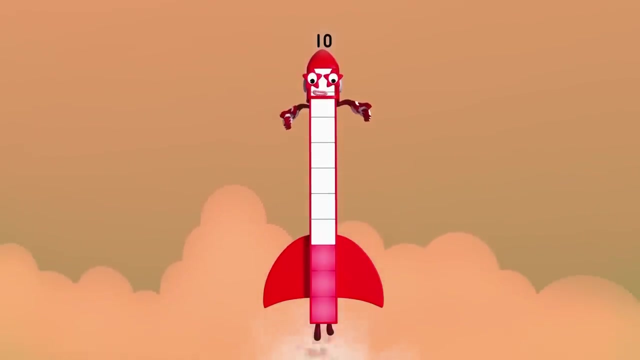 Oh, Oh Oh, Plop, Plop, Plop, Twiddle, twiddle Coming in for landing in 10, 9,, 8,, 7,, 6,, 5,, 4,, 3,, 2, 1.. 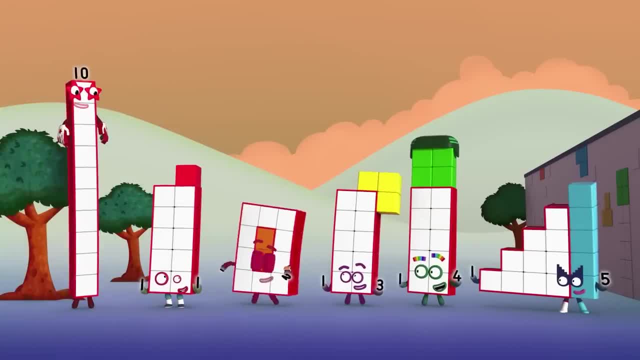 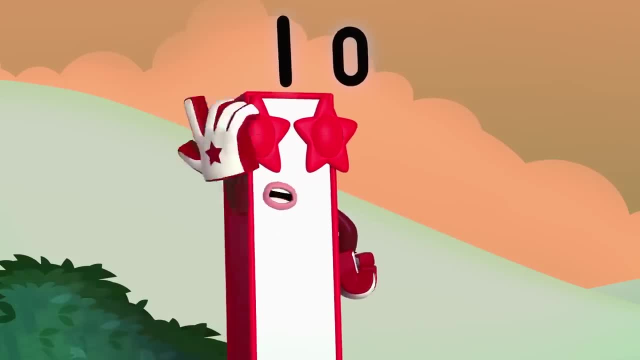 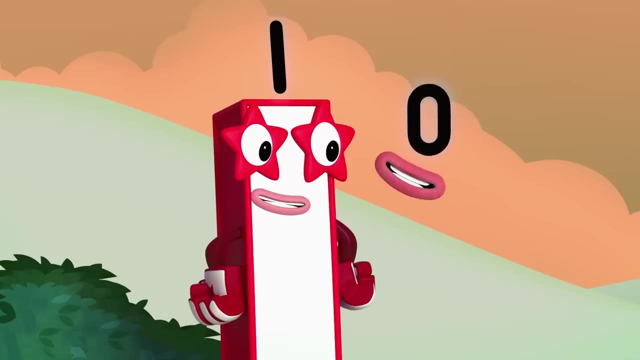 Touchdown: 10.. Your 10.. 10 lots of 1.. Or 110.. This 1 stands for 110.. 110 and no more. No more 1s. Nothing could be simpler, So each of us needs 2 numberlings. 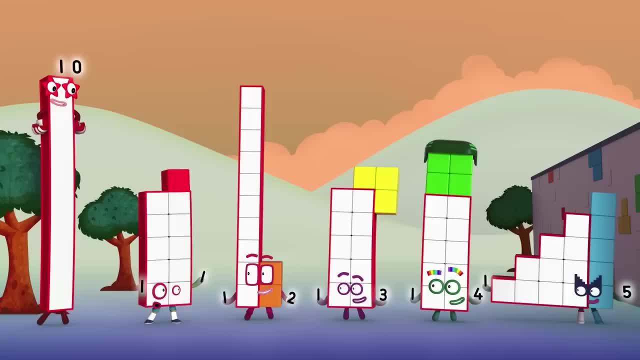 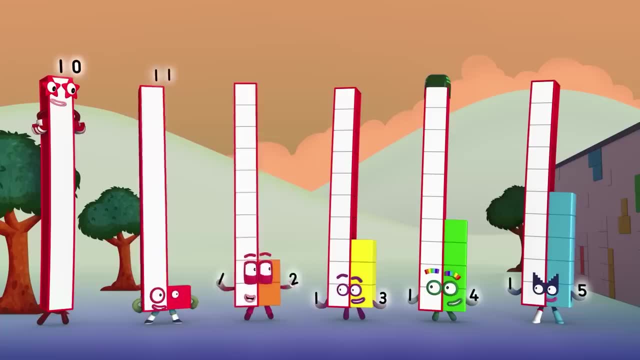 1 numberling for the big 10 block and 1 for the rest. I'm 1 10 block and 1 block more. I'm 11.. I'm 1 10 block and 2 1 blocks. I'm 12.. 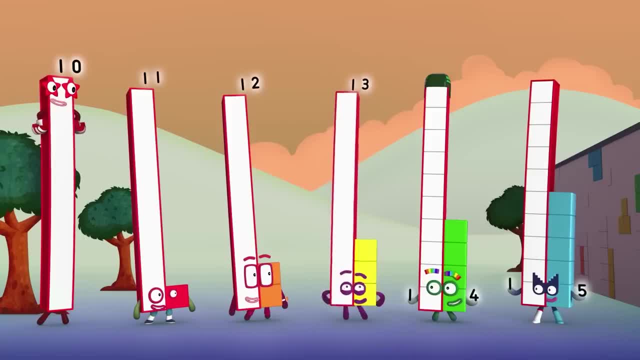 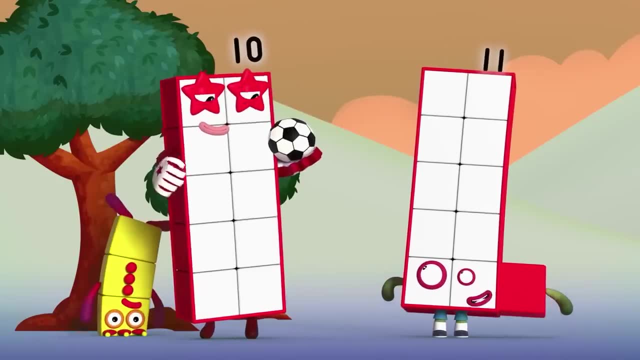 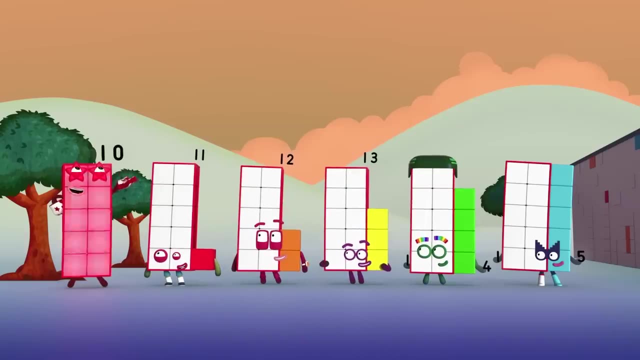 I'm 1 10 block and 3 1 blocks. I'm 13.. Duck, Duck, Duck, Nice, save 10.. Thanks. Now where were we? 1, 10 and 0, 10.. 1, 10 and 1, 11.. 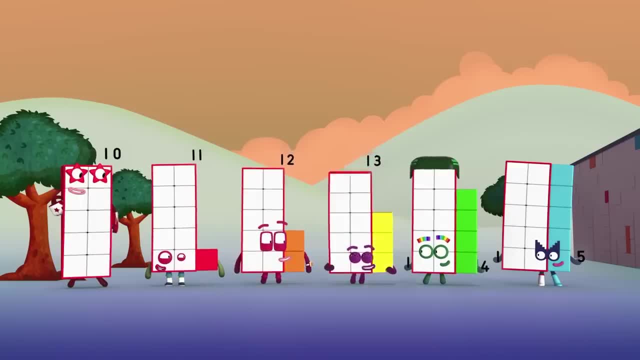 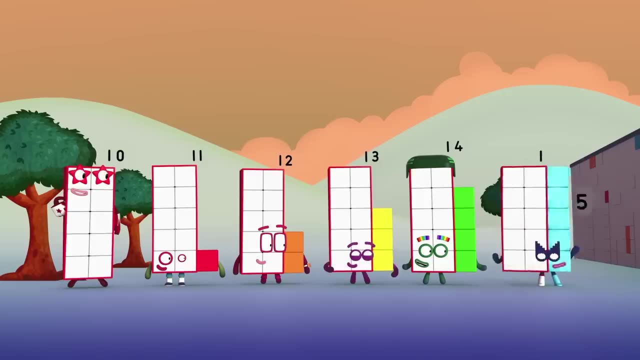 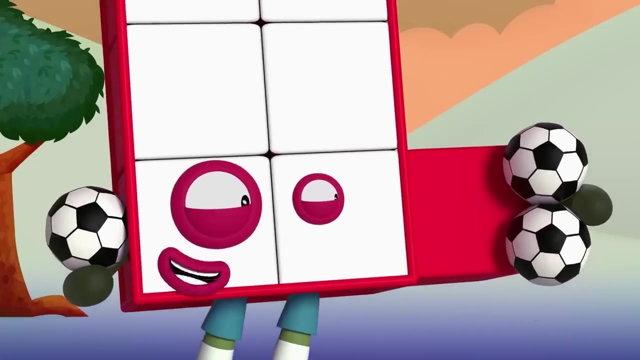 1- 10 and 2, 12.. 1- 10 and 3, 13.. 1- 10 and 4, 14.. 1- 10 and 5, 15.. Now we can play. Come on everyone. 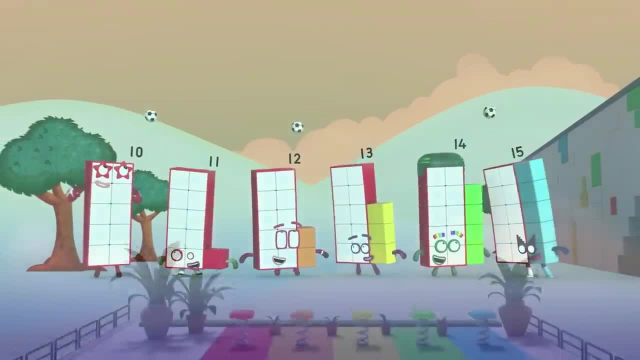 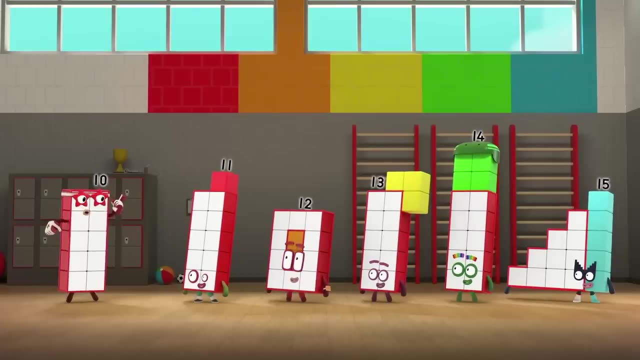 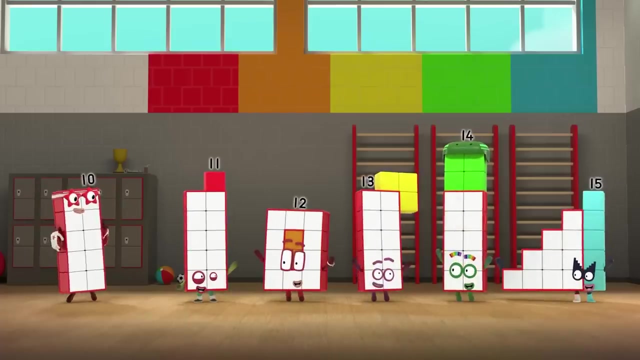 On your heads. Come on, Welcome to 10s Place. All of you are bigger than me. That means each of you has a 10 inside. you See, You are greater than 10. And you've got big dreams. You want fun. 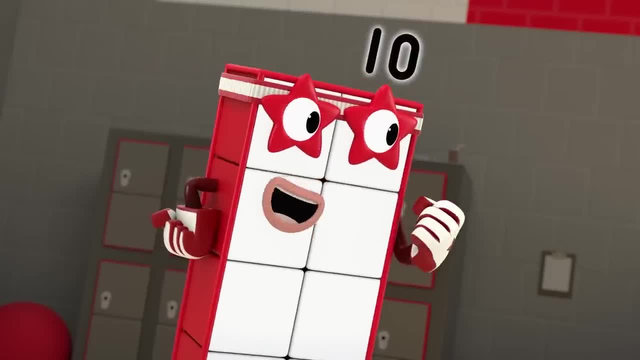 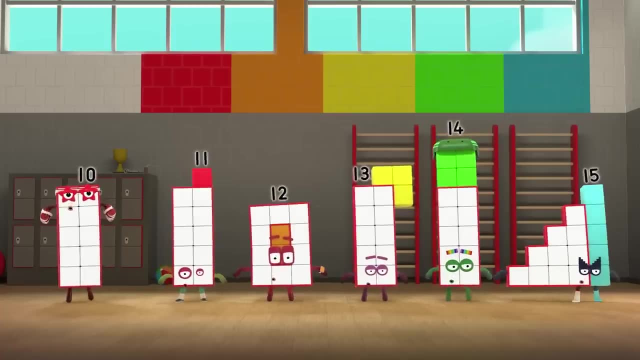 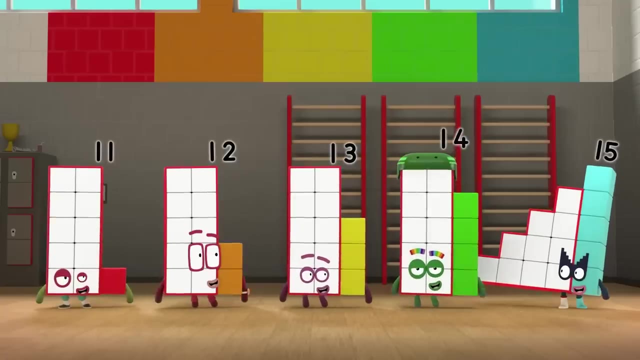 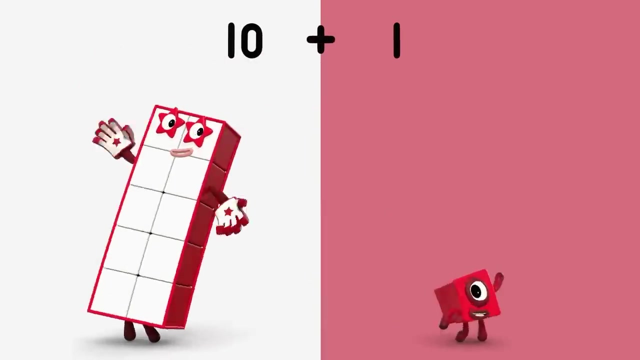 Well, fun it is. And right now is where you start playing Wow. Okay, let's pump those numbers. That's right Now. give me some squats. Let me see you do the jump and bump. Ten Plus one is eleven. Ten Plus two is twelve. 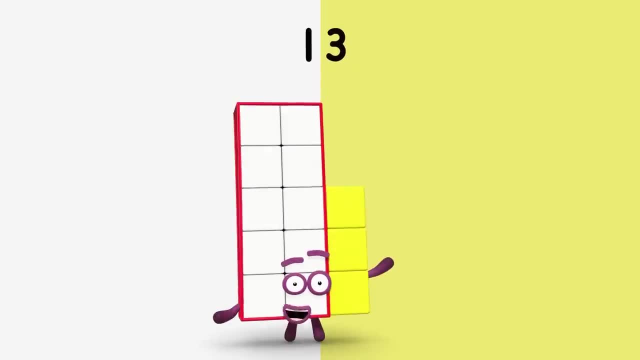 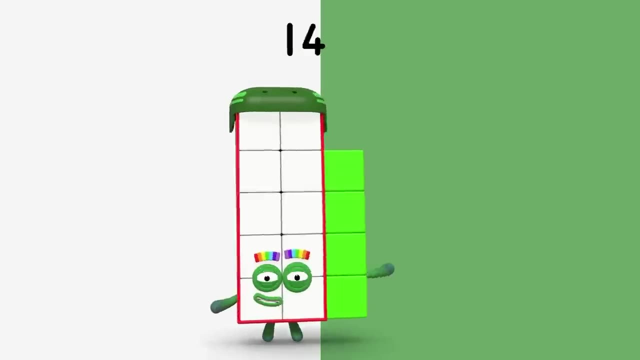 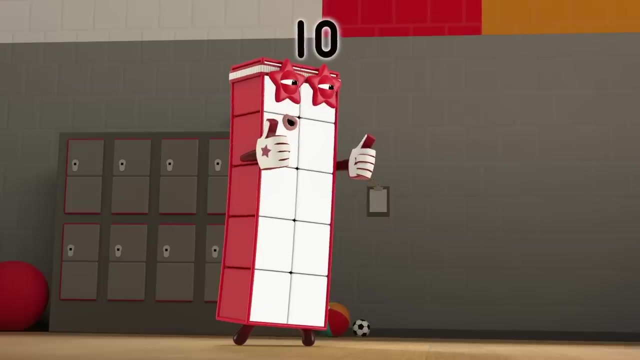 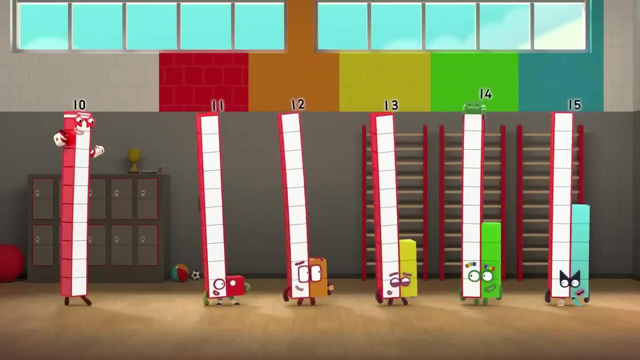 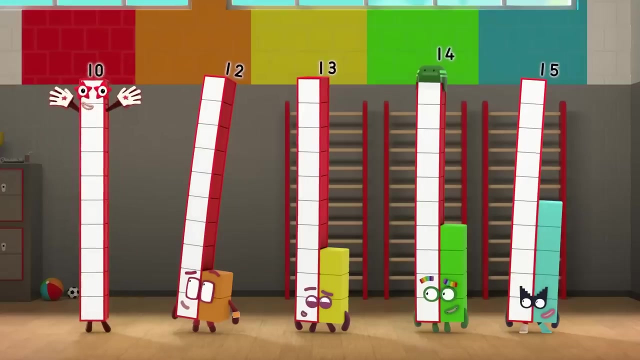 Ten Plus three is thirteen. Hooray, Ten Plus four is forty. Ten Plus five is fifteen. Terrific, Now let's stretch our tens Nice and tall. Bling those ones high in the air. Take it away. Eleven minus one is ten. Twelve Minus two is ten. 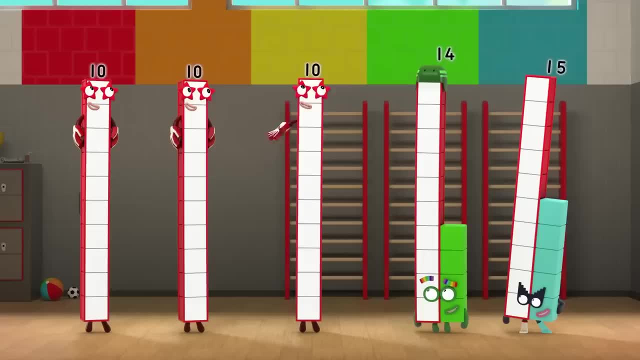 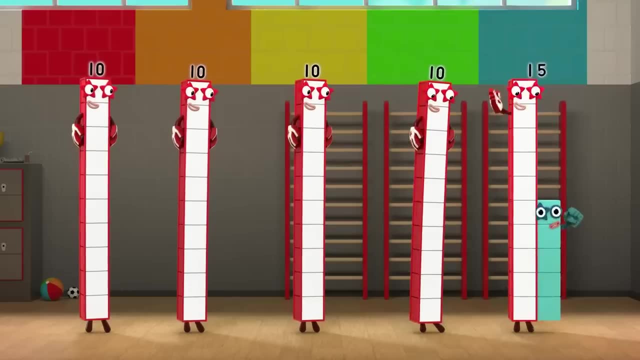 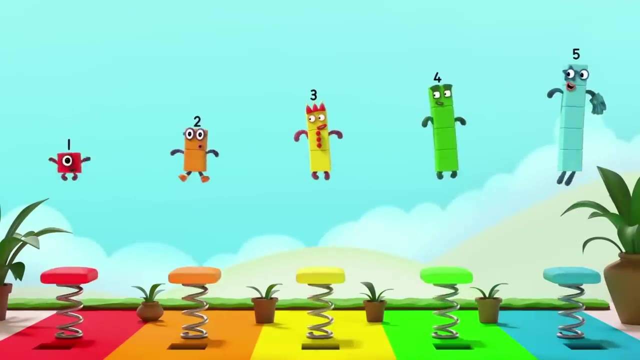 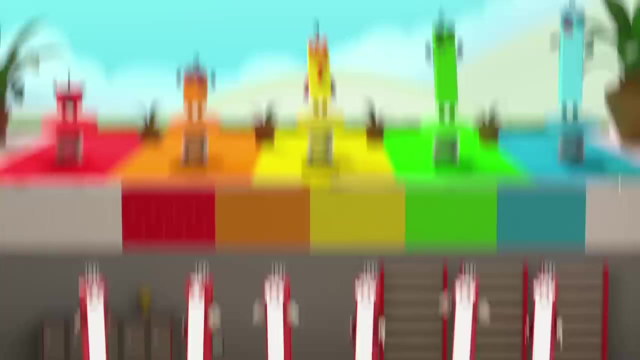 Thirteen Minus three is ten. Fourteen Minus four is ten, Fifteen Minus five is ten. Boing, woe, Boing, woe, Boing, woe. One, two ones, Three ones, four ones, Five ones. Ready, Let's work, those tens. 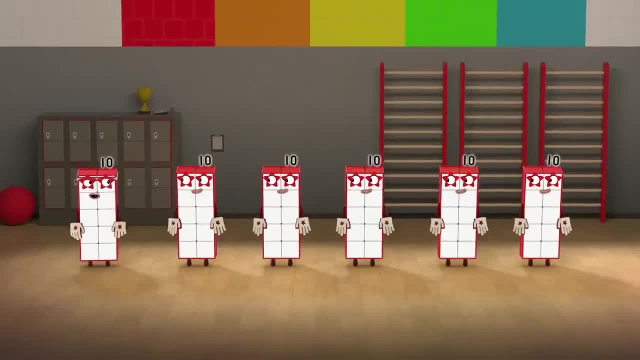 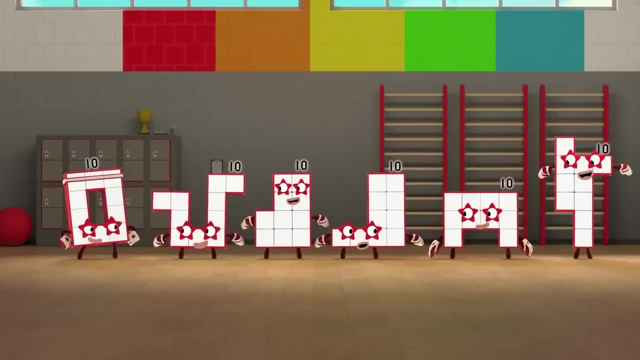 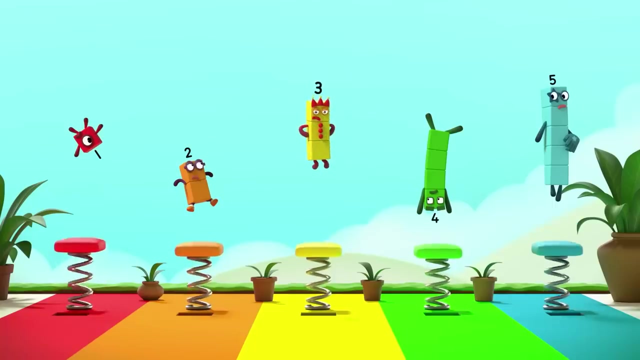 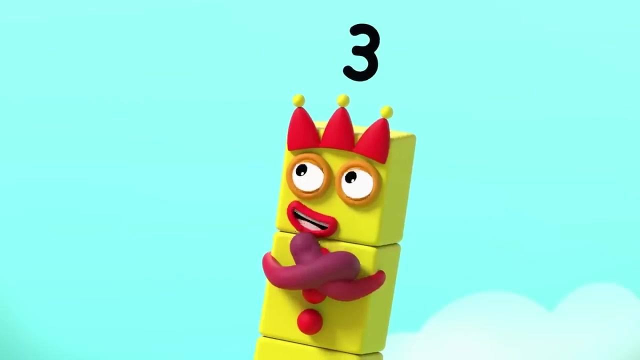 Yeah, Tall, Slide Two, I's Slide and go low, Rectangle with a hole And freestyle. Yeah, Boing, woe, Boing, woe, Boing, woe, Stop, Stop, Stop. If this is tens' place, where are the tens? Errr, I say we make this floor three's place. 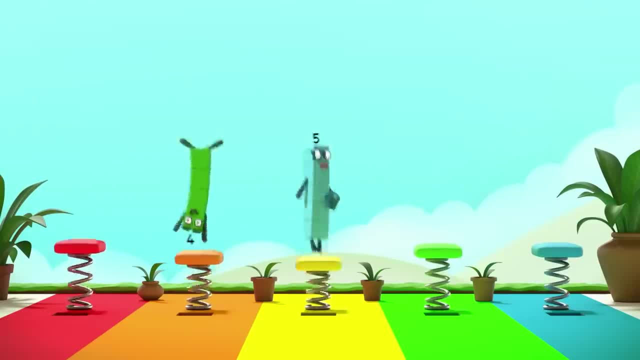 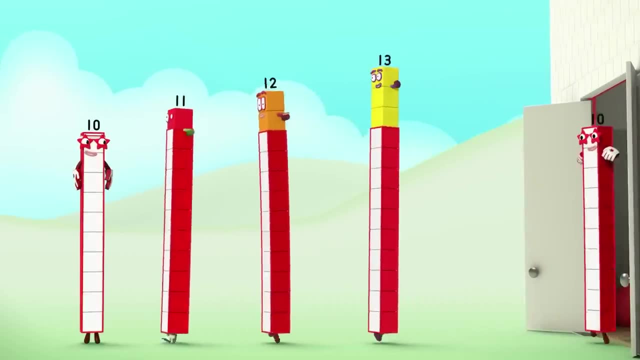 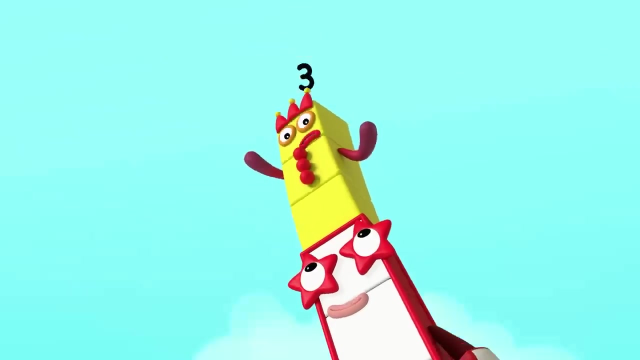 Uh, Everyone off Boing, woe, Boing, woe, Boing, woe. Ten, Eleven, Twelve, Thirteen, Wahoo Fourteen, Fifteen. Welcome to. Oh, It's a bit high up here. Put me down. All of you are bigger than me. 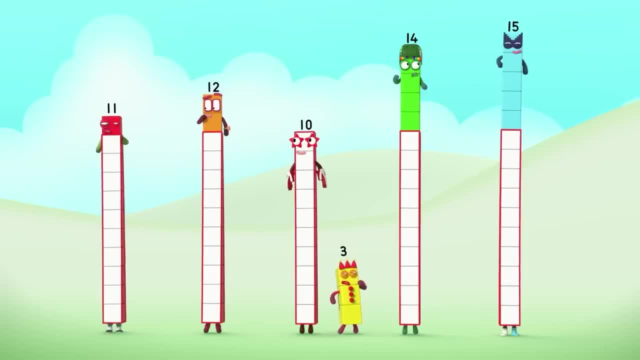 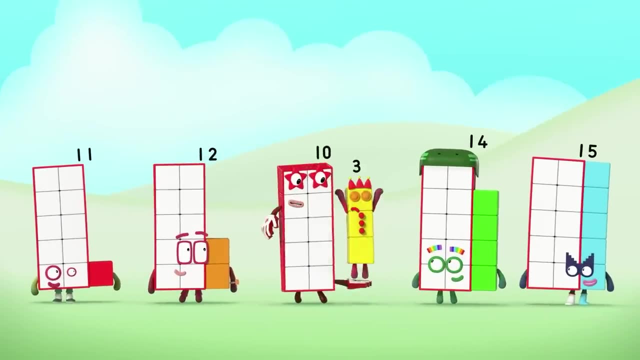 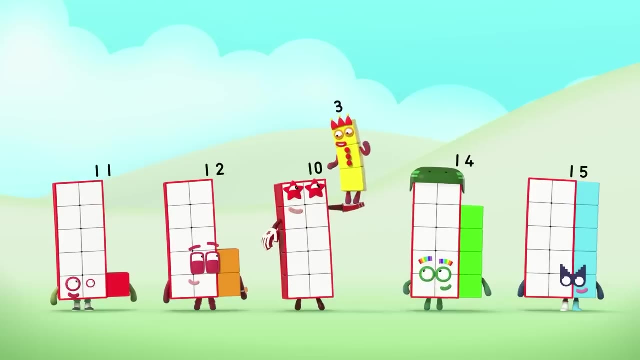 So make yourselves shorter, Even shorter. You've all got a three inside you, Well, except for Thirteen. He already pinged the part into Ten and me, Oh, Fourteen. You're one more than Thirteen, Extreme Fourteen. 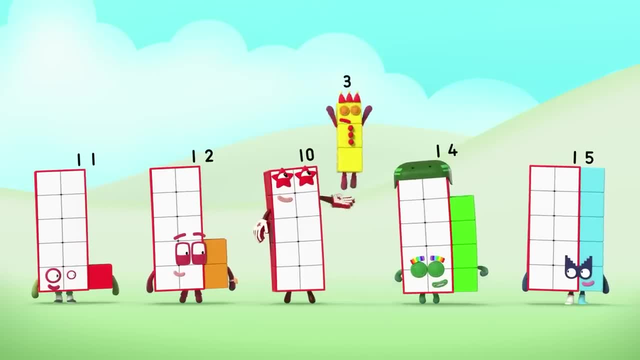 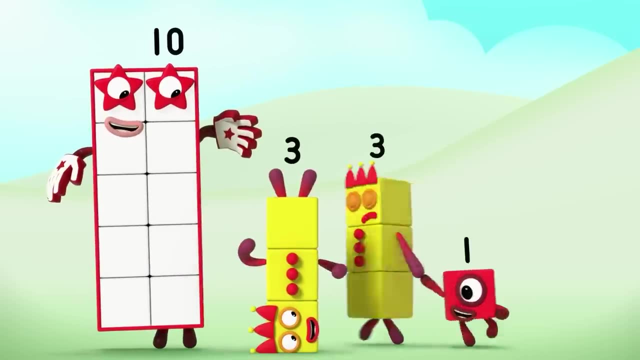 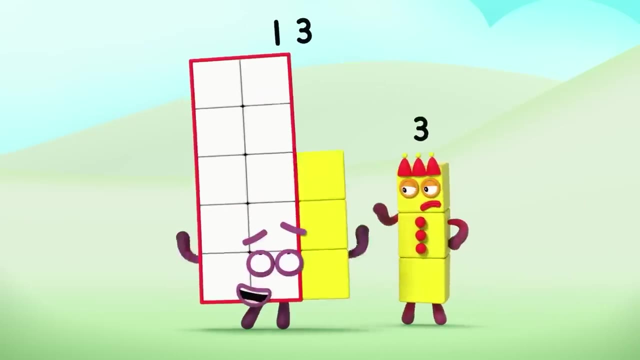 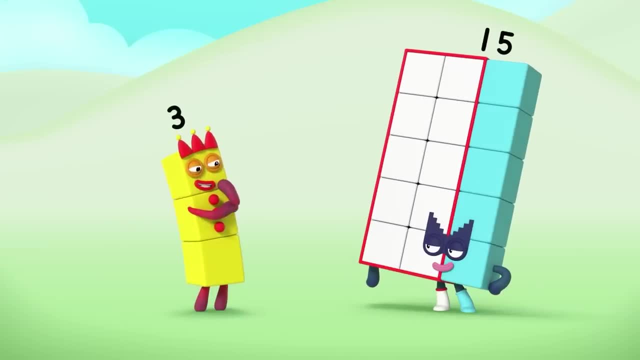 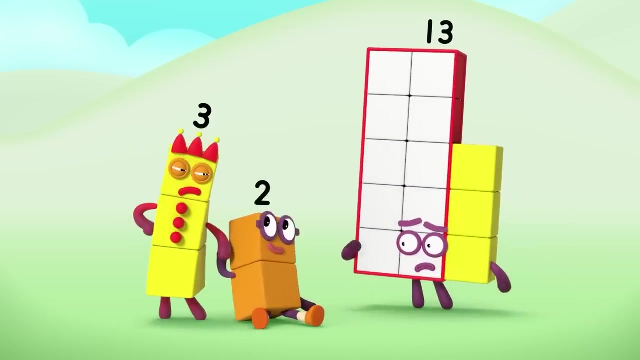 So my next trick: Twelve Plus one equals, Oh no, Ten and Three. Oh no, Your turn Fifteen. Let's say Ten and five, But I want Ten and Three, And Three is Two less than Five. 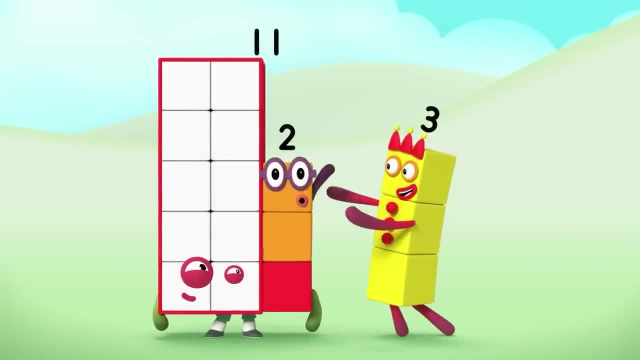 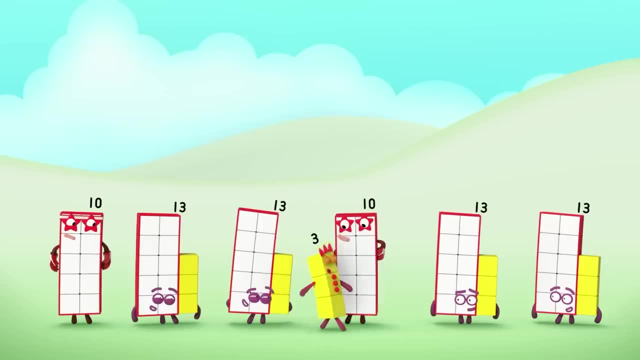 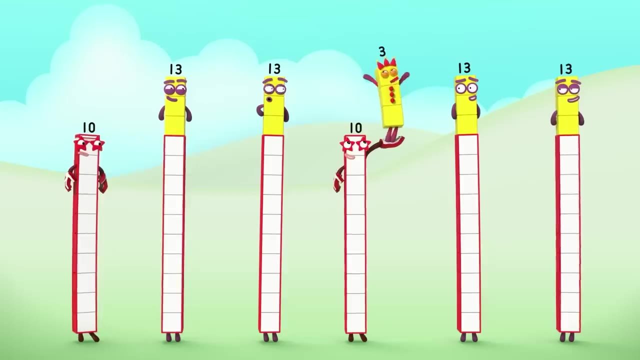 Ten and one plus two equals- Sir, Only joking- Ten and three. There. Now everybody stand tall, Ooh, When I say go, go, Go, my lovely 13!. Woo, Bolly-hoo, Bolly-ah. 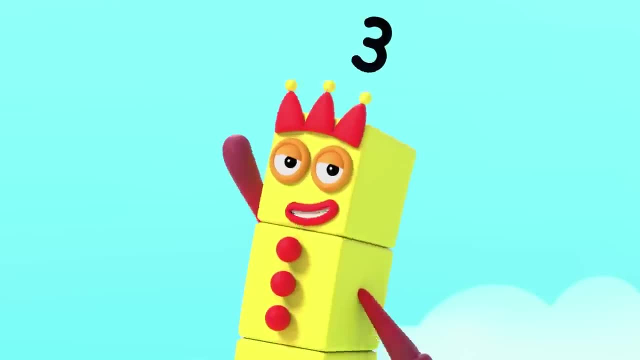 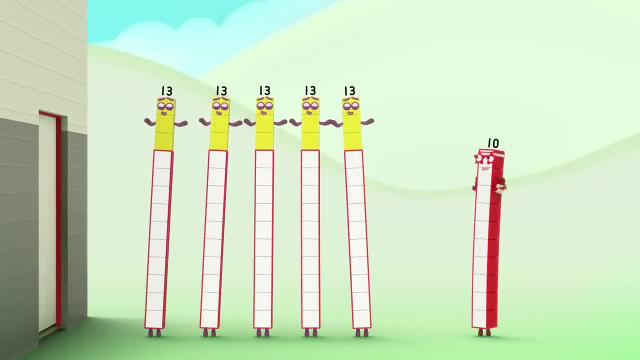 Welcome to Three's Place. Bolly-ah, Bolly-hoo, Bolly-ah. Never mind Tenth Place or Three's Place, we should call this 13!. I can't wait to visit the Pattern Palace, Is it fun? 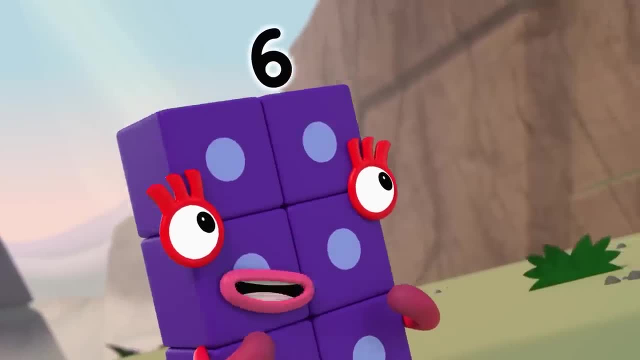 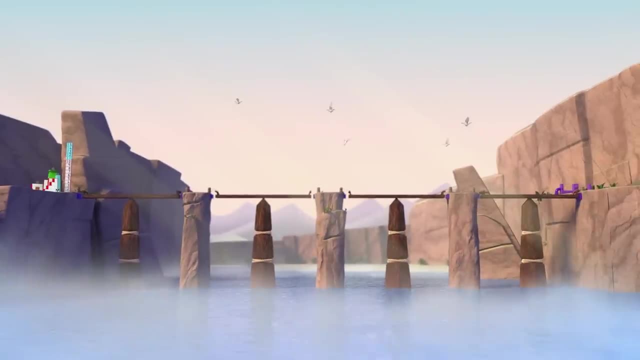 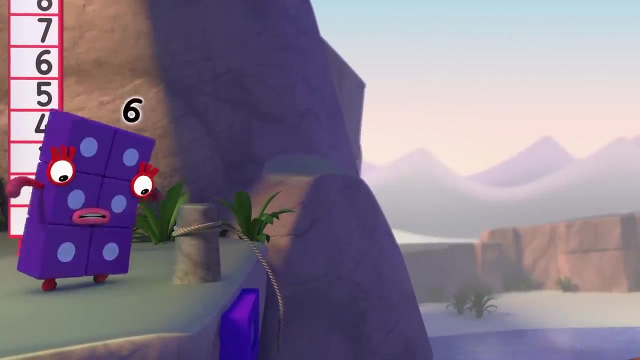 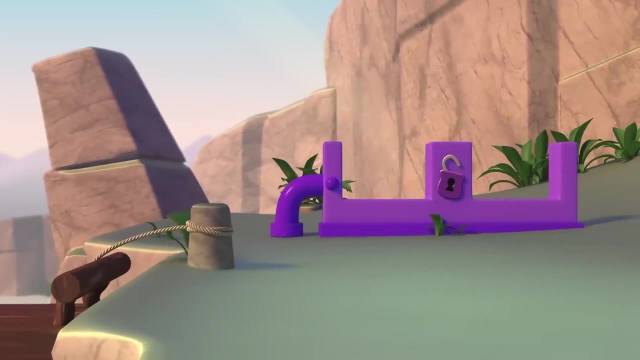 There's a shortcut round this ridge. if you can cross the balancing bridge, Hmm, Oh, Wow, Ta-da Ooh, Oh, Oh, Oh, Whoops, Guess I forgot to put the safety locks on. I say we go softly, softly. 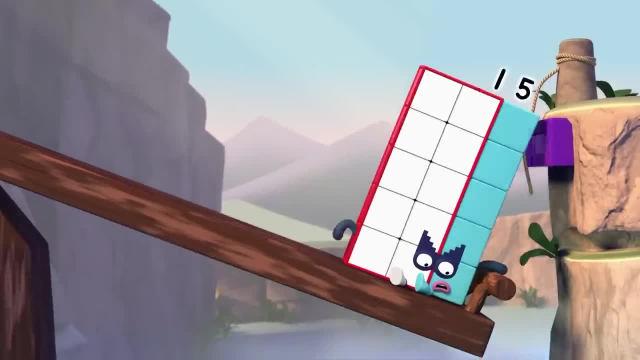 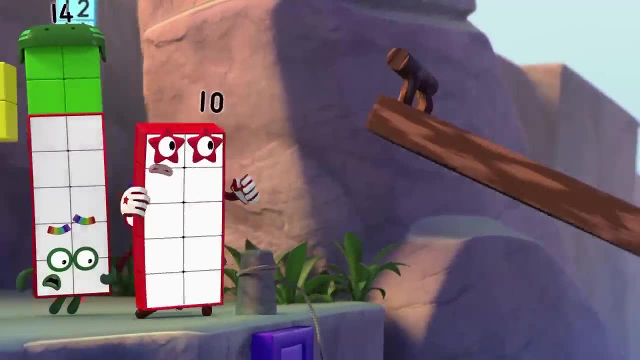 Like this: Yipe, Ooh, Ooh, Ooh, Bolly-ah, Bolly-ah. We need to balance the bridge out before 15 falls off, But I'm not big enough to do it alone. Ten is less than 15!. 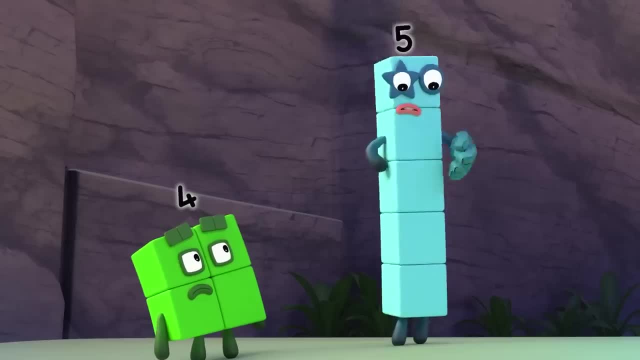 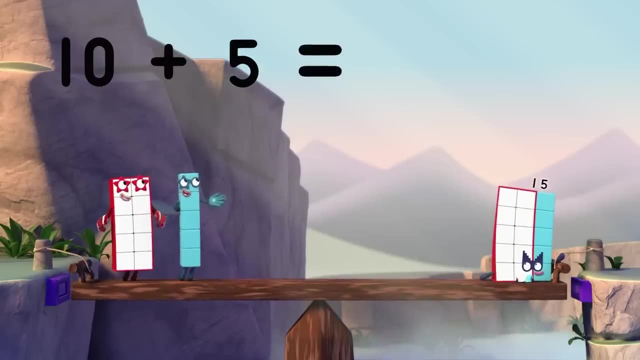 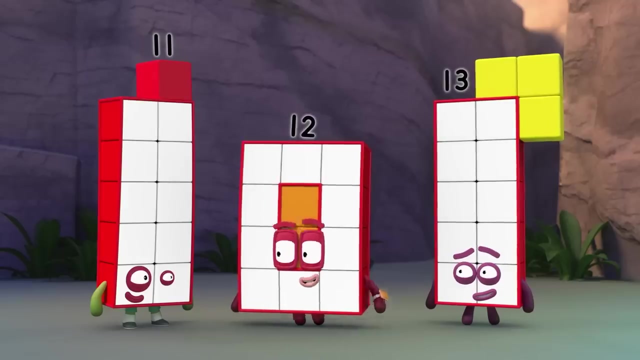 You need 15 blocks to balance me out. But 15 is ten and five, So if I land a hand, Hoo. two plus five equals Equals .15!. Grab, hold. We need to reach the far side so we can lock the bridge. 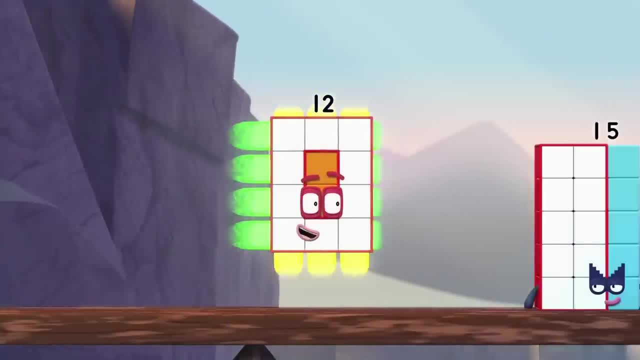 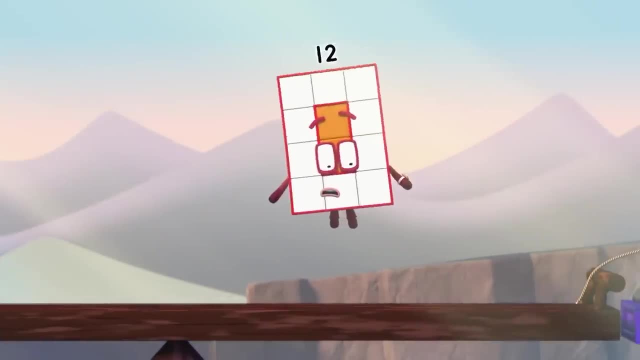 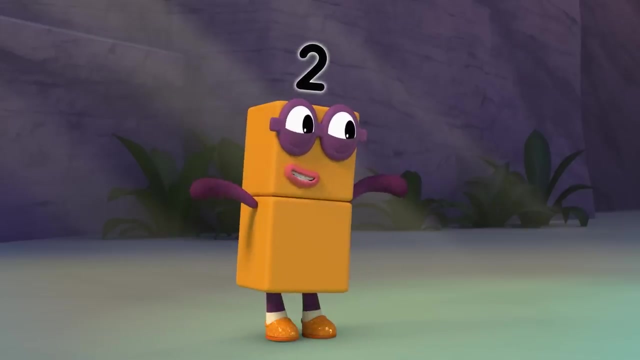 I can do this. I am three by four, I am a rectangle. Wow, That is so cool. Thanks Six. Ooh, Ooh, Ah, Ah. What's going on? Ooh, 12 needs balancing And 12 is ten plus two. 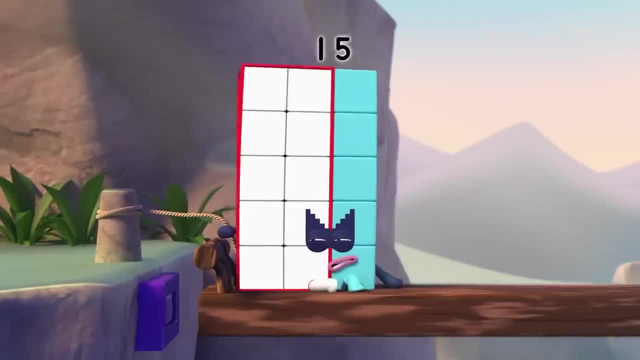 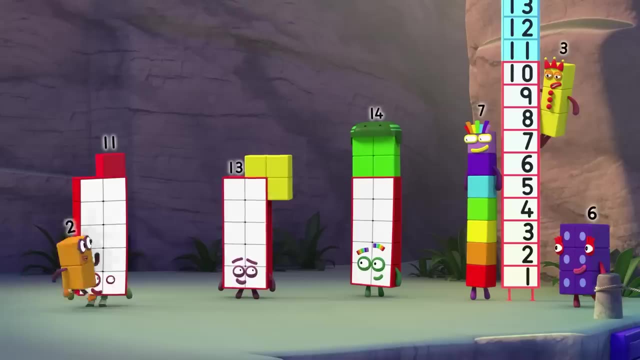 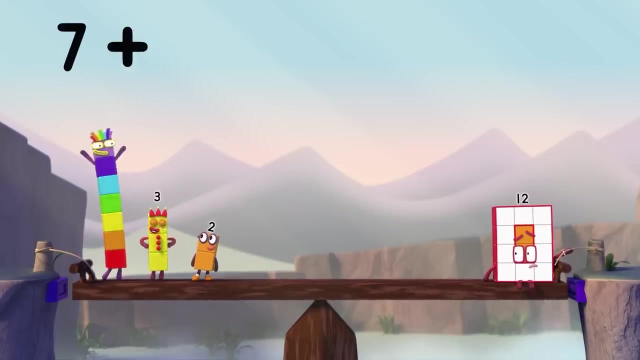 Come on ten. Wait, Where's ten? Ooh Bit busy, Sorry, Then we need another ten. Ah, Seven, three, You can make ten. Hoo-hoo, That's lucky. Seven plus three Plus two. 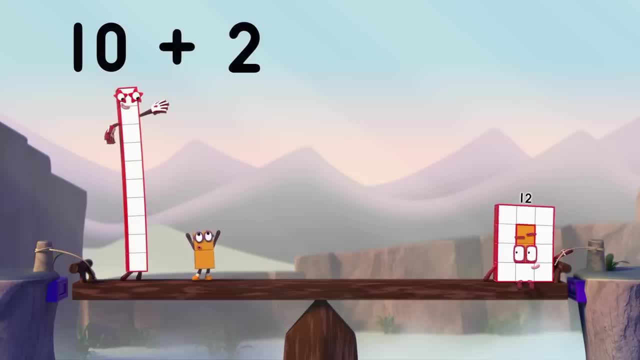 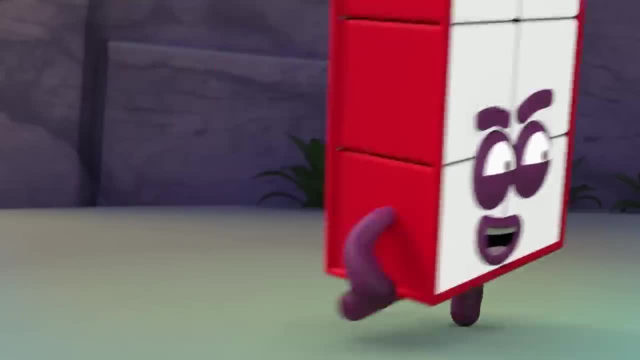 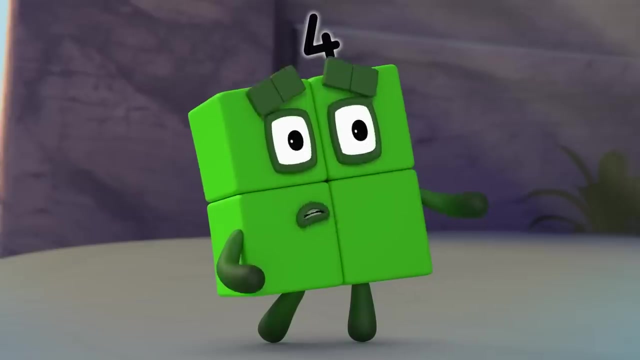 equals ten Plus two equals twelve. Grab, hold, Hooray, We're halfway there. What could possibly go wrong? Ooh, Look out Thirteen. Who said it? Ooh, We need to balance thirteen, but we haven't got a three or a ten. 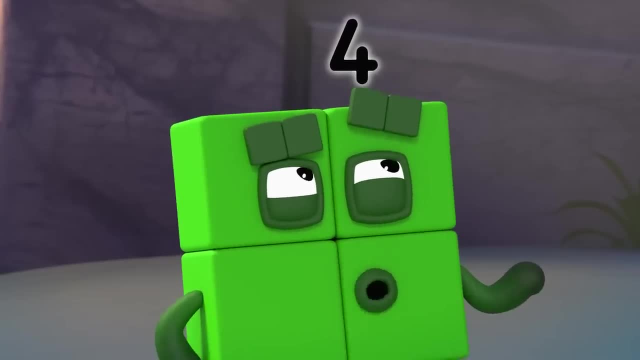 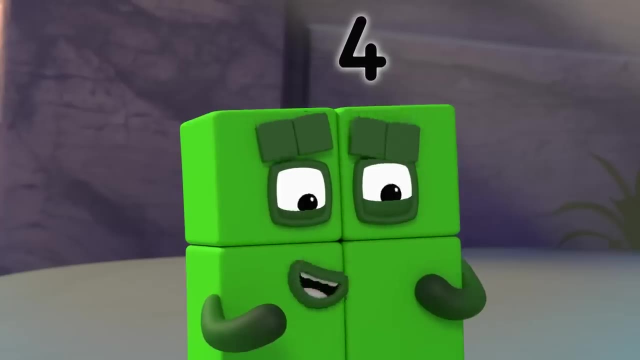 Maybe I can help. I'm only one less than ten. That's close, And after that I'm going to have to do the same thing over and over again, Ooh, Ooh, And after that we need three more blocks. 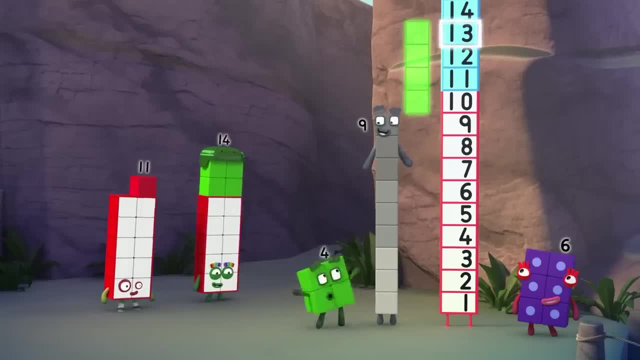 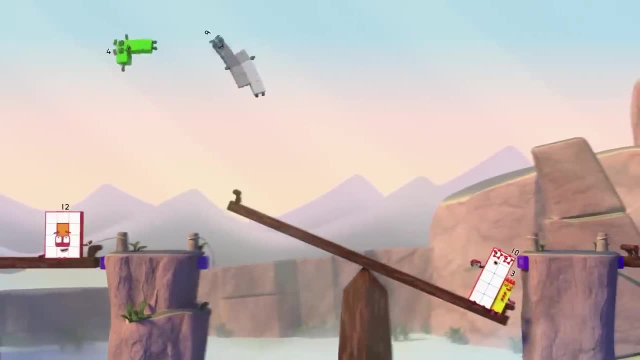 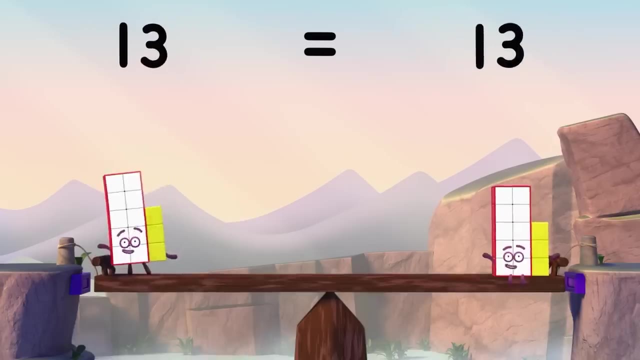 So that adds up to one, two, three, four, Four blocks. Oh, Square power, Ooh. Nine plus four equals ten plus three, And both sides equal thirteen. Whee Grab, hold One more bridge to go. 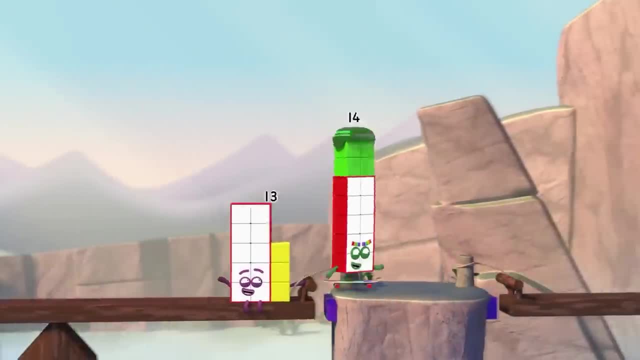 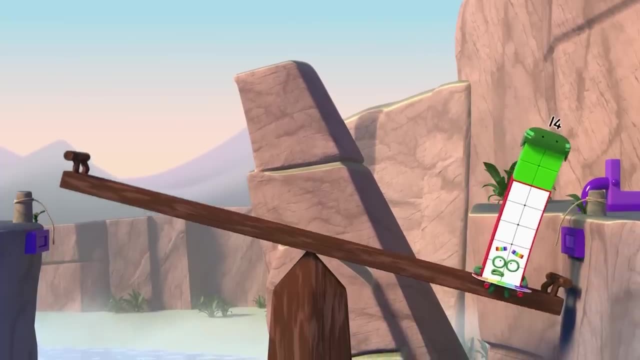 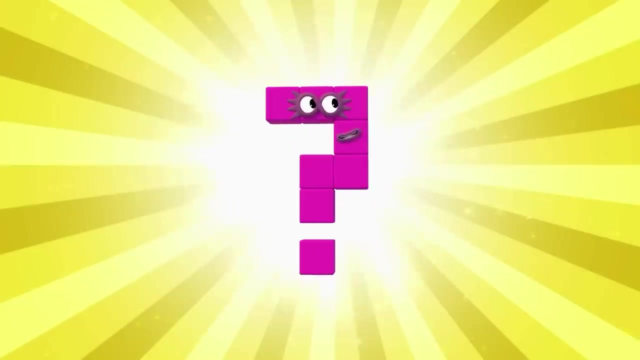 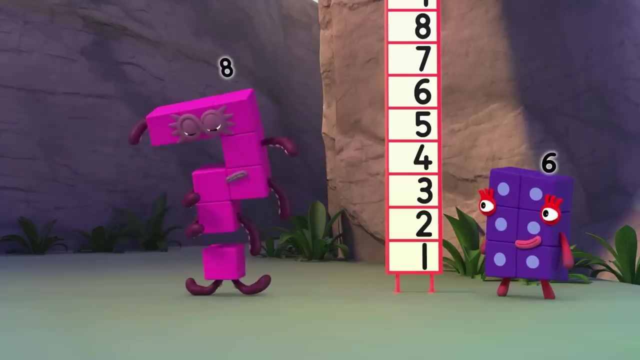 Three, three, three, Hooray, Ooh whoa, We need to balance out 14.. Somehow Octoblock, think One, two, three, four, five, six, seven, eight, Think Mm. 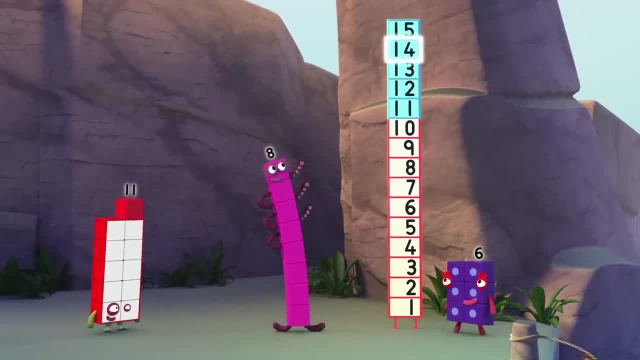 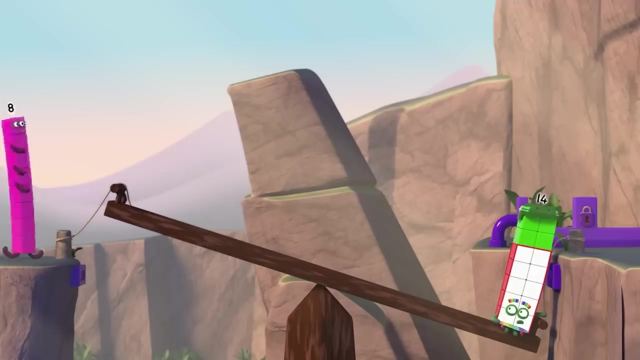 How do I get from 8 to 14?? Uh-oh Ha. So I need four blocks more, which makes One, two, three, four, five, six, Whoop, Whoop, Eight plus six. 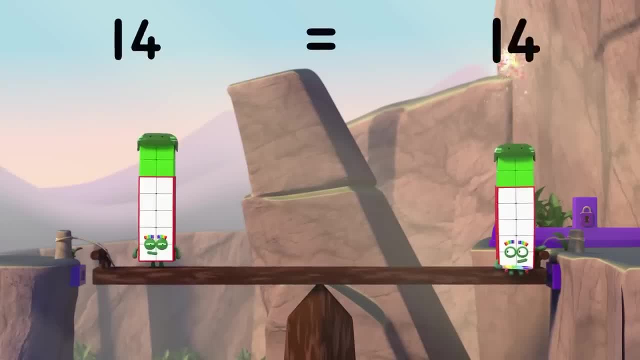 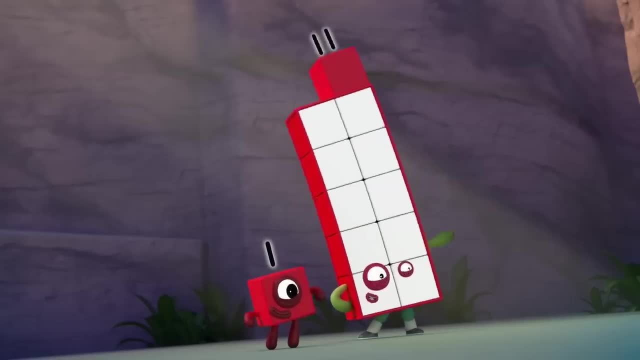 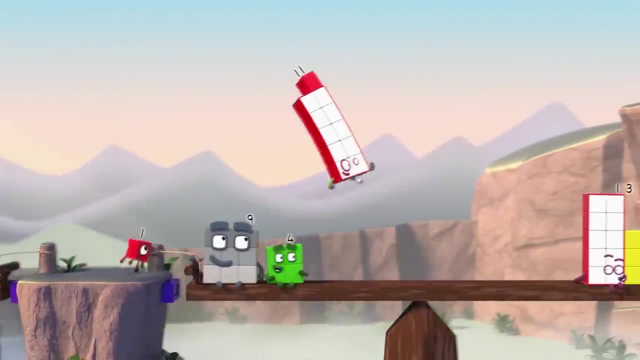 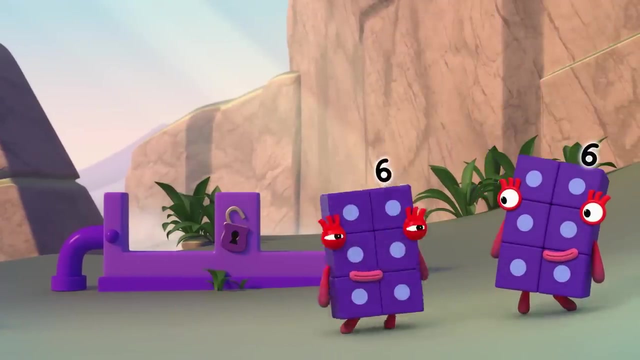 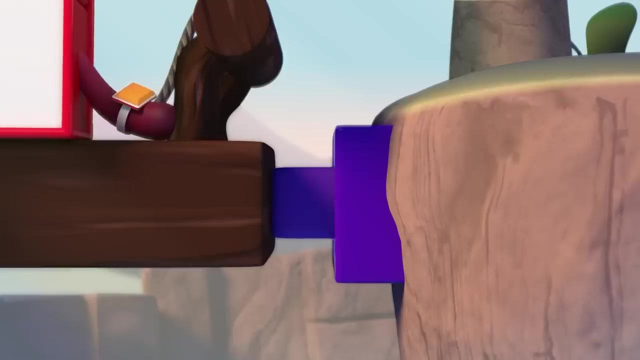 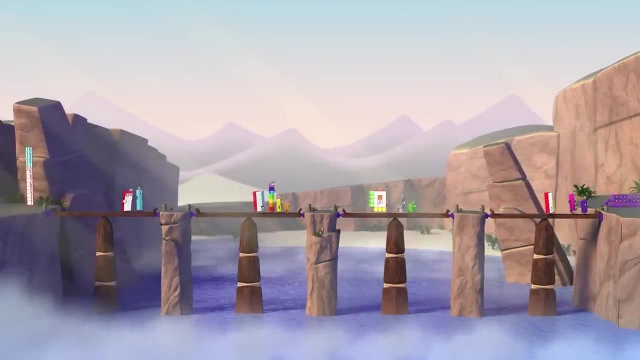 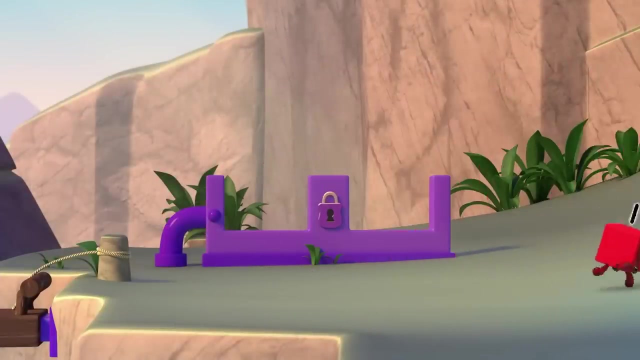 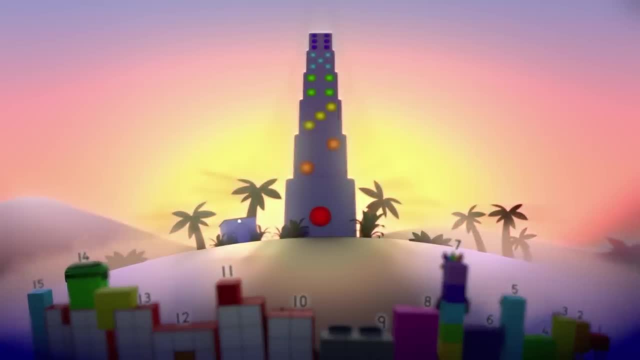 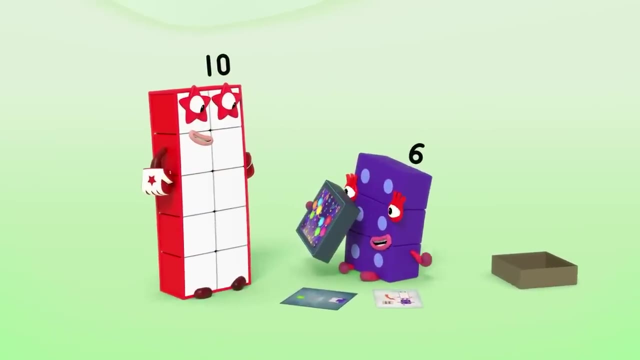 Hooray, I guess this shortcut's not so swift. Next time we can take the lift. There's a lift Six To play my new game. It's called Party in a Box. Ooh, First roll the dice. 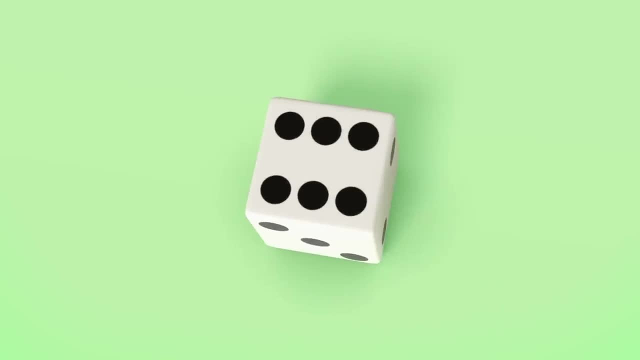 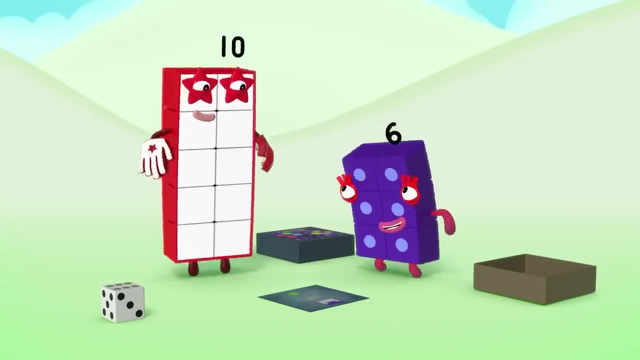 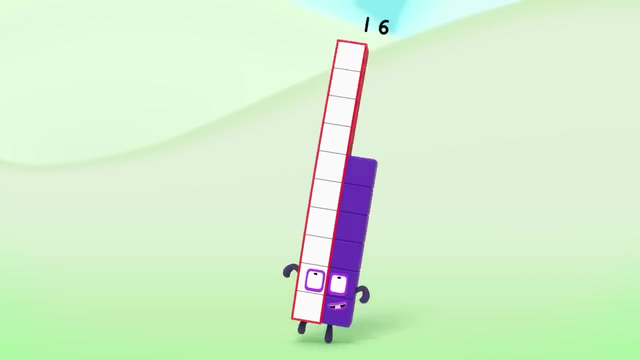 Let's roll Six. If you roll a six, jump on your friend's shoulders. Hmm, Ten plus six Equals Sixteen. Oh, look, Here I am then. Well, that's nice, isn't it? Right then? 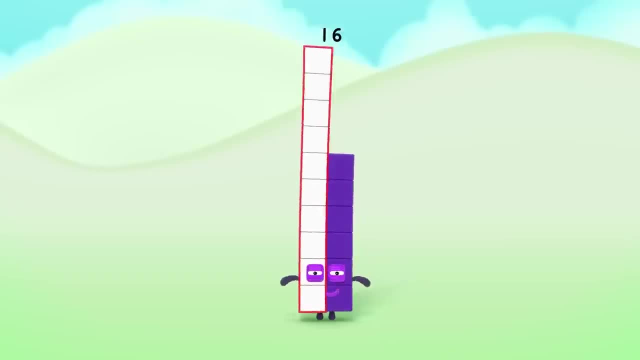 Let's get on with it. see what shapes I can make. Yeah, Hmm, Ooh, Um, Aha, Ooh, Ooh. No, No way, I can't believe it. I'm so excited. Guess what? 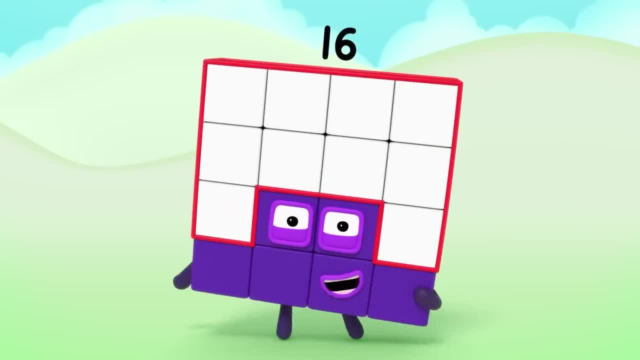 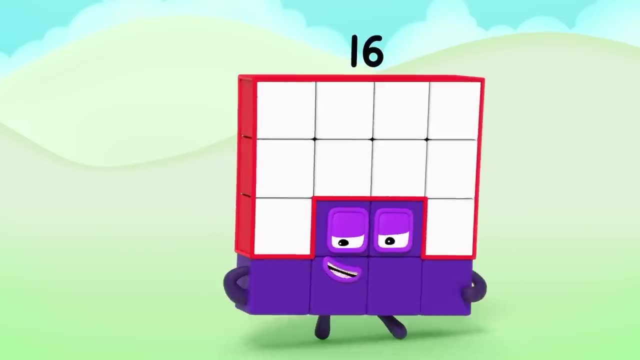 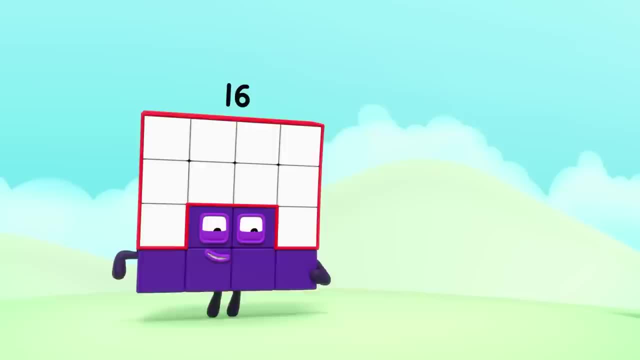 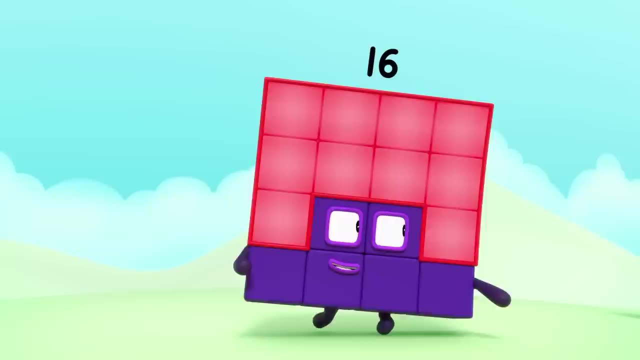 I know Square party One, two, three, four, five, six, seven, eight, nine, 10,, 11,, 12,, 13,, 14,, 15,, 16! I am 16.. Square as a box. 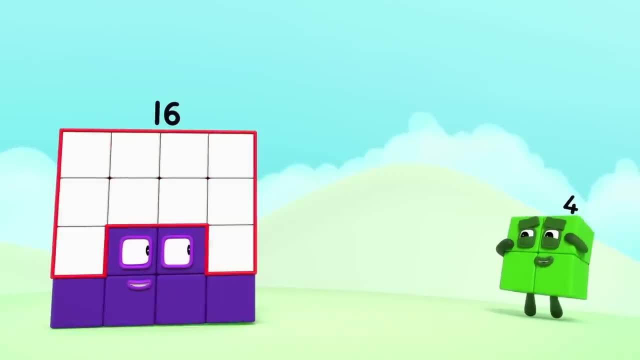 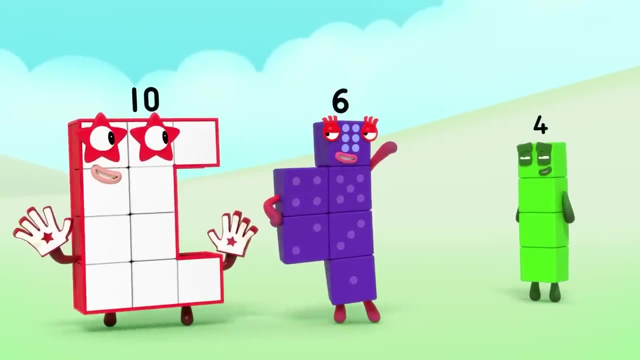 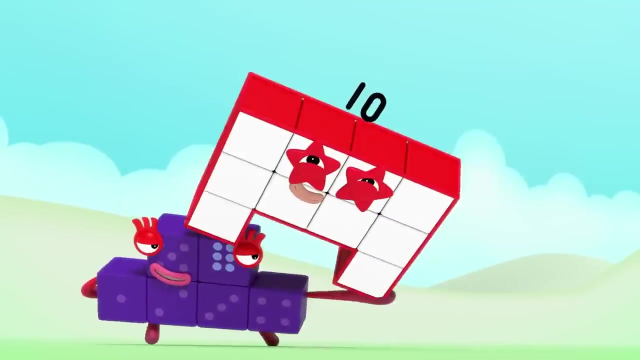 And guess what? I've got 16 blocks Square, Really big square- 16. 10 and 6.. I like this game. 16. 10 and 6. Party 16. I am 16.. I'm. 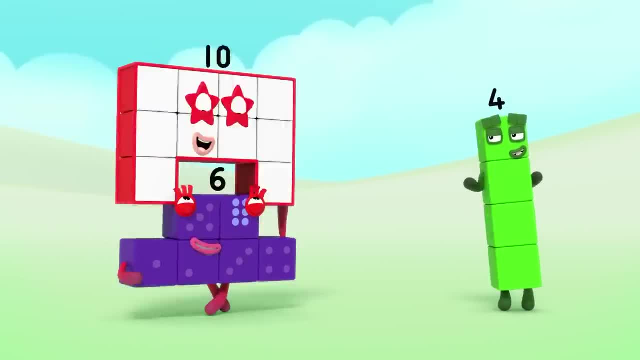 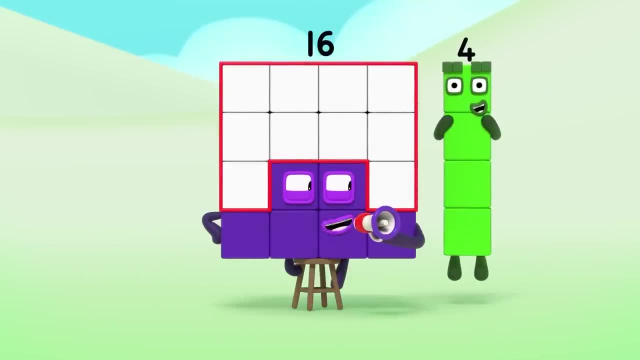 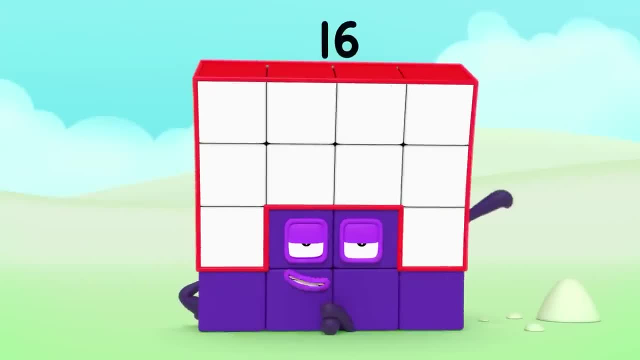 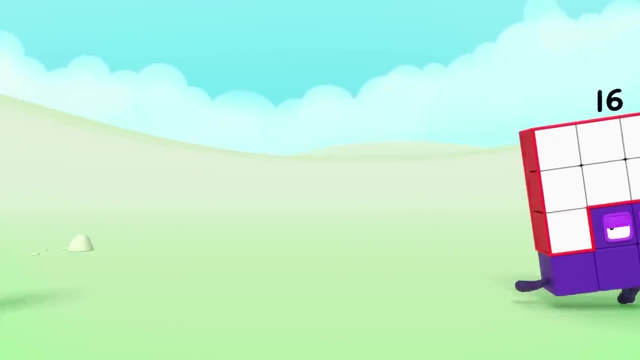 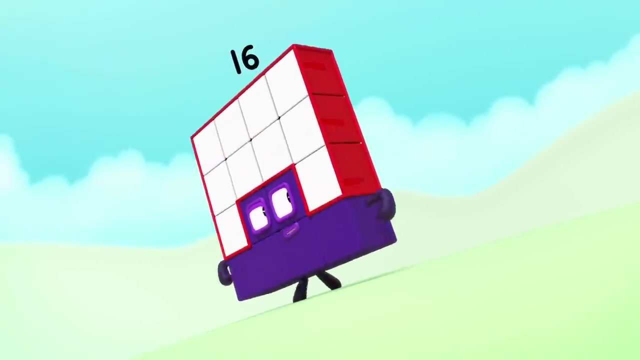 by four, four by four, four by four. I am a square, Are you sure? Of course I am. I'm four by four, 16. I have four columns and four rows. Four lots of four. I'm four of those. 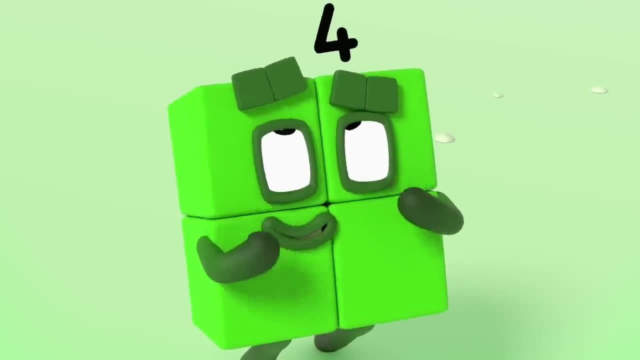 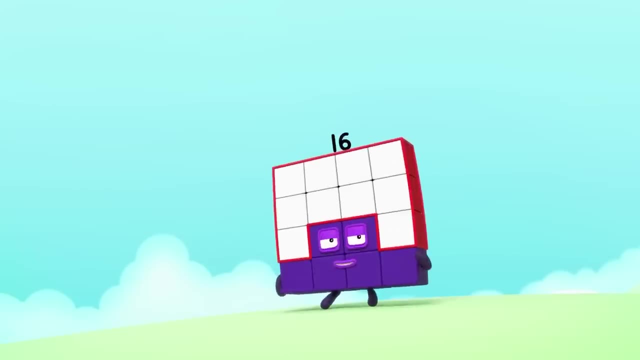 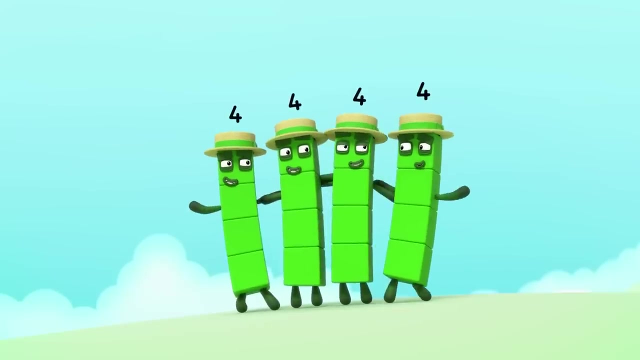 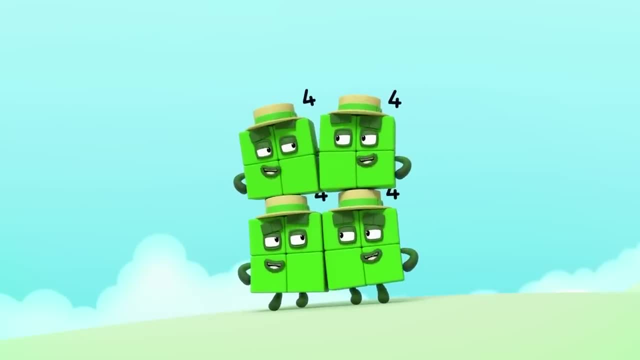 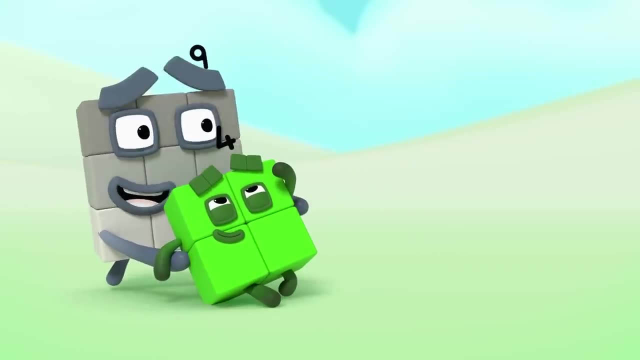 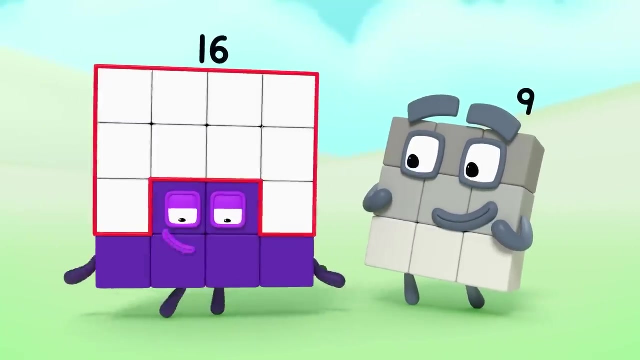 One, two, three, four, four, fours. You know what four fours are? 16.. Oh, um, it's all right. four, It's only a really big square. Wow, I am 16.. I'm four by four. I'm larger than a dinosaur. 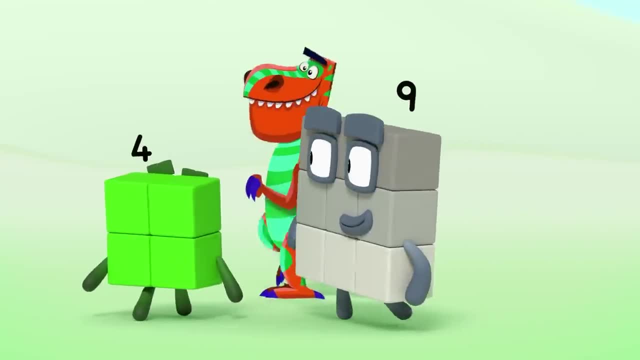 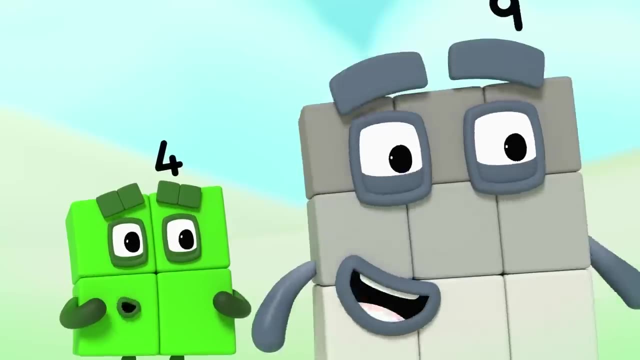 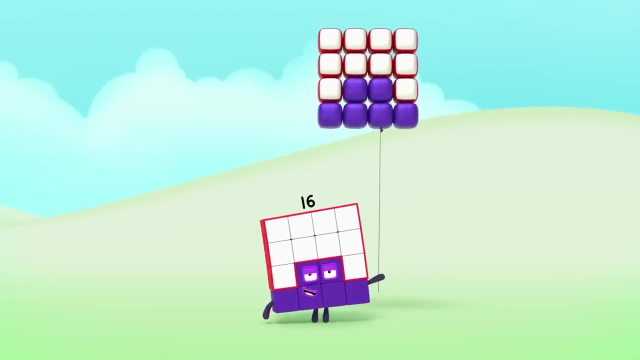 Whoa, Whoa Later, Rexy, I am 16.. I mean no trouble, But have you seen me? I'm a devil No Alone, 16.. I'm going to split in half now. Two eights. We're going to split in half now. 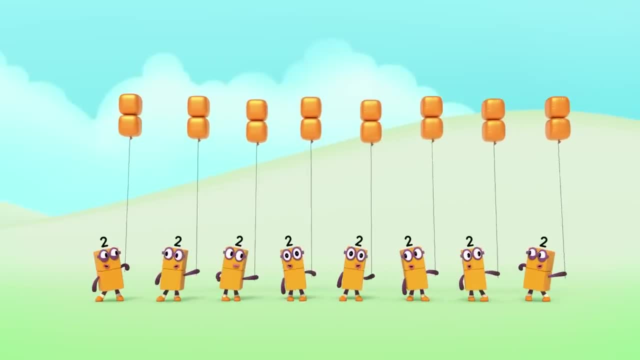 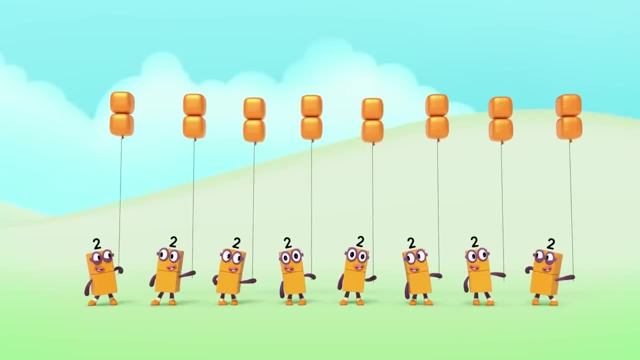 Four, fours. We're going to split in half now Eight twos. We're going to split in half now 16 ones. Hooray, We're going to double up now. Eight twos, We're going to double up now. 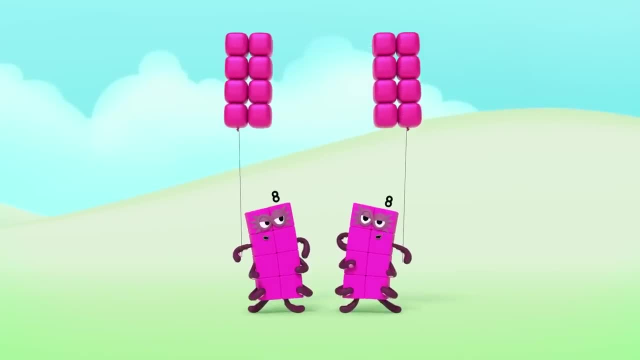 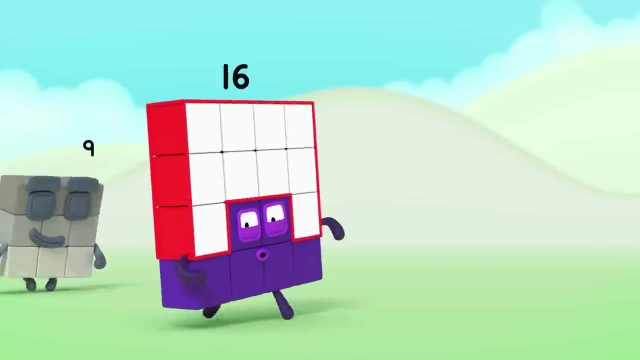 Four, fours, We're going to double up now Two. eights, We're going to double up now 16.. I'm going to- Oh it's me silly- Do-do-de-do, do-de-do, do-de-do, do-do-de-do, do-de-do, do-de-do, do-de-do. 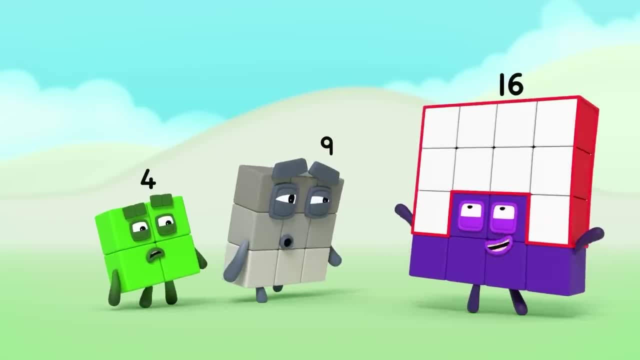 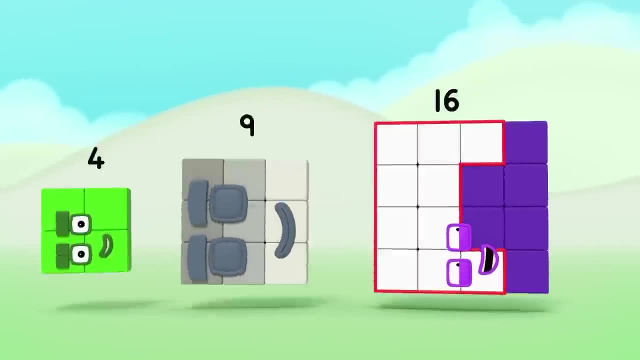 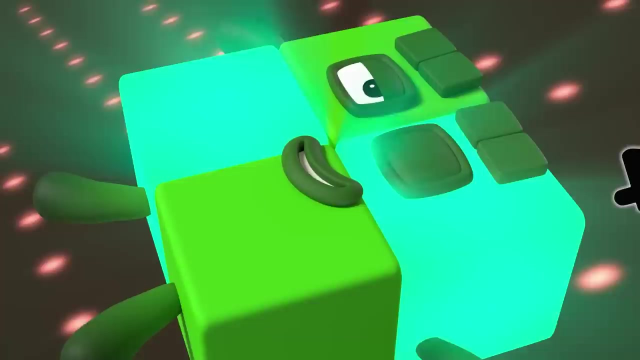 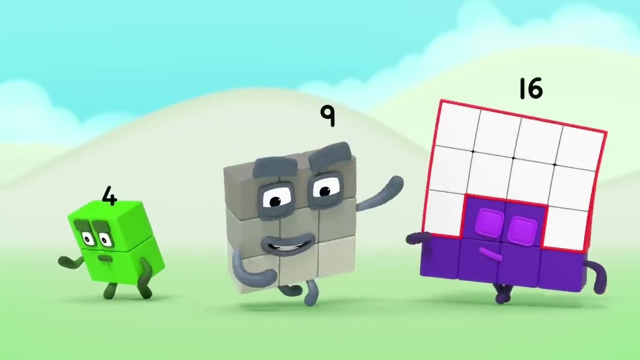 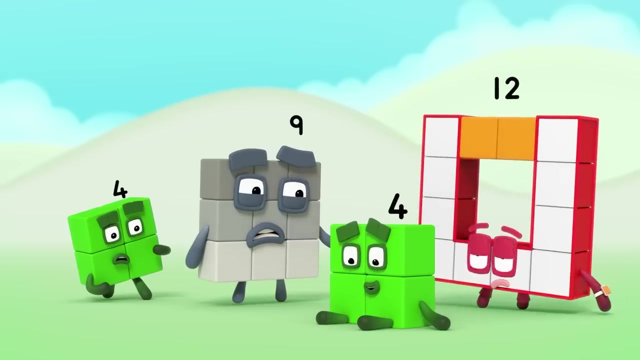 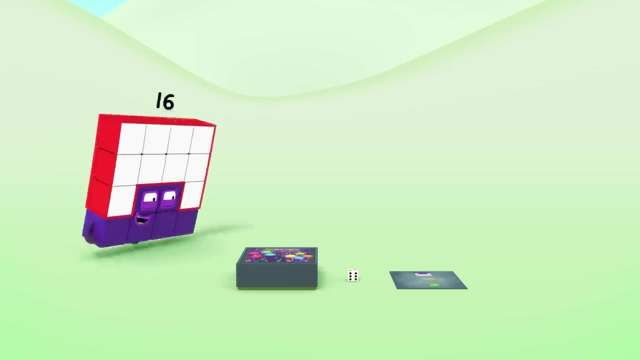 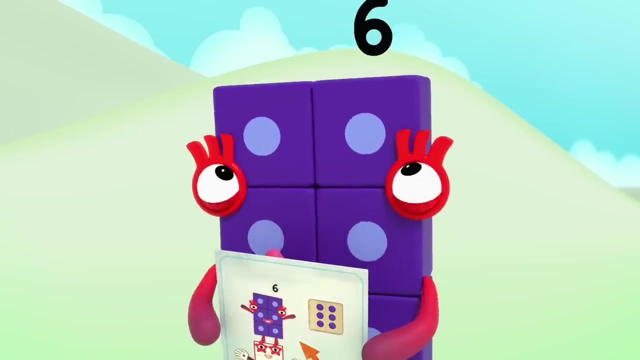 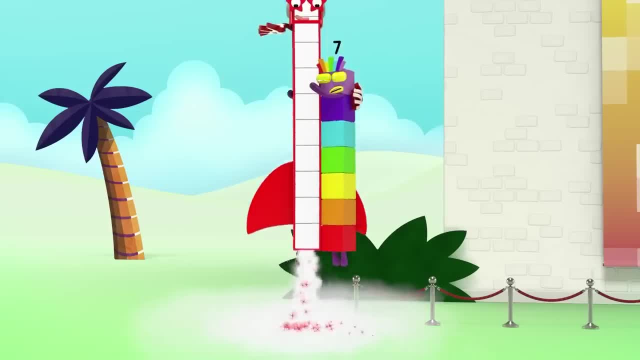 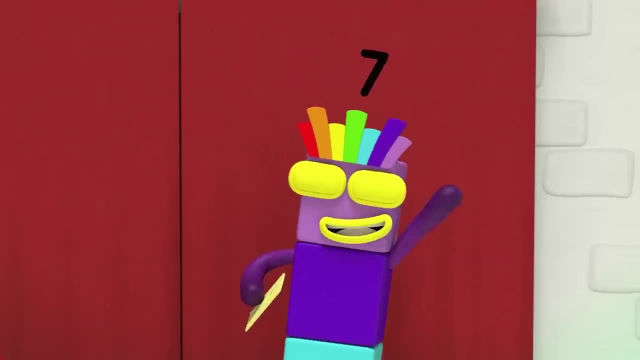 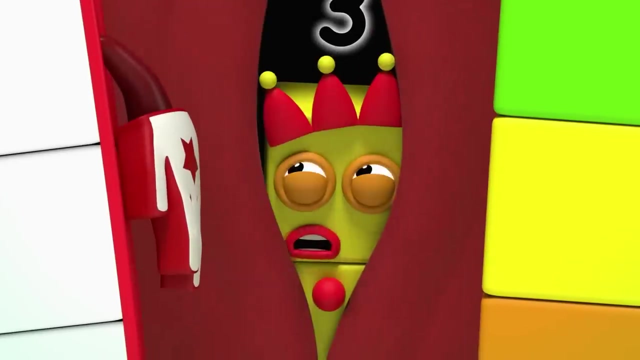 Thanks for the lift Ten. Are we in time? Yes, That's lucky. I wouldn't miss the opening of Numberland's first art gallery for the world. You and you, Ah, Oh, look at that. Oh, I like it. 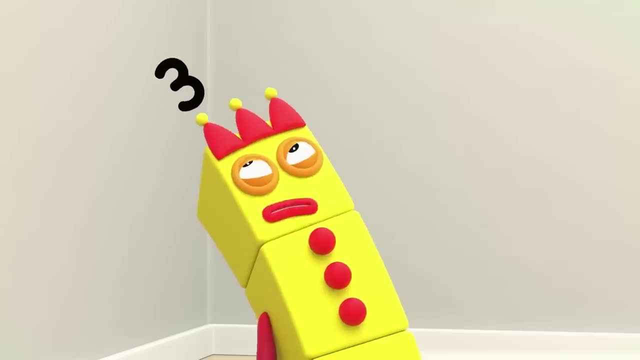 But where's the art? Oh, I spent so long making sparkly invitations, I forgot to get any. Ooh, Can we help? I thought you'd never ask: Are you sure you're a rocket? You're full of colors. 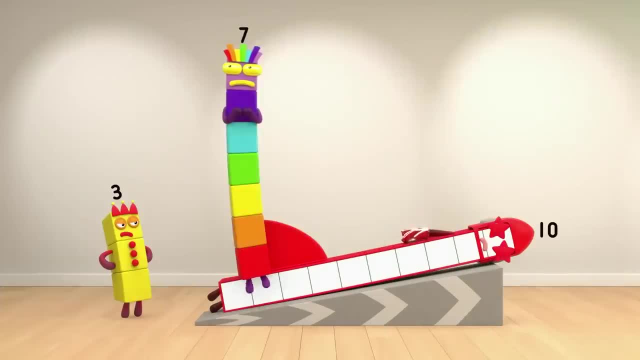 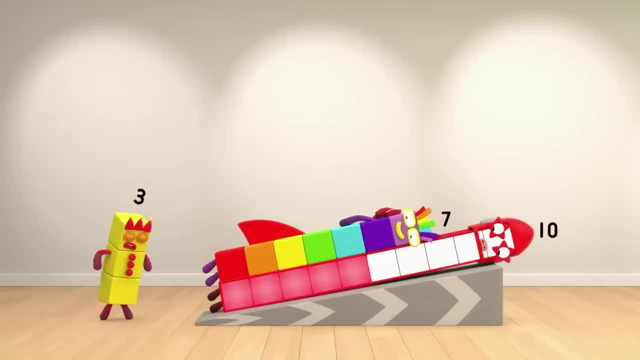 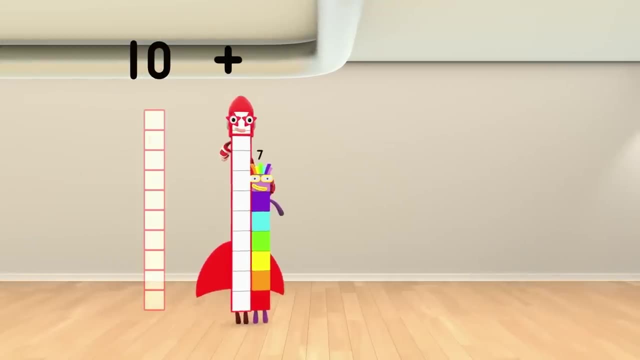 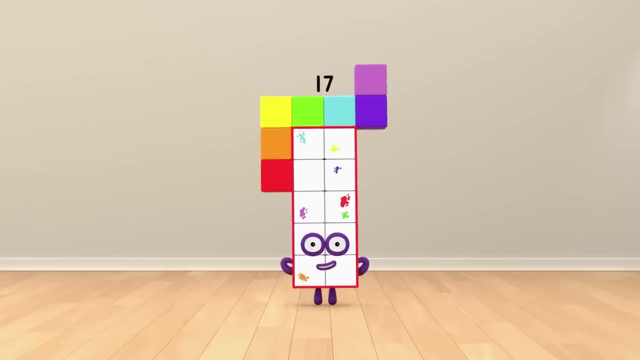 I'm a rocket. 10, plus 7, equals 17!. Ooh, now there's a surprise: I am 17 and I love to paint. They're coming in, Oh no, Go, go, go. 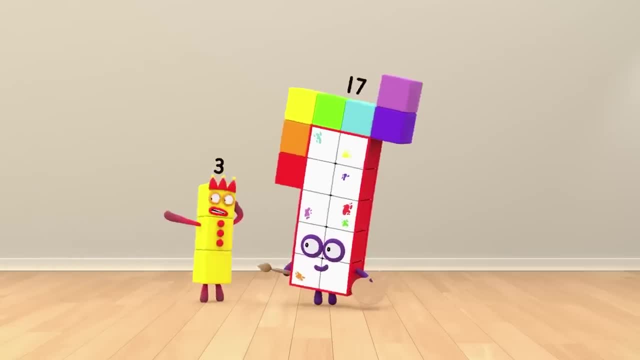 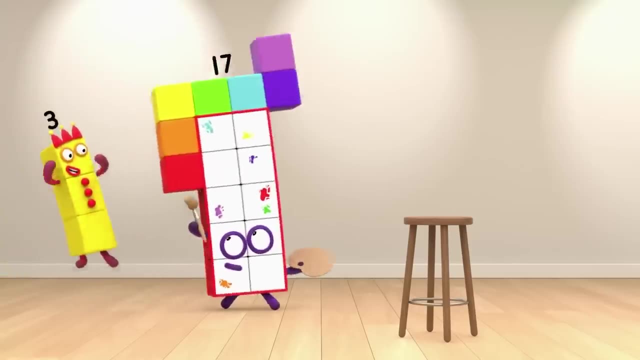 Don't mind if I do Check it out. I'm going to paint. I'm going to paint. I'm going to paint. Don't mind if I do. Some painters only paint portraits- majestic and serene. I can also paint portraits. 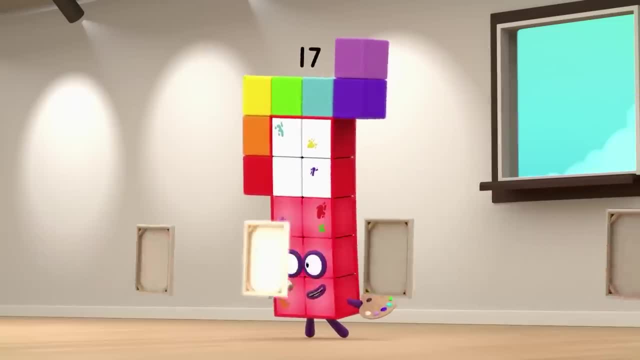 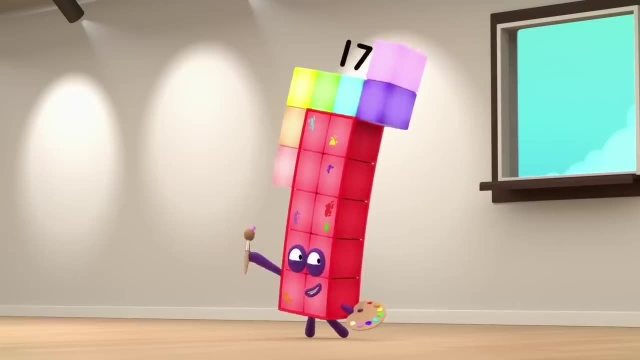 but I paint 17.. 1,, 2,, 3,, 4,, 5,, 6,, 7,, 8,, 9,, 10,, 11,, 12,, 13,, 14,, 15,, 16,, 17.. 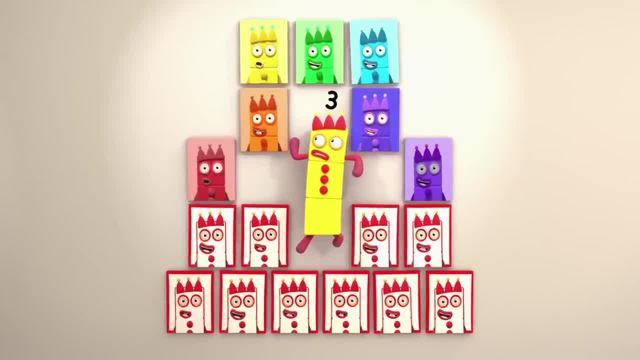 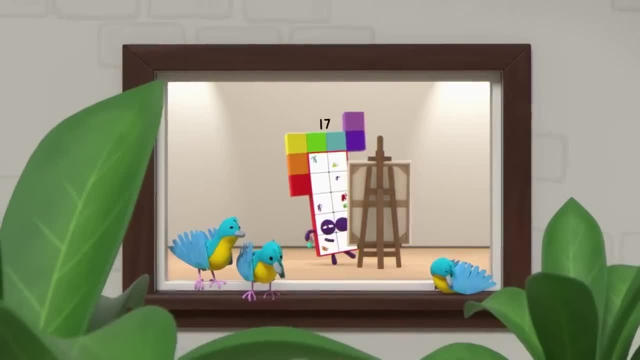 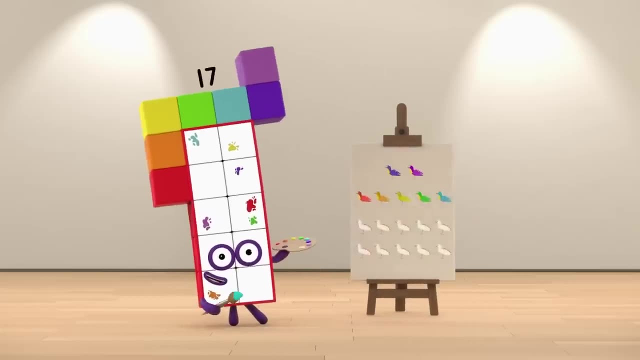 Look at me. Ooh, Look at me. Hmm, Nice juxtaposition. Some painters like to paint bluebirds in a lovely nature scene. Why paint only a few birds when I paint 17?, 10 and 7. 17!. 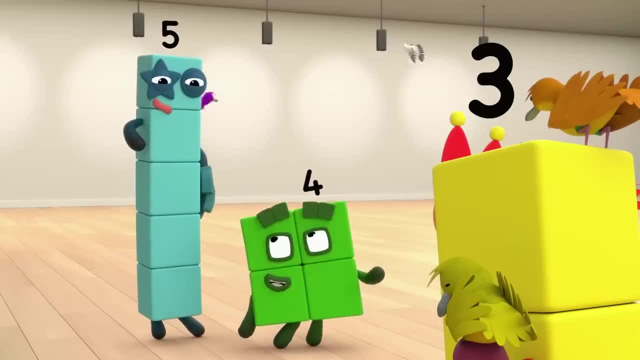 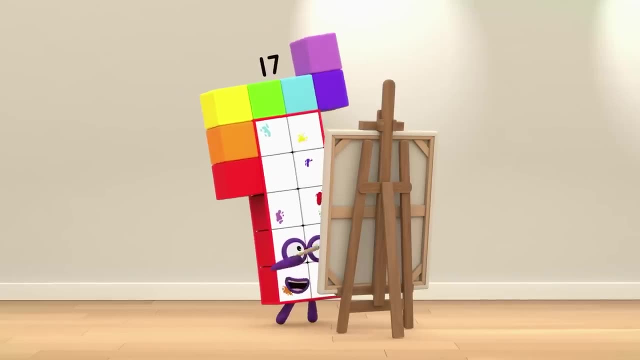 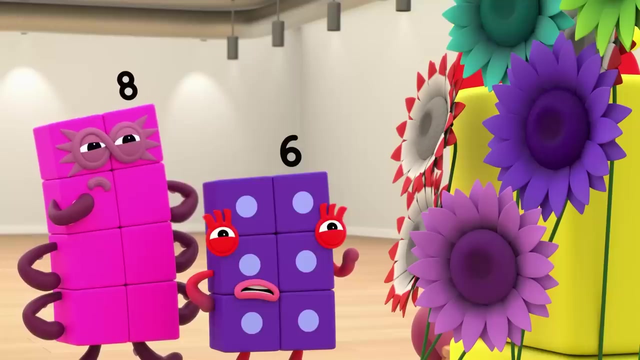 Ooh, hey, Ooh, Ooh. Nice juxtaposition. Some painters paint flowers. They look so sublime. I paint for hours. 17 of everything takes time. What, Mmm. Nice juxtaposition. Hmm, Some painters like to paint apples. 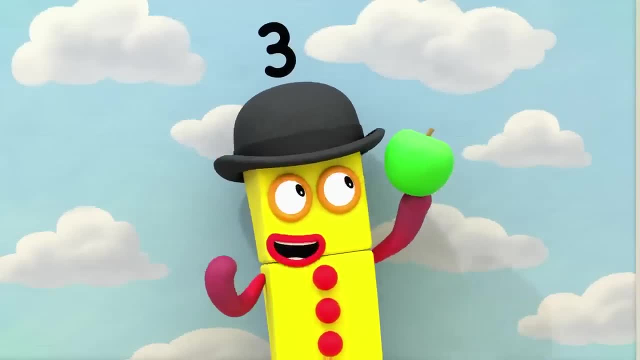 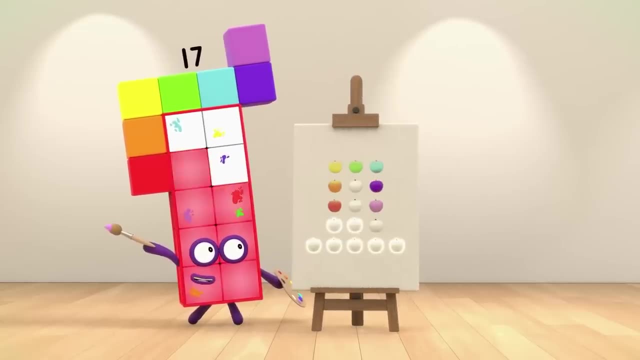 in brilliant shades of green. I can also paint apples, but I paint 17.. 1,, 2,, 3,, 4,, 5,, 6,, 7,, 8,, 9,, 10,, 11,, 12,, 13,, 14,, 15,, 16,, 17.. 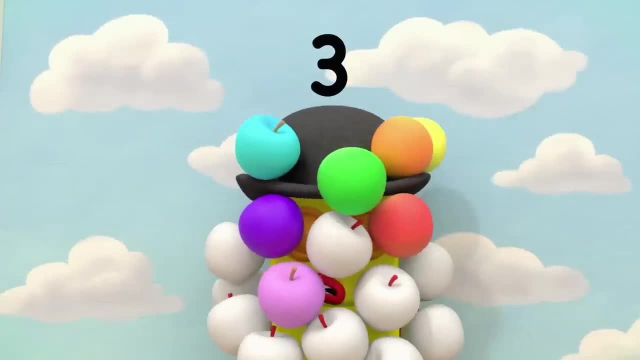 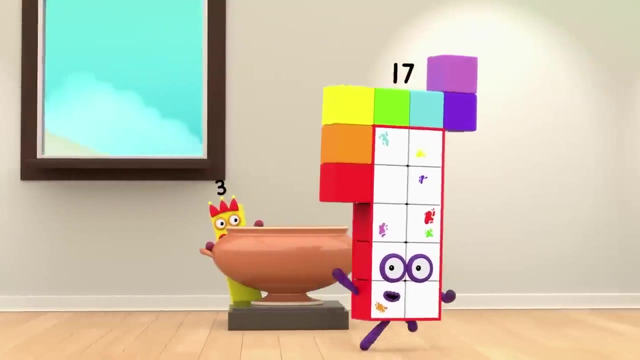 Hey No, Get off, silly apple, Not even close. Nice juxtaposition. Some painters like to paint soup cans. I like a whole tureen, So I paint plenty of soup cans. I paint 17.. 10 and 7.. 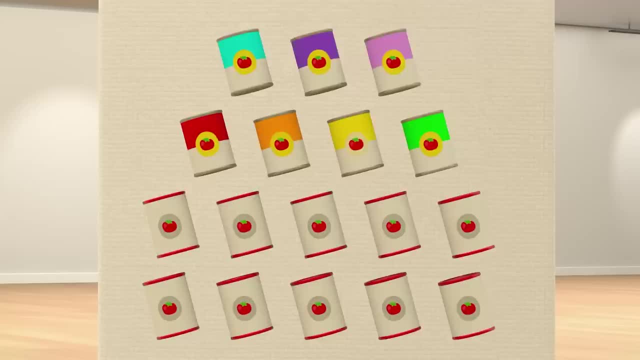 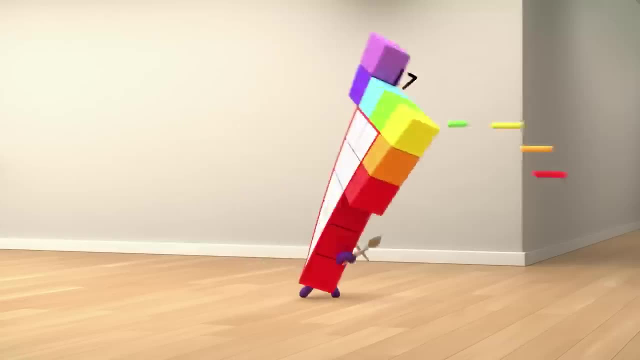 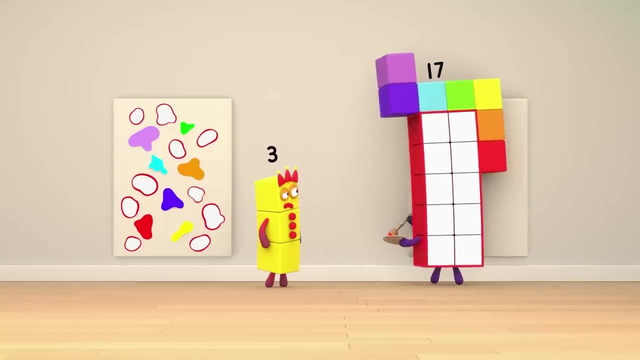 17! At least two, Hmm, Nice juxtaposition, Brrr Ooh. Some painters paint splatters, Some painters paint dots. My numbers, What matters, 17 is lots and lots of spots, Hoo-hoo-hoo. 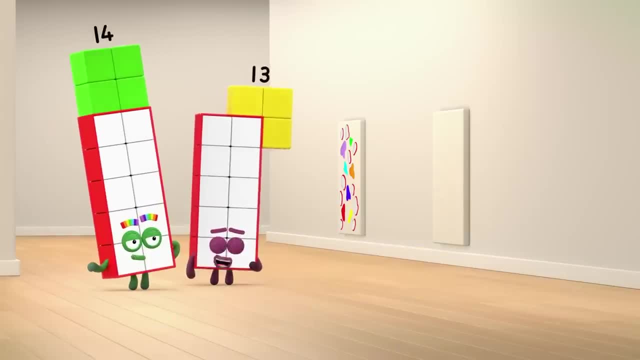 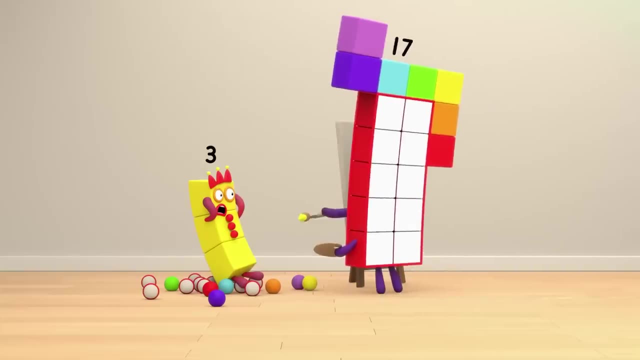 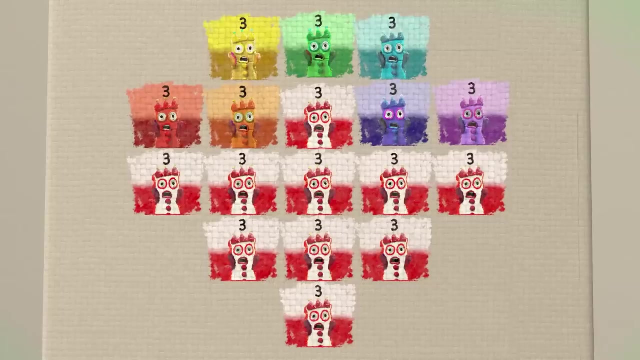 Hoo-hoo-hoo, Ooh, Nice juxtaposition. Ha-ha, Ha-ha, Ha, Hold that pose. Some painters like to paint faces that look like they might scream. I can also paint faces, but I paint 17.. 1,, 2,, 3,, 4,, 5,, 6,, 7,, 8,, 9,, 10,, 11,, 12,, 13,, 14,, 15,, 16,, 17!. 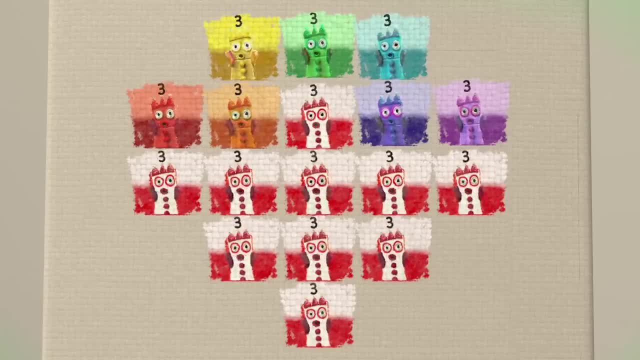 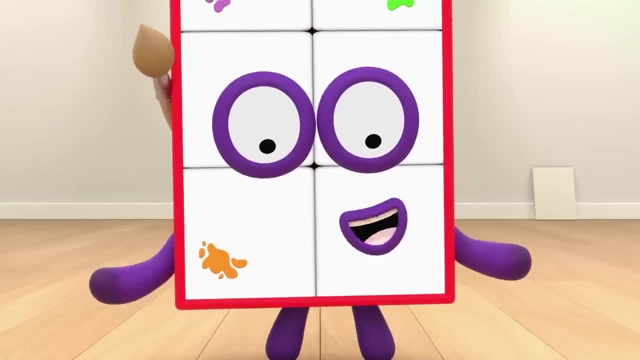 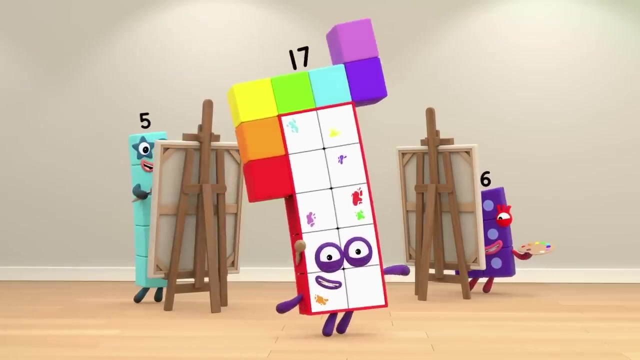 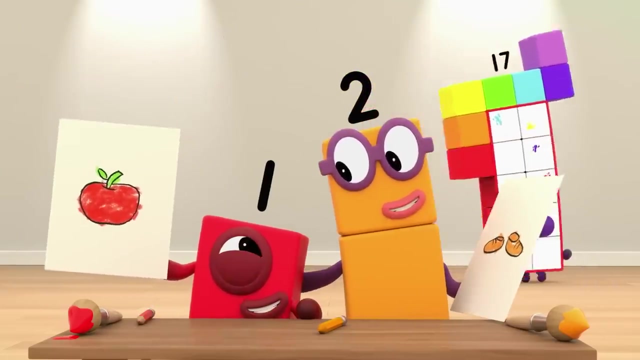 I scream, you scream, we all scream for ice cream, Ah, Yummy. Wait, I know what this gallery needs: Your art, Let your imagination play. Paint what you want, Go your own way. A piece of paper's purpose is to be your picture one day. 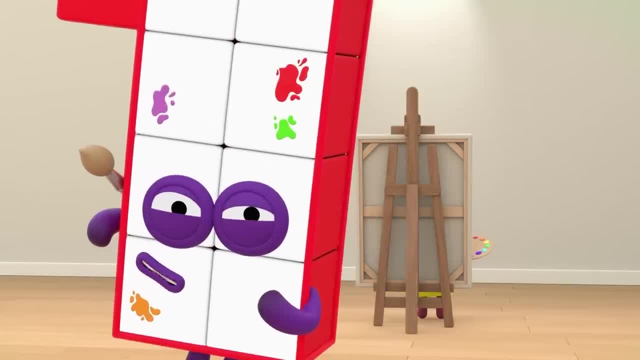 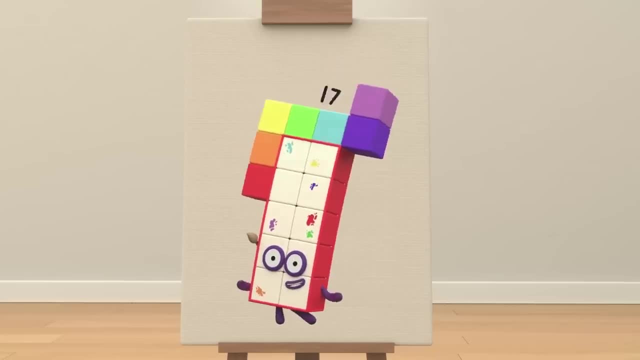 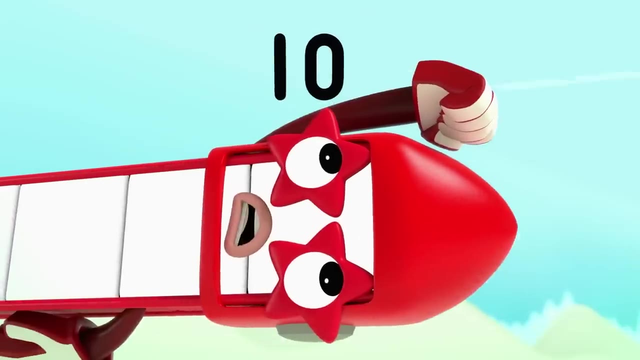 You could be an artist- the best there's ever been- But why paint only one of things when you could paint 17?? Hey-hey, Octo-speedy, Ah Too fast. Uh-oh, 10! Plus 8!. 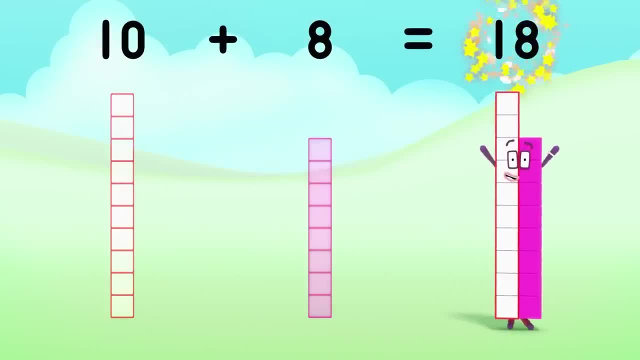 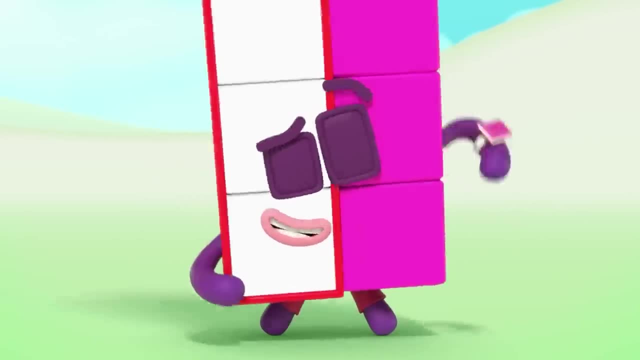 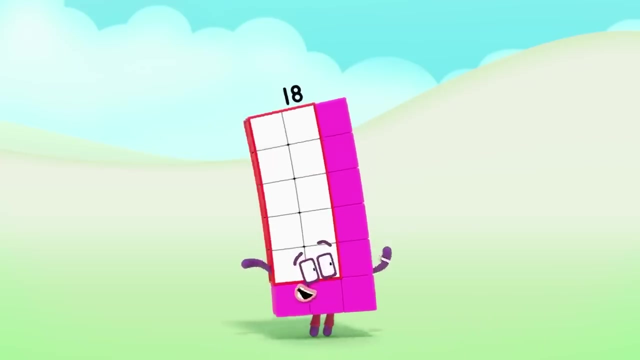 Equals: Whoa, 18!. Refreshing, Hey, time to discover who I am. Ha, Oh, Uh, Oh Done, I am 18, and I'm a super-speedy, super-rectangle And I like to go fast. 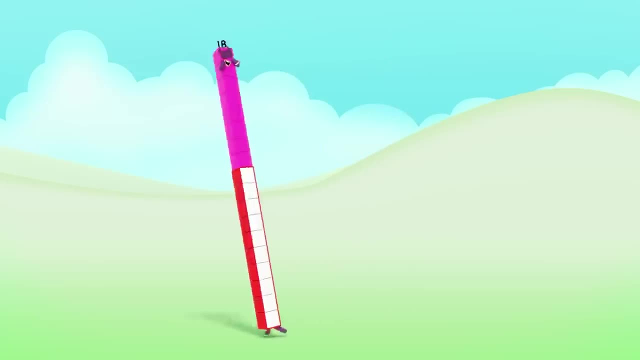 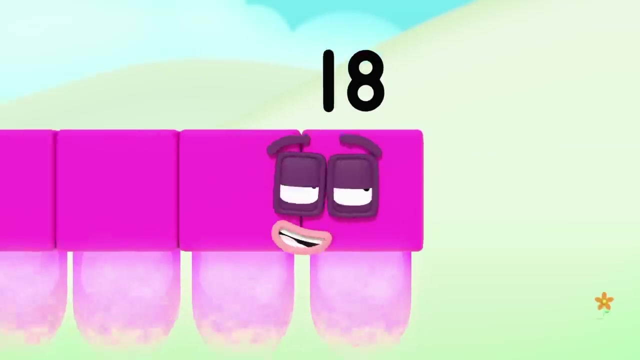 Ah, Oh, so tall, Ooh, Falling-over competition. Ah Oof, I win Ah-ha 18 by 1! One ray is all I need One ray to build up speed. I start to glow and I go, go, go. 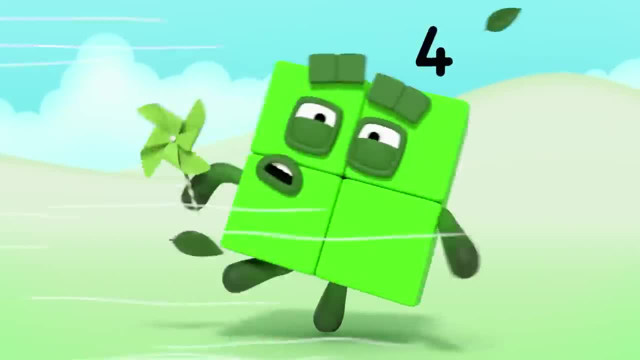 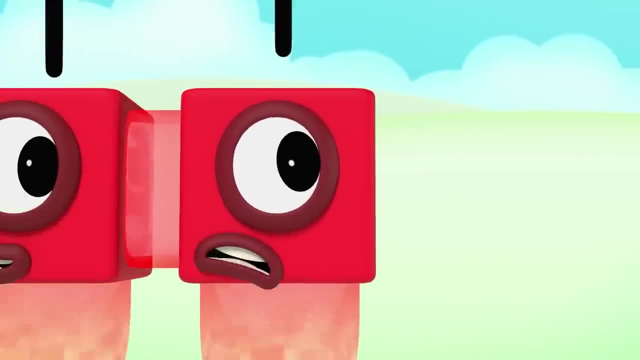 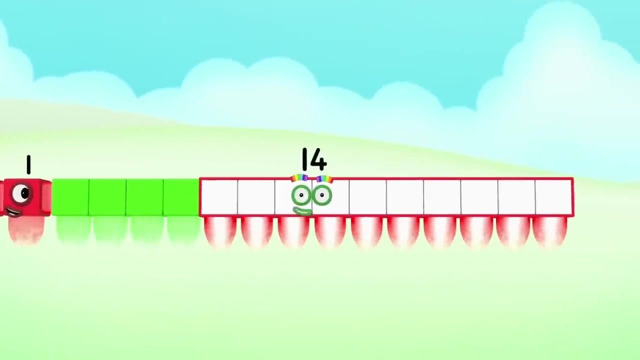 Whoa Ha-ha, Ooh, Ooh, 18 ones. This is fun Too fast. 1, 2,, 3,, 4,, 5, 6,, 7,, 8,, 9,, 10,, 11,, 12,, 13,, 14,, 15,, 16,, 17,, 18!. 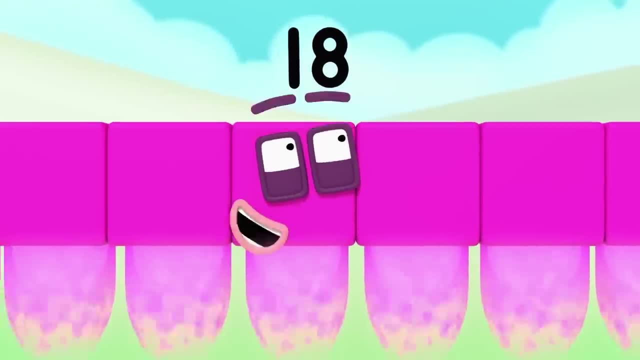 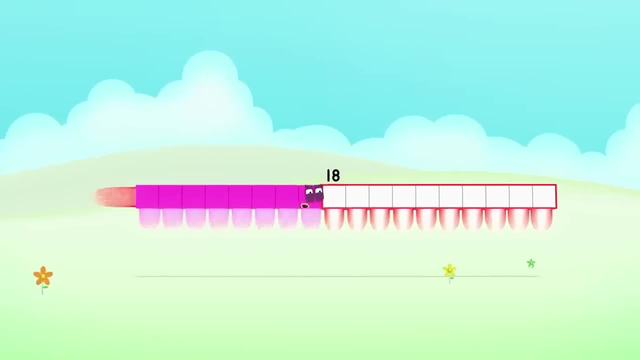 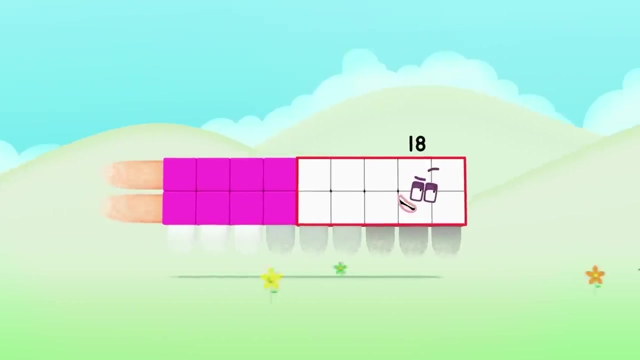 Ha. When it comes to acceleration, I'm the undisputed master. I'm the quickest in the nation. I change shape when I want to go faster. Switch 9 by 2 to race it away. I'm 18!, I'm a speed machine. 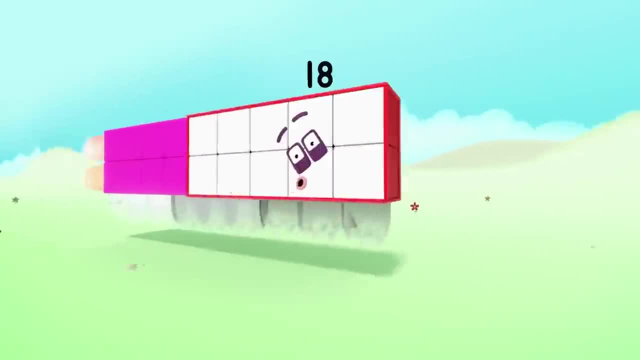 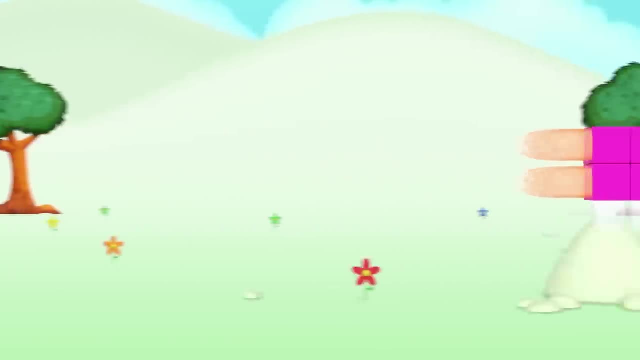 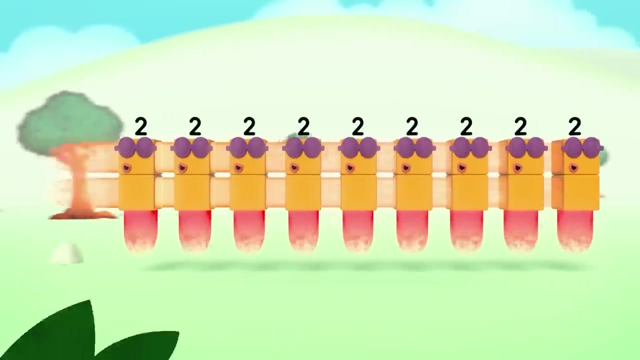 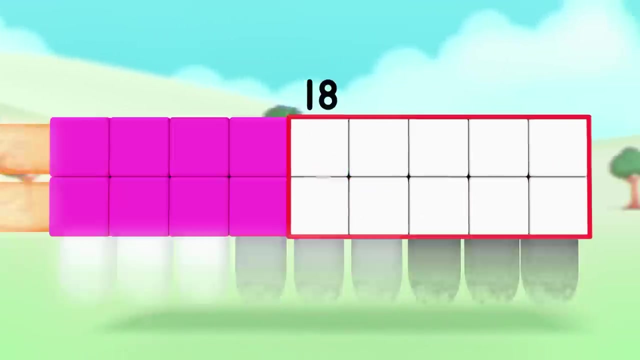 I can set the world. I'm blaze. Watch me zoom With a sonic boom. I was born to ride the race. Wahoo, Oh, Oh, 9, twos, Woo-hoo Ooh. 2,, 4,, 6,, 8,, 10,, 12,, 14,, 15,, 18!. 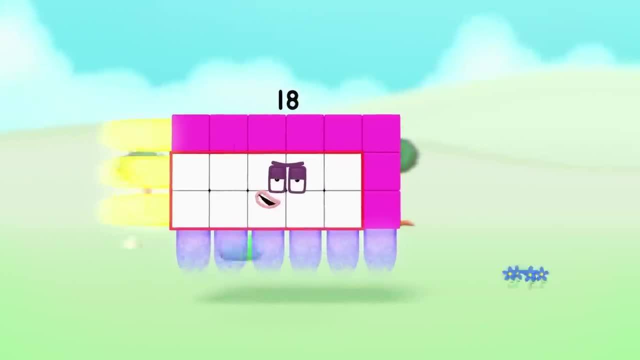 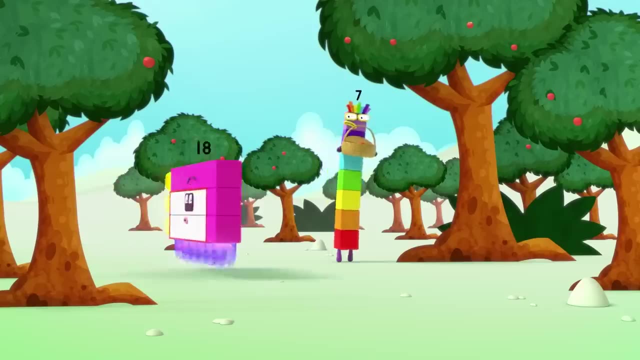 Switch 6 by 3!. 3 rays are what I need, 3 rays and I build up speed, I start to glow and I go, go, go, Whoa, Whoa, 6, threes, Yippee. 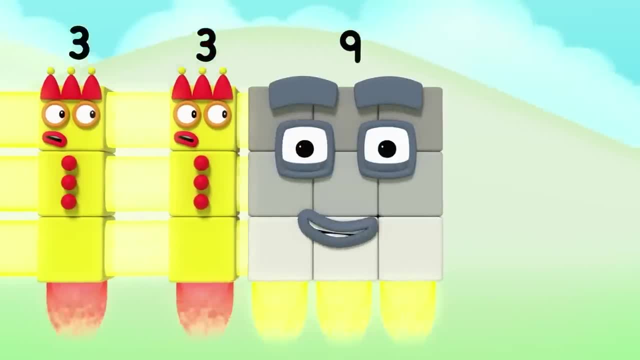 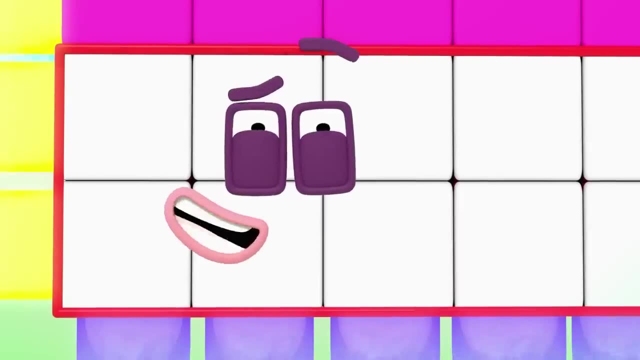 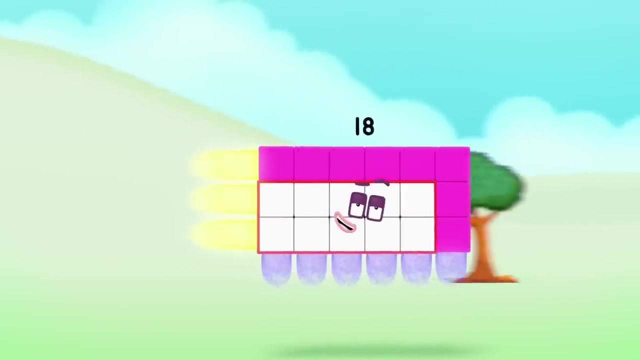 Too fast: 3,, 6,, 9,, 12,, 15,, 18! Cool time. When it comes to acceleration, I'm the undisputed master. I'm the quickest in the nation. I change shape when I want to go faster. 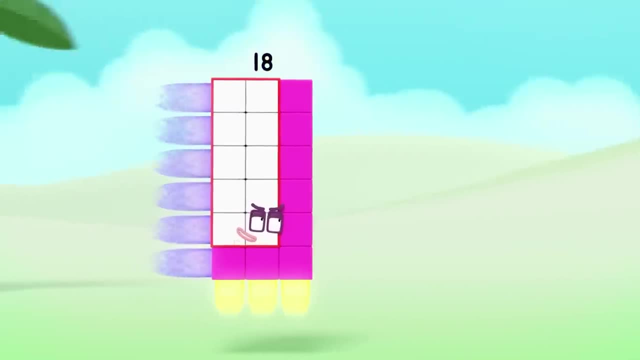 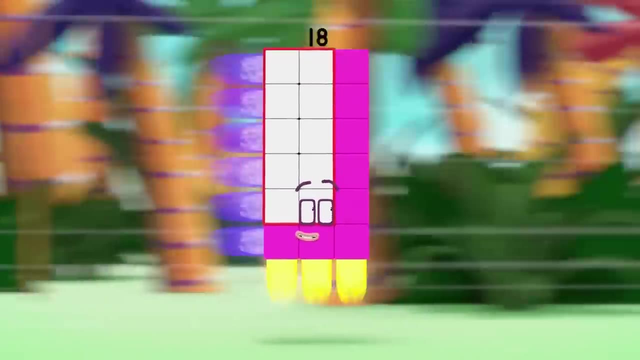 Time. 3 by 6!. 3 by 6!. 6 rays in a way. 1!. I'm 18!. I'm a speed machine. I can set the world ablaze. Watch me zoom With a sonic boom. 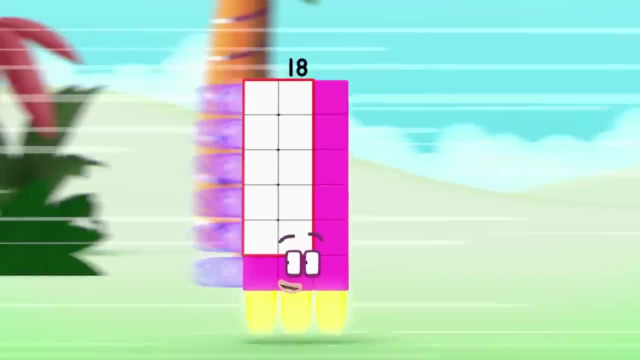 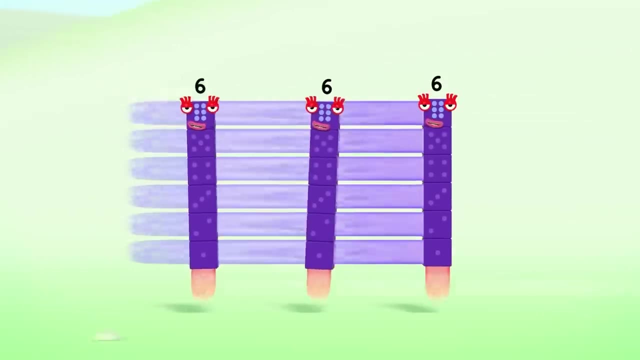 I was born to ride the race. Hey Woo, Whoa, Yeah, 3 sixes, Let's remix this. We're coming past, We're going too fast. Yikes, 6!, 12!, 8!, 9!. 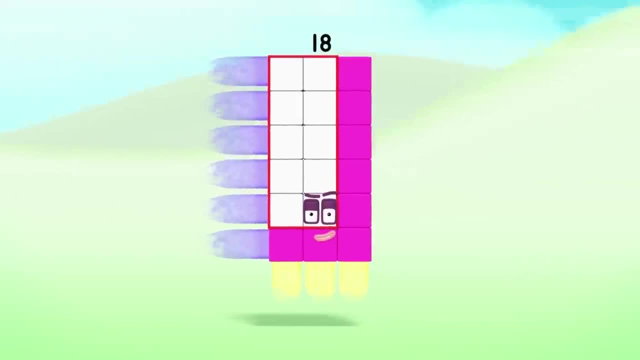 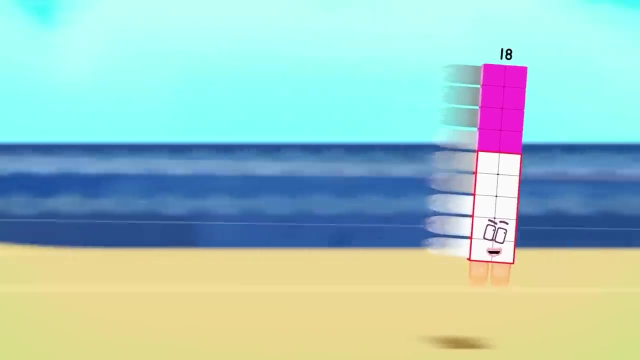 12!, 18!. Me again: Switch 2 by 9!. 9 rays are what I need, 9 rays, and I build up speed. I start to glow and I go, go, go, Ah, 3,, 5,, 4!. 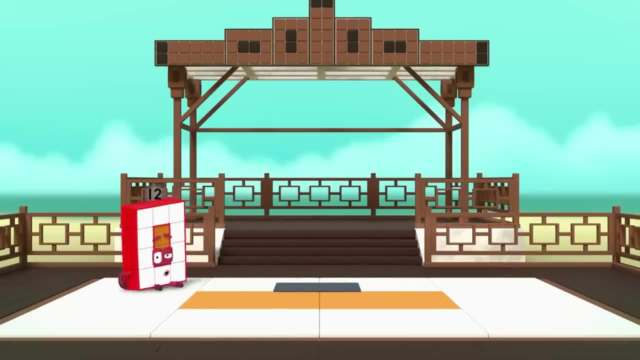 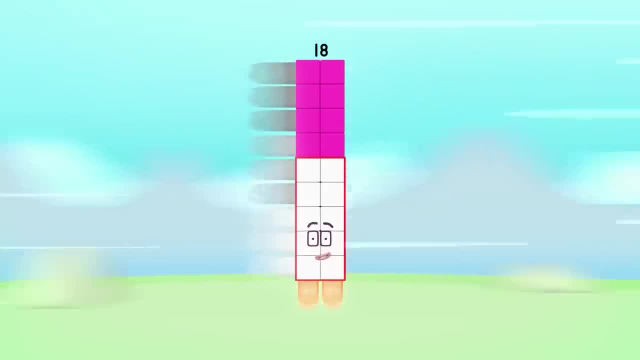 Whoa, Whoa, Whoa, Whoa. Ah. 2, nines Parallel lines, Whoa, 9!, 18!. Did you miss me? When it comes to acceleration, I'm the undisputed master. I'm the quickest in the nation. 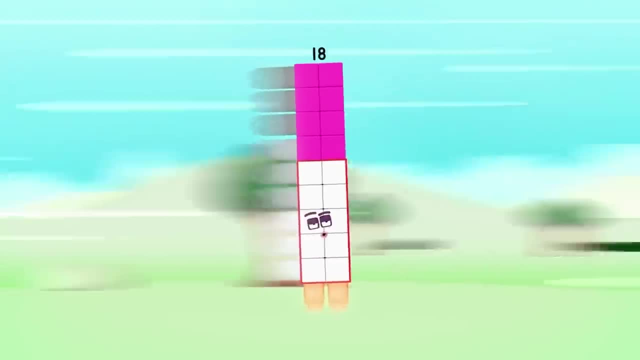 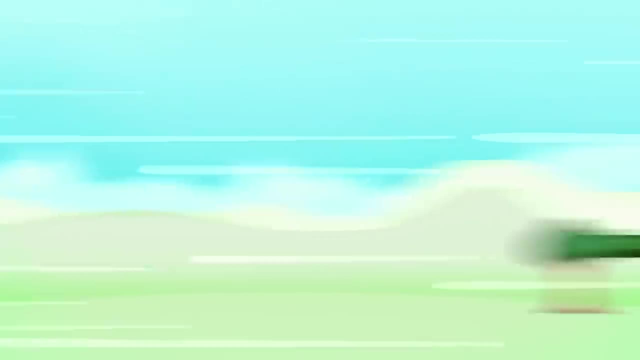 I change shape when I want to go faster, Ready for the big one. Switch 1 by 18!. 18 rays and away. I'm so fast I'll be out of the gate before you can lock it. I go at a rate no one can clock it. 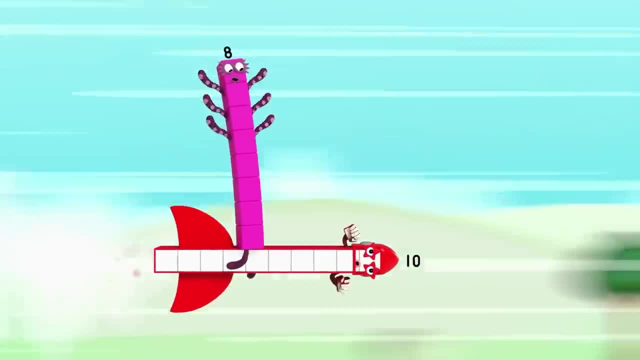 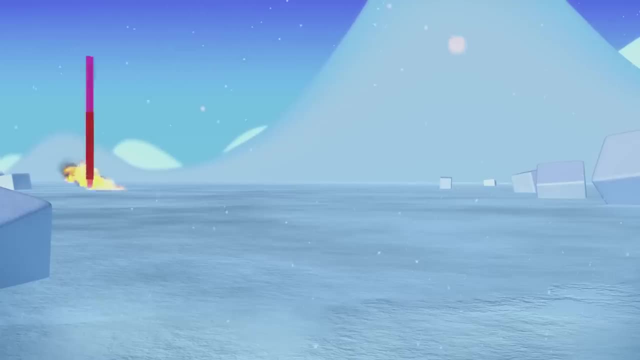 I'm 10 and 8!. I'm never late. I'm Foxes, Locker and Rockets. Yee-haw, Yee-haw, I'm 18!. I'm a speed machine. I can set the world ablaze. 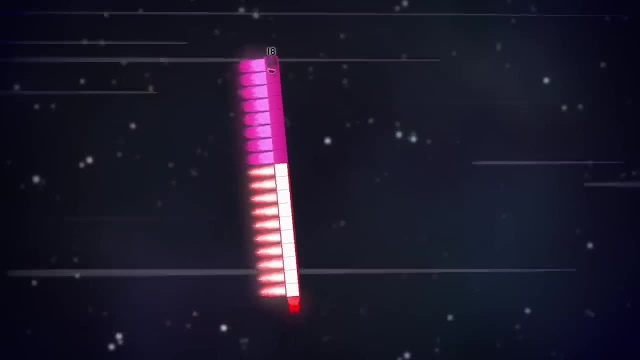 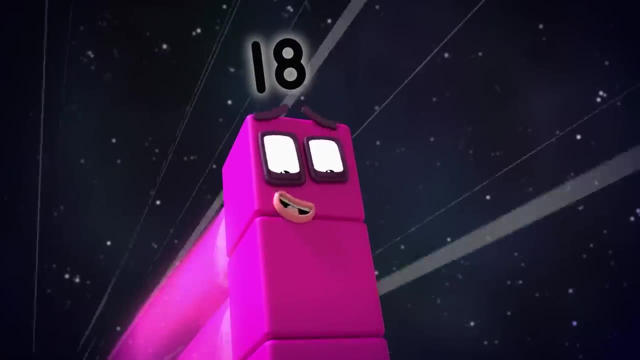 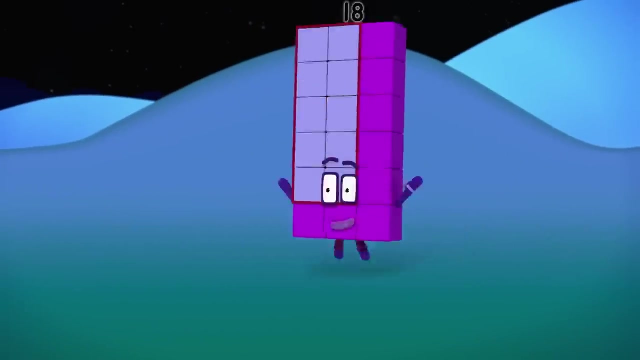 Watch me zoom with a sonic boom. I was born to ride the rays round the world. Whoa, Whoa. Um, how do I stop this thing? Ah, Blam, Woo-hoo. Oh, That's one way to do it. 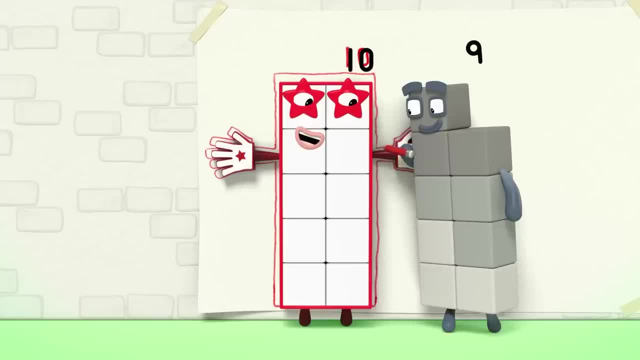 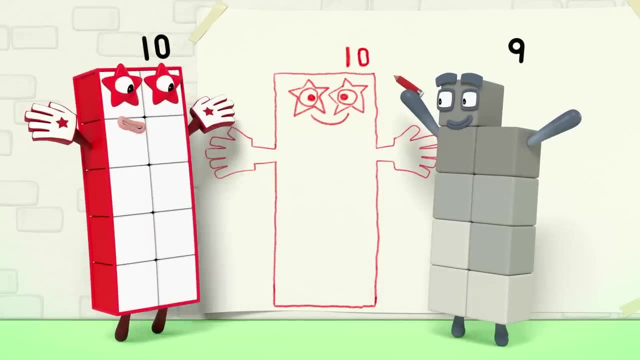 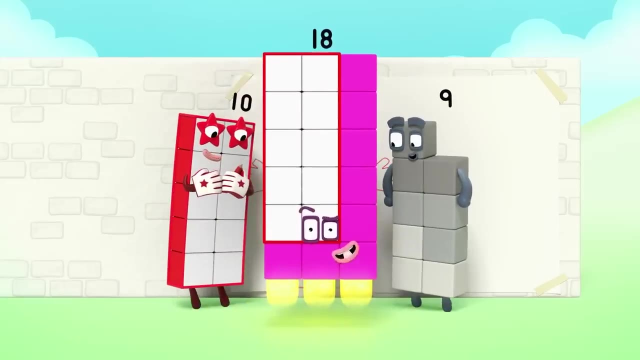 Blah Refresh. Hmm, Hmm, Hmm, Hmm, Hmm, Oh, Oh, Ta-da, I love it, My turn. Ha-ha, Ha-ha, Hmm, Hmm, Super Rectangle, Ha-ha, Whoa. 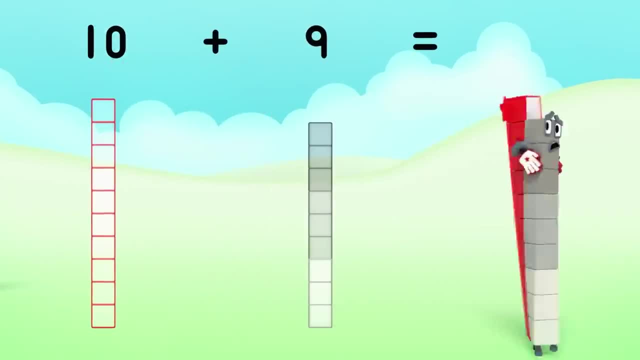 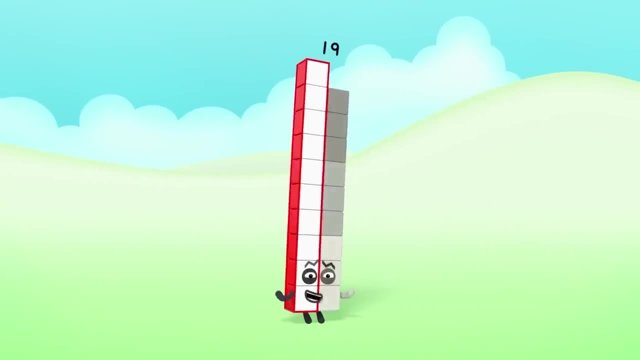 Whoa, 10 plus 9 equals 19!, Woo-hoo. Ah, All right then I am 19! And I, Who am I? Oh, Maybe it's something to do with Super Rectangle, Ha-ha. 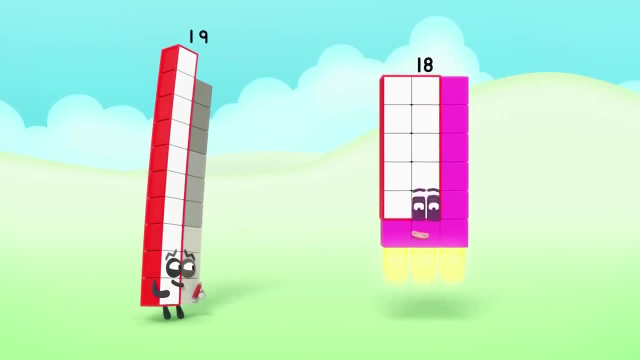 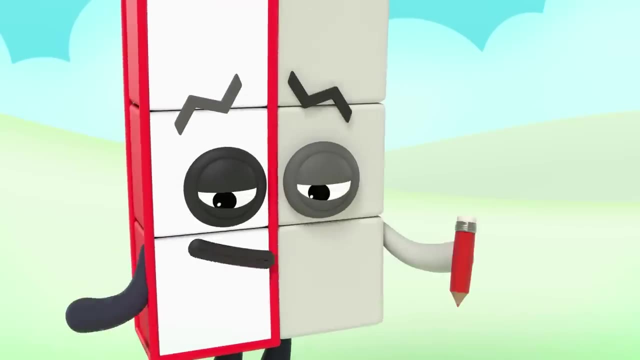 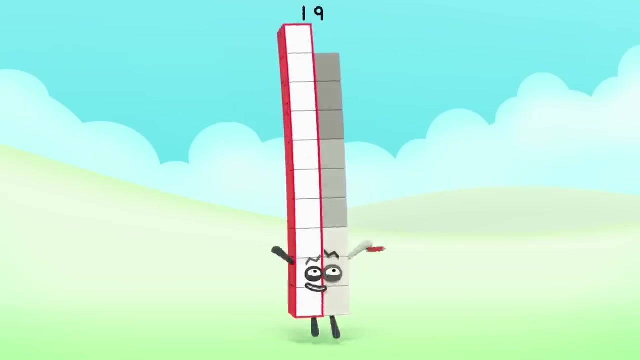 Switch, Switch, Turn. See ya, Meow Ooh, Maybe I can make lots of rectangles, Right, Let's do this Two by Oh, Oh, silly me, One block missing. Oh, Oh, Oh, Oh. 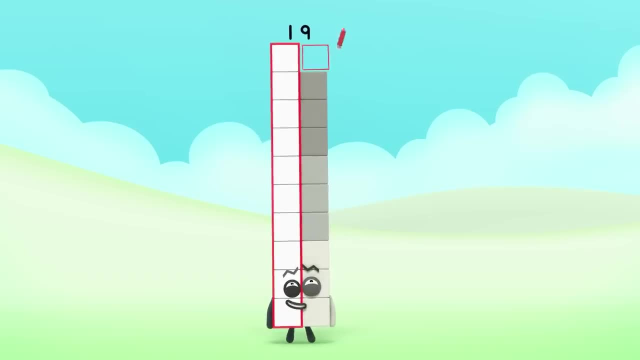 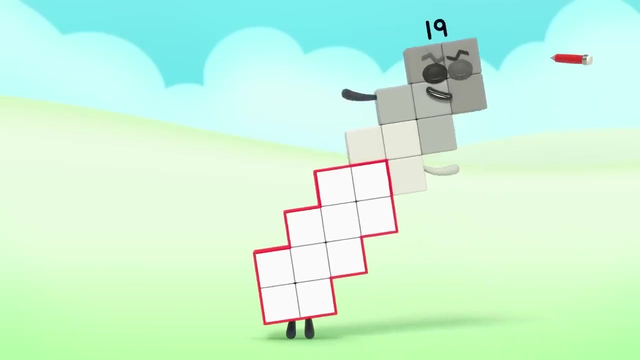 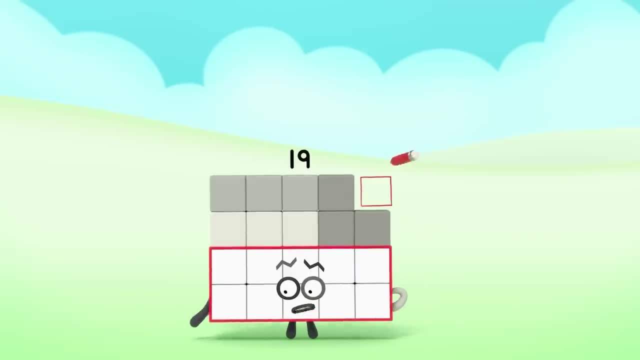 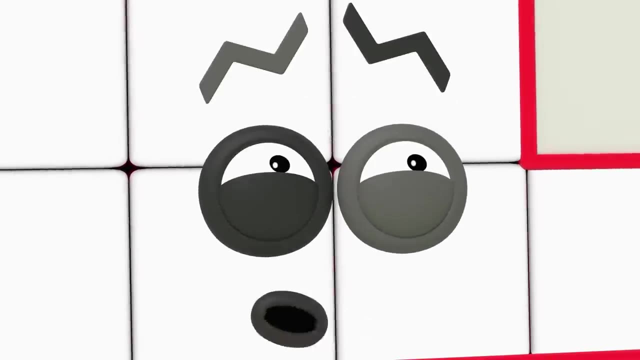 Concentrate. Oh, I can't do it. Oh, I'll never be a super rectangle, I'm just a silly old teapot. I mean elephant, I mean like, I mean monster. 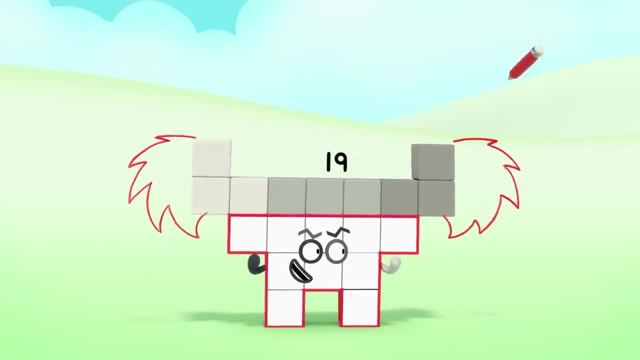 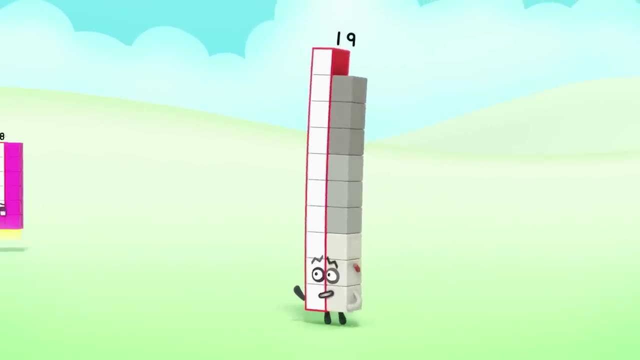 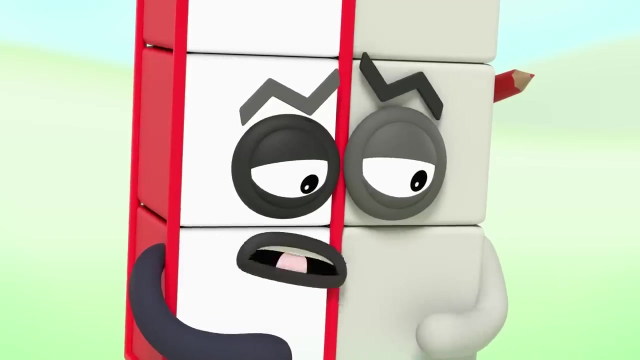 Super rectangle. I wish I could be like 18.. Make 18.. Make 18.. I wish I could be like 18.. Make everyday shapes with neat, straight lines. But there's always something not quite right, So I make crazy shapes. 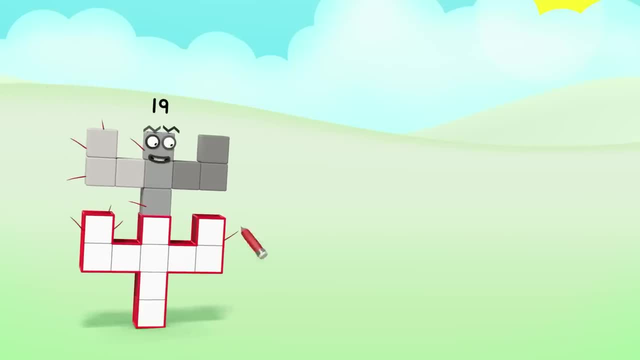 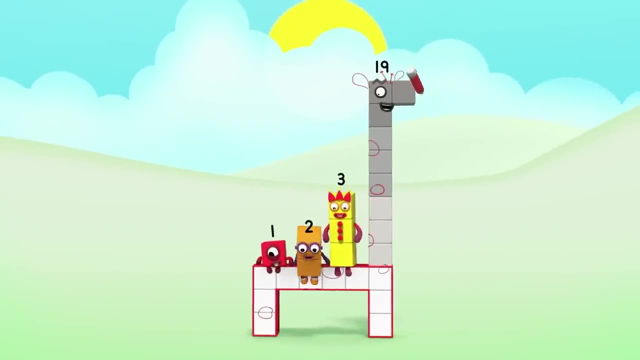 That's where 19 shines. I can be a cactus in the desert, An umbrella when it rains, Oh. I can stretch right out to make a tall giraffe- Oh, thanks. And if you need some building blocks, I can make a crane. 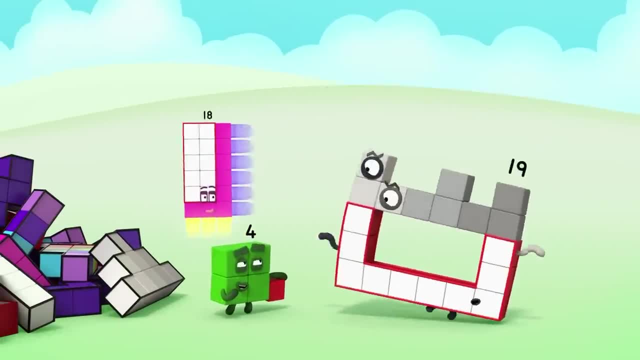 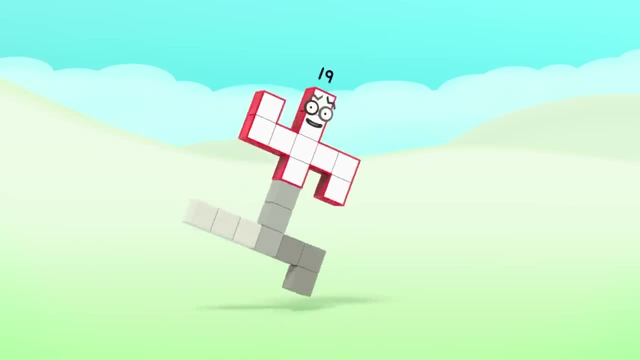 And make lots of funny faces to make you laugh, Cos. I make crazy shapes. Crazy shapes are what I do: Thingamabobs and whatsits and whatchamacallits too. I can make most anything. So put me to the test. 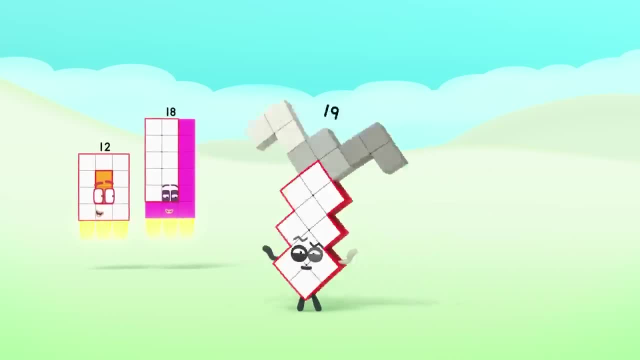 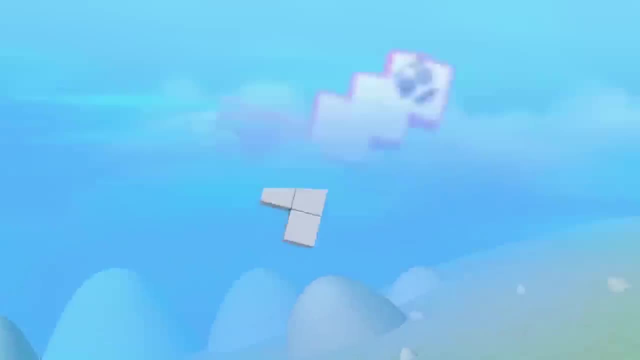 Crazy shapes. crazy shapes are the thing that I do best. Oh, I can make a table. Crazy shapes are the thing that you can eat at, Or a funny kind of fish When you're digging. I can make a garden spade. 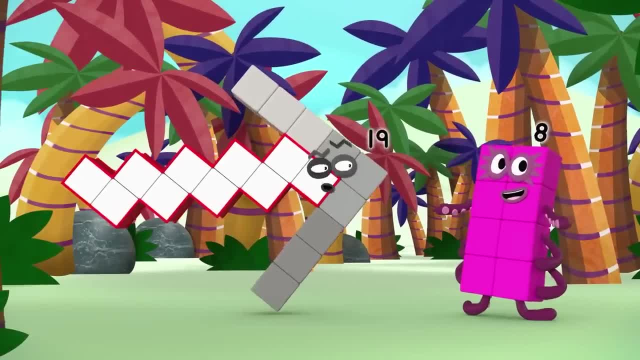 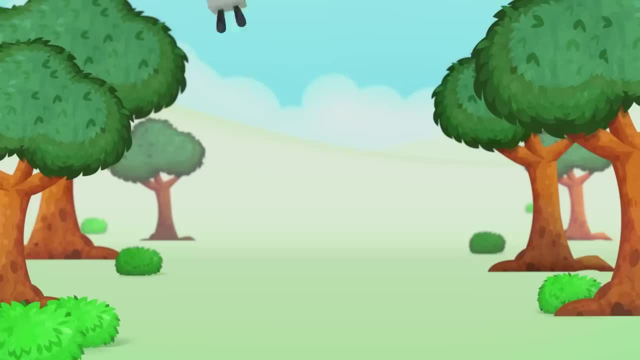 When you're lost, I'll give directions with an arrow if you wish. When it comes to making wacky shapes, I've got it made Cos I make crazy shapes. Crazy shapes are what I do: Thingamabobs and whatsits and whatchamacallits too. 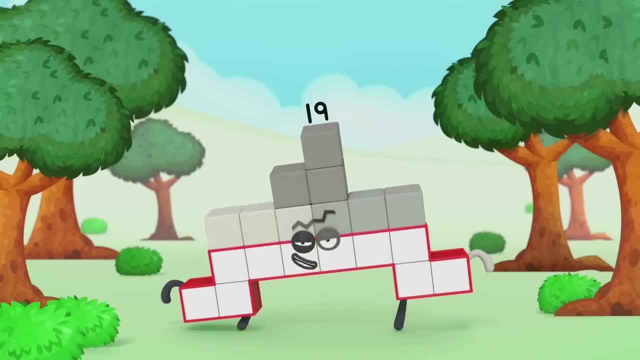 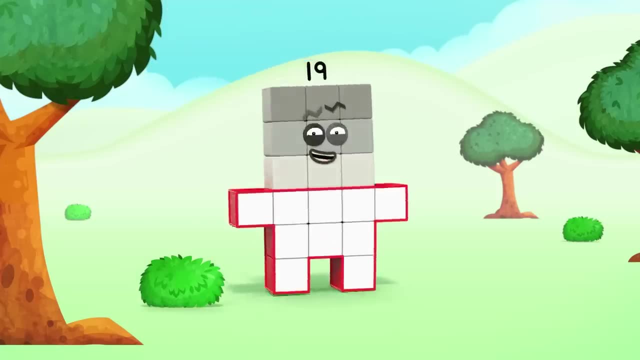 I can make most anything, So put me to the test: Crazy shapes. crazy shapes are the thing that I do best. Oops, I'm a one-off. I'm unique, As I'm sure that you'll agree. I'm a one-off. 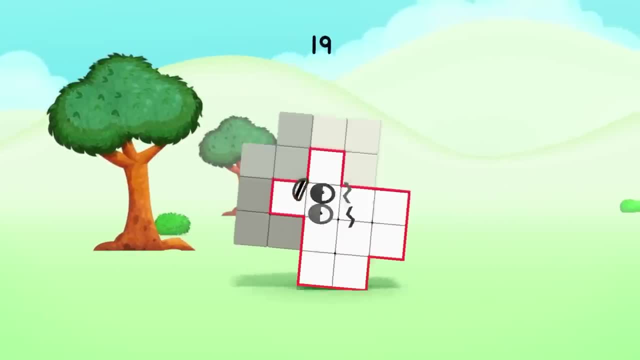 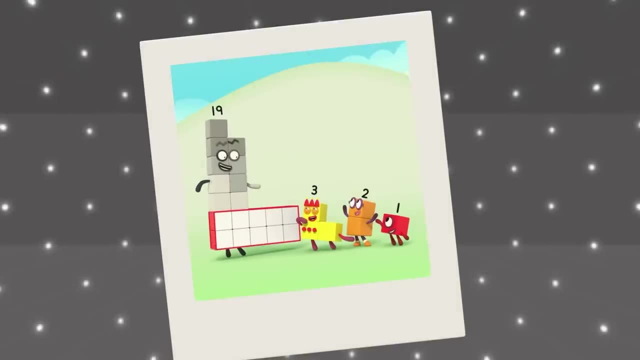 I'm at my peak. No-one's better at being me than me. Come on, everyone throw some shapes with me, Cos I make crazy shapes. Crazy shapes are what I do: Thingamabobs and whatsits and whatchamacallits too. 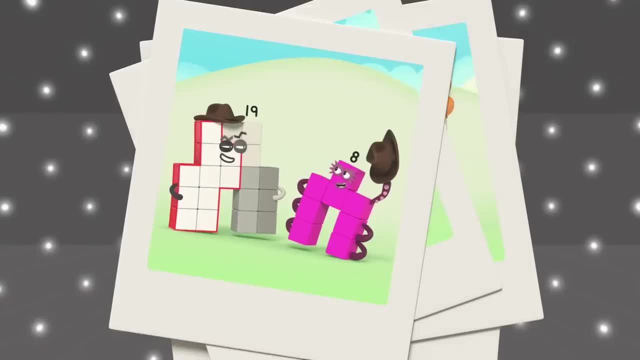 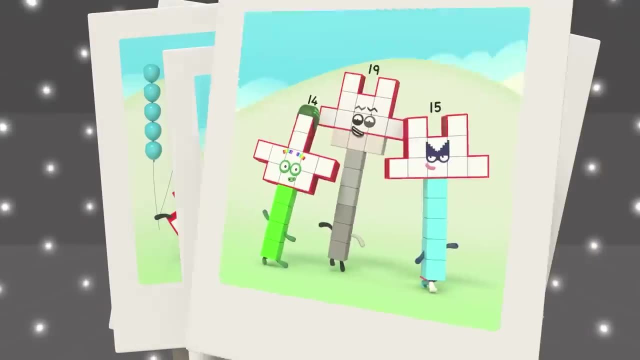 Thingamabobs and whatsits and whatchamacallits too. I can make most anything, So put me to the test. Crazy shapes, crazy shapes are the thing that I do best. Crazy shapes, crazy shapes are the thing that I do best. 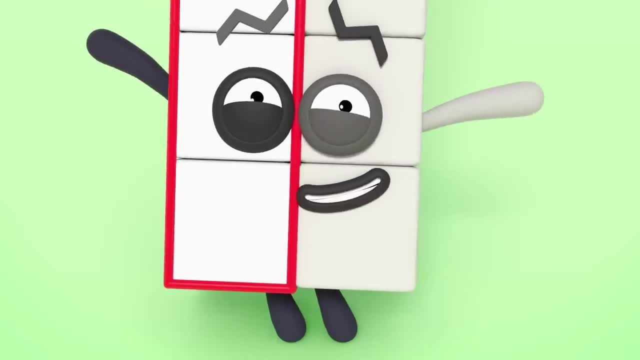 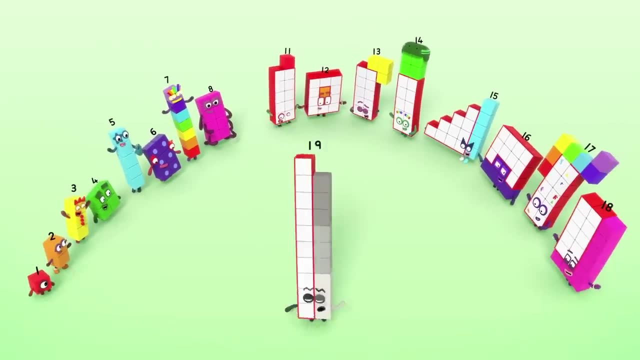 I am 19. And I am a one-off And I love it. Ahh, Da-da-pa-da-pa-doo, Da-da-pa-da-pa-doo, Da-da-pa-da-pa-doo, Who wants to dance with me? 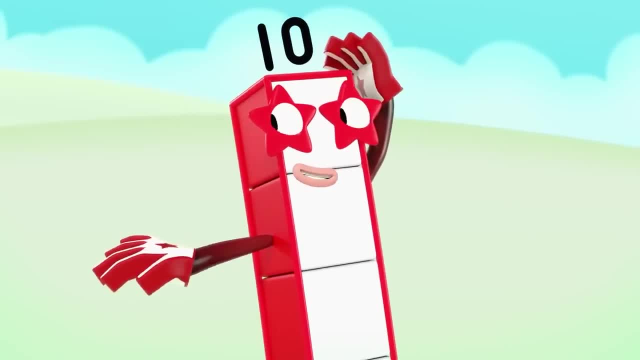 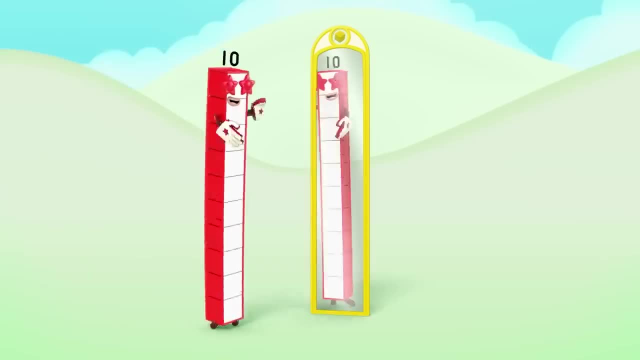 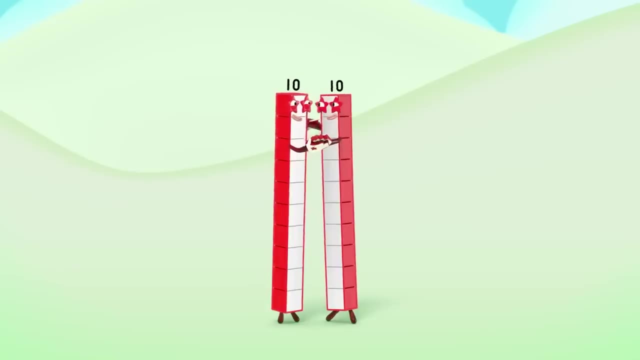 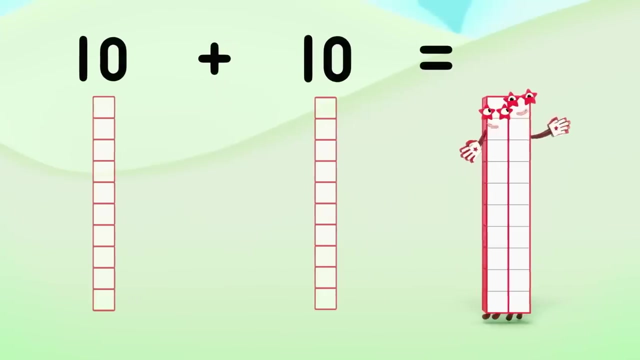 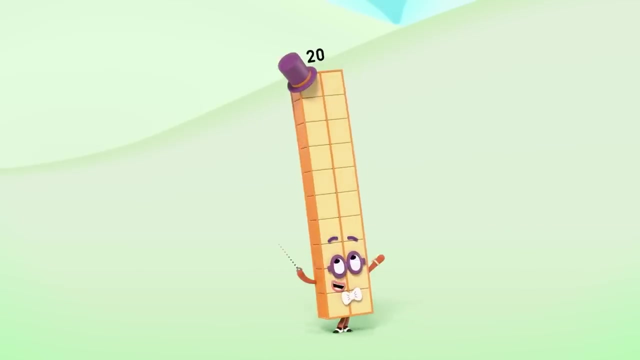 I know someone who wants to dance Me. Shall we dance Cha-cha-cha. Ten plus ten equals Four. Four, Ten plus ten equals Twenty. Hello, hello. Did somebody say Dance? I've got the shoes. 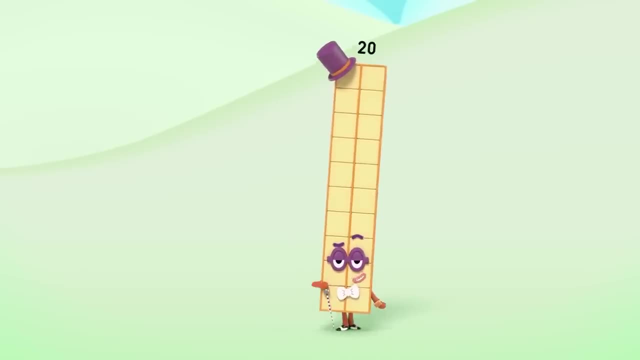 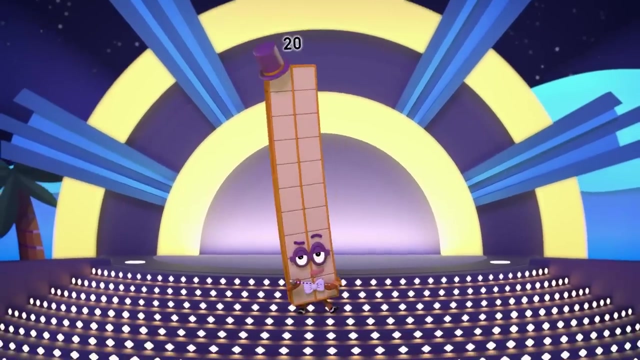 Tap, I've got the cane. Tap, I've got the tip Tap, Top, hat, Tap, tap, tap. Are you ready for the big dance number? That's me, I am twenty and I love to dance With plenty of moves to my name. 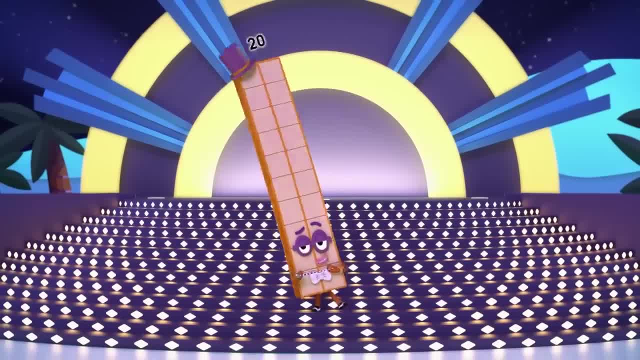 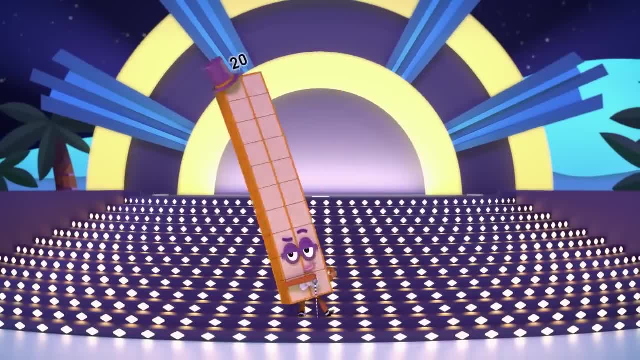 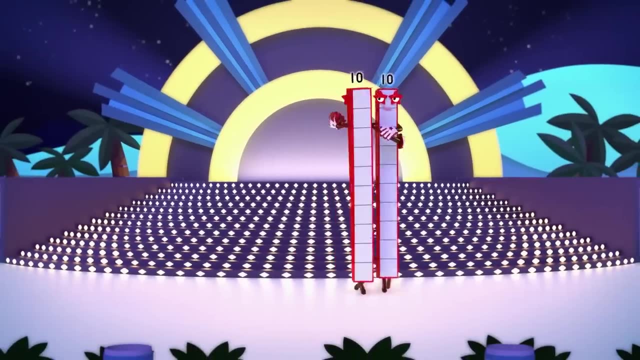 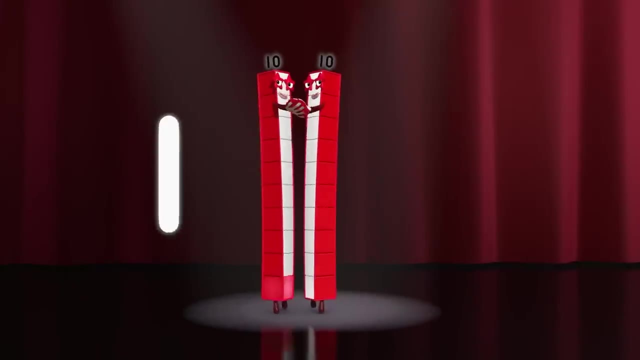 I'm tall and I'm slender, I'm graceful and tender. I sway as I do the fandango- Two tens, nothing more- As I take to the floor And dance to the two tens: tango One, two, three, four, five. 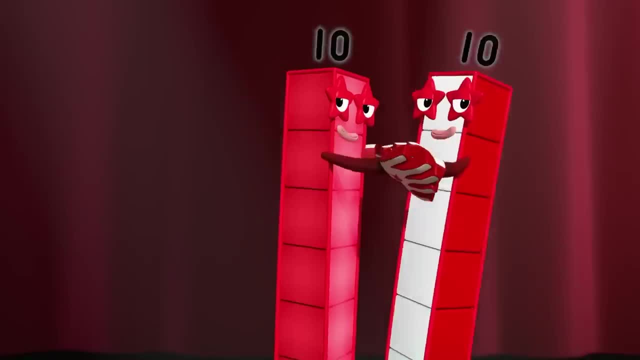 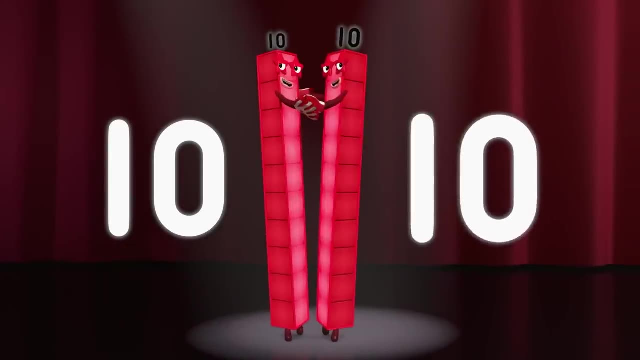 Six, seven, eight, nine, ten. Drop to the floor and go round again. One, two, three, four, five, Six, seven, eight, nine, ten. Two friends, two tens make twenty. One, two, three, four, five. 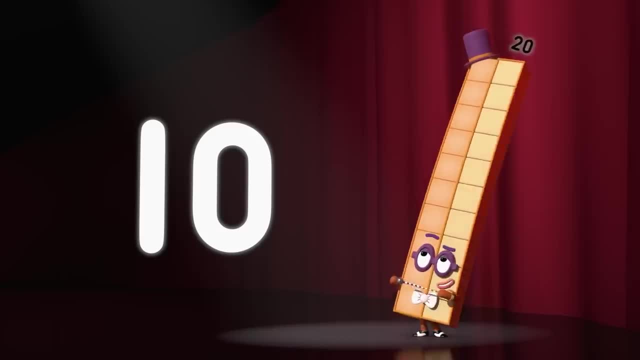 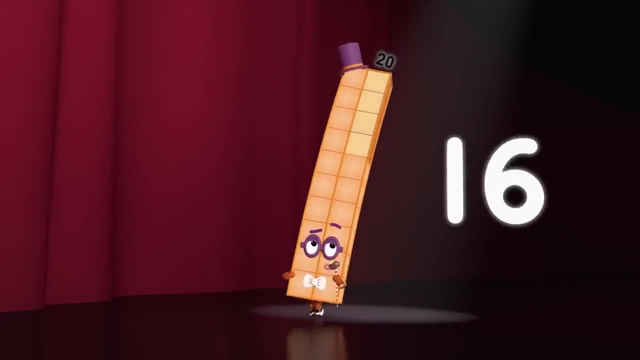 Six, seven, eight, nine, ten, Halfway to twenty. go round again: Eleven, twelve, thirteen, fourteen, fifteen, then Sixteen, seventeen, eighteen, nineteen, twenty, Sixteen, seventeen, eighteen, nineteen, twenty. 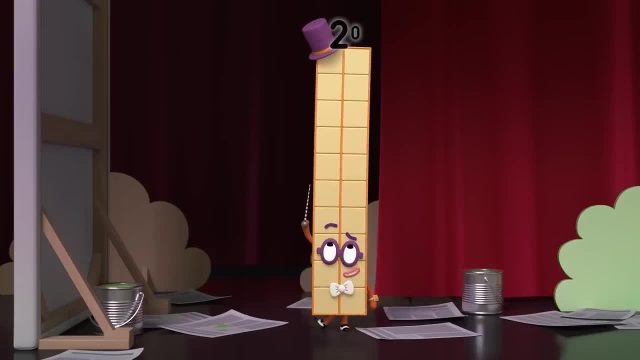 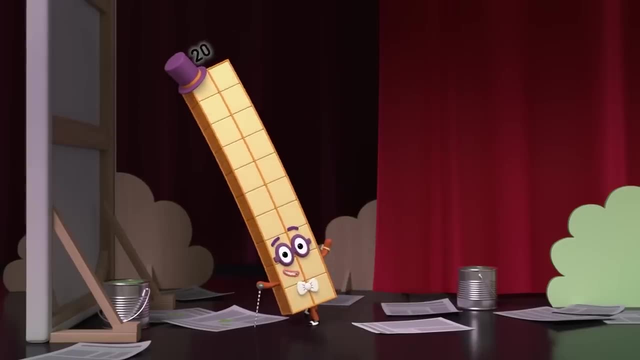 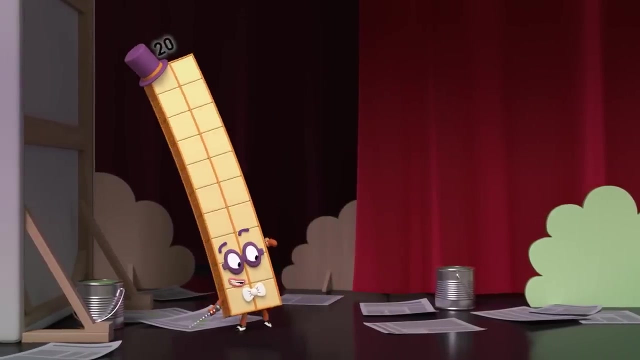 My two says I'm made of two tens, And who says I need any more, I say no more. That's how I'm created. I'm perfectly weighted To move to the beat of a mambo, And then, right on cue, I can split into two. 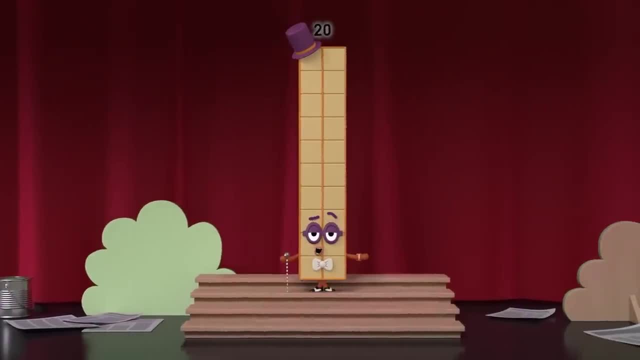 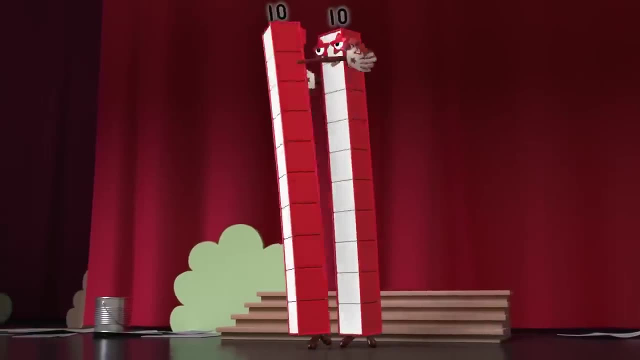 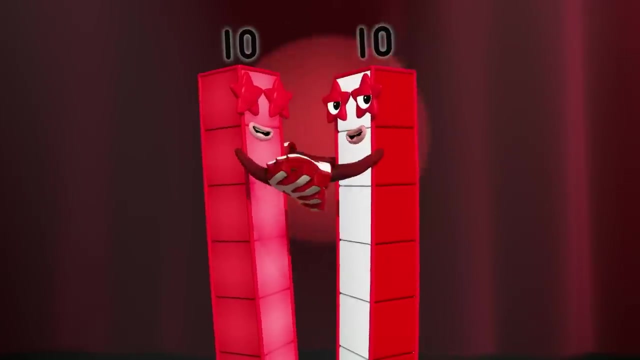 And dance to the two tens tango: One, two, three, four, five, Six, seven, eight, nine ten. Drop to the floor and go round again: One, two, three, four, five, Six, seven, eight, nine ten. 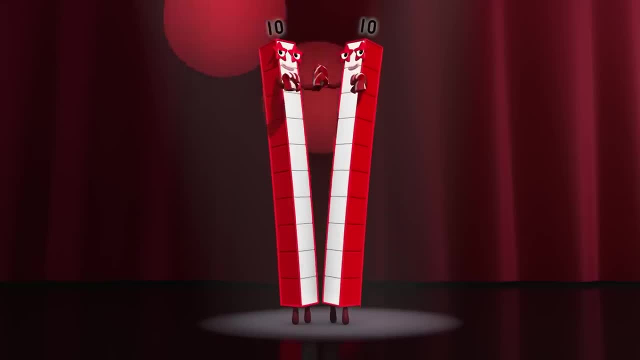 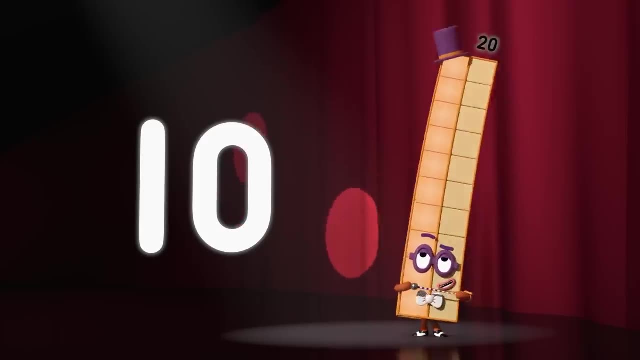 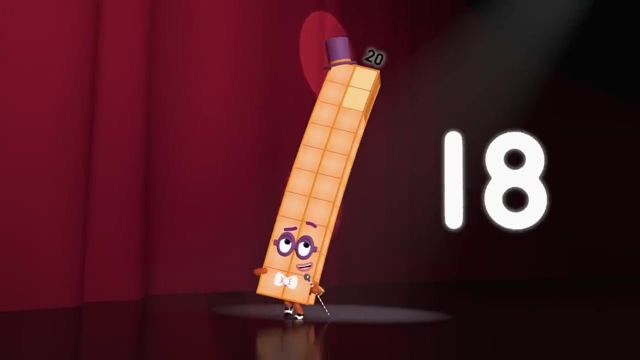 Two friends, two tens make twenty. One, two, three, four, five, Six, seven, eight, nine, ten, Halfway to twenty. go round again Eleven, twelve, thirteen, fourteen, fifteen, then Sixteen, seventeen, eighteen, nineteen, twenty. 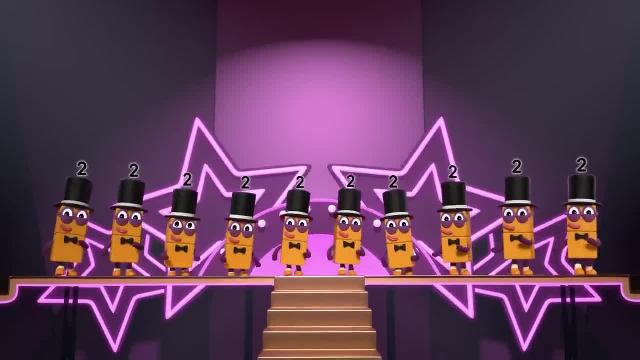 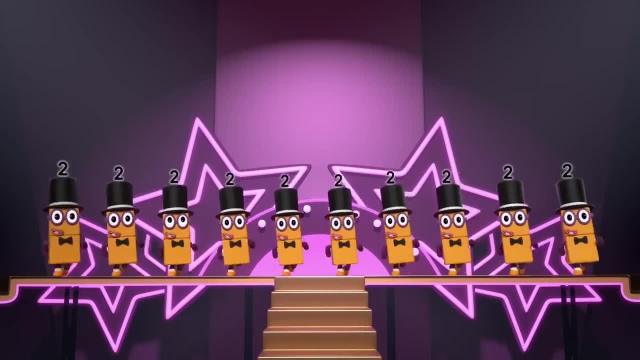 I have some more friends I'd like you to meet. It's the ten twos hot shoe shuffle. Ten of us twos in a row. It's the ten twos hot shoe shuffle. Welcome to the ten twos hot shoe show. 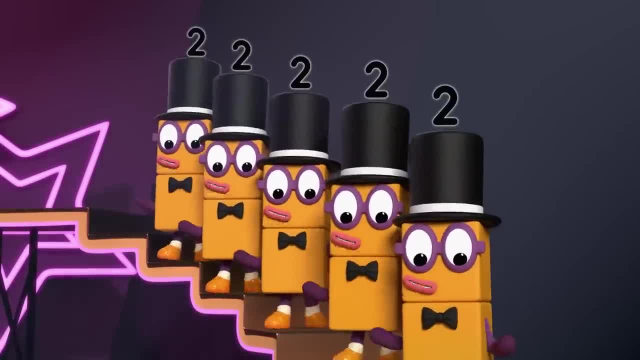 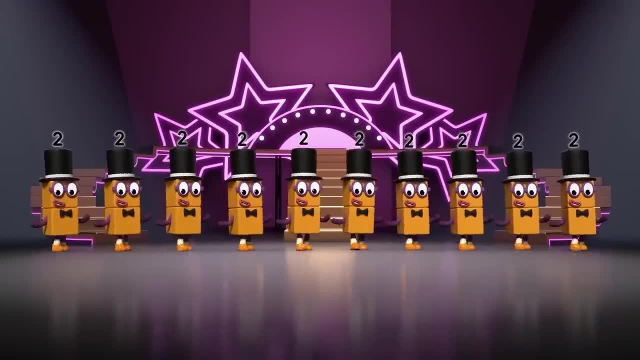 We can shuffle to the beat, so we shuffle our feet. People say your shuffling sure looks sweet. It's the ten twos hot shoe shuffle. Ten of us twos in a row. It's the ten twos hot shoe shuffle. 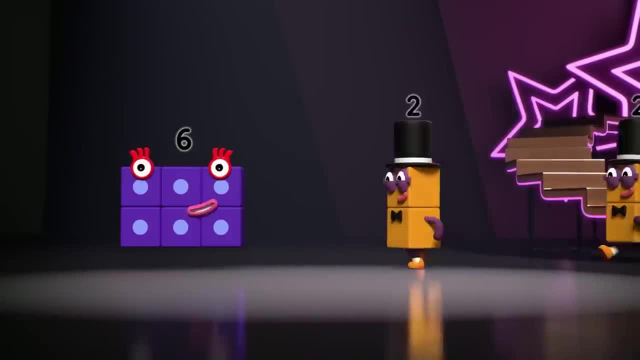 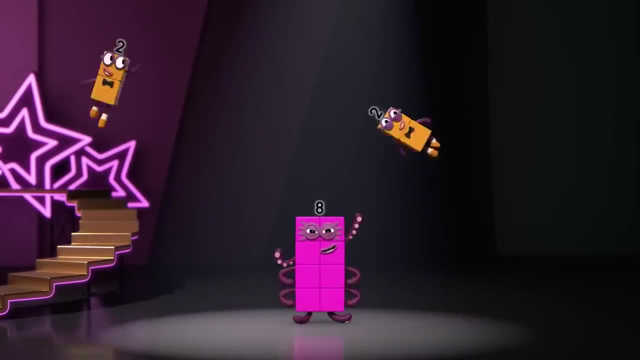 Five, five, and now it's time to go. Two, four, six, oh ten, twelve, fourteen, sixteen, eighteen, twenty. Two, four, six, oh ten, twelve, fourteen, sixteen, eighteen, twenty. 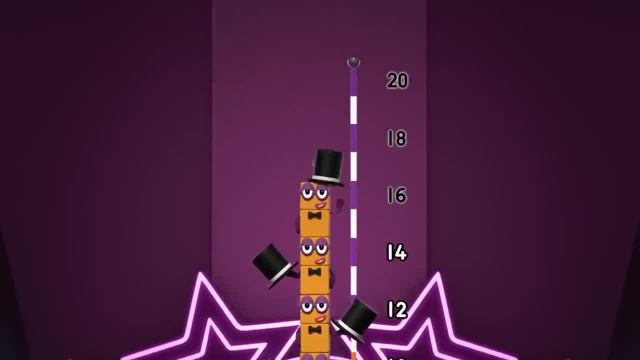 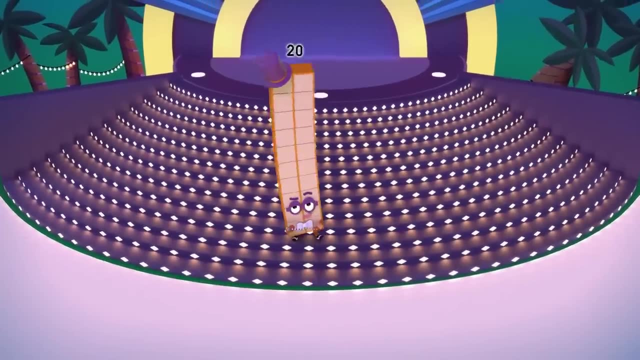 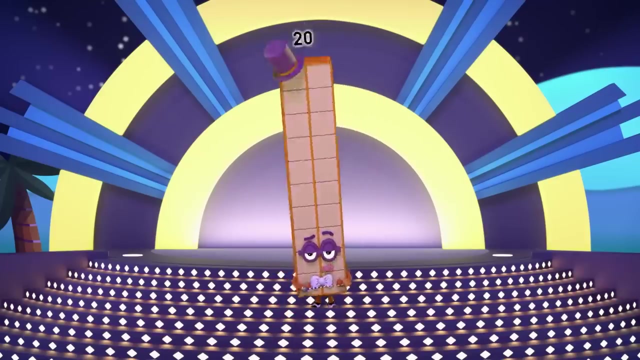 Two, four, six, eight, ten, twelve, fourteen, sixteen, eighteen, twenty. I'm twenty and I love to dance With plenty of moves to my name. I'm tall and I'm slender. I'm graceful and tender. 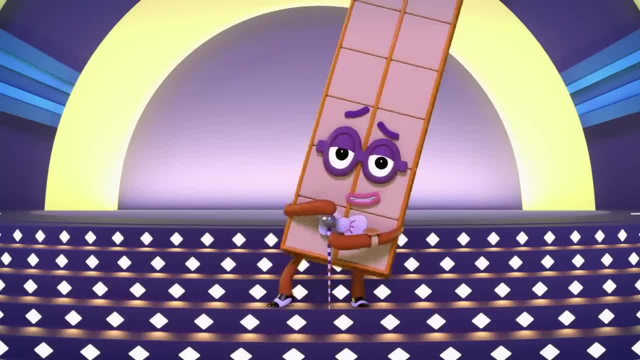 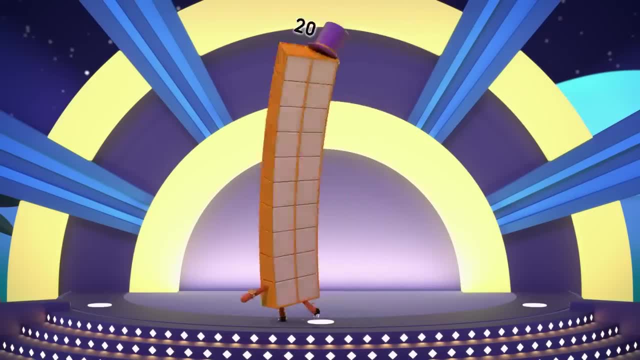 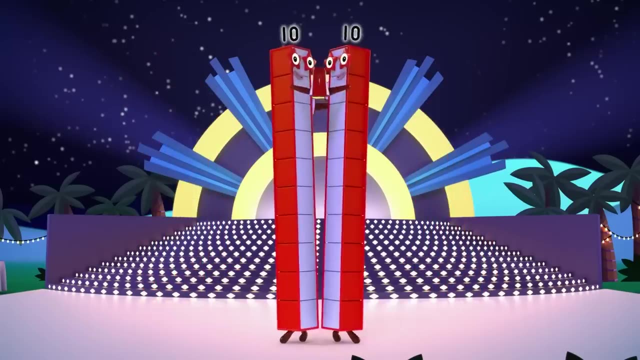 I sway as I do the fandango. Two tens, nothing more, as I take to the floor And dance to the two tens tango. Two tens, nothing more, as we take to the floor And dance to the two tens tango. Music. 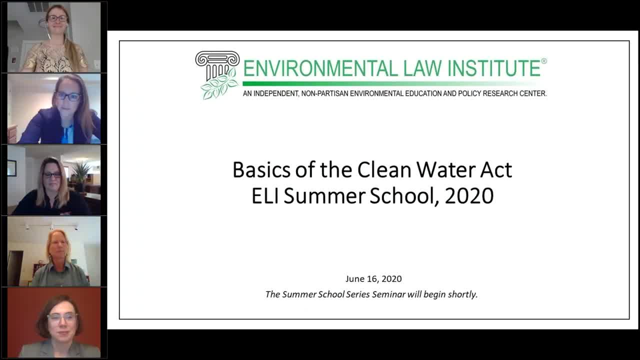 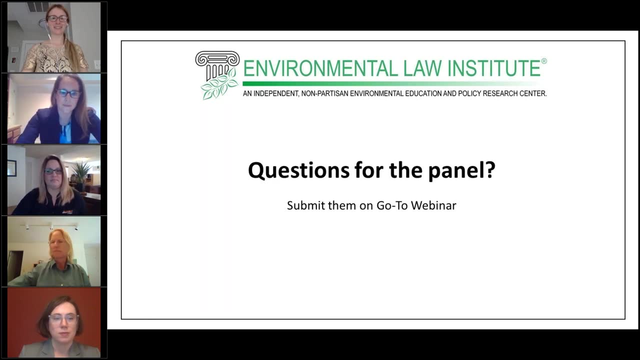 Good afternoon and welcome to the Environmental Law Institute. You have joined us for the basics of the Clean Water Act. My name is Kaitlin McCarthy and I'm the Director of Education Associates and Corporate Partnerships here at ELI. We are delighted to welcome everyone.